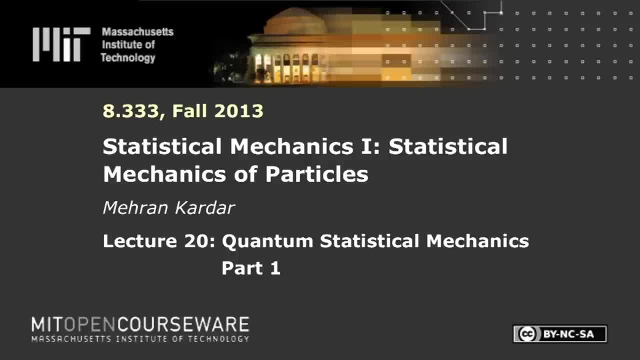 The following content is provided under a Creative Commons license. Your support will help MIT OpenCourseWare continue to offer high quality educational resources for free. To make a donation or view additional materials from hundreds of MIT courses, visit MIT OpenCourseWare at ocwmitedu. 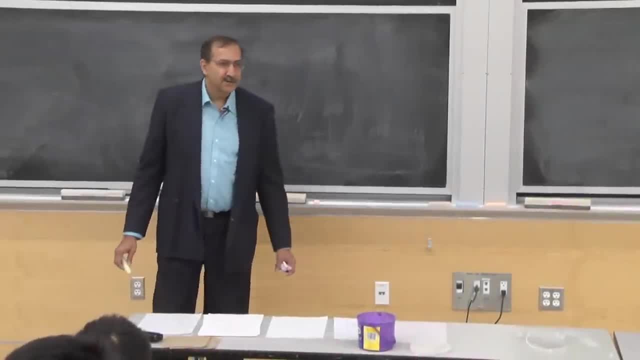 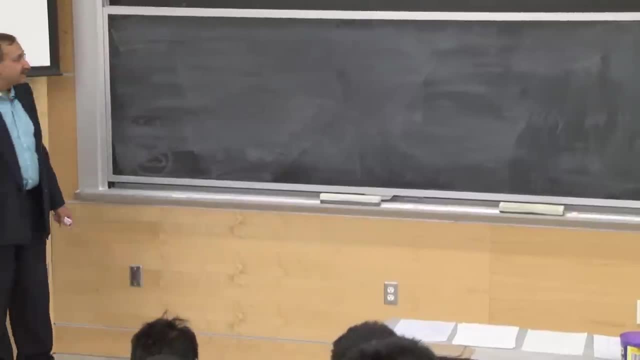 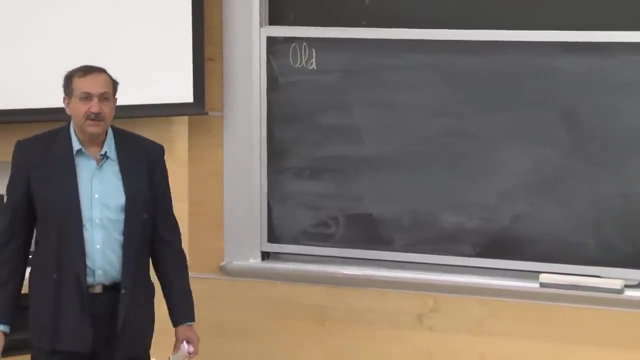 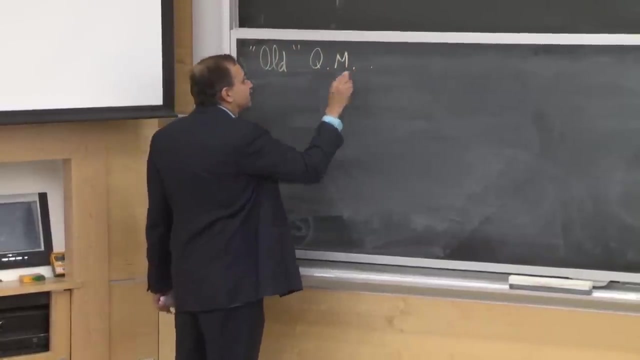 OK, let's start. So last lecture, what we talked about was limitations of classical statistical mechanics And what I will contrast with what I will talk about today, which is new version, the old version of quantum mechanics, which was based on the observation originally. 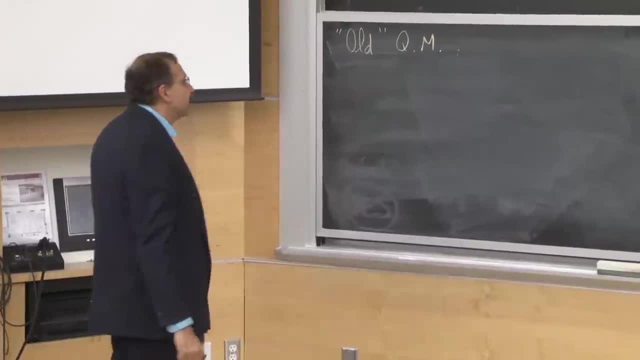 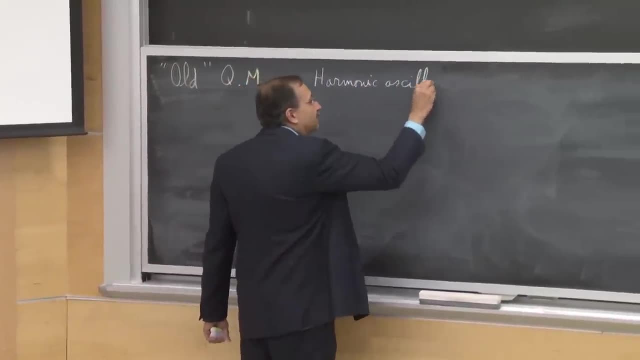 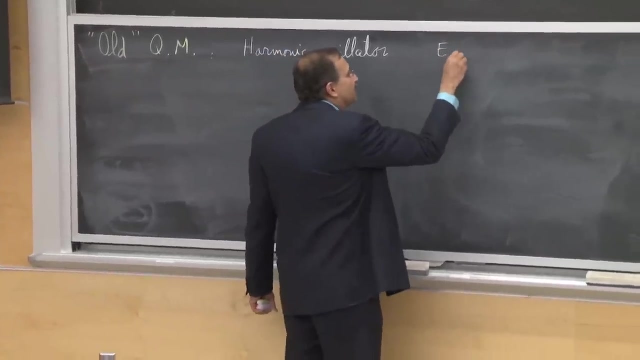 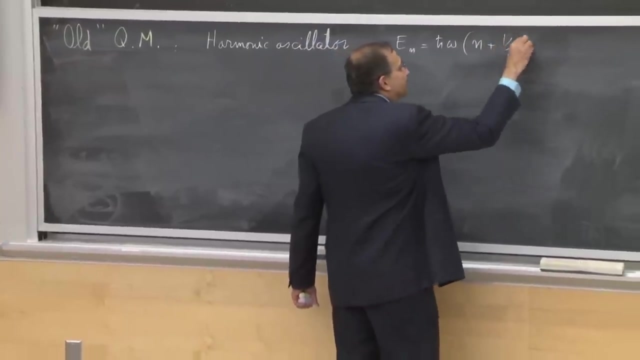 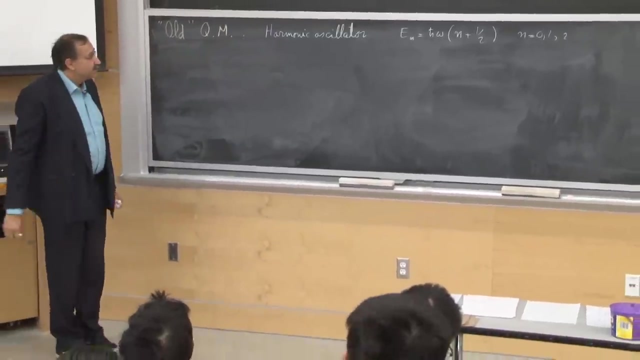 from Planck and then expanded by Einstein, that for a harmonic oscillator we have a frequency of frequency omega. The energies cannot take all values, but values that are multiples of the frequency of the oscillator and then some integer n. What we did with this observation? 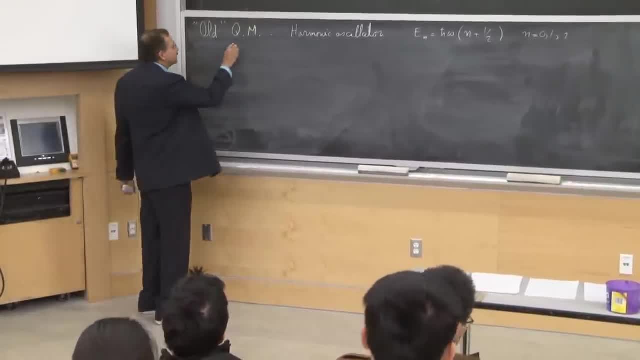 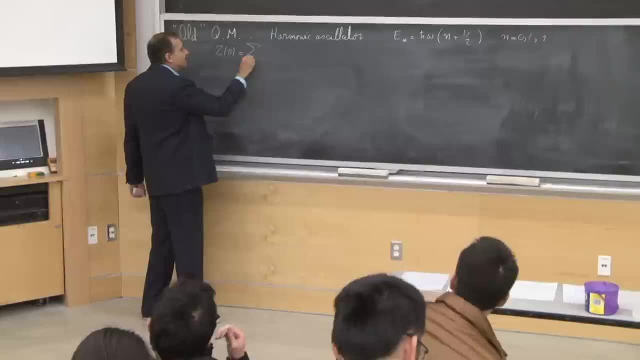 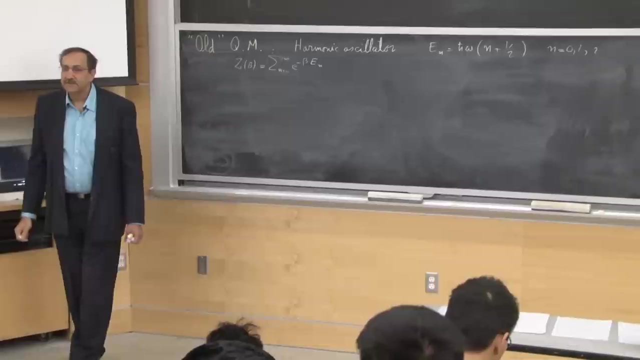 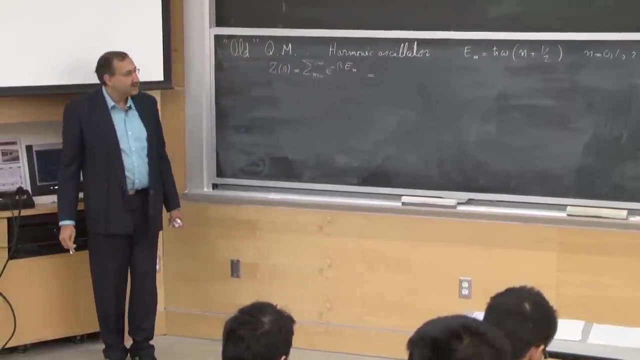 to extract thermal properties was to simply say that we will construct a partition function for the harmonic oscillator by summing over all of the states of e to the minus beta en, according to the formula given above. just thinking that these are allowed states of this oscillator. 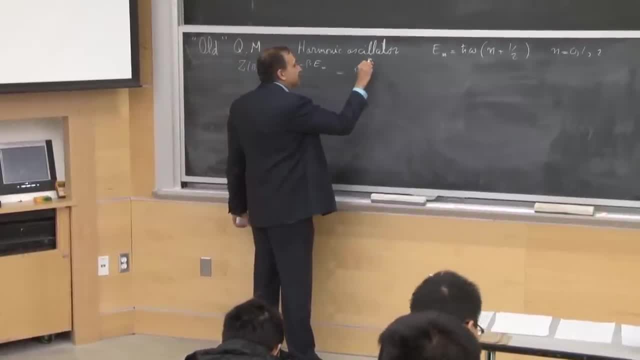 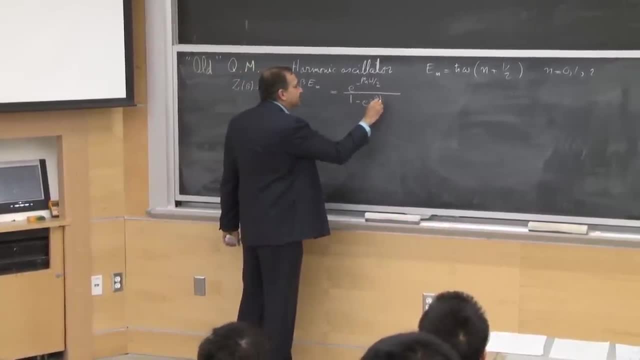 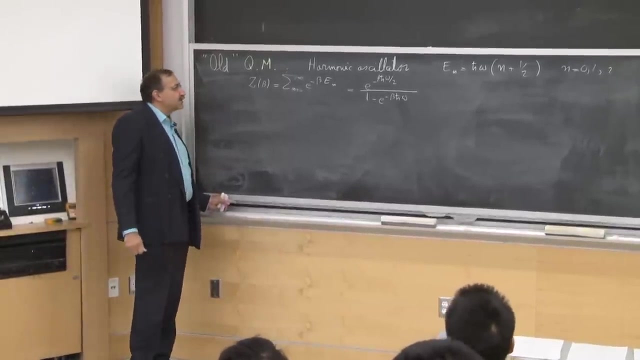 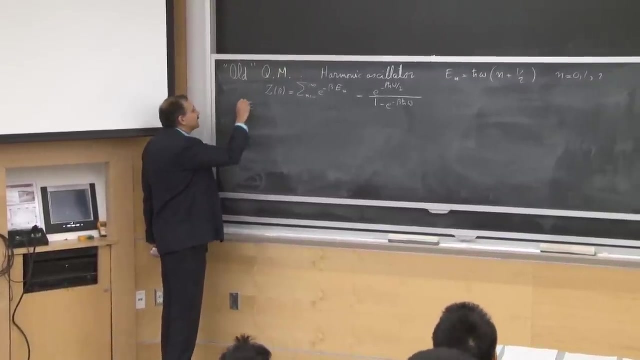 And this sum you can very easily do starts with the first term and then itself. This is the algebraic series which will give you that formula. Now, if you are sitting at some temperature, T you say that the average energy that you have in your system. 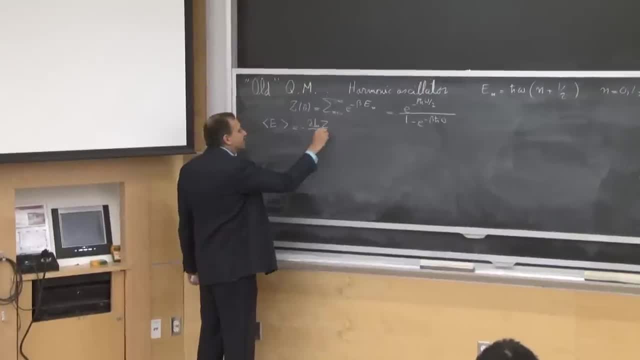 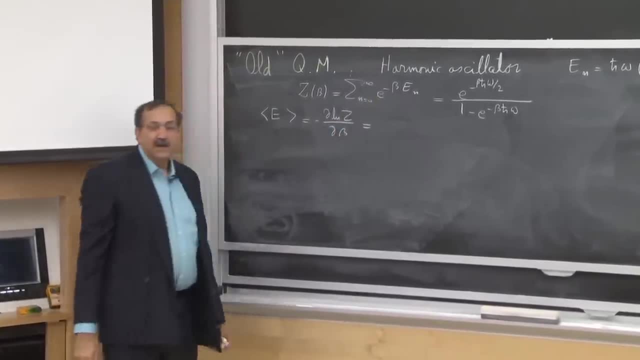 well, the formula that we had is minus d log z by d beta, which, if I apply to the z that I have above, essentially it's going to be minus d log z by d beta. So essentially it weighs each one of these Boltzmann weights. 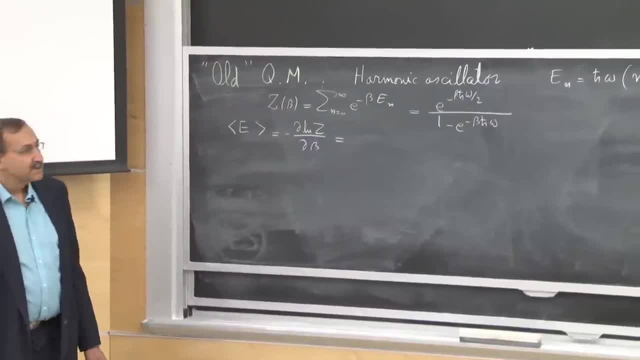 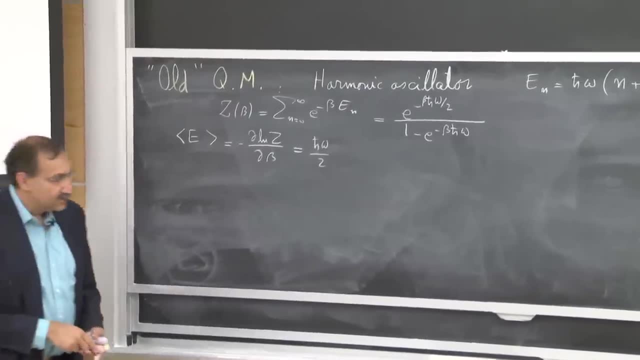 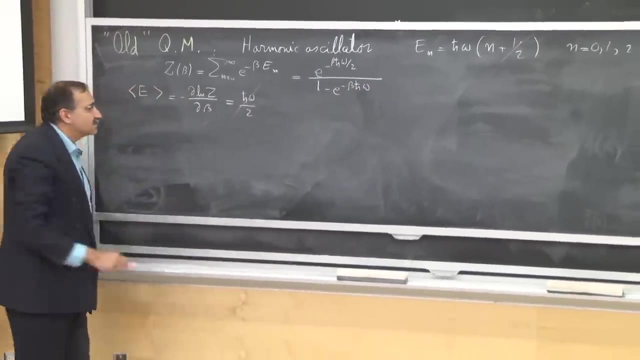 by the corresponding energy and sums them, What we do is we get essentially the contribution of the ground state. Actually, for our intents and purposes we can ignore this, and hence this. But for completion, let's have them around. And then, from what is in the denominator, if you take a 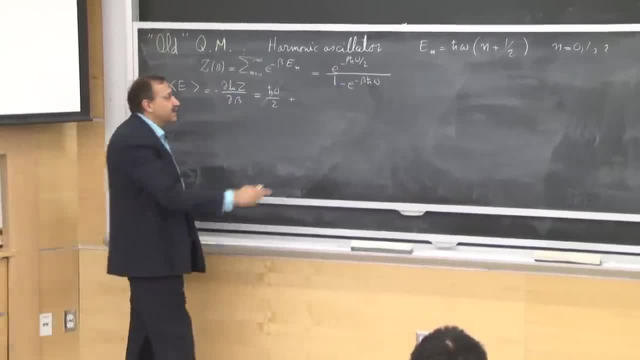 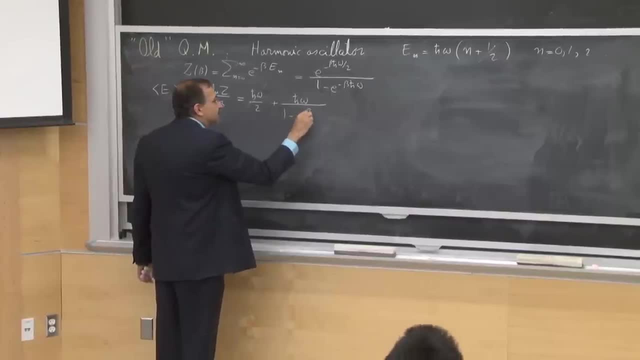 let's have them around. And then, from what is in the denominator, if you take a, the derivative with respect to beta, you will get a factor of h bar omega. And then this factor of 1 minus e to the minus beta h bar omega. 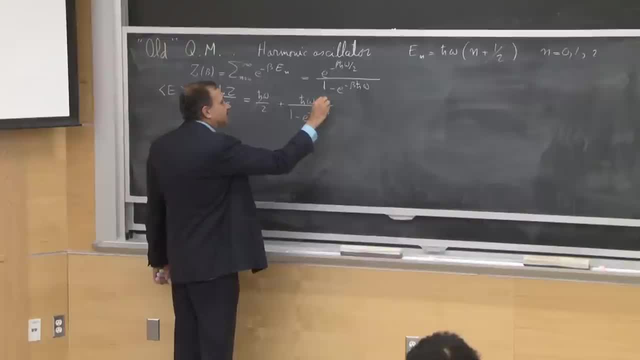 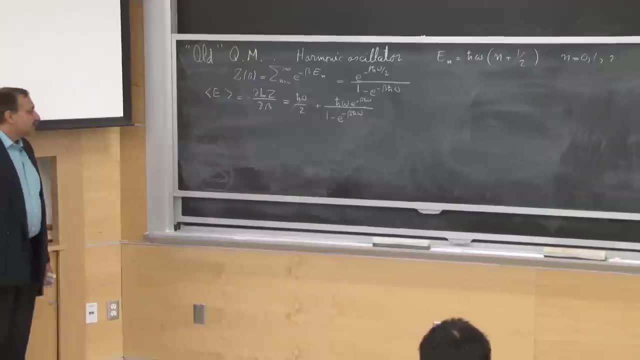 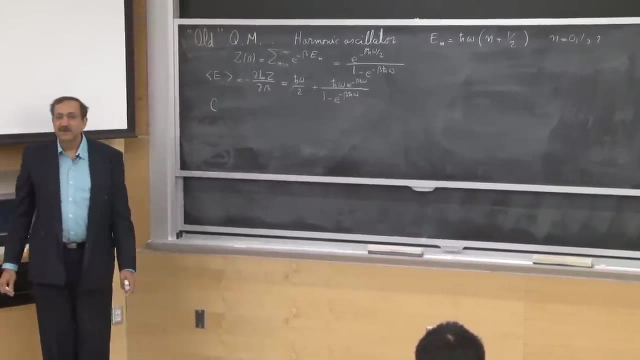 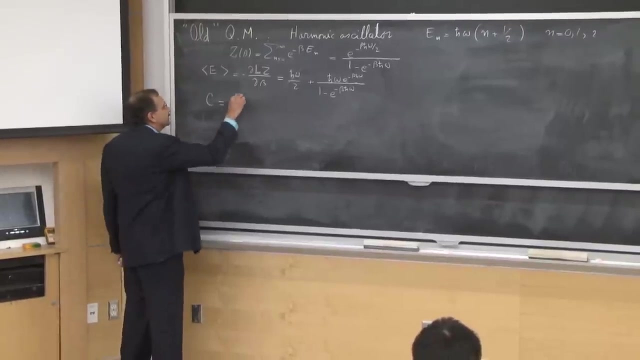 Actually with an additional e to the minus beta, h, bar, omega. Now the thing that we really compared to was what happens if we were to take one more derivative To see how much the heat capacity is that we have in a harmonic oscillator. 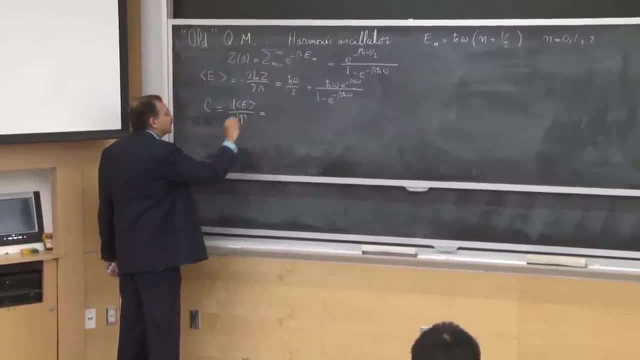 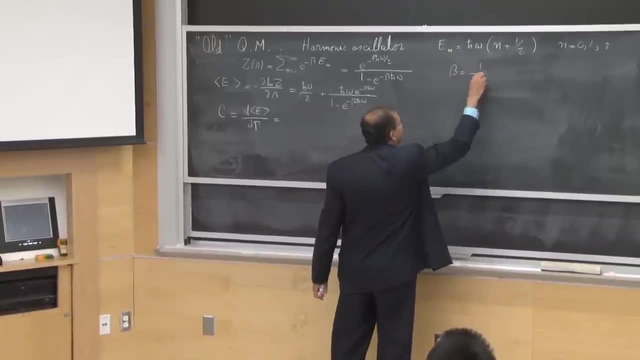 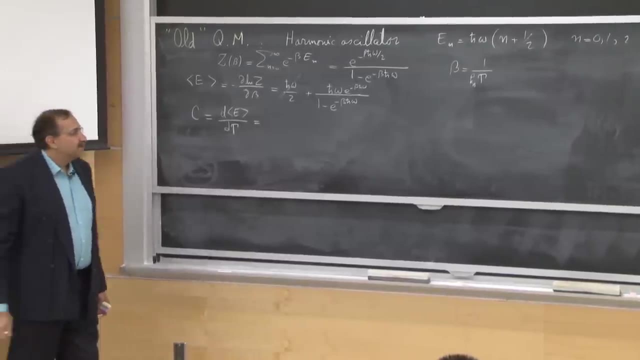 So, basically taking an average of the above formula with respect to temperature, realizing that these betas are inverse temperatures, So derivatives with respect to t will be related to derivative with respect to beta, except that I will get an additional factor of 1 over kbt. 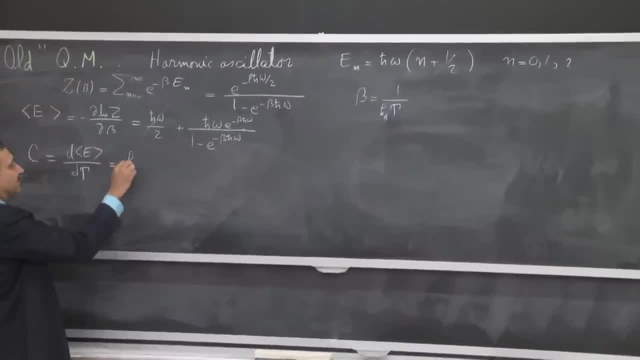 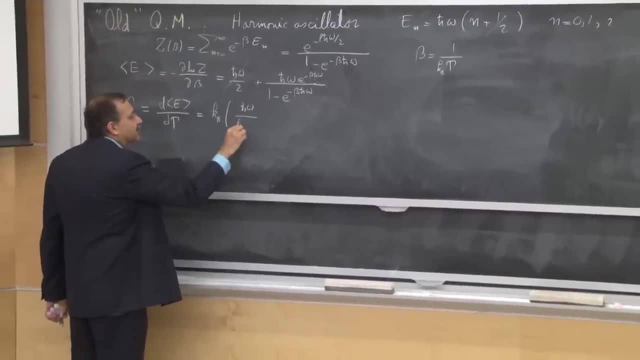 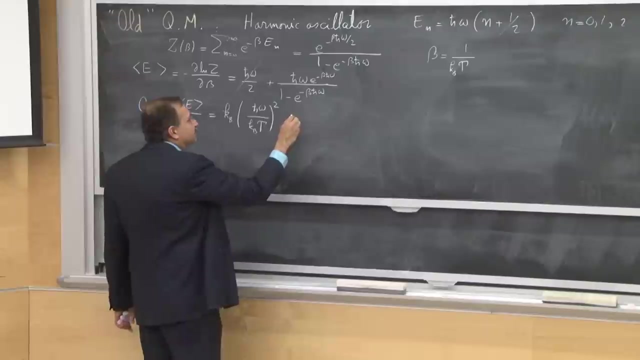 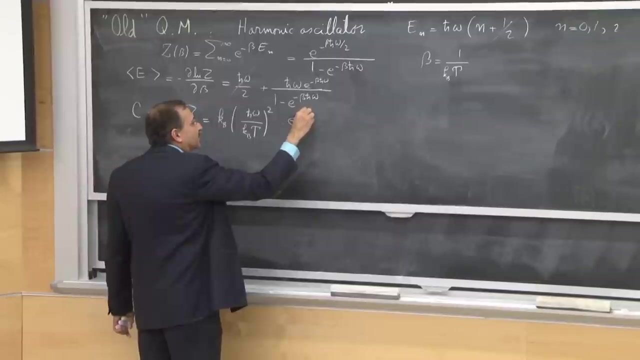 3. OK, Squared. So the whole thing I could write as kb. And then I had h bar omega over kt squared And then from these factors I had something like e to the minus, e to the h bar omega over kt. 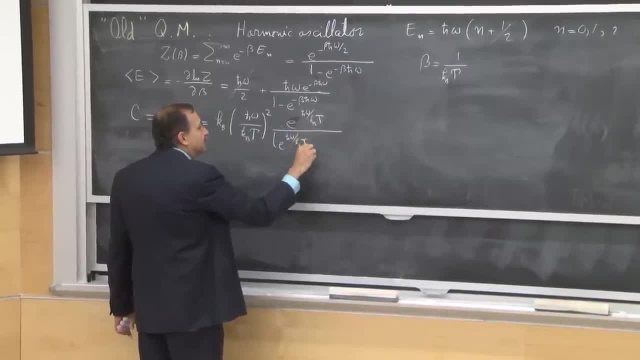 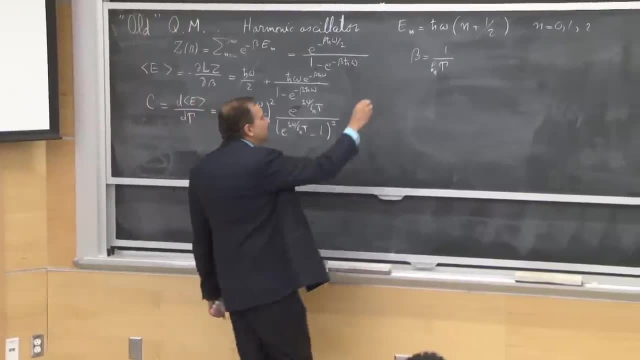 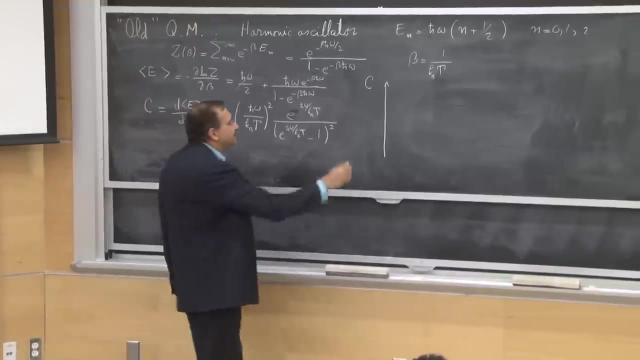 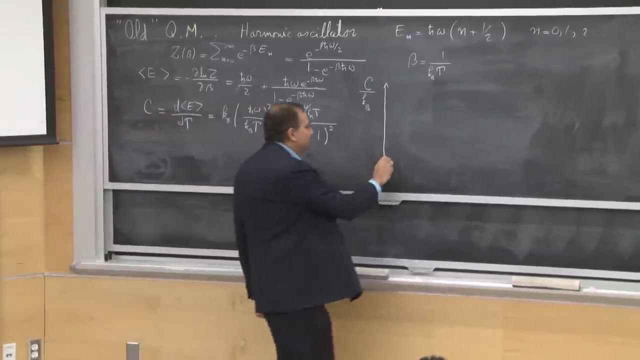 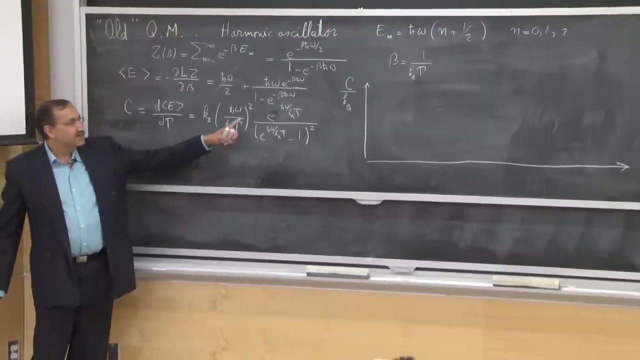 e to the h bar omega over kt Minus 1 squared. So if we were to plot this function, the heat capacity, in its natural units, that are, this kb, Then as a function of temperature we get behavior that we can actually express. 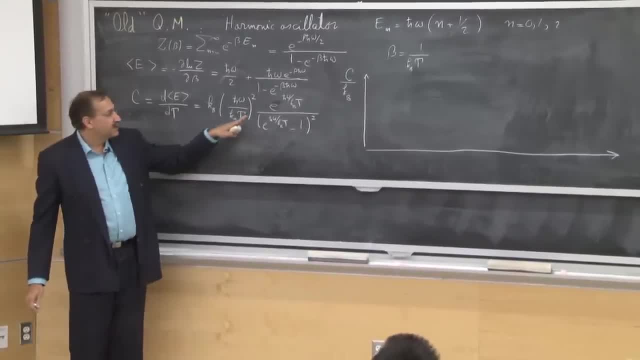 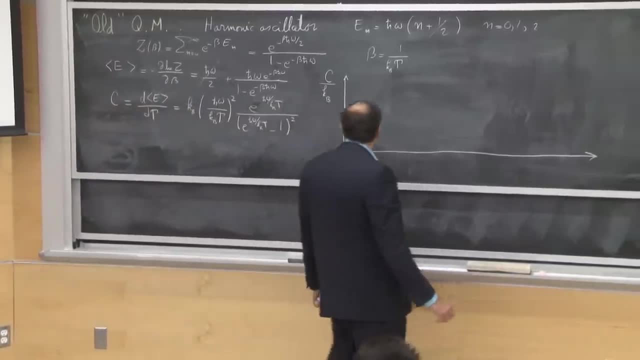 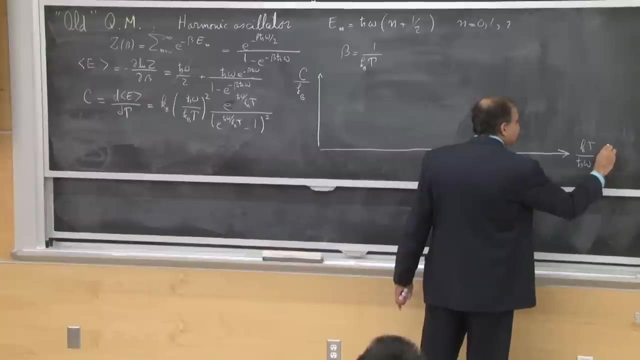 Correctly in terms of the combination. you can see, always we get temperature in units of kb over h bar omega. So I can really plot this in the form of, say, kt over h bar omega, which we call t, to some characteristic temperature. 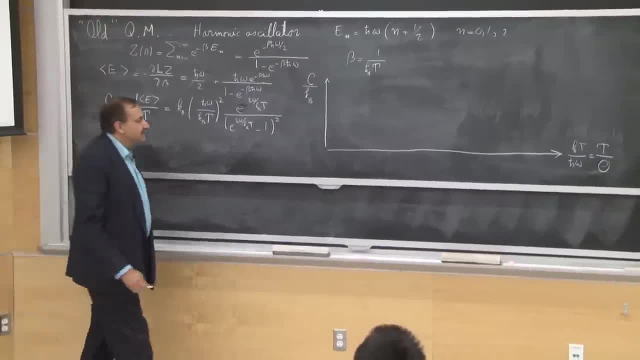 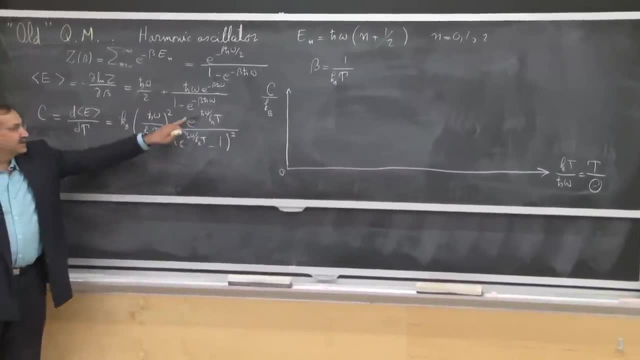 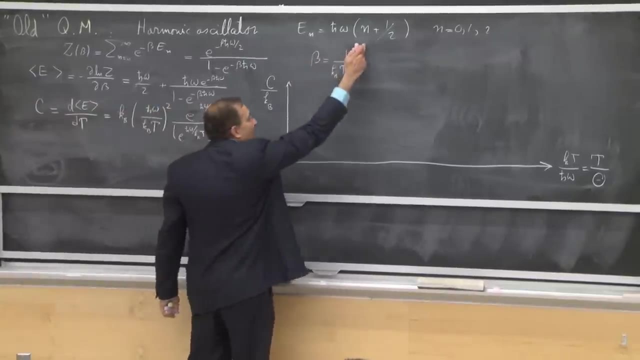 And the behavior that we have is that, close to 0 temperatures, you go to 0 exponentially. because of, essentially, the ratio of these exponentials, We leave 1 exponential in the denominator. So the gap that you have between n equals to 0 and n equals to 1. 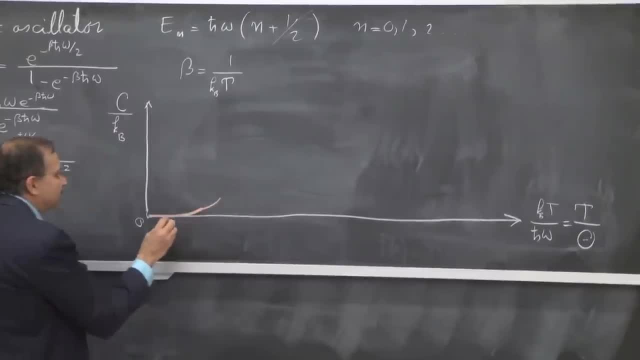 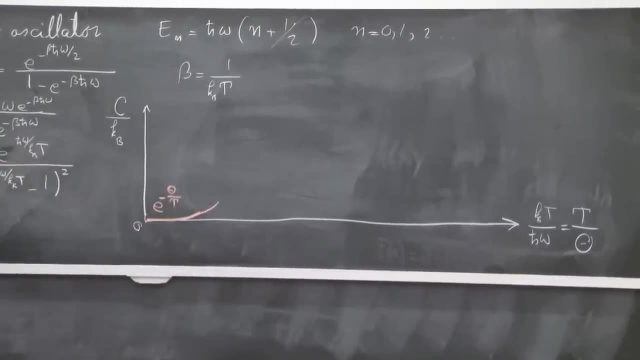 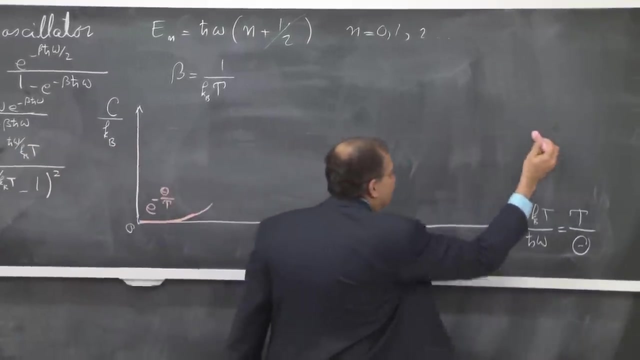 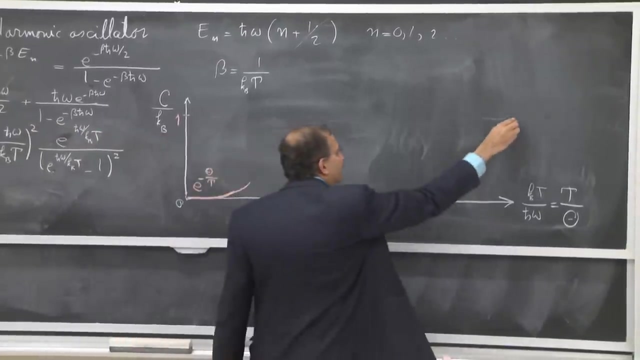 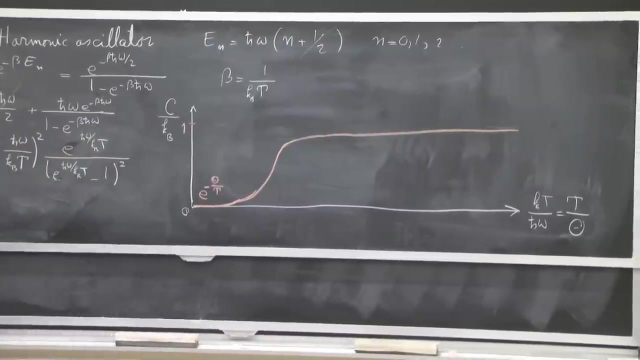 translates to a behavior that, at low temperatures, is exponentially decaying to leading order. OK, Eventually, at high temperatures, you get the classical result where you saturate to 1. And so you will have a curve that has a shift from one behavior to another behavior. 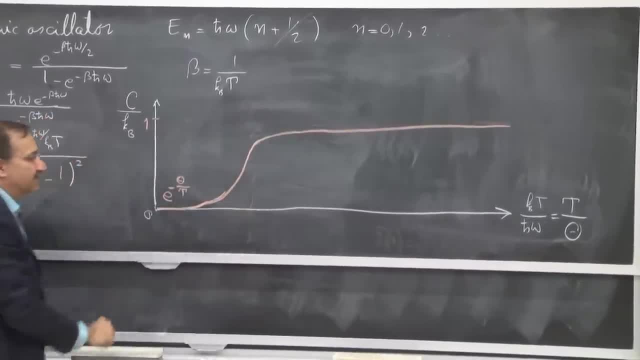 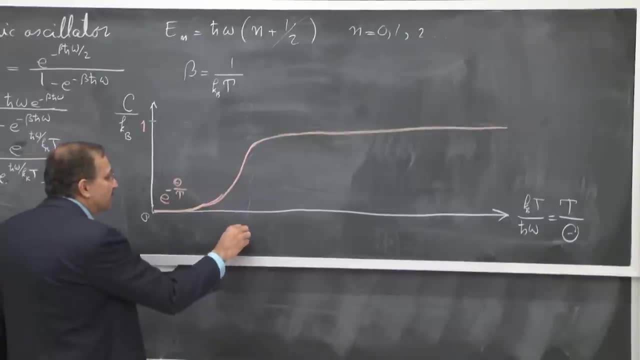 And the place where this transition occurs is when this combination is of the order of 1.. I'm not saying it's precisely 1, but it is of the order. OK, It's of the order of 1.. So, basically, you have this kind of behavior. 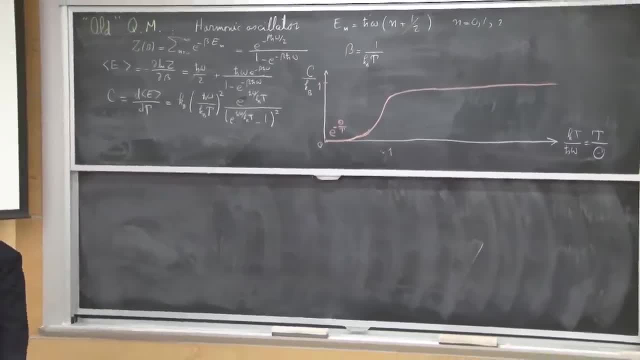 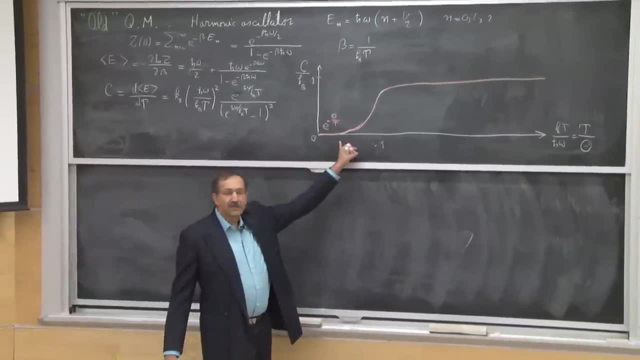 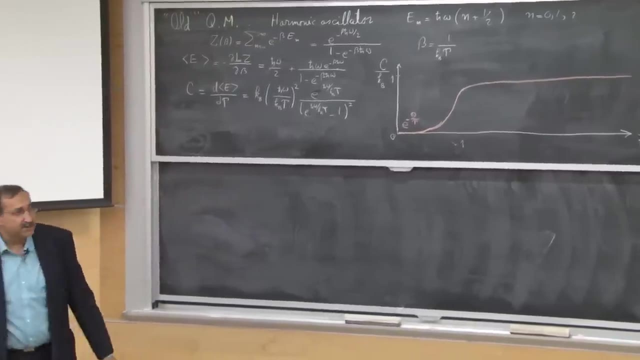 So we use this curve to explain the heat capacity of the atomic gas, such as the gas in this room, and why, at room temperature, we see a heat capacity in which it appears that the vibrational degrees of freedom are frozen, are not contributing anything, while at temperatures above a characteristic vibrational frequency, which for a gas, is of the order of 10 to the 3 degrees K. you will get energy in the harmonic oscillators, also in the vibrations, And the heat capacity jumps because you have another way. 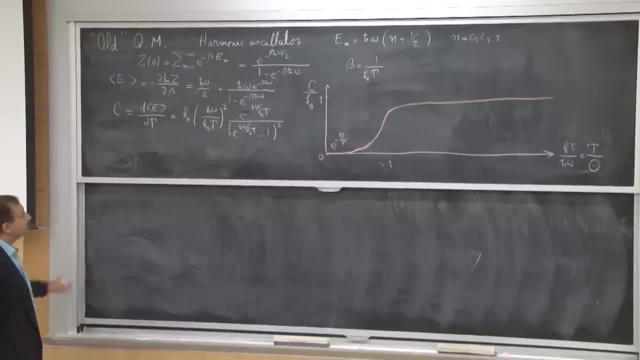 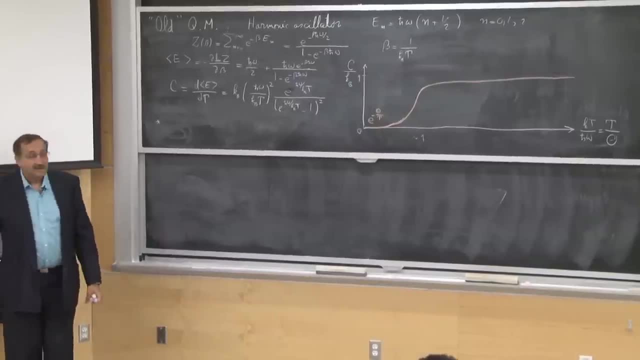 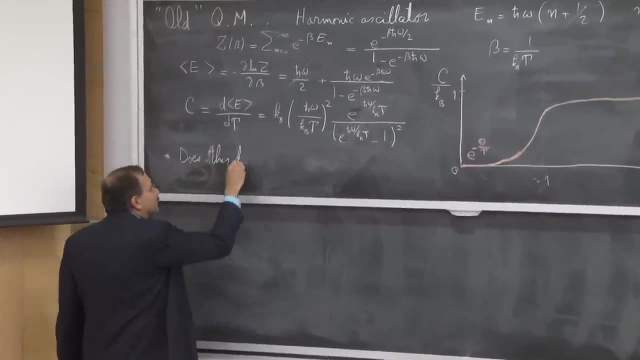 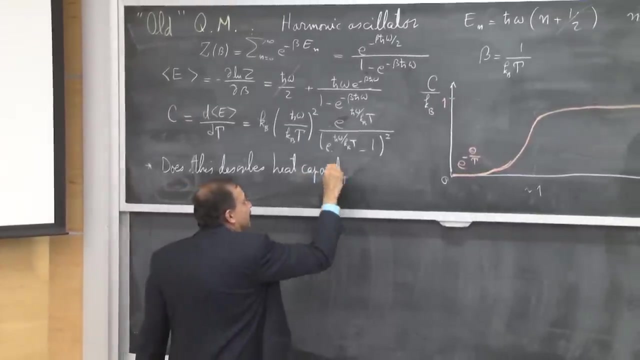 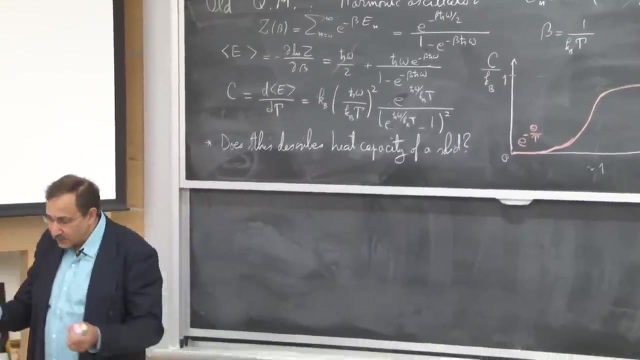 of storing energy. So the next thing that we asked was whether this temperature, this temperature is going to change. OK, Let's describe also heat capacity of a solid. So basically, for the diatomic gas, you have two molecules, two atoms. sorry, 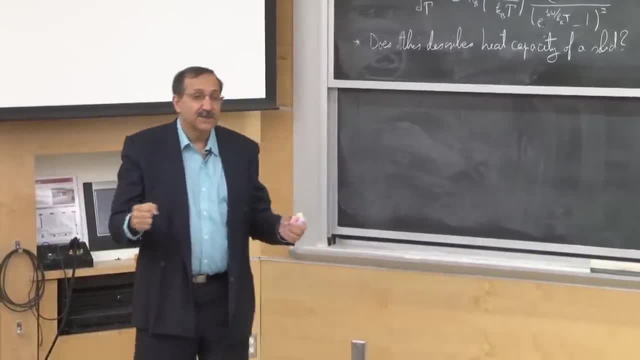 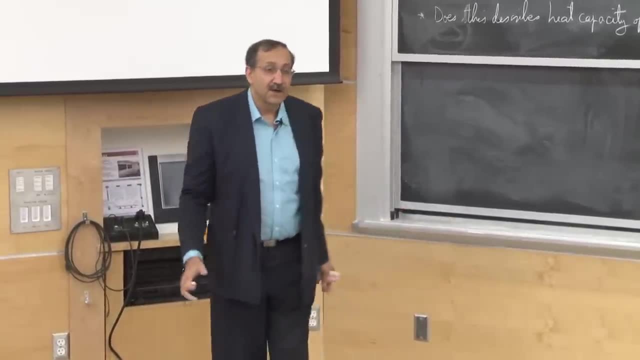 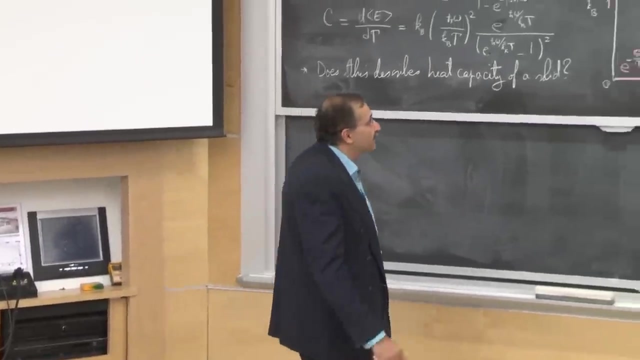 that are bounded together into a molecule And you consider the vibrations of that, You can regard the solid as a huge molecule, A molecule with lots of atoms joined together And they have vibrations. And if you think about all of those vibrations giving you 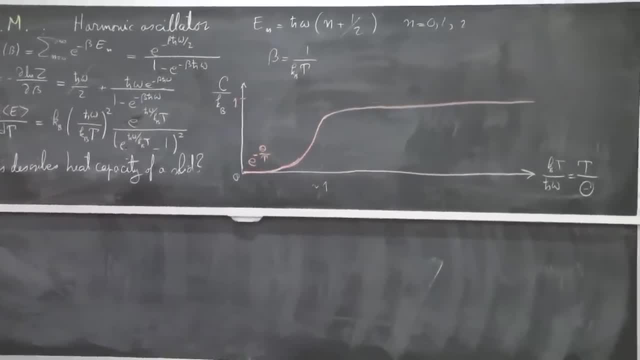 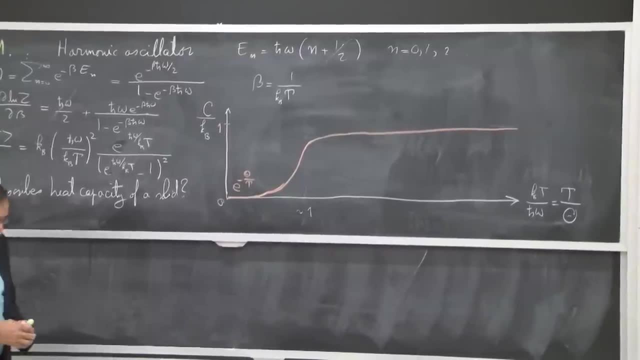 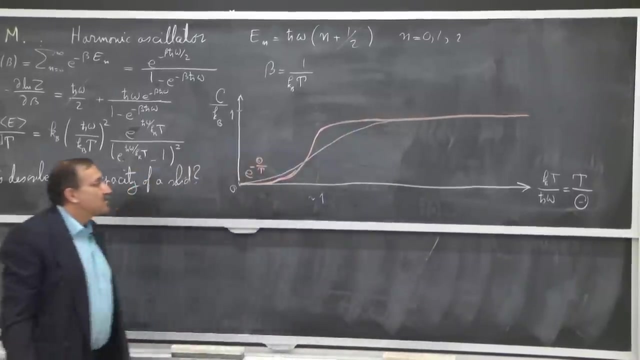 something that is similar to this, you would conclude that the heat capacity of the solid should also have this kind of behavior, Whereas we noted that, in actuality, the heat capacity of the solid vanishes much more slowly, Lowly at low temperatures. 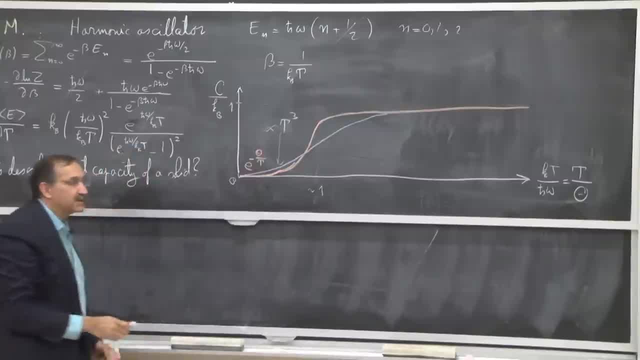 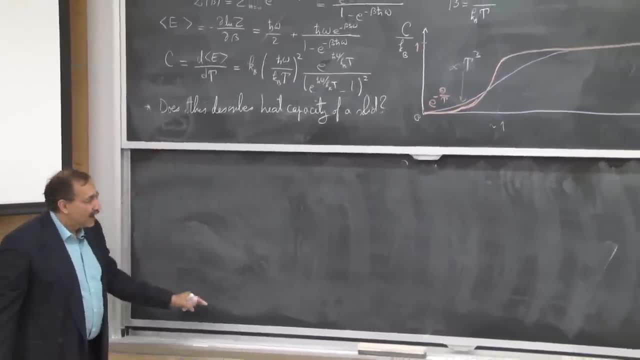 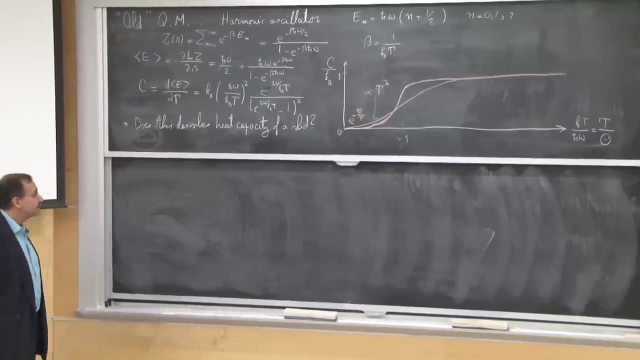 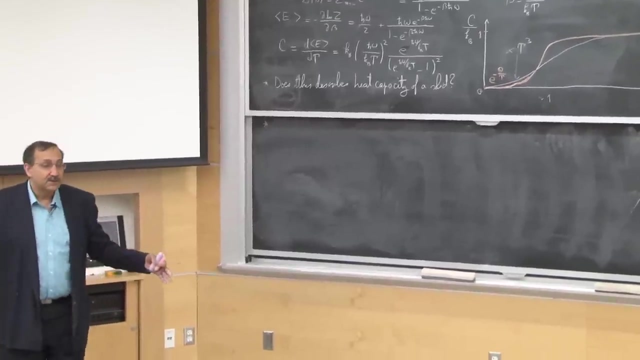 And the dependence at low temperatures is proportional to T cubed. So at the end of last lecture we gave an explanation for this, which I will repeat Again. the picture is that the solid, like a huge molecule, has vibrational modes. 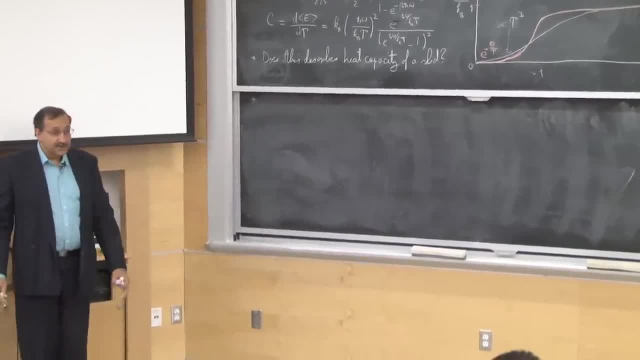 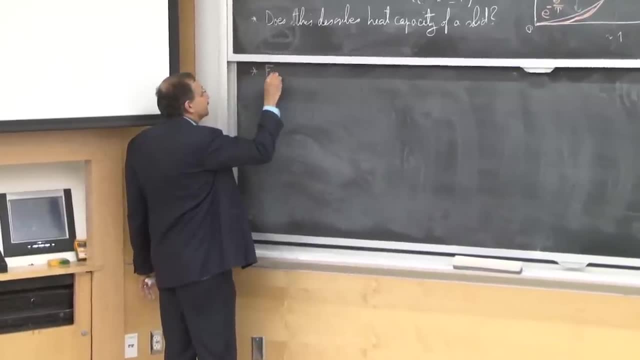 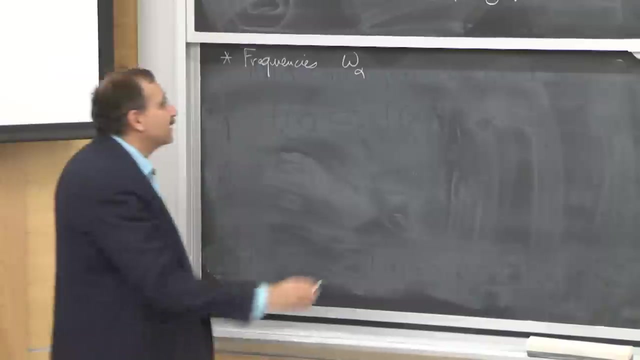 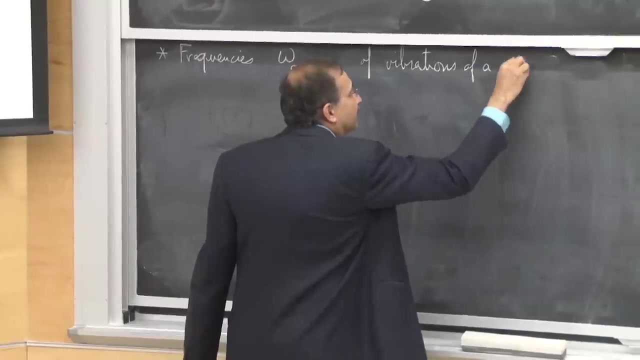 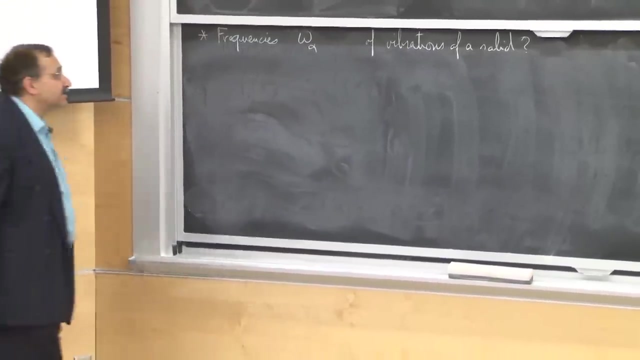 But these vibrational modes cover a whole range of different frequencies, And so if you ask what are the frequencies, omega, alpha of vibrations of a solid, the most natural way- I think OK, OK- To characterize them is, in fact, 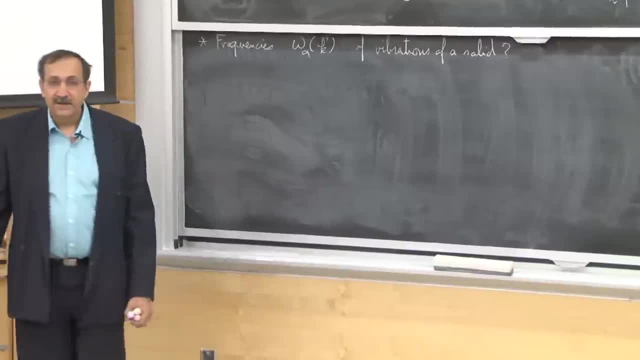 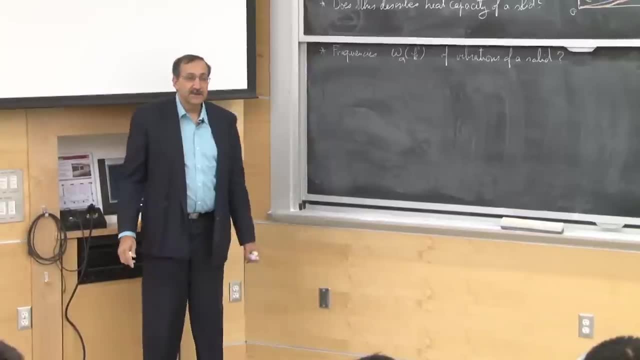 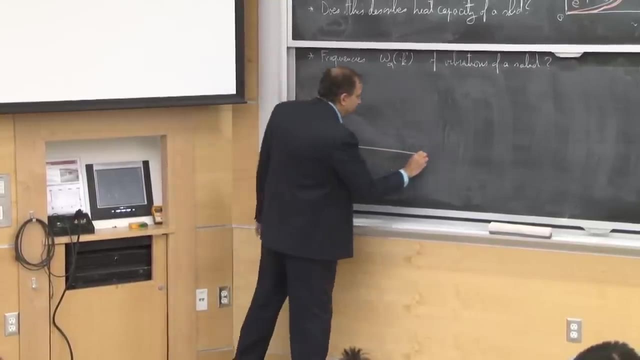 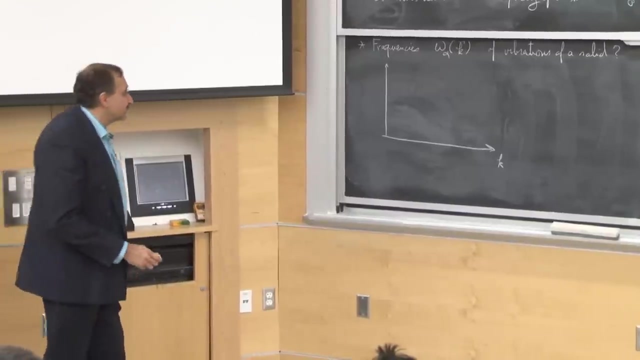 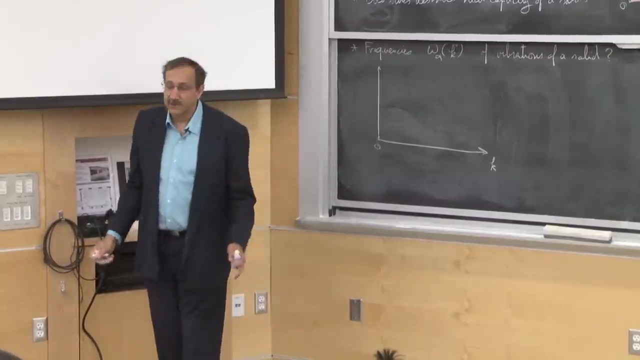 in terms of a wave vector, k, that indicates the direction for the oscillatory wave that you set up in the material And depending on k, you have different frequencies. And I said that essentially the longest wavelength corresponding to k equals to 0- is taking the whole solid. 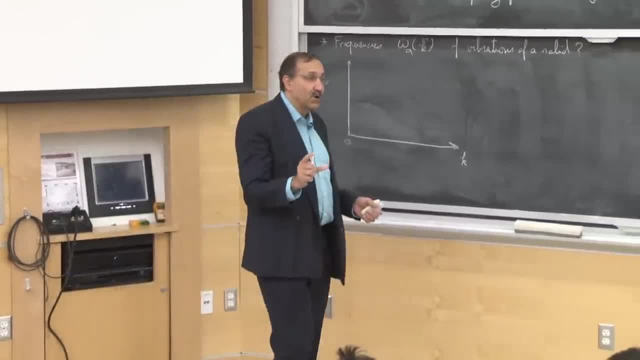 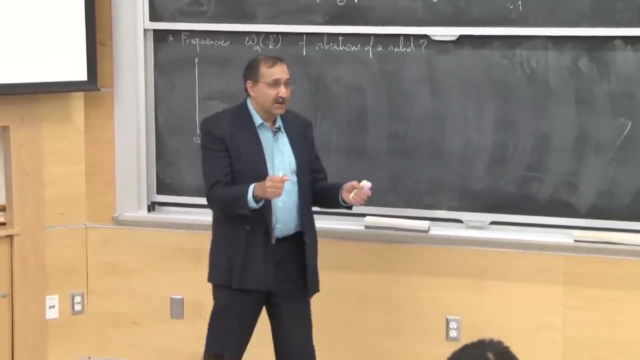 and translating it Again, thinking back about the oxygen molecule. the oxygen molecule, you have two coordinates. It's the relative coordinate that has the vibration And you have a center of mass coordinate that has no energy. If you make a molecule more and more complicated, you're going. 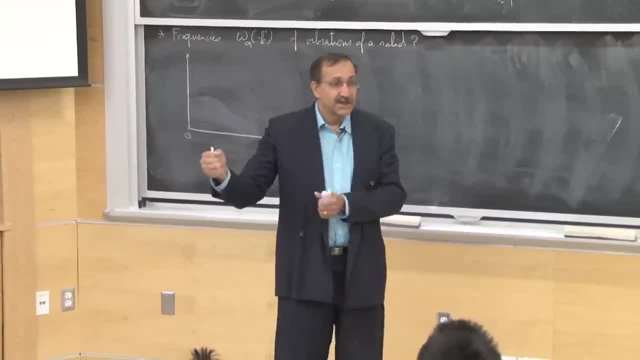 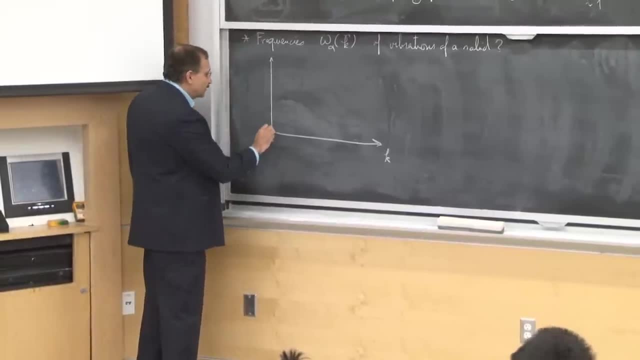 to have more modes, But you will always have the 0 mode that corresponds to the translation And that carries over all the way to the solid. So there is a mode that corresponds to translations and, in fact, rotations that would carry no energy. 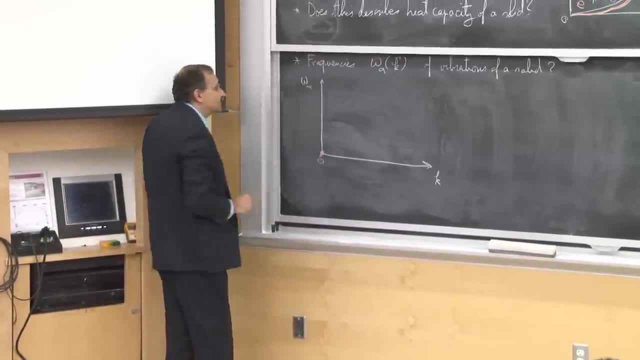 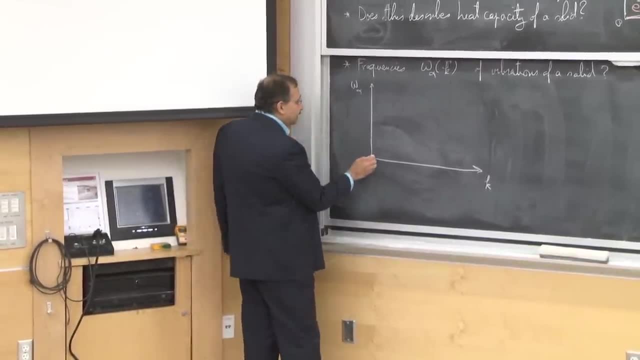 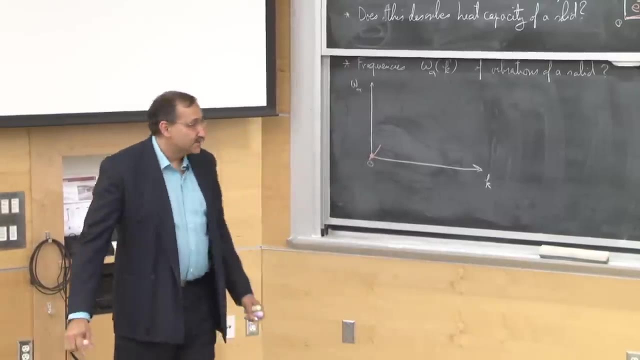 and correspond therefore to 0 frequency. And then, if you start to make long wavelength oscillations, the frequency is going to be small And indeed, what we know is that we tap on the solid and you create sound waves which 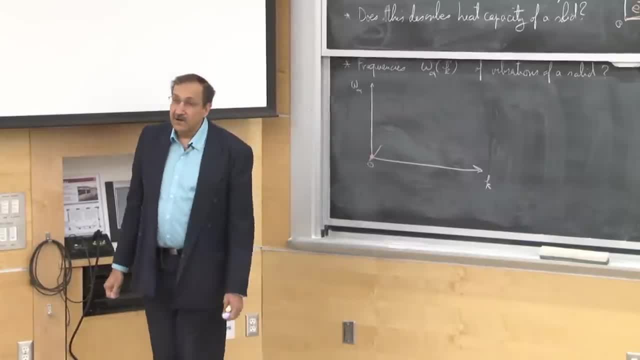 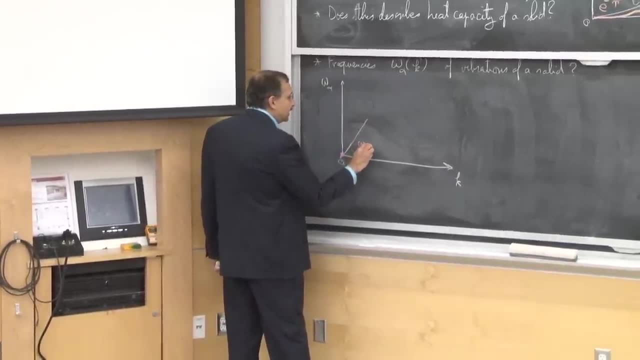 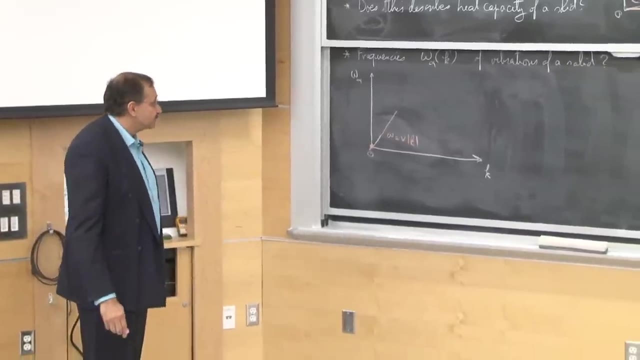 means that the low frequency, long wavelength modes have a dispersion relation in which omega is proportional to k, And we can write that as omega is v times k, where v is the velocity of the sound in the solid. Now, of course, the shortest wavelength that you can have. 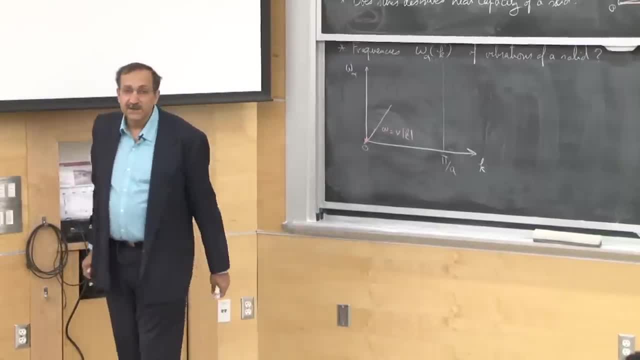 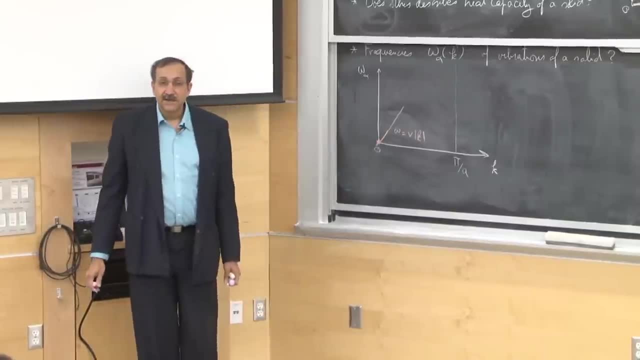 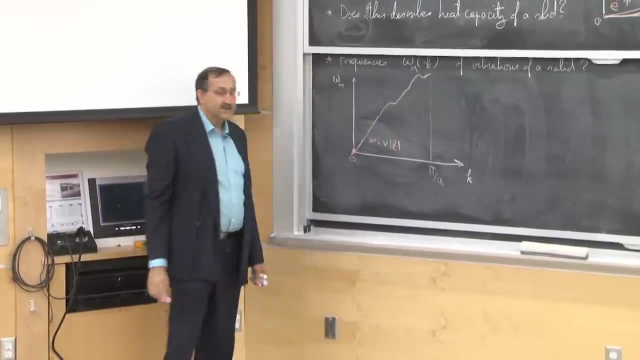 let's see, It is related to the separation between the atoms in the solid, And so, basically, there is a limit to the range of k's that you can put in your system, And this linear behavior is going to get modified once you get towards the edge of the solid. 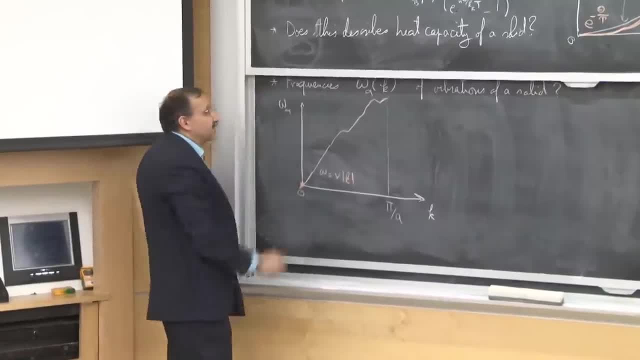 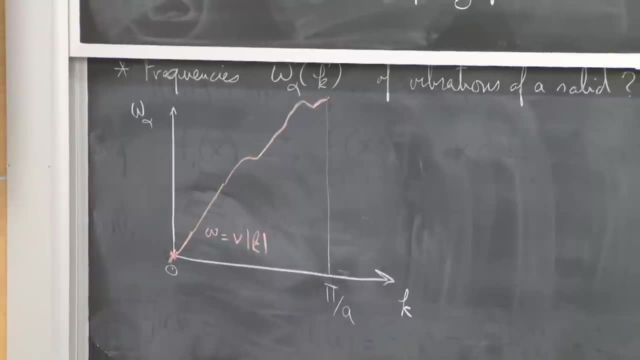 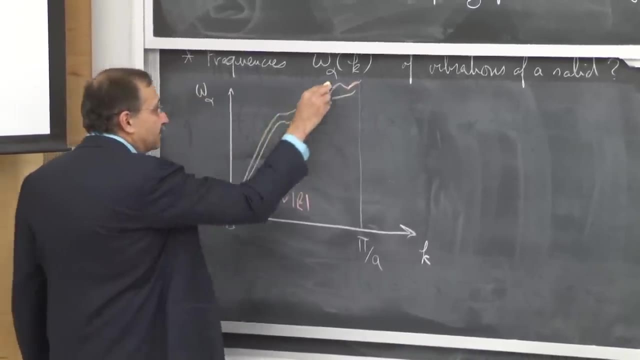 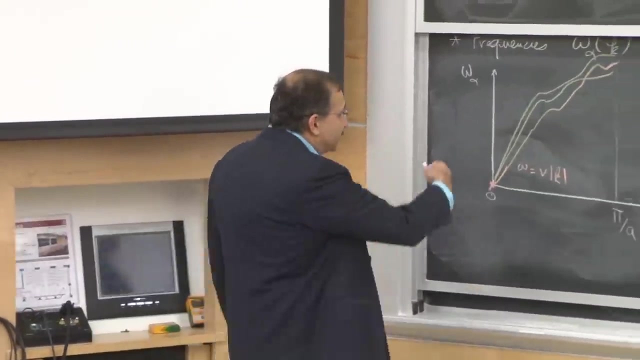 And the reason I have alpha here is because you can have different polarizations. There are three different possible polarizations, So in principle you will have three of these curves in the system And these curves could be very complicated when you get to the edge of Brillouin zone. 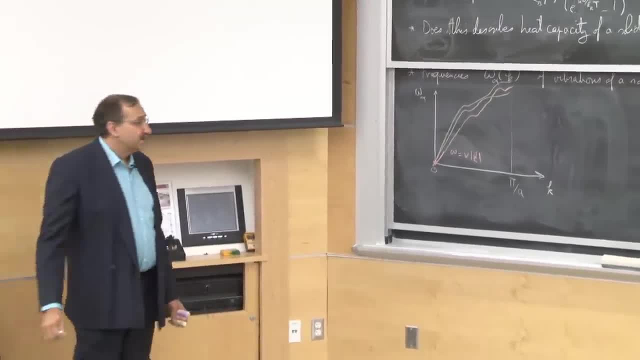 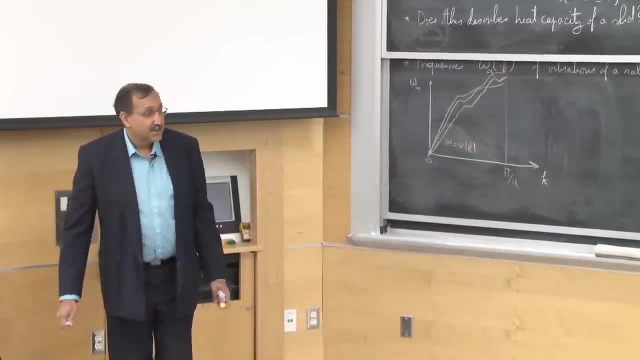 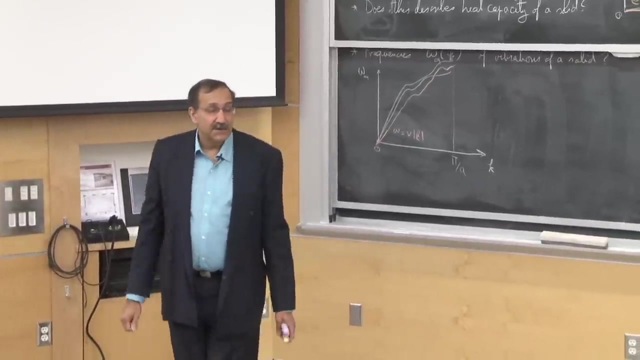 and you have to solve a big dynamical matrix in order to extract what the frequencies are if you want to have the complete spectrum. So the solid is a collection. It's a collection of these harmonic oscillators that are, in principle, very complicated. 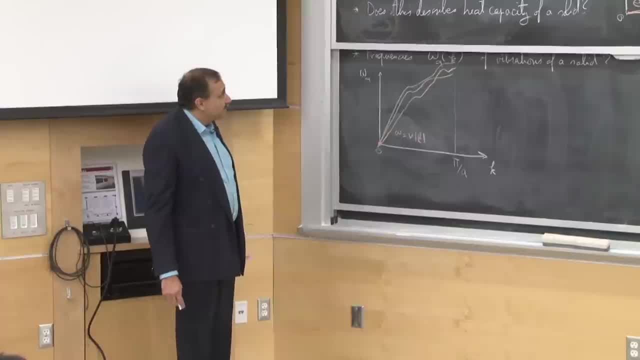 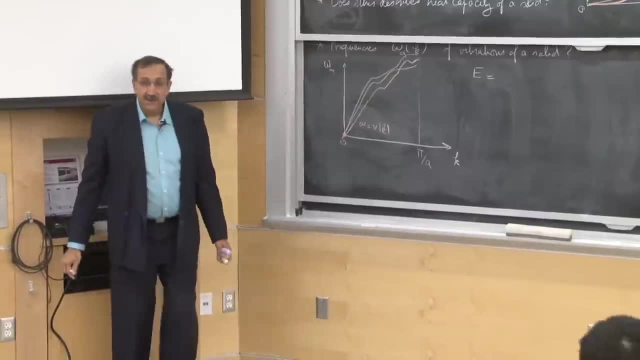 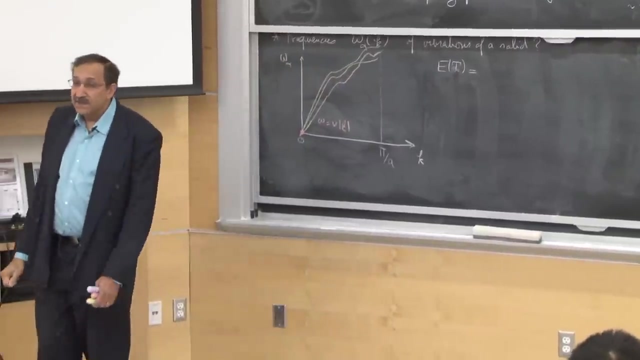 But we have the following. So I say, OK, I have all of these And I want to calculate, at a given temperature, how much energy I have put in the solid. So this energy that I have put in the vibrations at some temperature, t, assuming that these vibrations are- 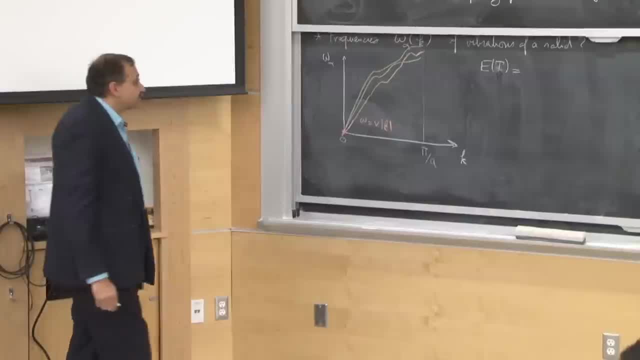 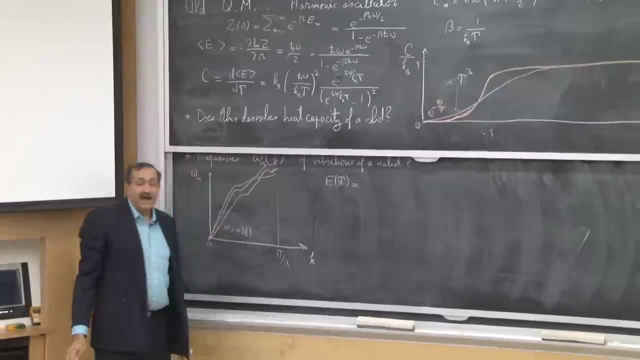 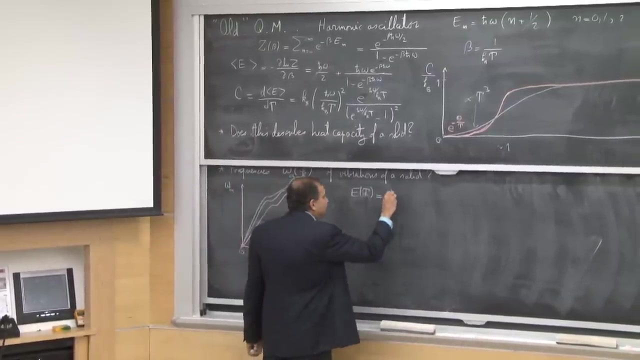 really a collection of these oscillators. Well, what I have to do is to add up all of these terms. There's going to be adding up all of the h-bar, omega over 2s for all of these. OK, That will give me something that I will simply call E0,. 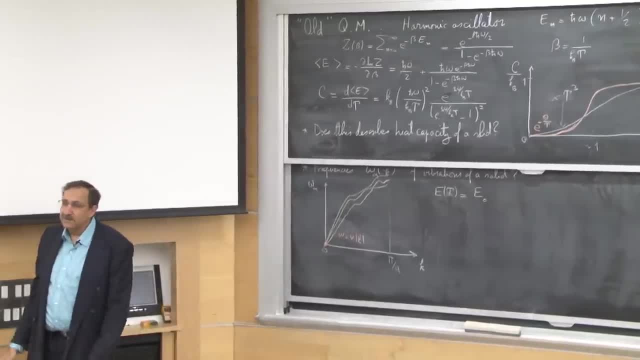 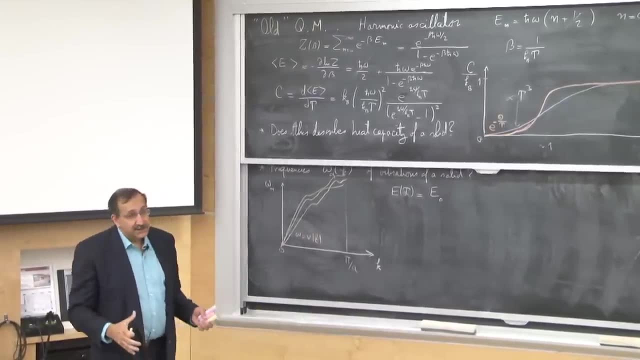 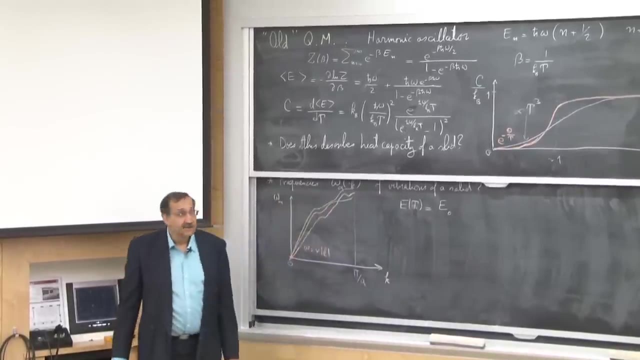 because it doesn't depend on temperature. Presumably it will exist at 0 temperature, And I can even fold into that: whatever the value of the potential energy of the interactions between the particles is at 0 temperature- 0 temperature. What I'm interested in really is the temperature dependence. 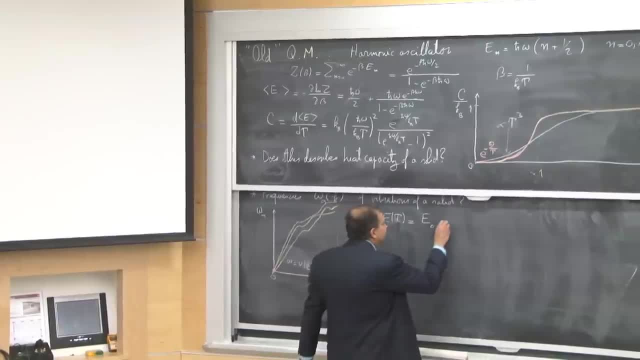 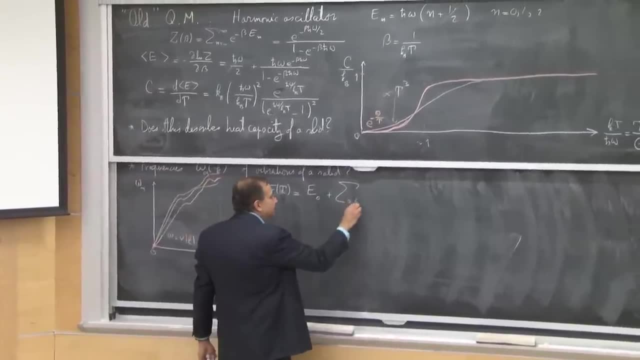 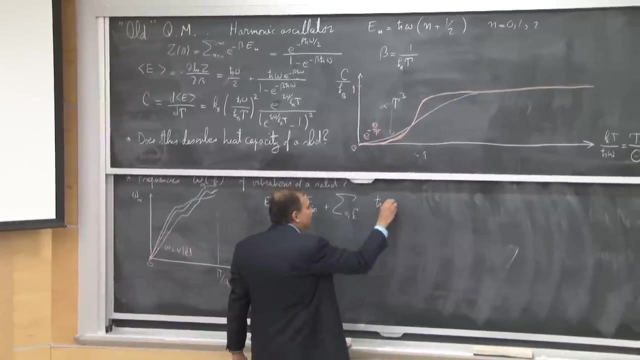 So I basically take the formula that I have over there and sum over all of these oscillators. The oscillators are characterized by the polarization and by the wave vector k, And then I have essentially h-bar omega alpha of k divided by e to the beta h-bar omega alpha of k. 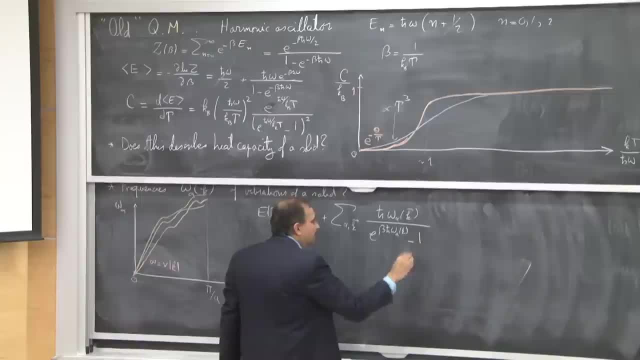 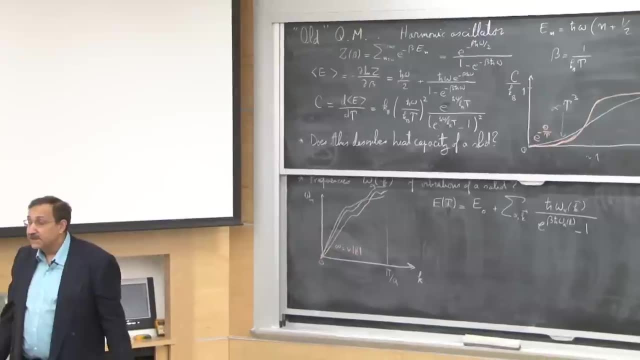 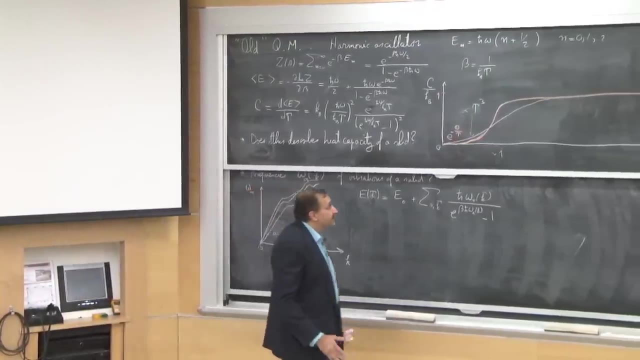 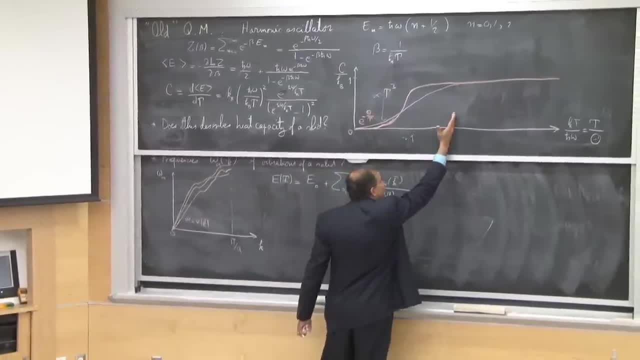 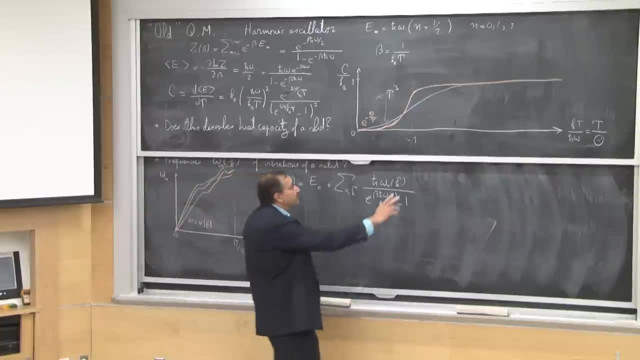 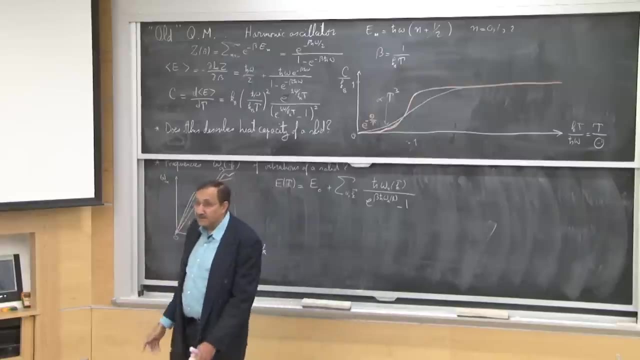 you would say that the heat capacity is 1 if you are on this side to 0 if you are on that side. OK, And what distinguishes those two sides is whether the frequency in combination with temperature is less than or larger than 1.. 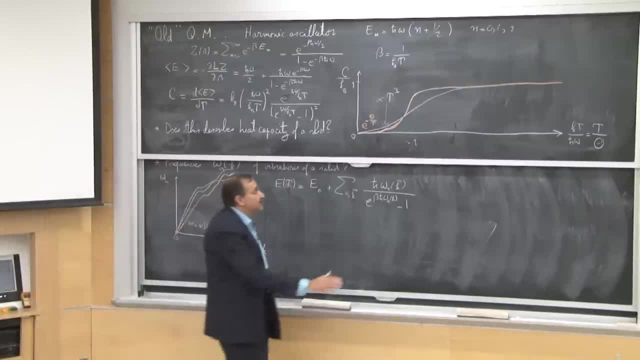 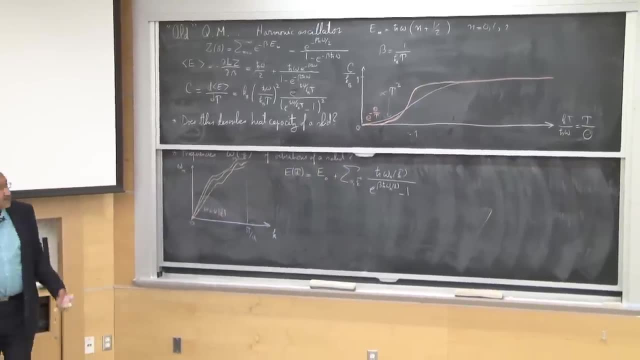 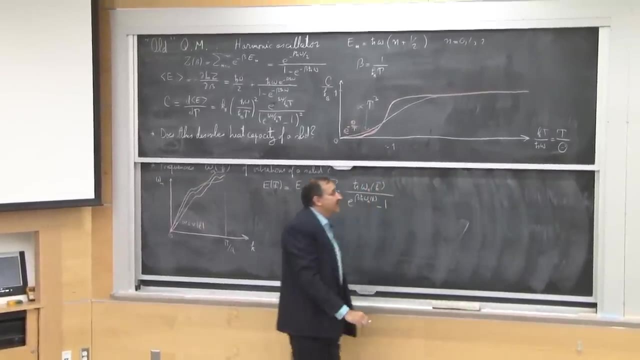 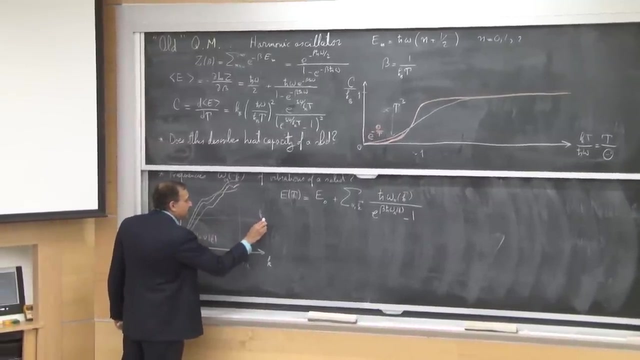 Basically low frequencies would end up being here. High frequencies would end up being here and would not contribute. So for a given temperature there is some borderline. That borderline would correspond to kt over h bar. So let me draw where that borderline is: kt over h bar. 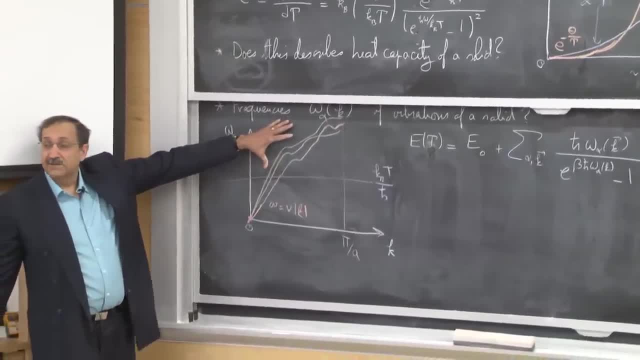 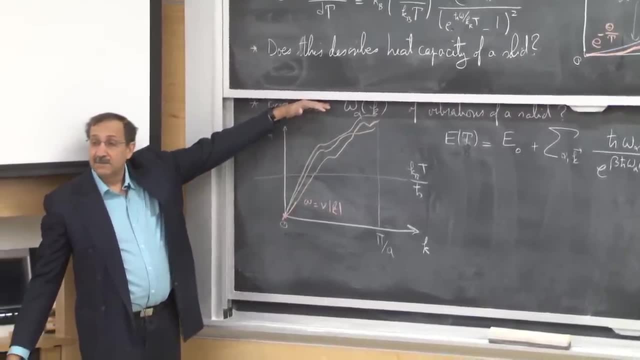 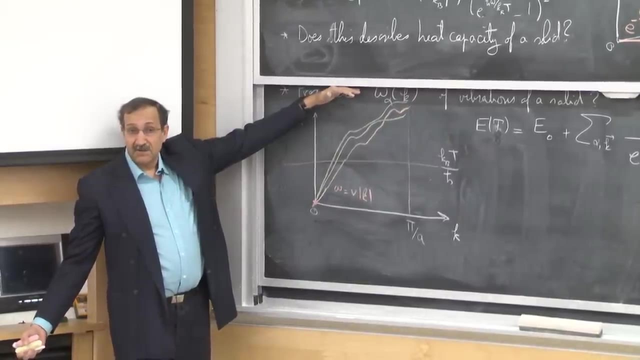 For a particular temperature. all of these modes are not really contributing. All of these modes are contributing If my temperature is high enough. everything is contributing And the total number of oscillators is 3n- It's the number of atoms. 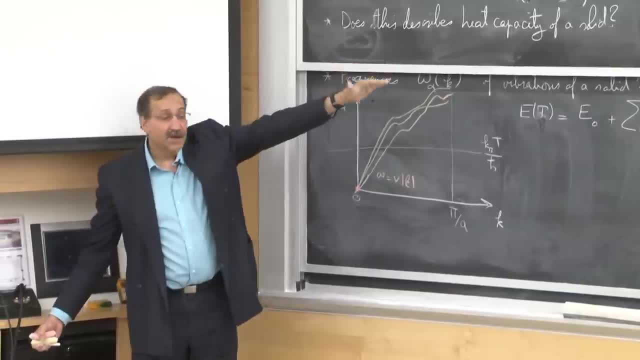 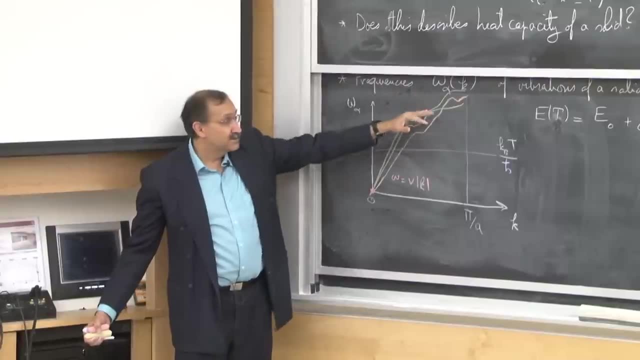 So. So essentially, I will get 3n times whatever formula I have over there As I come further and further down. there is some kind of complicated behavior as I go through this spaghetti of modes, But when I get to low enough structures, 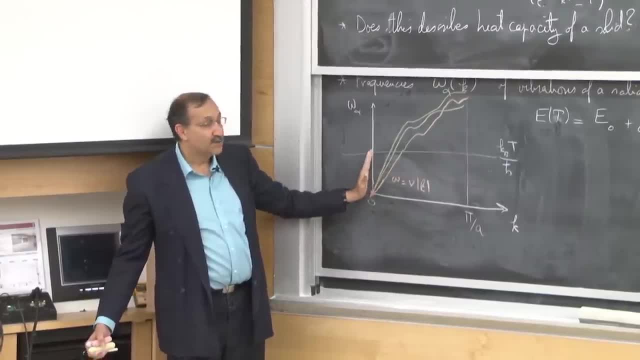 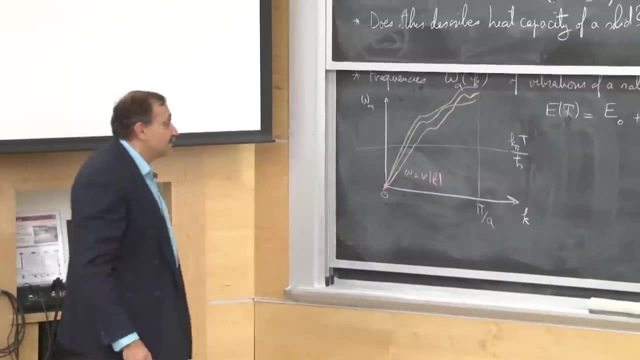 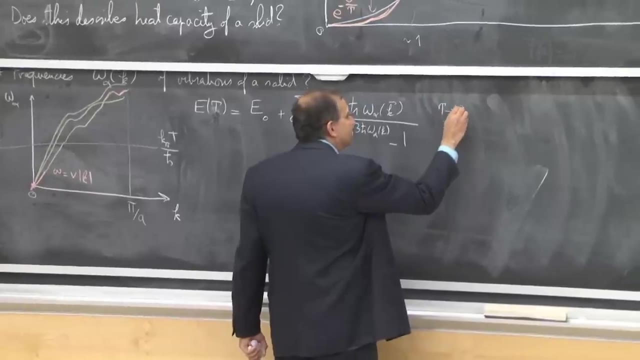 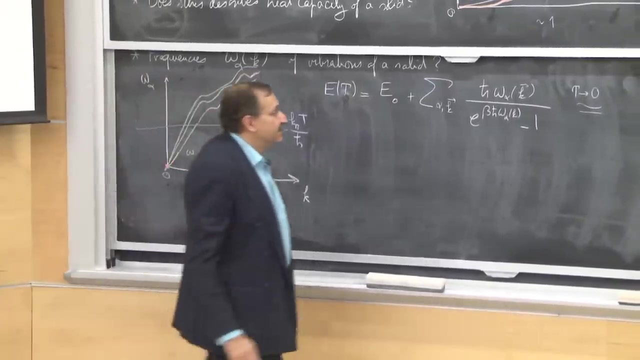 then again things become simple, because I will be only sensitive to the modes that are described by this, omega being vk. So if I'm interested, And t going to 0 means less than some characteristic temperature that we have to define shortly. So let's say, replace this with t less than some theta d. 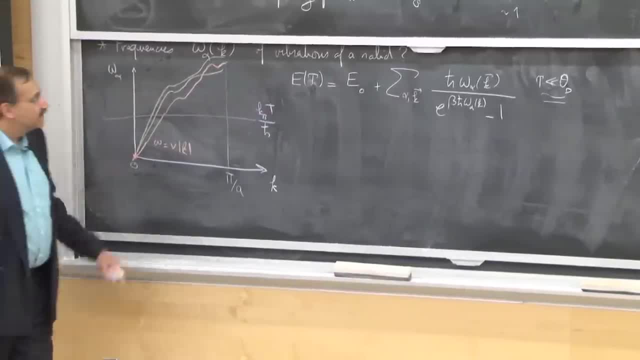 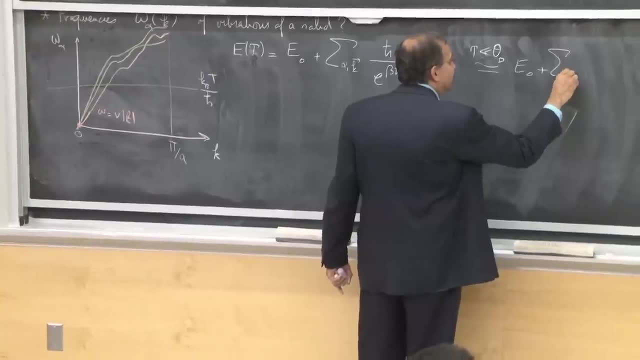 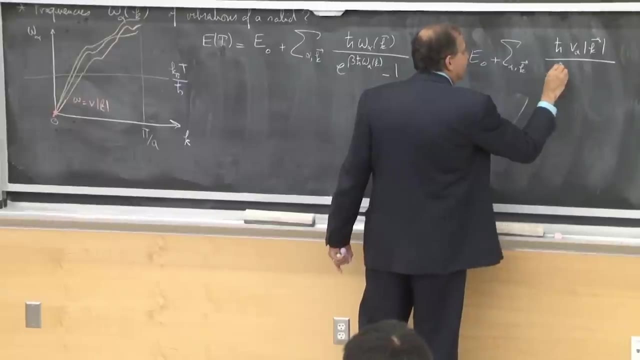 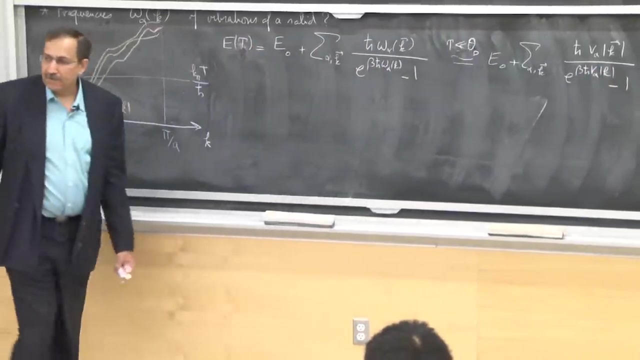 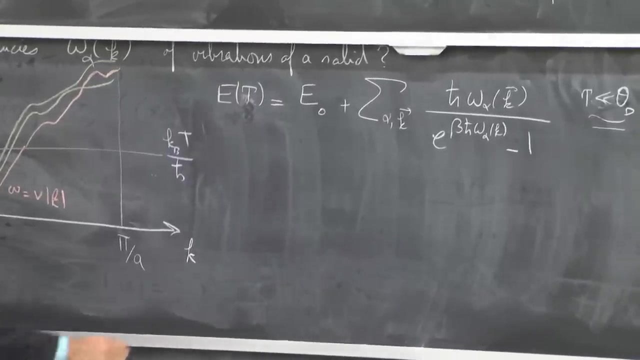 that I have to get for you shortly. Then I will replace this with E0 plus sum over alpha and k of h bar v- alpha k e to the beta h bar v- alpha k minus 1.. Now for simplicity. essentially I have to do three different sums. 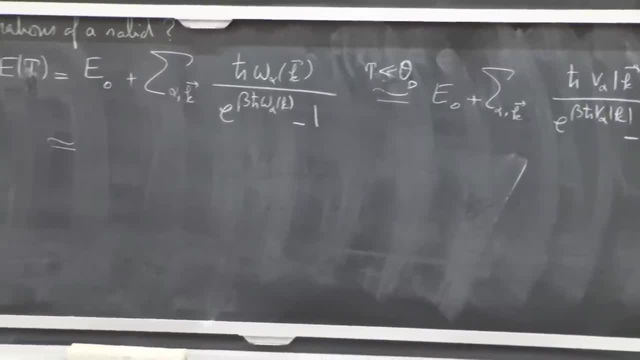 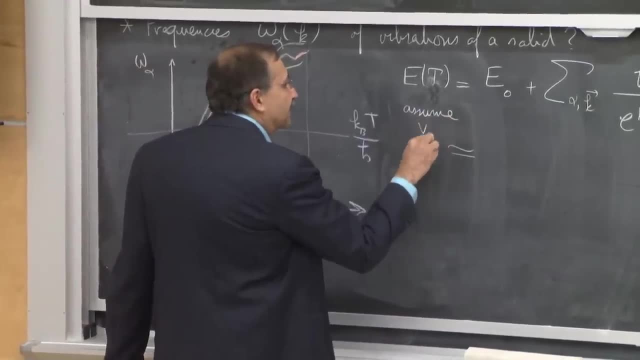 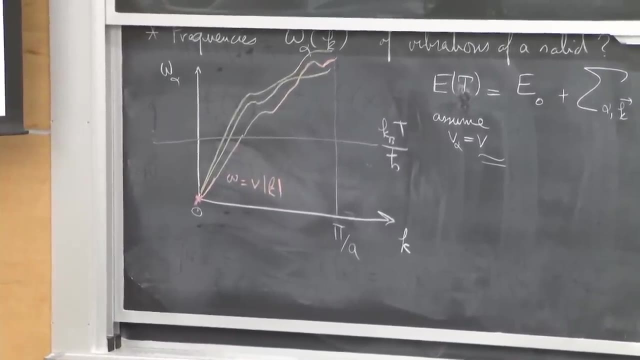 All of them are the same, up to having to use different values of v. Let's just for simplicity, assume that all of the v alphas are the same v, So that I really have only one velocity. There's really no difficulty in generalizing this. 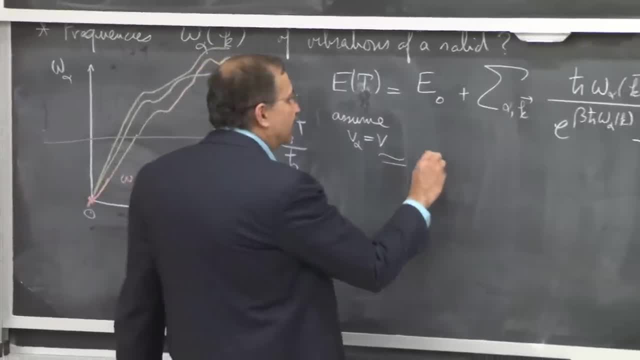 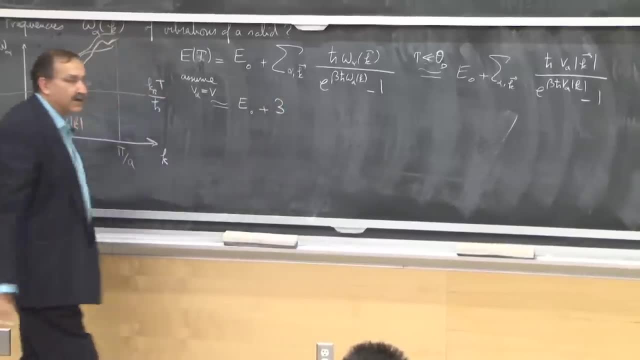 So let's do this for simplicity of algebra. So if I do that, then the sum over alpha will simply give me a factor of 3.. There are three possible polarizations, So I put a 3 there And then I have to do the summation over k. 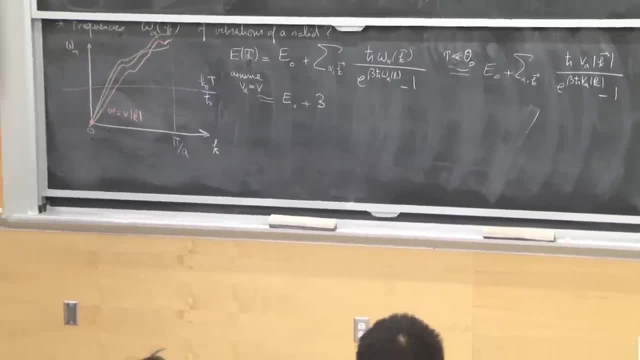 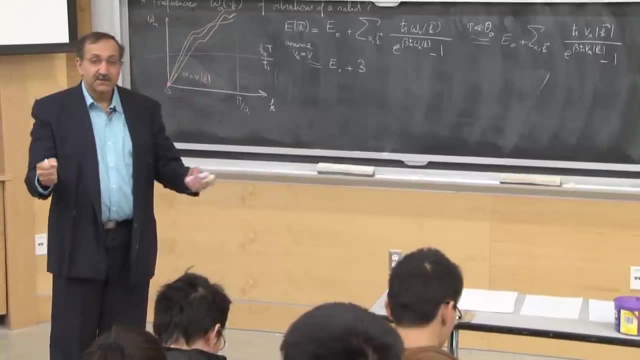 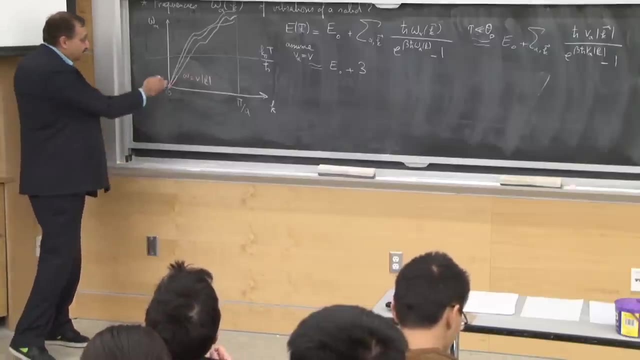 Well, what does the summation over k mean When I have a small molecule for the, let's say, three or four atoms? then I can enumerate what the different vibrational states are. As I go to a large solid, I essentially 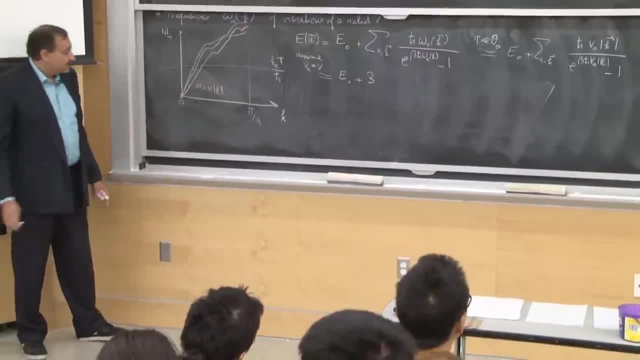 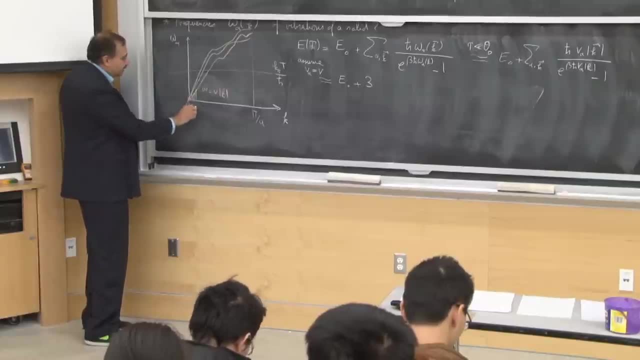 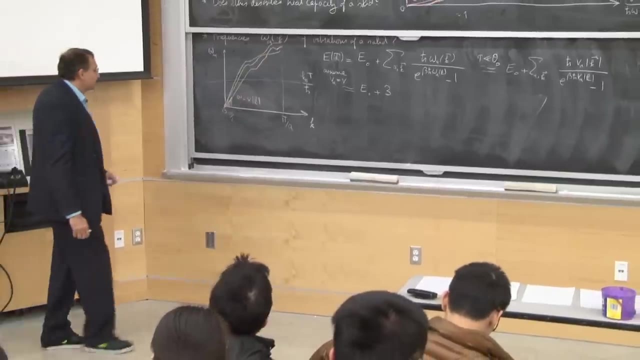 have modes that are at each value of k But in reality they are discrete. They are very, very, very, very finely separated by a separation that is of the order of 2 pi over the size of the system. So to ensure that eventually, when you count all of the modes, 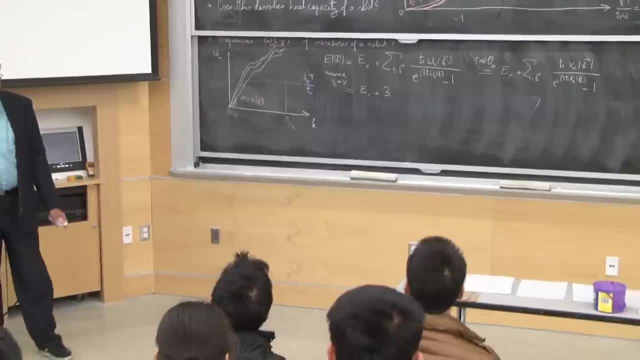 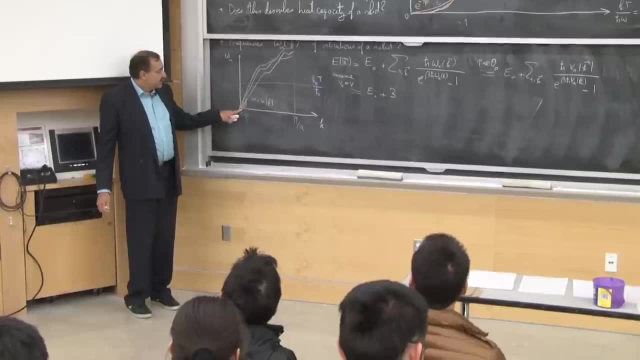 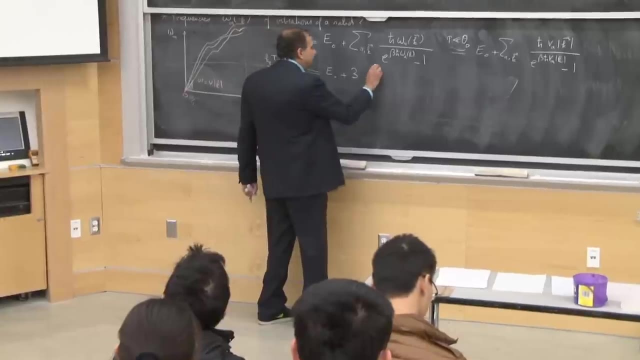 that you have here you again end up to have of the order of n states. So if that's the case, this sum really I can replace with an integral, Because going from one point to the next point does not make much difference, so I will have an integral. 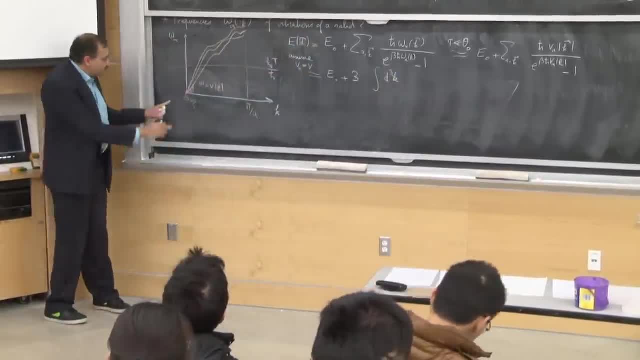 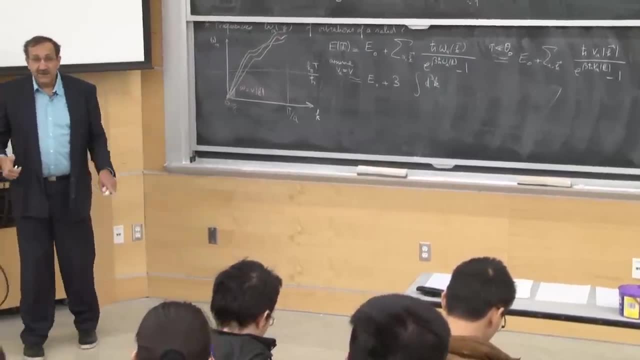 So this is 2 pi over k, But I have to know how densely these things are. And in one direction it is 2 pi over l, So the density would be l over 2 pi If I look at all three directions. 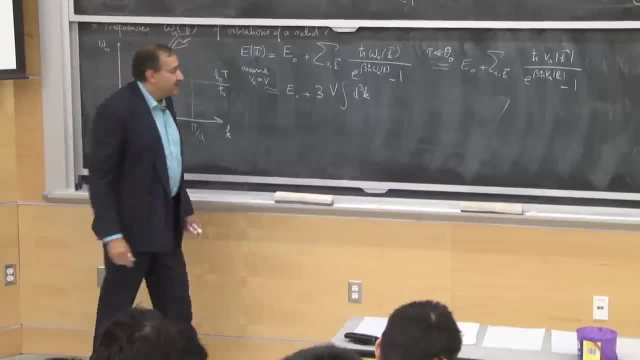 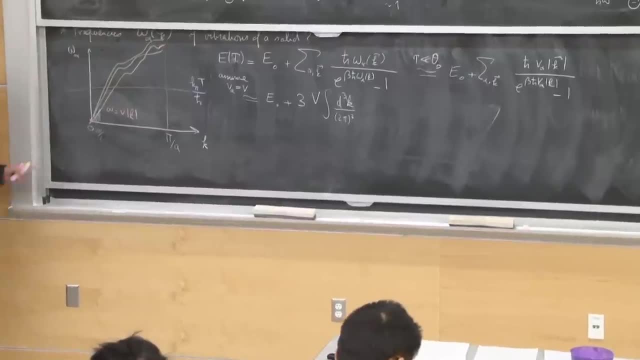 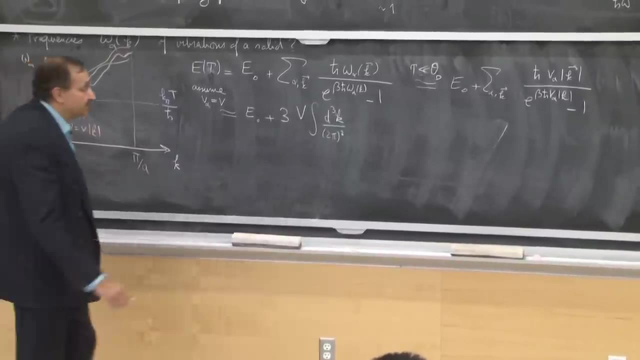 I have to multiply all of them, So I will get v divided by 2 pi cubed. So this is the usual density of states. Then you go to description in terms of wave numbers Or, later on, in terms of momentums. 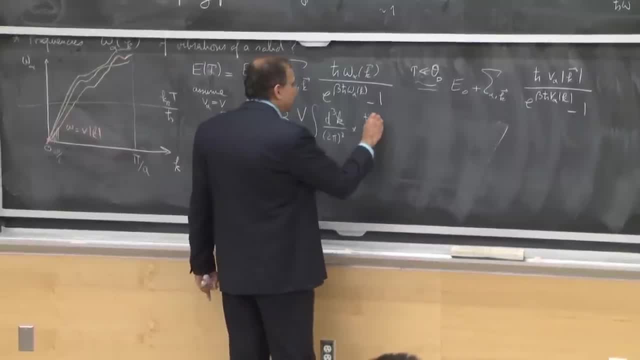 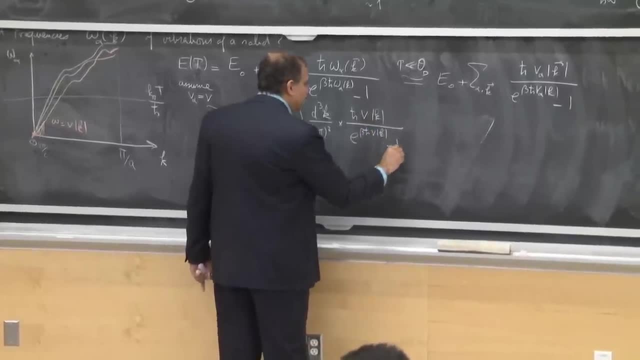 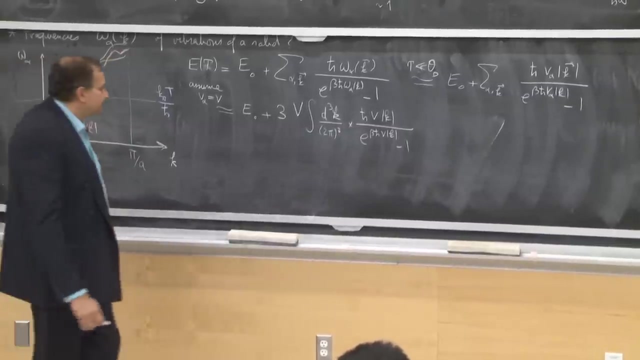 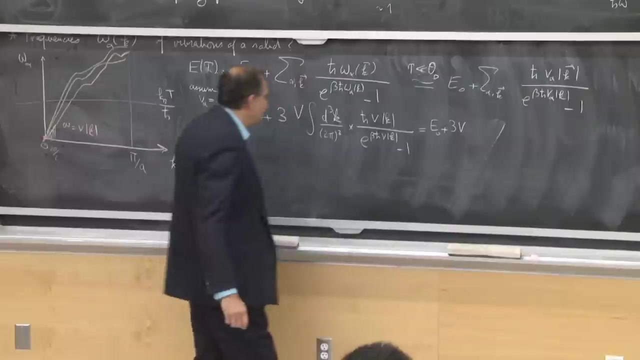 And what we have here is this integral h bar vk e to the beta h bar vk minus 1.. So let's simplify this a little bit further. I have e0.. I have 3v. The integrand only depends on the magnitude of k. 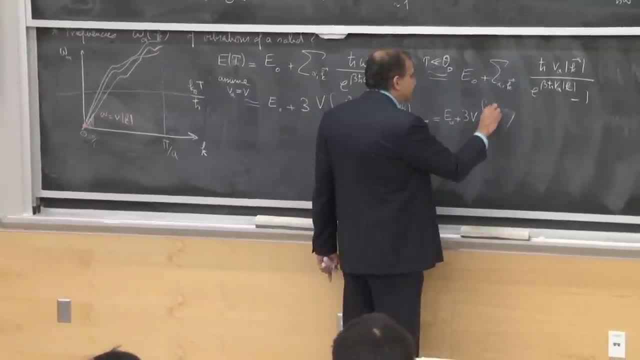 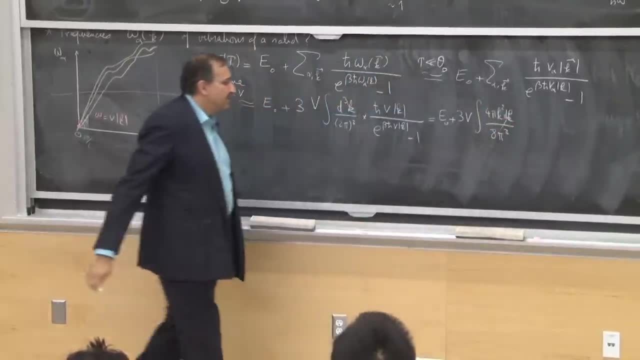 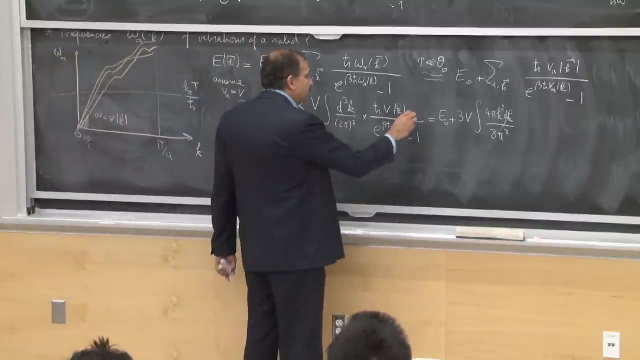 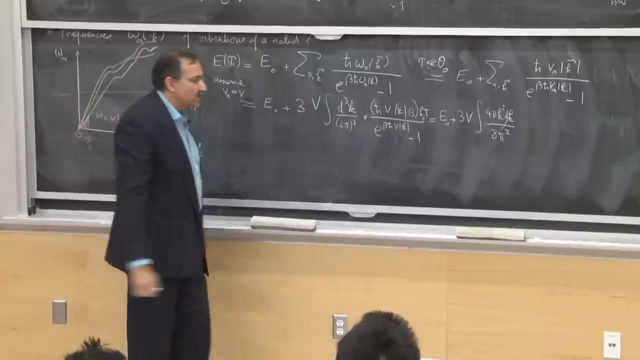 So I can take advantage of that spherical symmetry and write this as 4 pi k squared dk divided by this, 8 pi cubed. What I can do is I can also introduce a factor of beta here and multiply by kt. Beta kt is 1.. 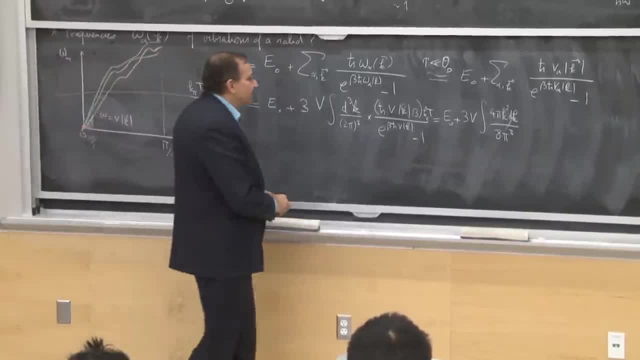 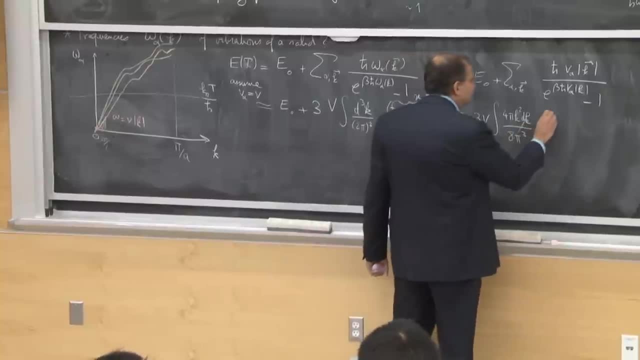 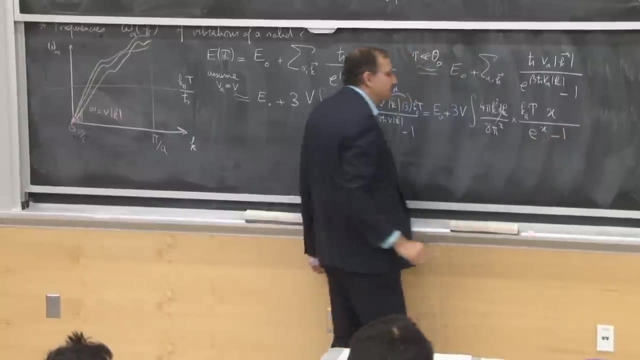 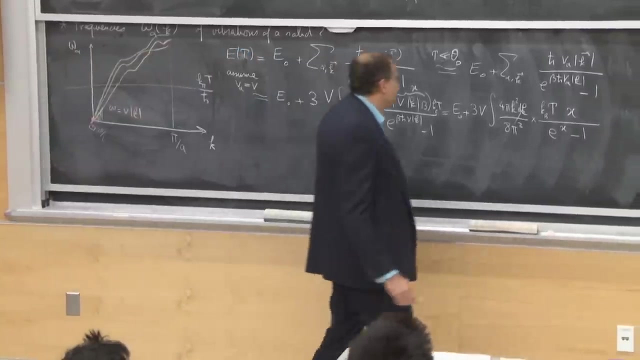 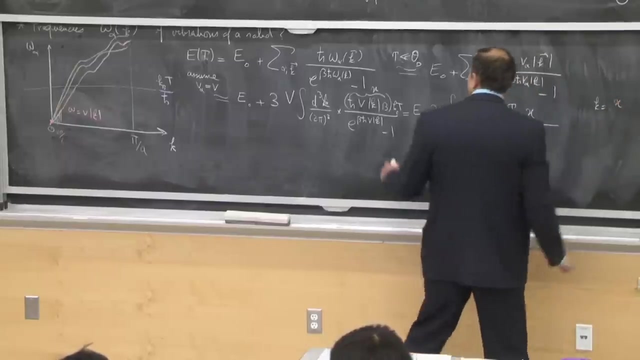 OK, And if I call this combination to be x, then what I have is kbt x e to the x minus 1.. And of course k is simply related to x by k being x 2, 2. So that's kt over h bar v. 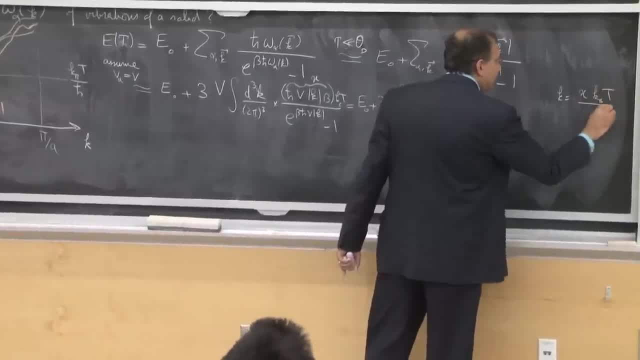 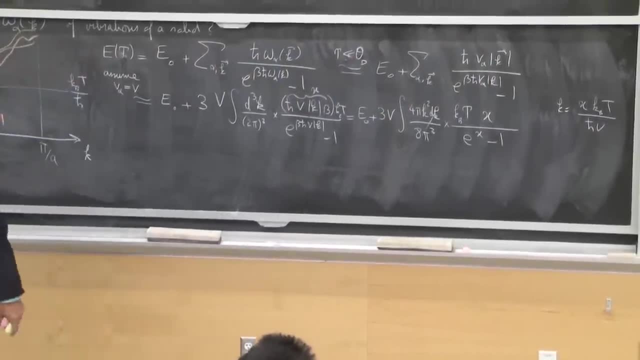 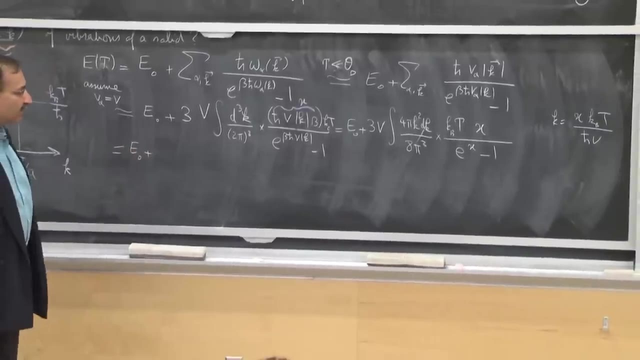 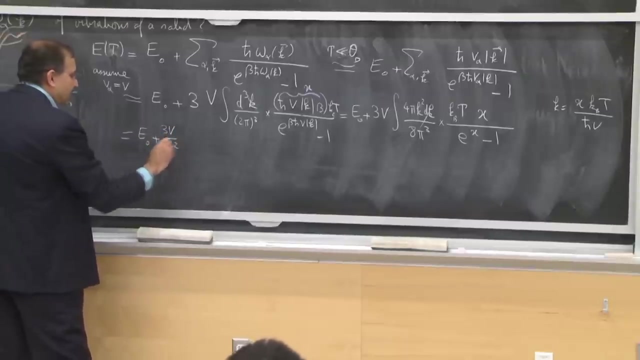 And so, at the next level of approximation, this k squared dk, I will write in terms of x squared dx. And so what do I have? I have e0.. I have 3v divided by 2 pi squared, And I have kt. 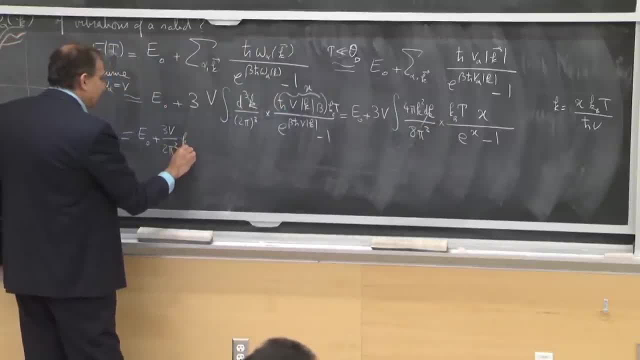 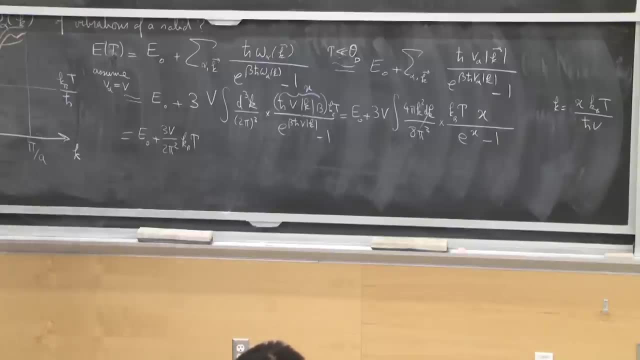 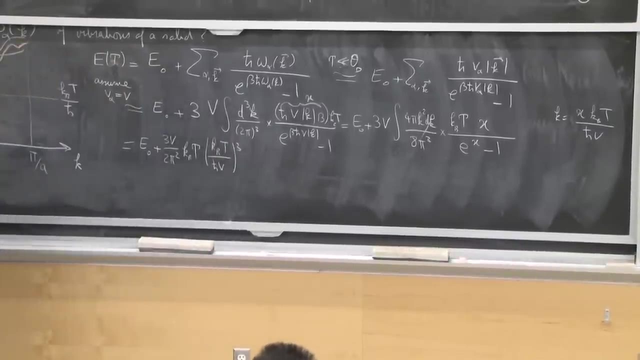 Because of this factor of kt that I will take outside. I have a kt, I have a k squared dk that I want to replace with x squared dx And that will give me an additional factor of kt over h bar v cubed. And then I have an integral 0 to 0 dx, x cubed, e to the x minus 1.. 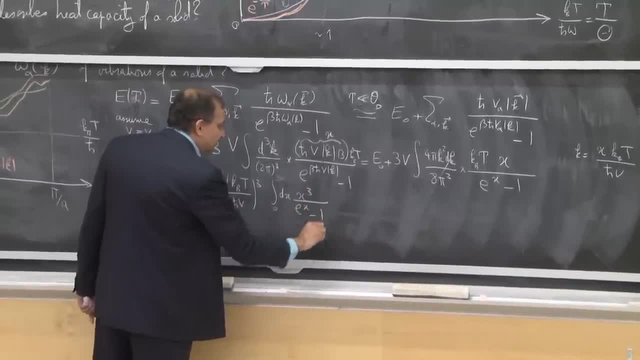 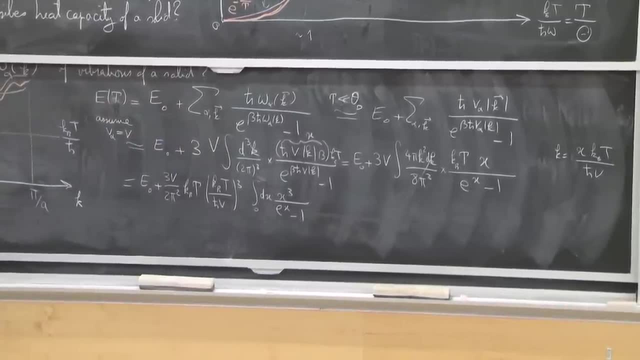 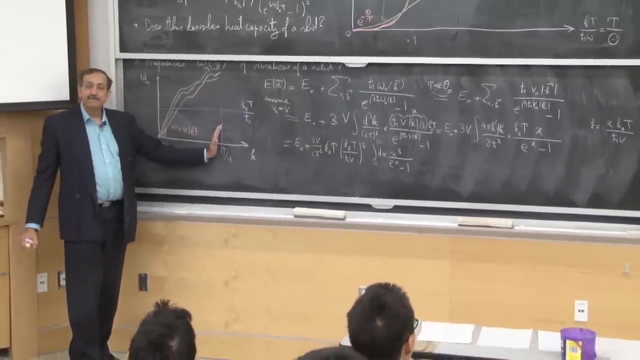 OK, So I have a k squared dk that I want to replace with x squared dx, And that will give me an additional factor of kt over h bar v cubed. OK, Now, in principle, when I start with this integration, I have a finite range for k, which presumably 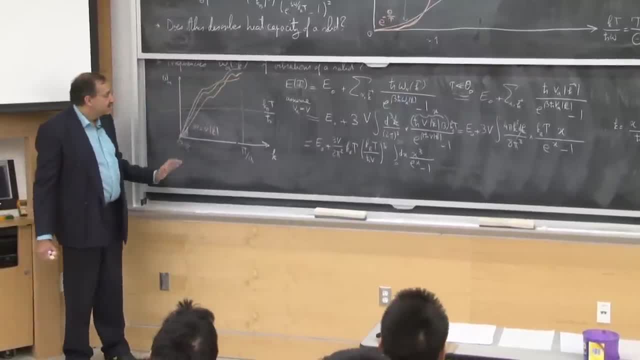 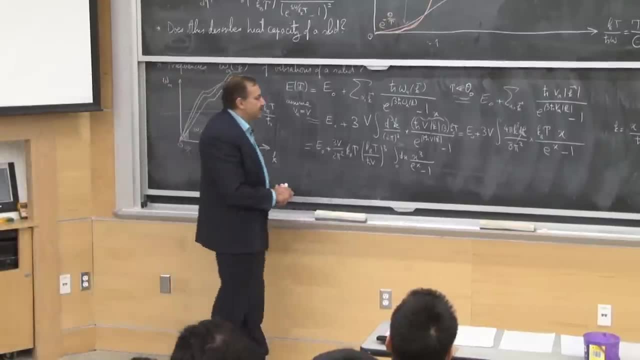 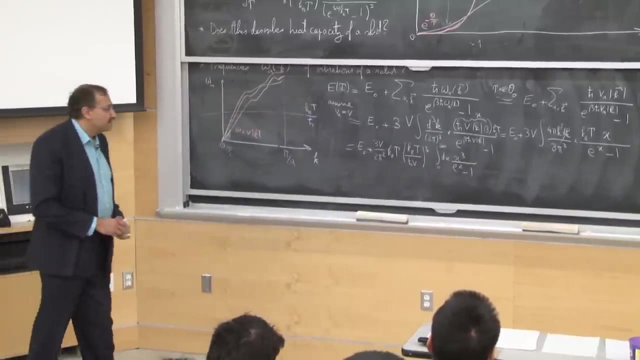 would translate into a finite range for x, But in reality none of these modes is contributing. So I could extend the range of integration all the way to infinity And make a very small error at low temperatures, And the advantage of that is that then this: 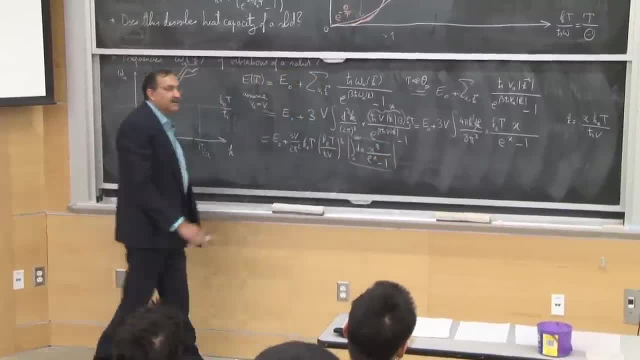 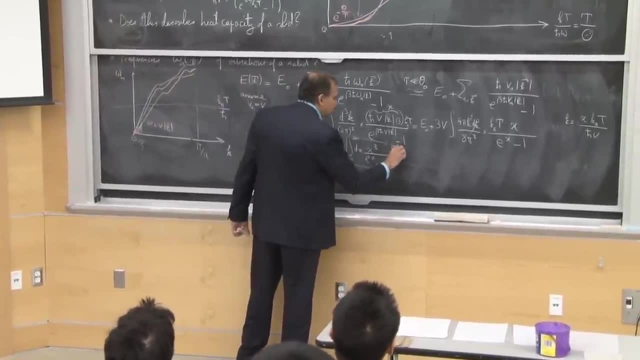 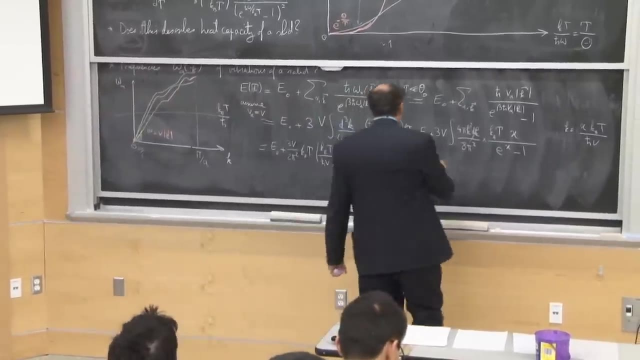 becomes a definite integral, something that you can look up in tables, And its value is in fact pi to the fourth over 15.. So, substituting that over there, what do we have? We have that the energy is E0 plus. 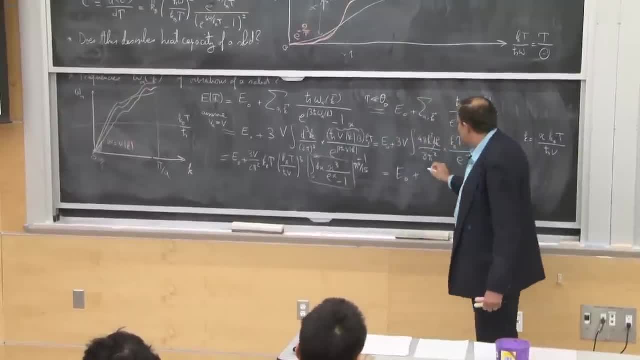 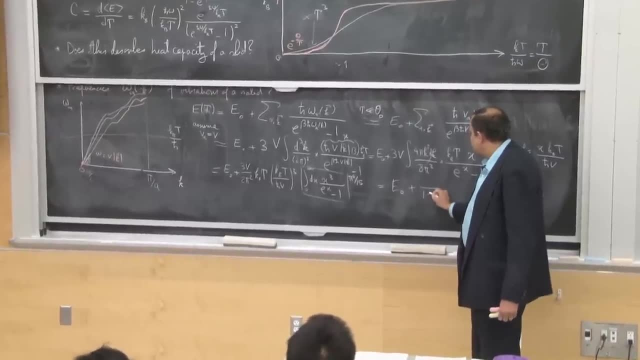 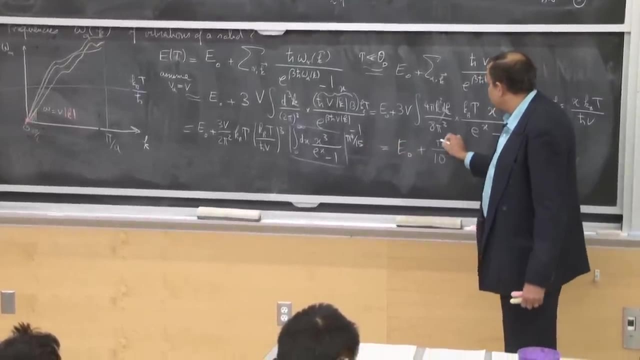 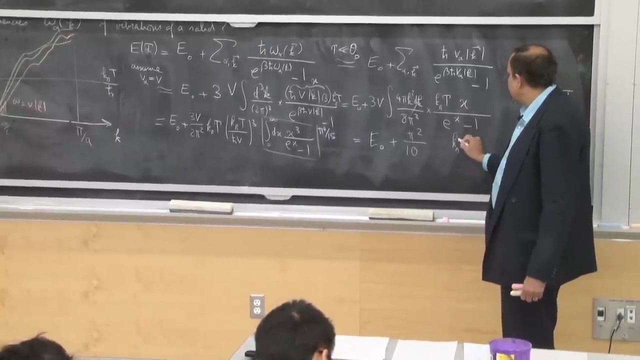 OK, So we have 3 divided by 15 will give me 5, which turns the 2 into a 10.. I have pi to the fourth divided by pi squared, So there's a pi squared that will survive out. here I have a kt. 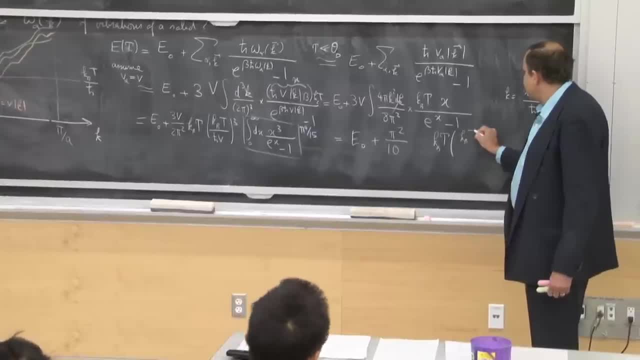 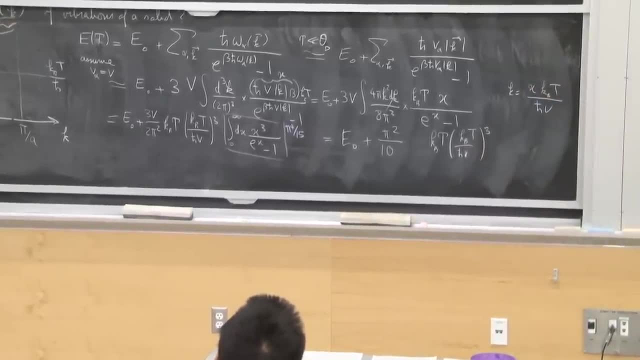 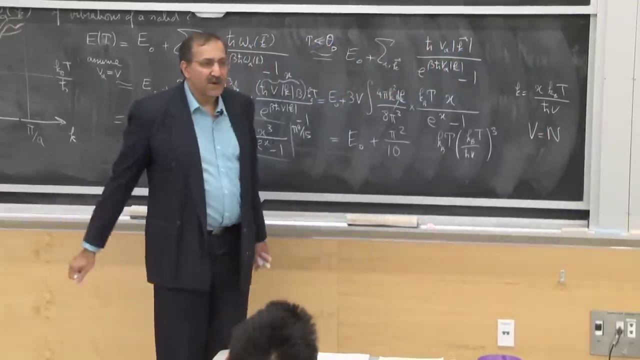 I have kt over h bar- OK, OK, Over h bar, v cubed. And then I have a factor of volume. What volume is proportional to the number of particles that I have in the system? times the size of my unit cell. let's call that a cubed. 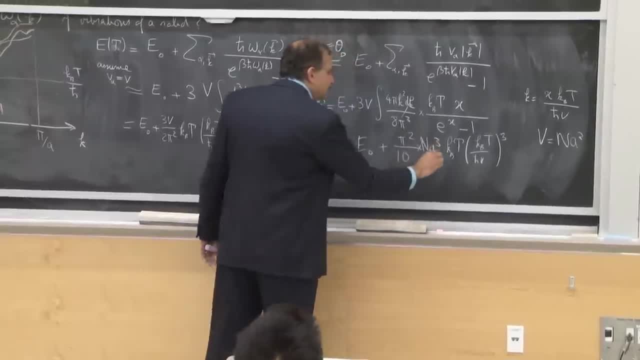 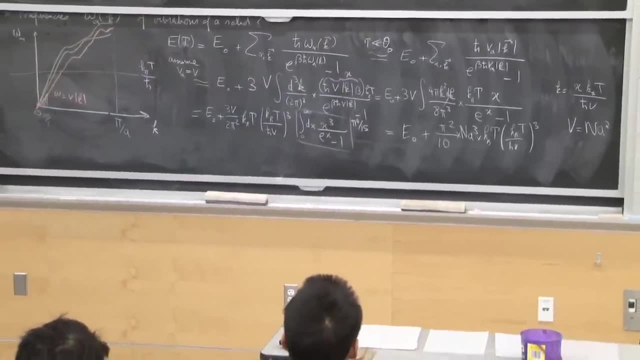 So this I can write as n a cubed. Why do I do that is because when I then take the derivative, I'd like to write the heat capacity per particle. OK, OK. So indeed, if I now take the derivative which 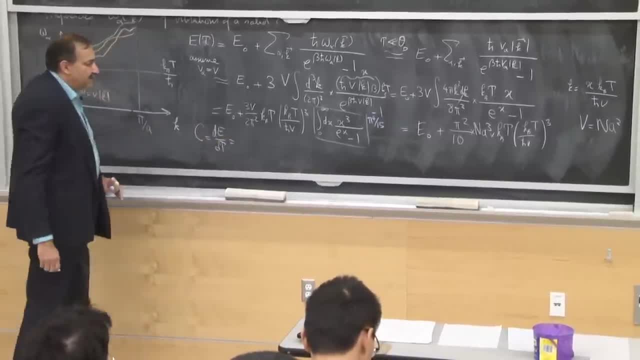 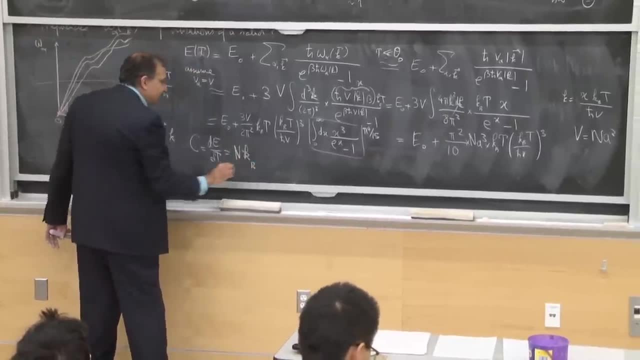 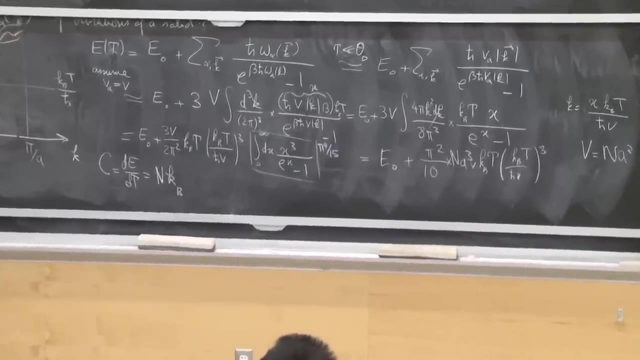 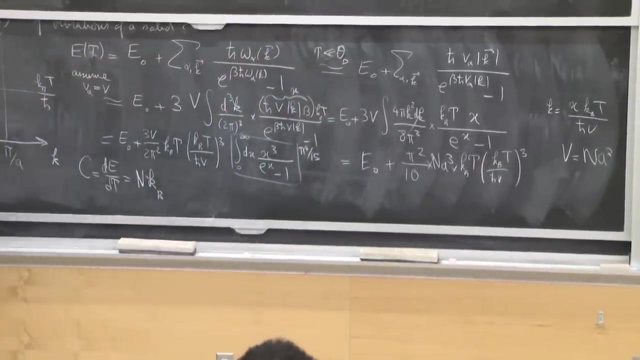 is dE by dt, the answer will be proportional to n and kb, the number of particles, and this kb, which is the function, the unit of heat capacities. The overall dependence is t to the fourth. So when I take derivatives I will get 4t to the fourth. 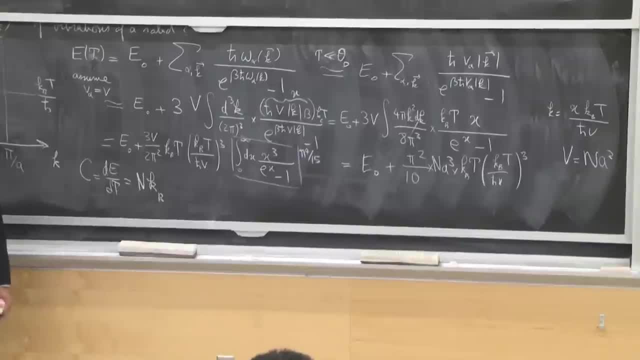 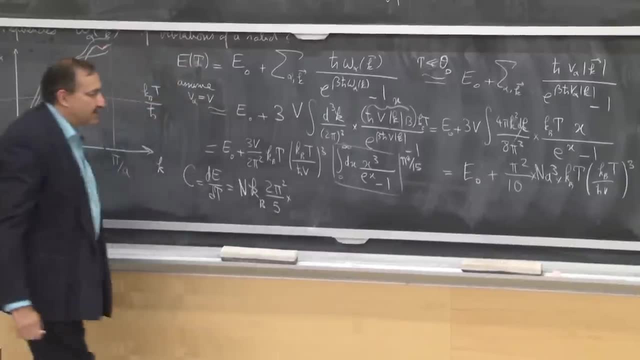 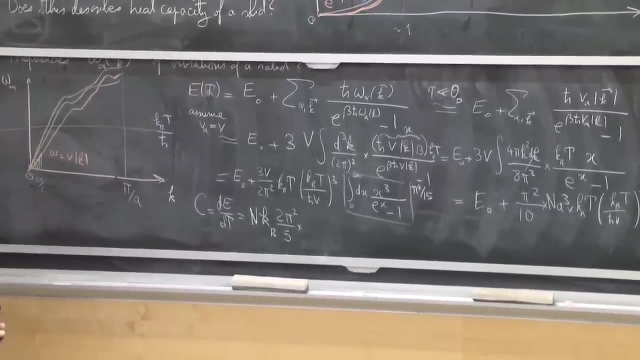 OK, So t cubed, That 4 will change the 1 over 10 to 2 pi squared over 5.. And then I have the combination kb, t, h, bar, v And that factor of a raised to the third power. So the whole thing is proportional to t cubed. 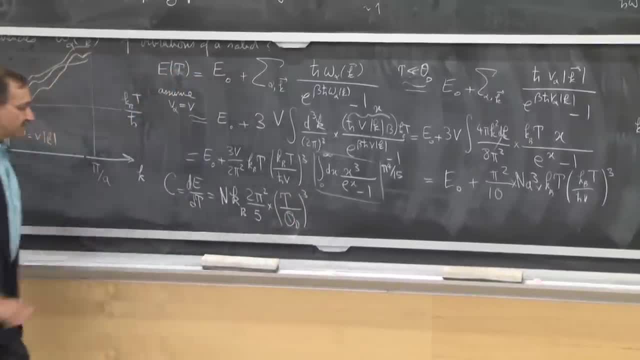 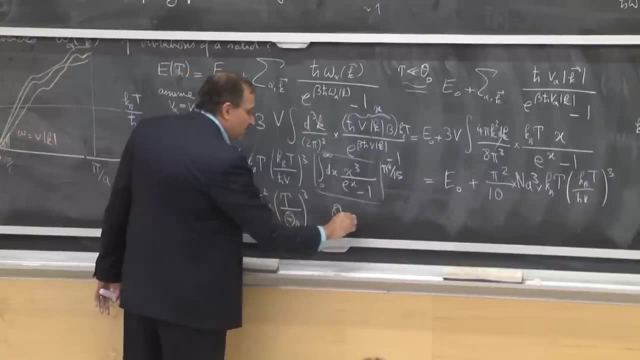 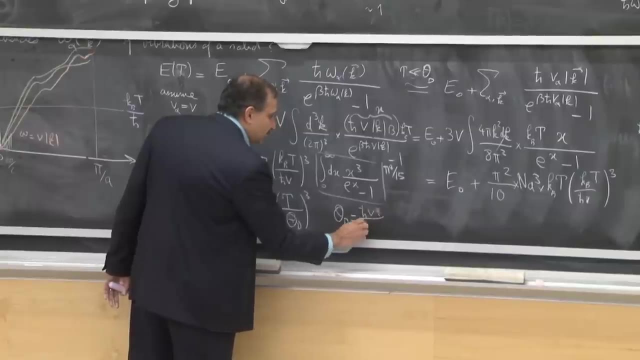 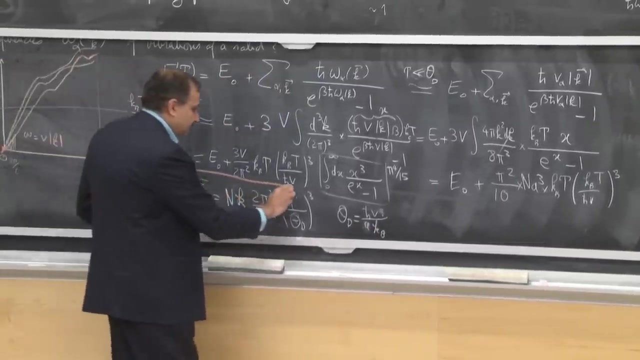 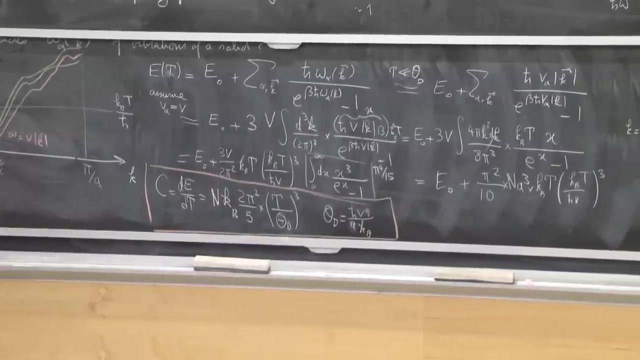 And the coefficient. I will call theta d for d by, And theta d I have calculated to be h bar v over a h bar v. a over kb. No, h bar v over a kb. OK, So the heat capacity of the solid at low temperatures. 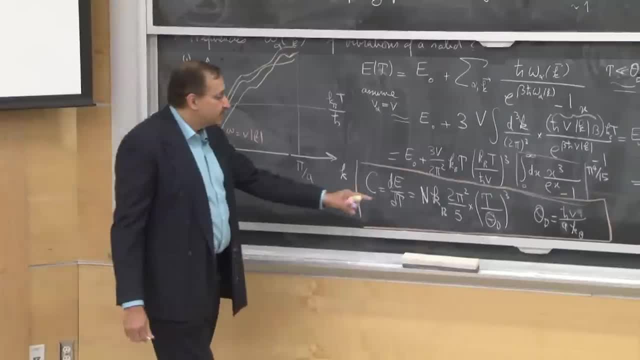 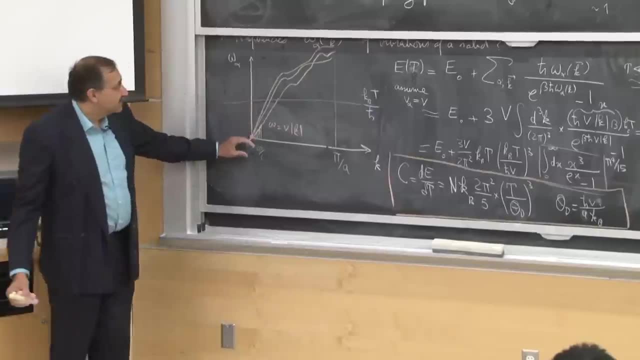 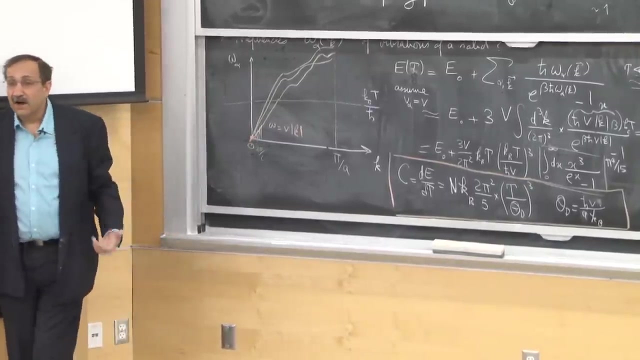 is going to be proportional, of course, to n kb, But most importantly, it is proportional to t cubed, And t cubed just came from this argument that I need low omegas, And how many things I have at low omega. 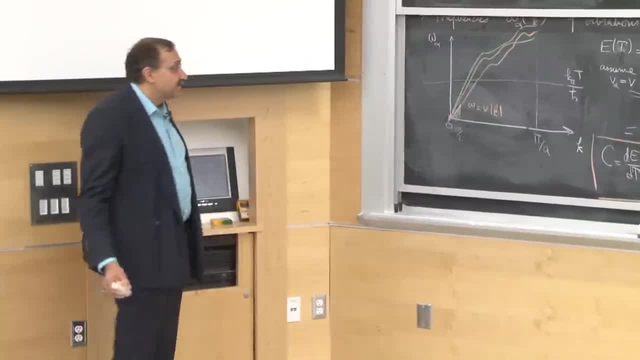 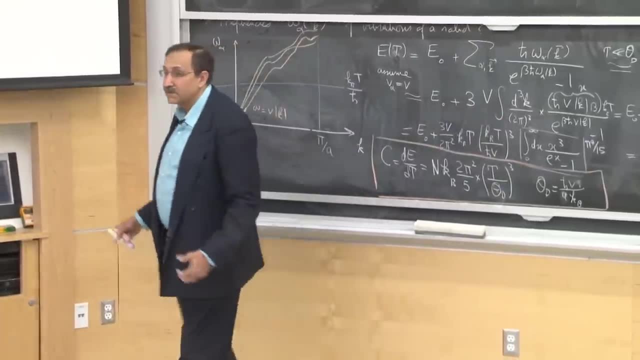 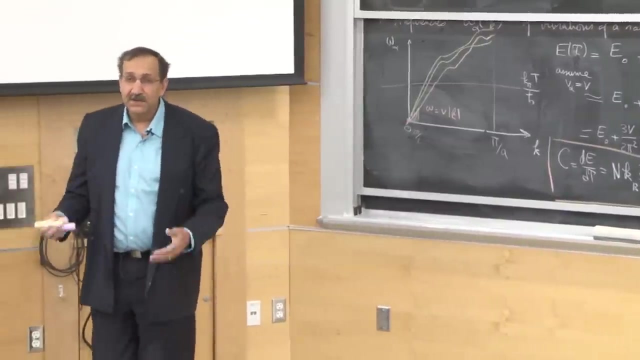 how many frequencies do I have that are vibrating? The number of those frequencies is essentially the size of a cube in k space. So it goes like this: Match Match Maximum k cubed in three dimensions. In two dimensions it would be squared, and all of that. 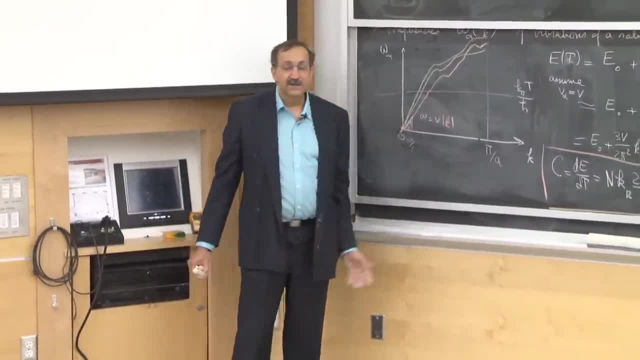 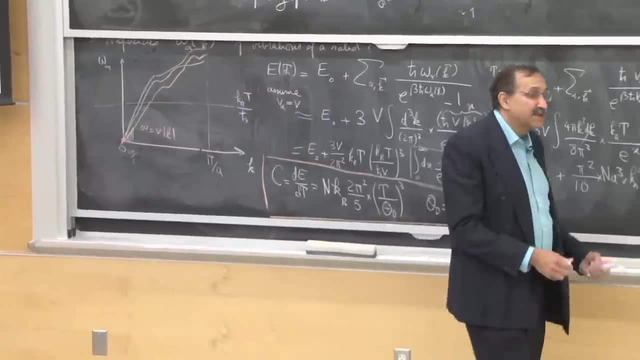 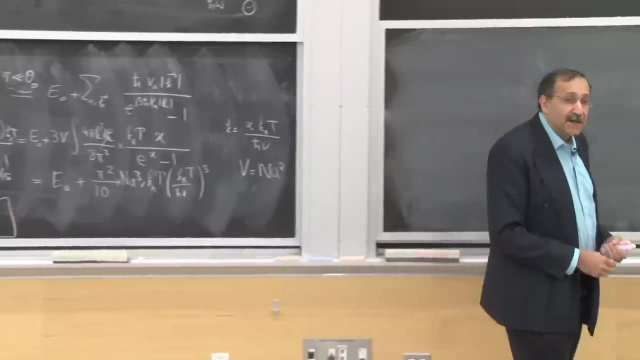 So it's very easy to figure out from this dispersion relation what the low temperature behavior of the heat capacity has to be, And we will see that this is in fact predictive, In that later on in the course we will come an example where the heat capacity of a liquid which 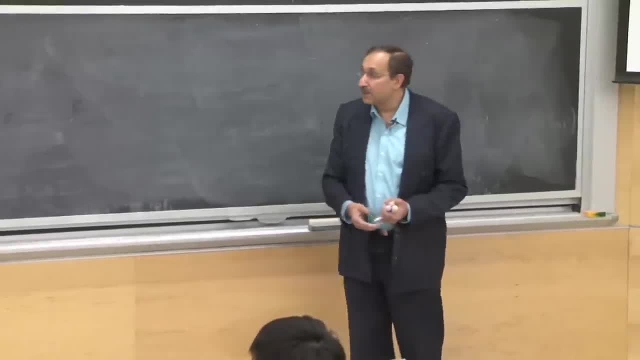 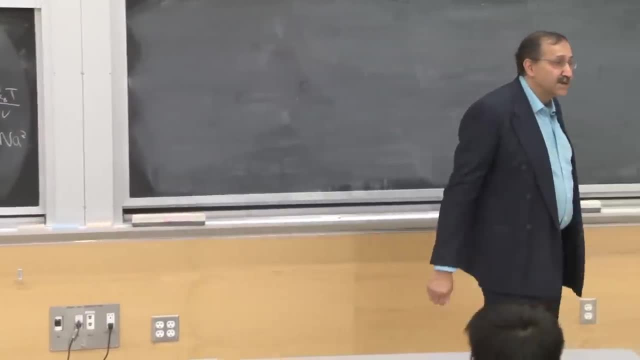 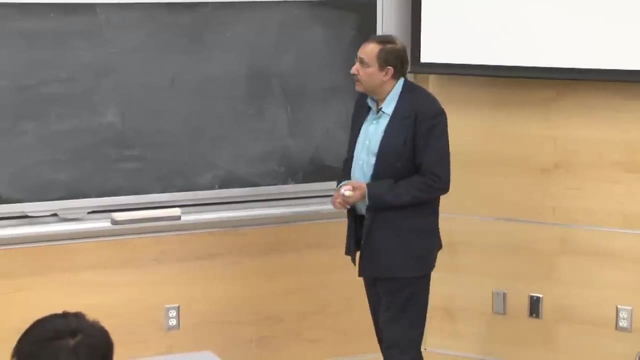 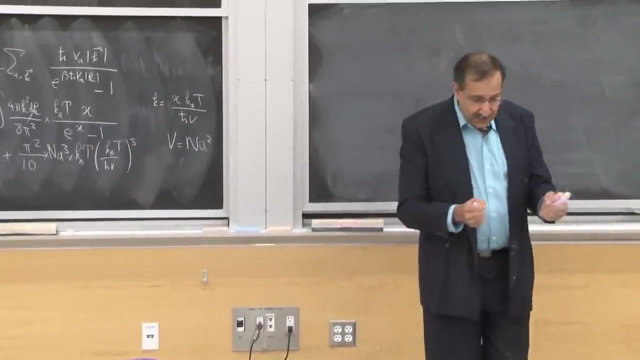 was helium was observed to have this t cubed behavior. based on that, Landau immediately postulated that there should be phonon-like dispersion inside that super fluid. So that's the story of the heat capacity of the solid. So we started with the molecule. 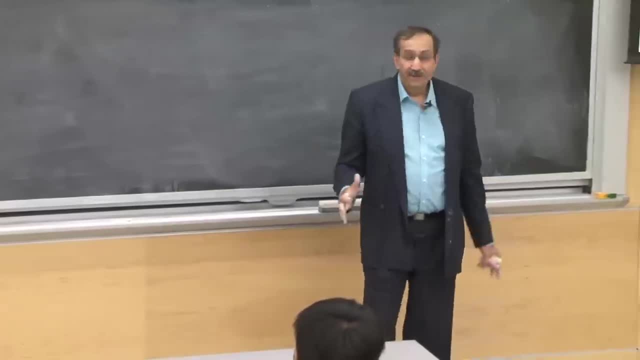 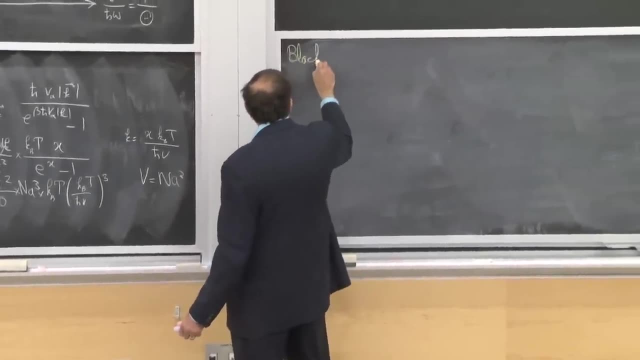 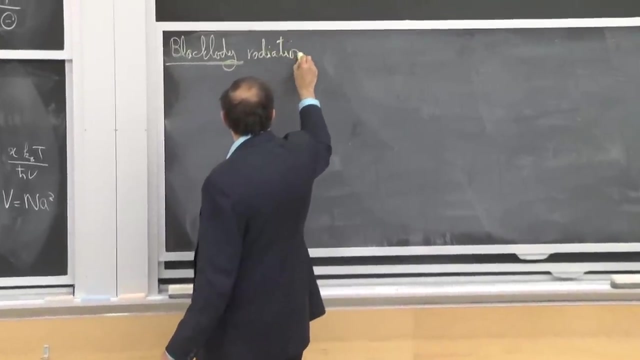 We went from a molecule to an entire solid. Now the next step- that's what I'm going to do- Is I'm going to remove the solid and just keep the box. So, essentially, the calculation that I did, if you think about, 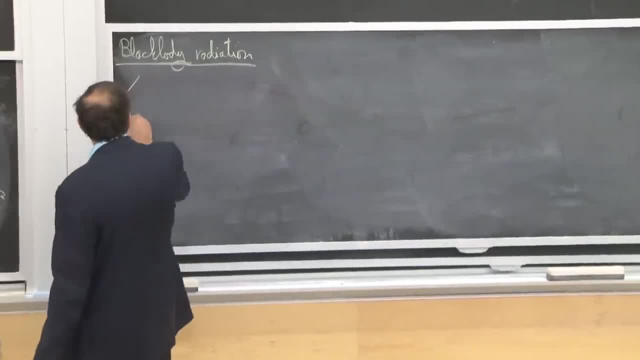 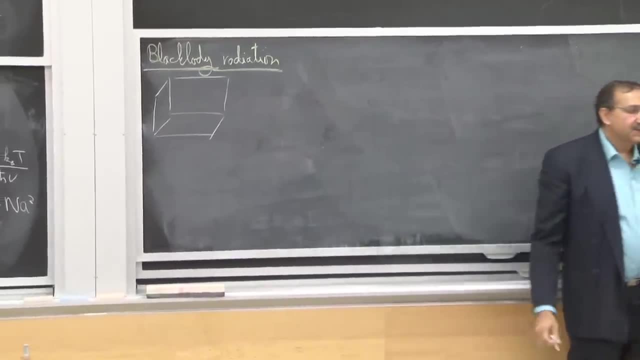 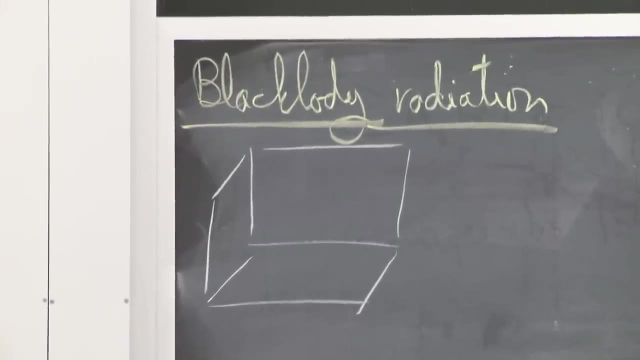 it corresponded to having some kind of a box and having vibrational modes inside the box. But let's imagine that it is an empty box. But we know that. We know that even in empty space we have light. So within an empty box we can still. 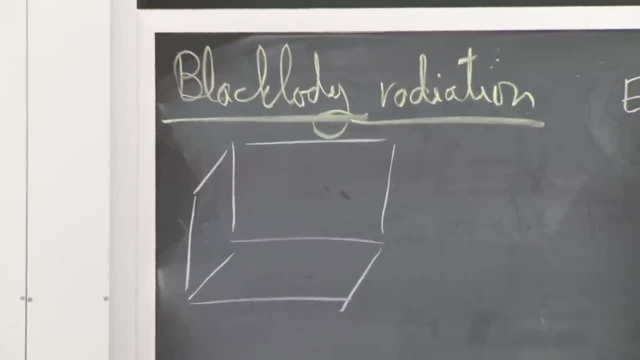 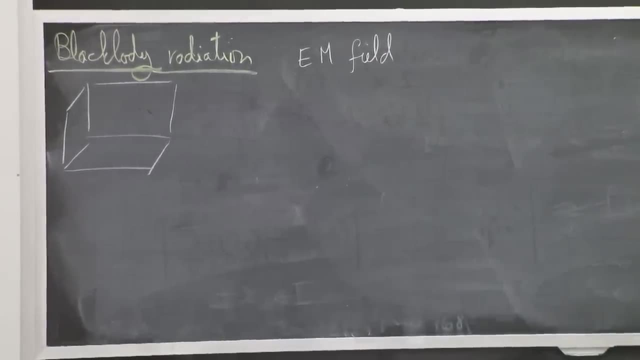 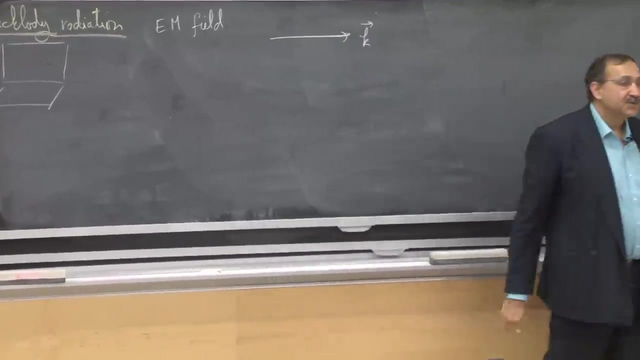 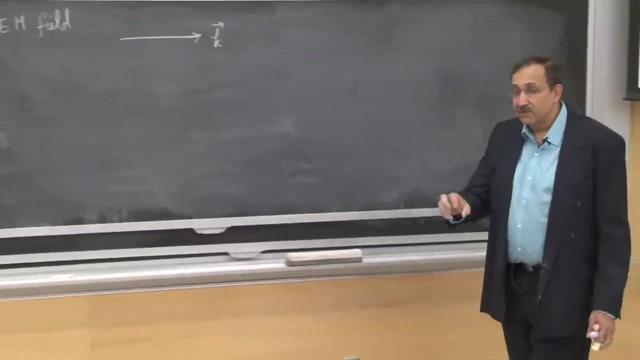 have modes of the electromagnetic field. The modes of the electromagnetic field, just like the modes of a solid, we can characterize by a direction along which oscillations travel, And whereas for the atoms in the solid they have displacement and the corresponding momentum. 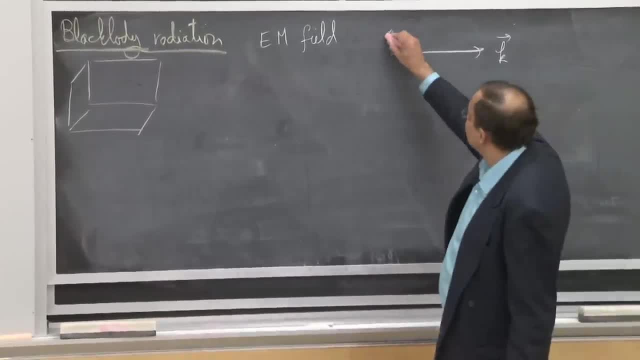 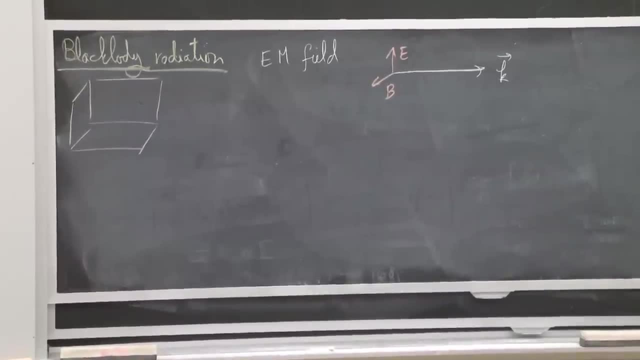 for the electromagnetic field, you have the electric field And its conjugate is the magnetic field, And these things will be oscillating to create for you a wave, except that, whereas for the solid it's oscillating, It's oscillating. 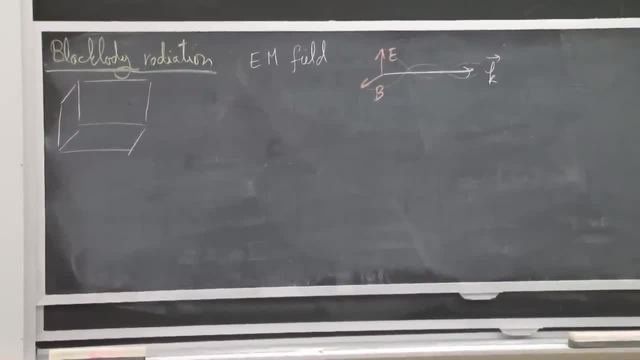 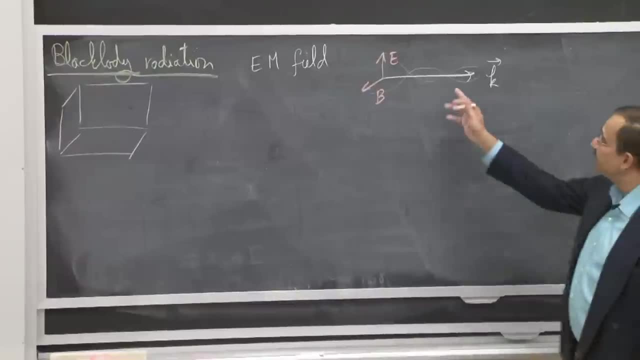 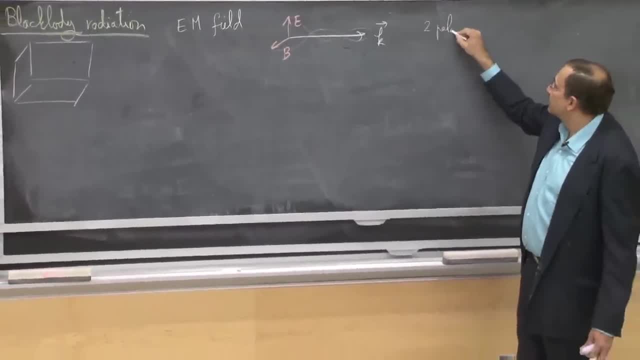 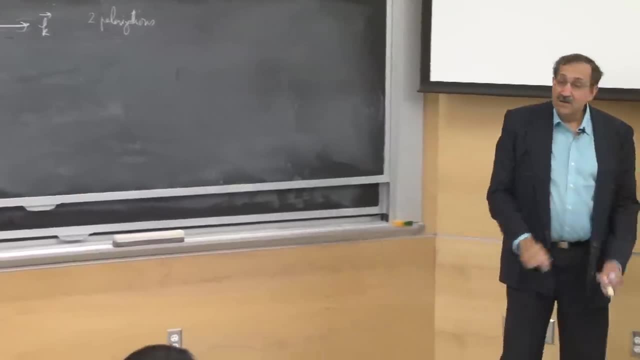 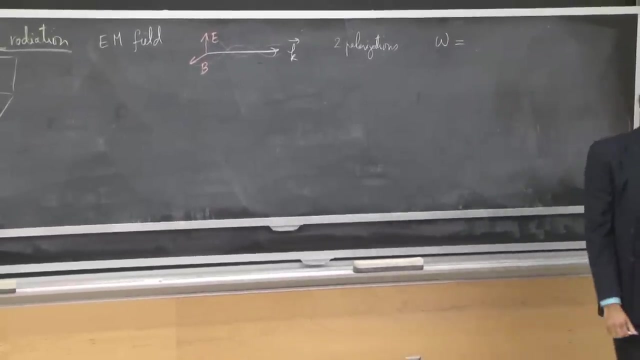 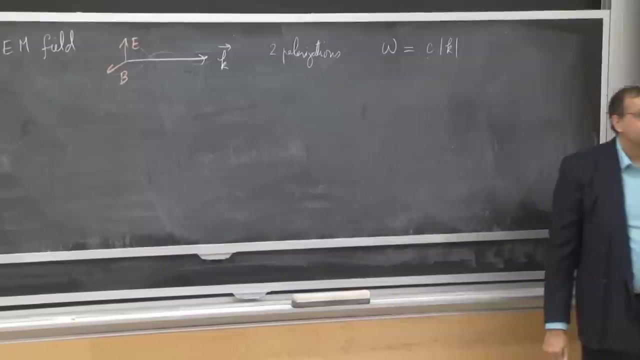 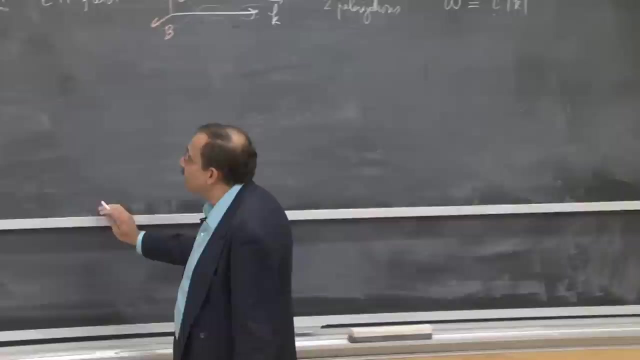 you really have only two polarizations, And but apart from that, the frequency spectrum is exactly the same as you would have for the solid. It's at low temperature, replacing the V that we have with the speed of light, And so you would say, OK, if I were. 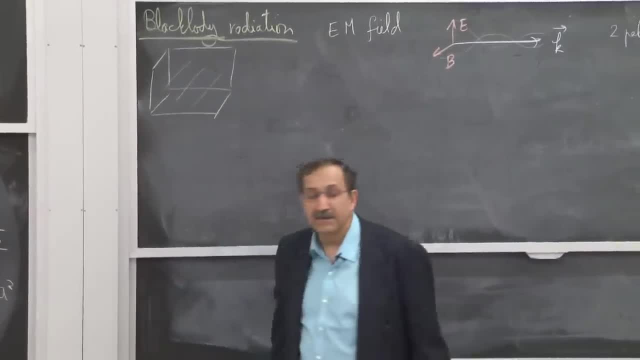 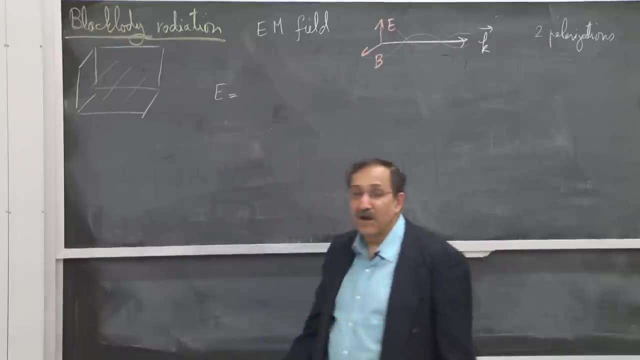 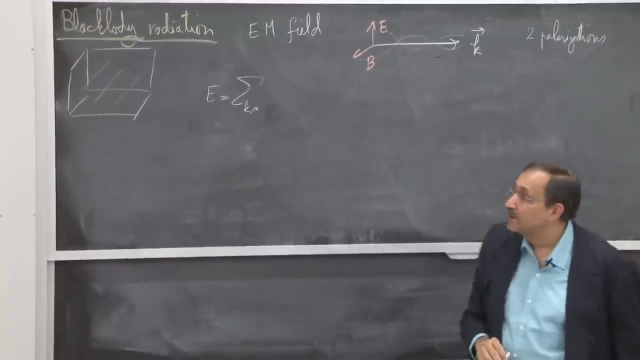 to calculate the energy content that is inside the box. what I have to do is to sum over all of the modes and polarization, And that's what we're going to do in the next class, Regarding each one of these as a harmonic oscillator. 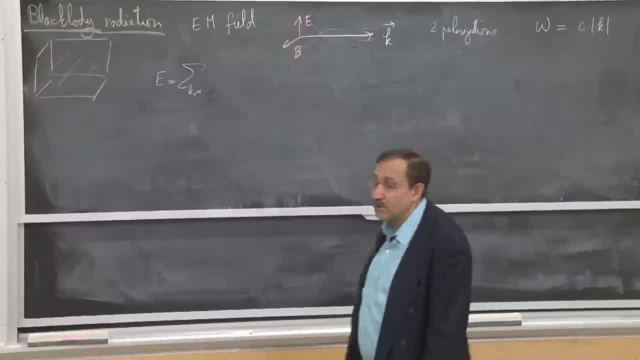 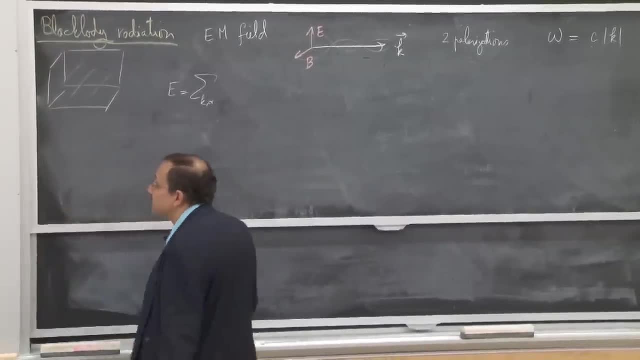 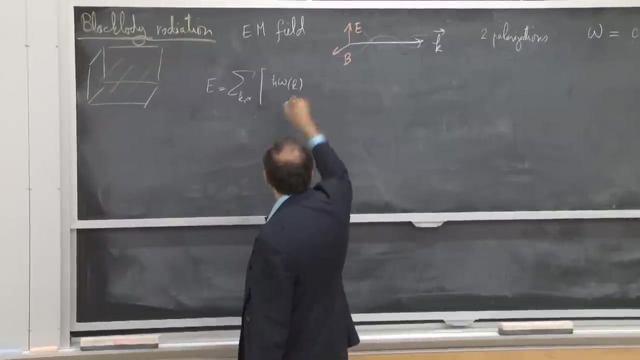 going through this system of quantizing according to these old quantum mechanics, the harmonic oscillators, I have to add up the energy content of each oscillator. So what I have is this h bar omega of K, And then I have 1 half plus 1 over e to the power of k. 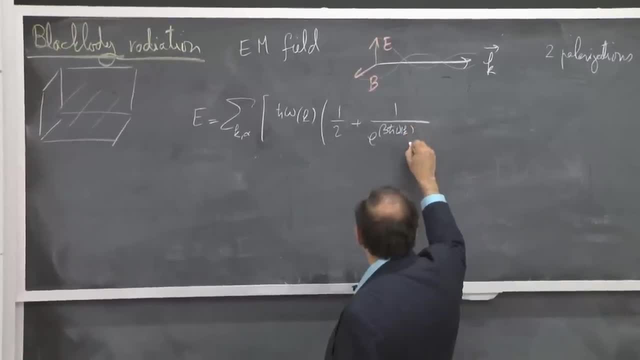 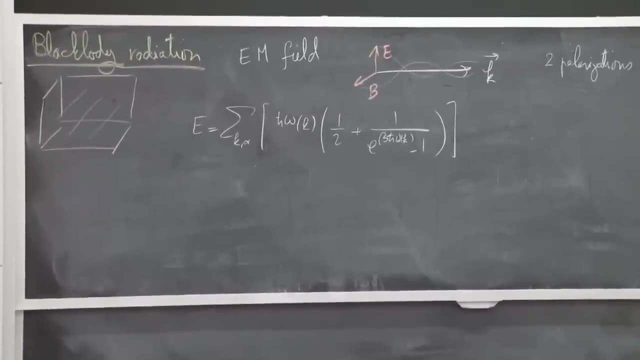 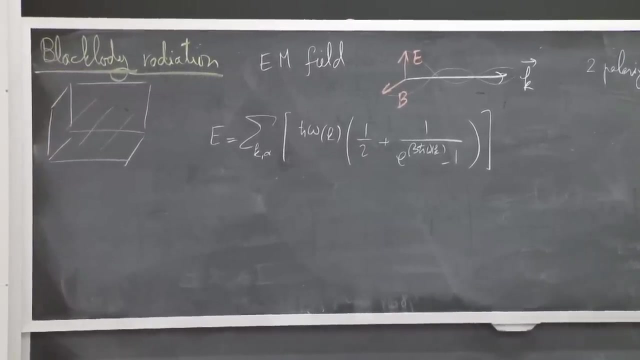 OK, e to the beta h bar omega of k minus 1.. And then I can do exactly the kinds of things that I had before, replacing the sum over k with a V times an integral. So the whole thing would be, first of all, 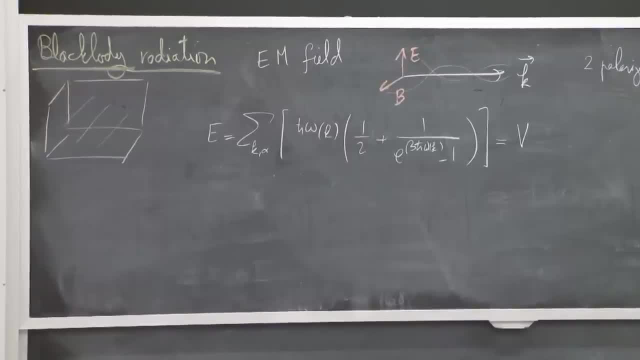 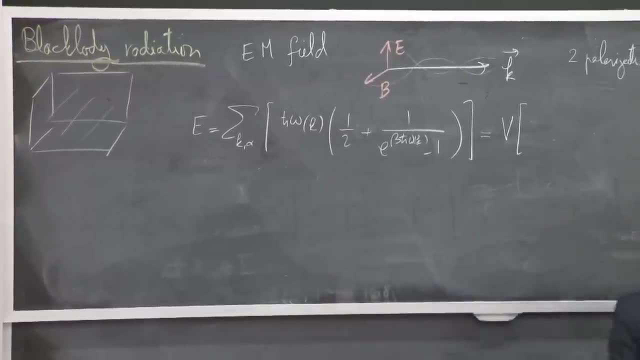 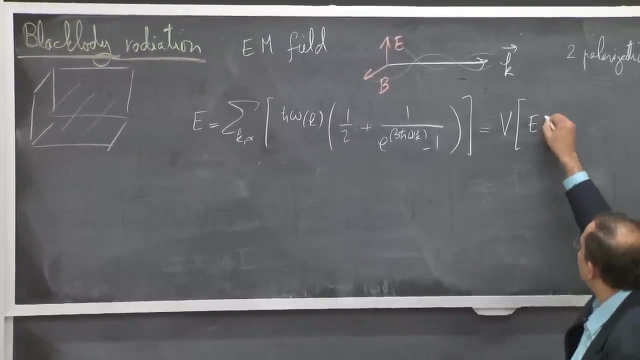 proportional to V. in going from the sum over k to the integration over k I would have to. I would have to add all of these h bar. omega over 2's Has no temperature dependence, so let me just again call it some E0.. 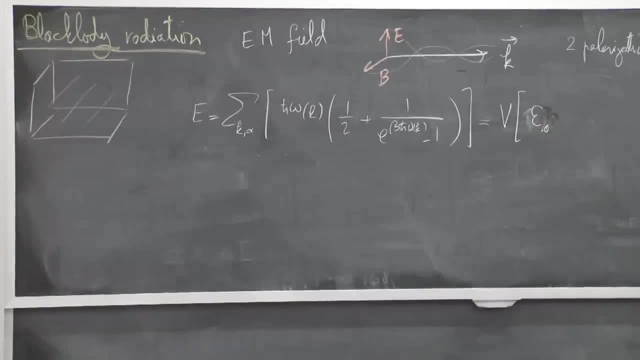 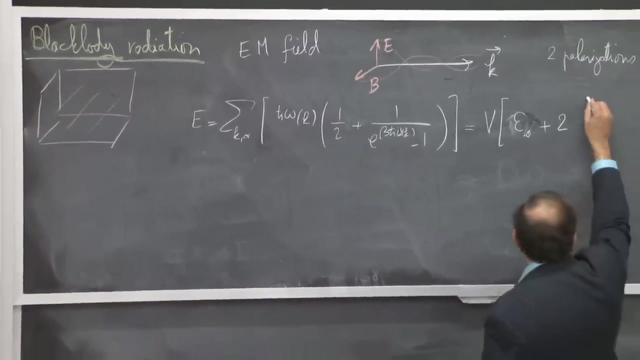 Let's call it epsilon 0, because it's more like an energy density, And then I have the sum over all of the other modes. There are two polarizations, So as opposed to the three that I had before, I have two. I have again the integral over k. 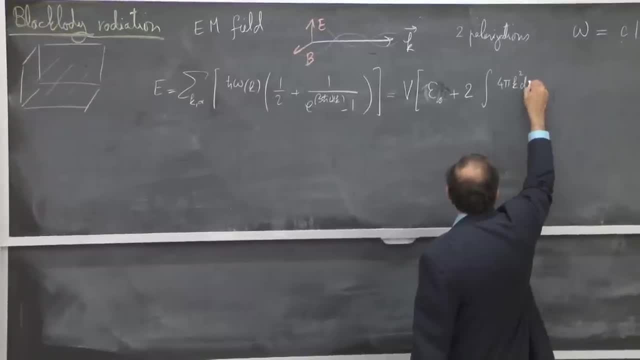 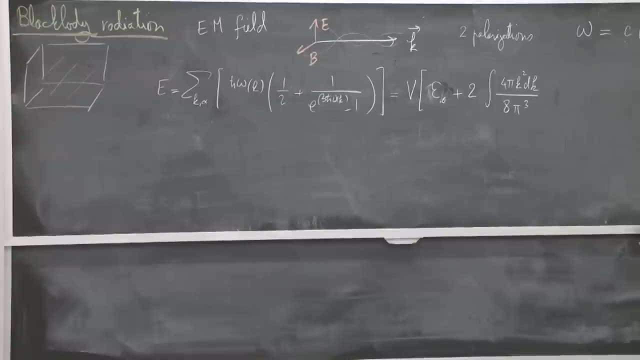 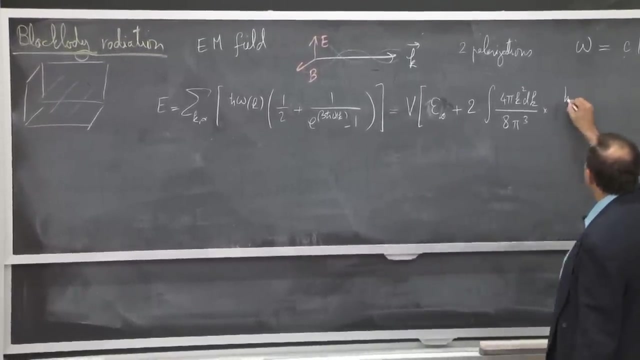 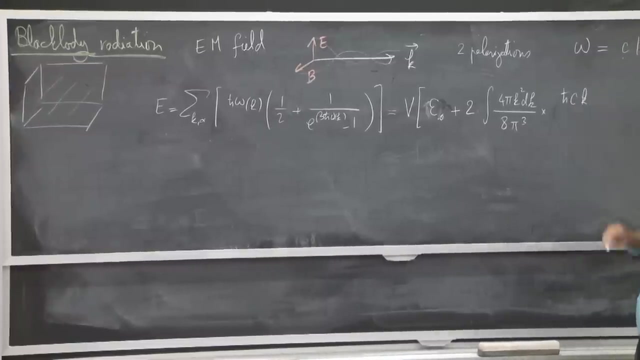 I have 4 pi k squared dk divided by 8 pi cubed, which is part of this density of state calculation. I have again a factor of h bar omega. Now I realize that my omega is ck, So I simply write it as h bar ck. 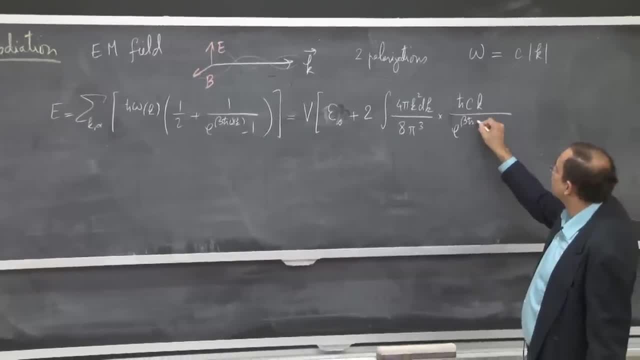 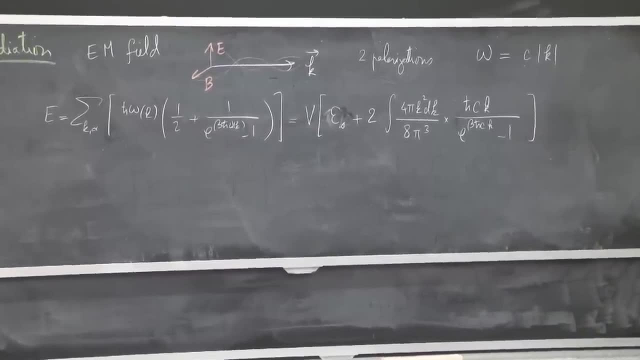 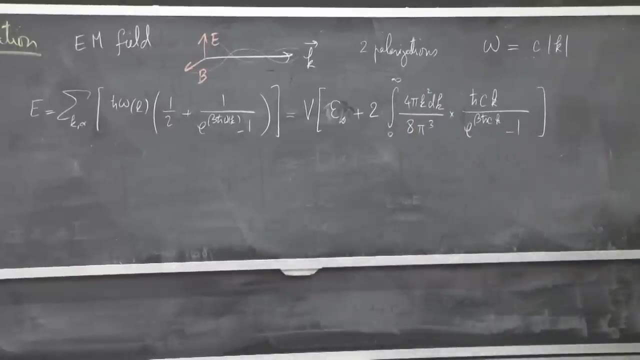 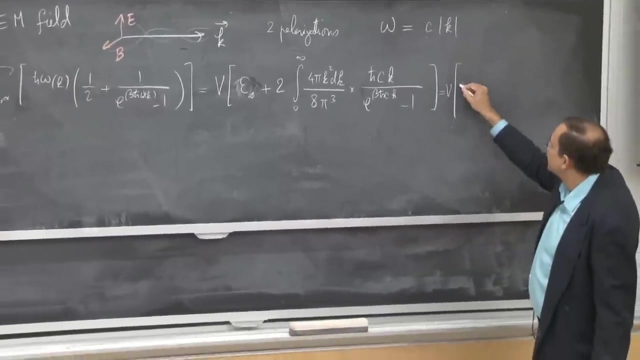 And then I have e to the beta h bar, omega h bar, ck minus 1.. So we will again allow this to go from 0 to infinity. And what do we get? We will get V epsilon 0 plus, well, the 8 and 8 cancel. 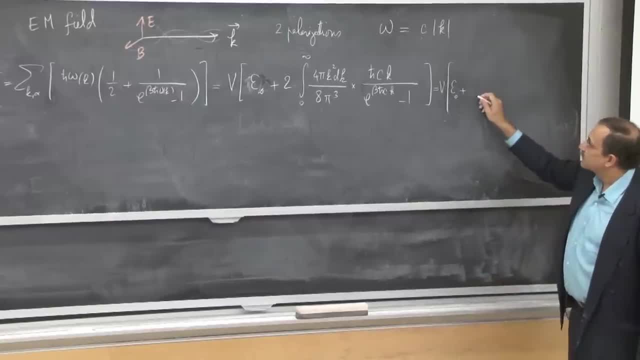 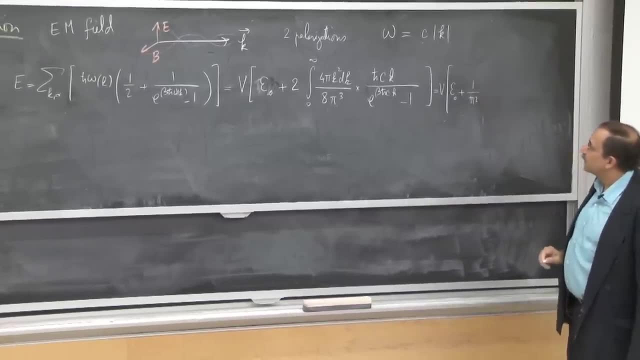 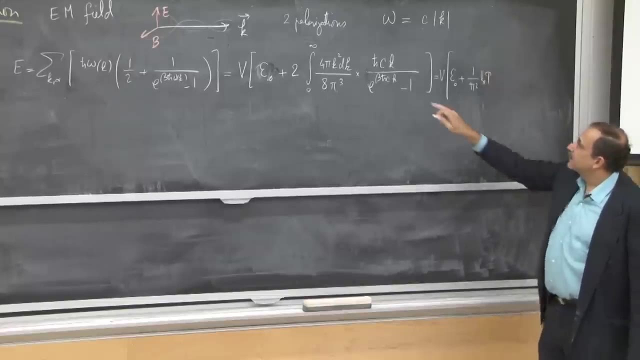 I have pi over pi squared, I have pi over pi squared, So pi over pi cubed. So it will give me a 1 over pi squared. I have one factor of kt Again when I introduce here a beta and then multiply by kt. 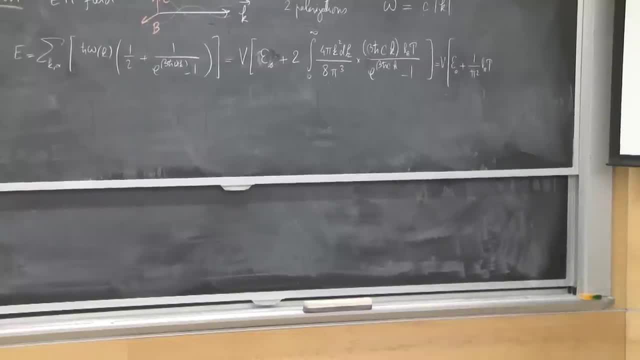 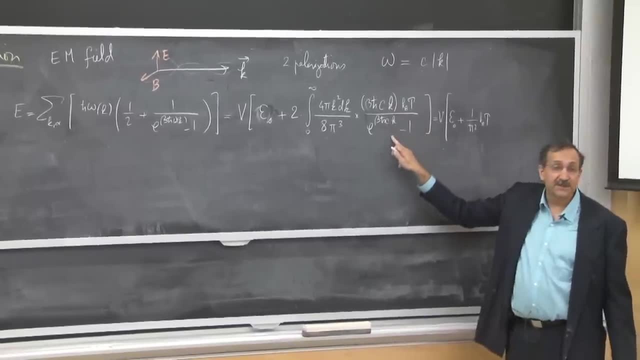 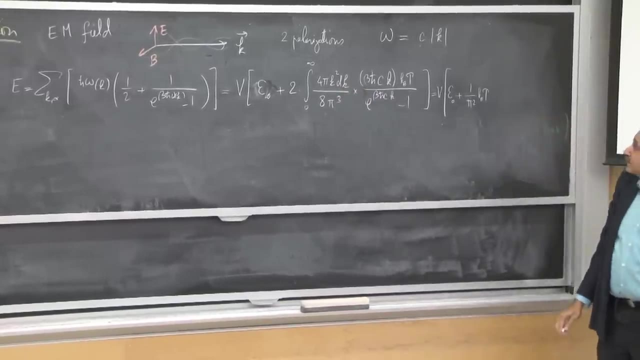 so that this dimensionless combination appears. Then I have, If I were to change, If I were to change variable and call this the new variable, I have a factor of k squared dk, which gives me, just as before over there, a factor of kt over h bar c. 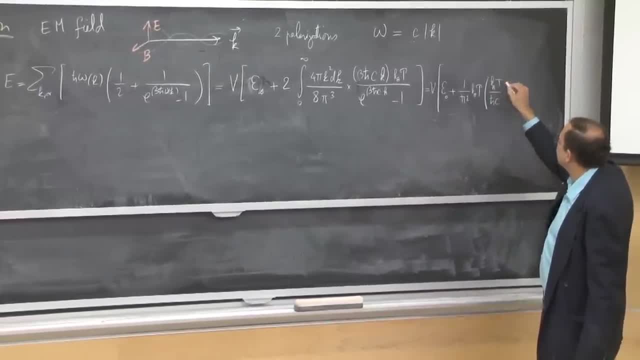 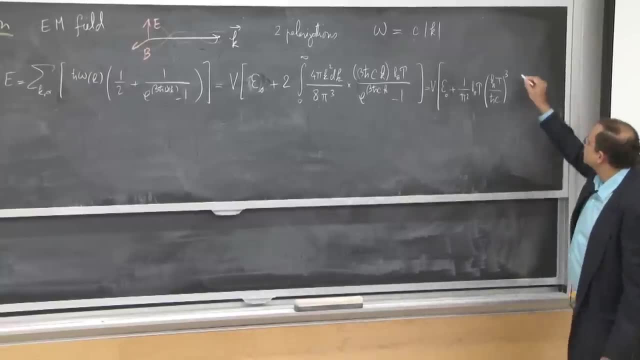 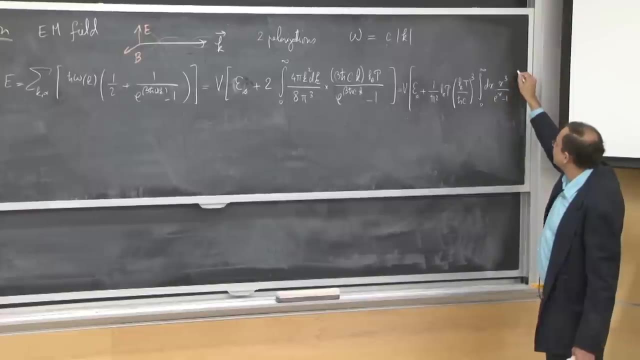 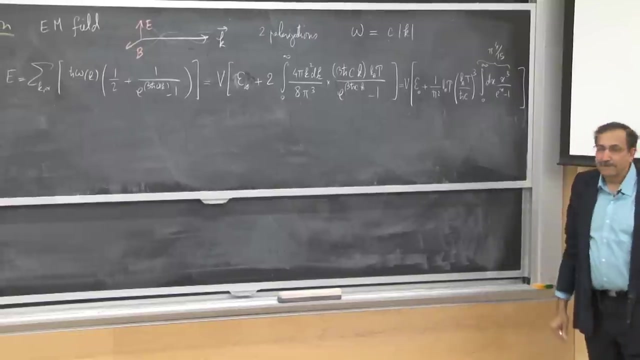 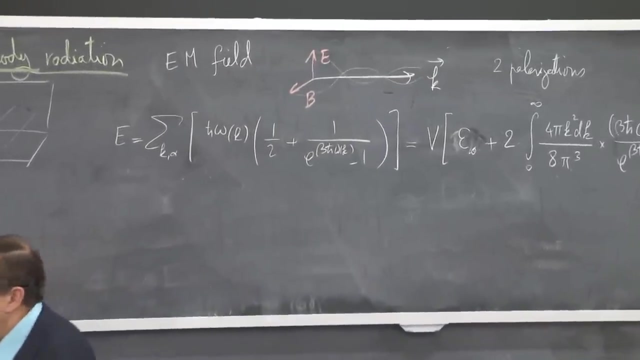 cubed. And then I have this integral left, which is the 0 to infinity dx. This is x cubed, e to the x minus 1.. Which we stated is pi to the fourth over 50.. So the part that is dependent on temperature, the energy content. 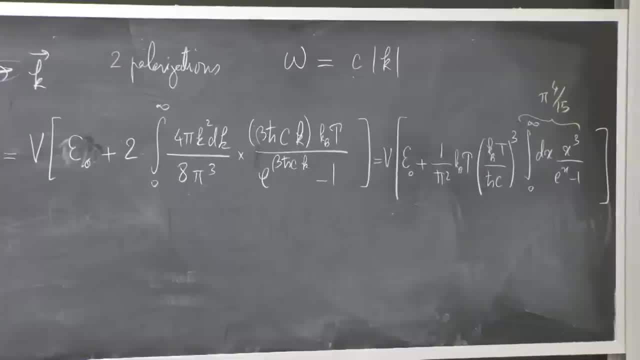 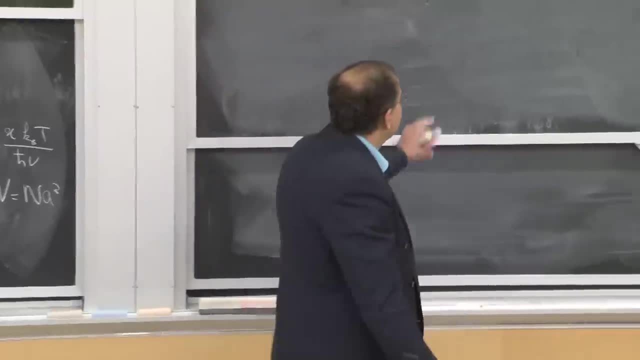 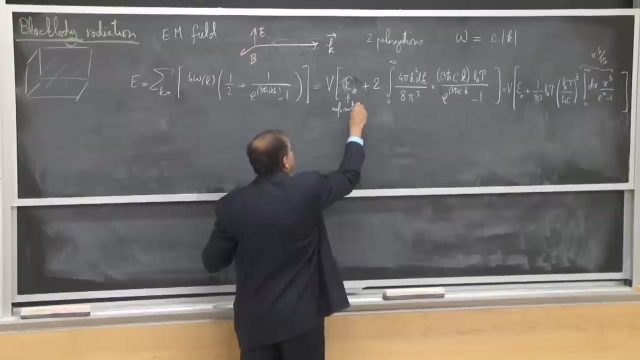 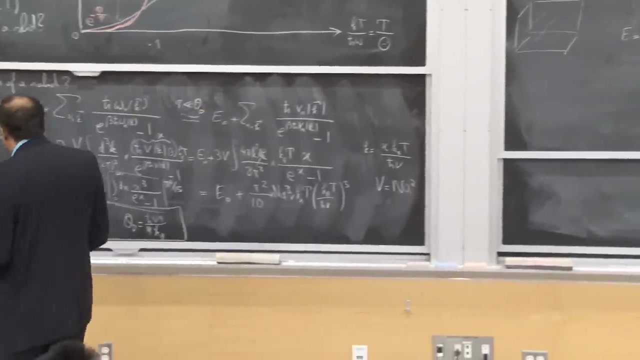 just as in this case, scales as t to the fourth. OK, There is one part that we have over here from all of the zeros which is in fact an infinity, And maybe there is some degree of worry about that. We didn't have to worry about that infinity in this case. 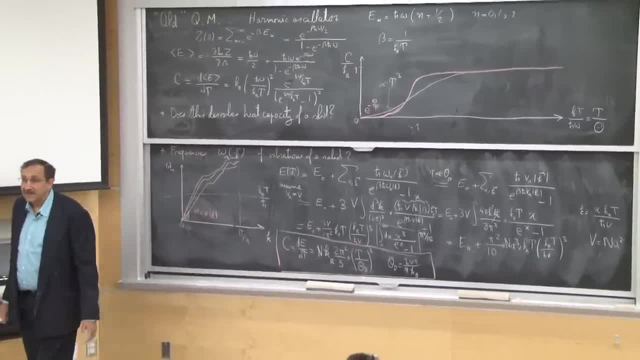 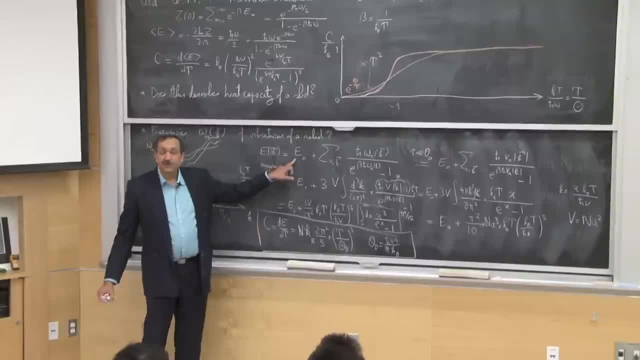 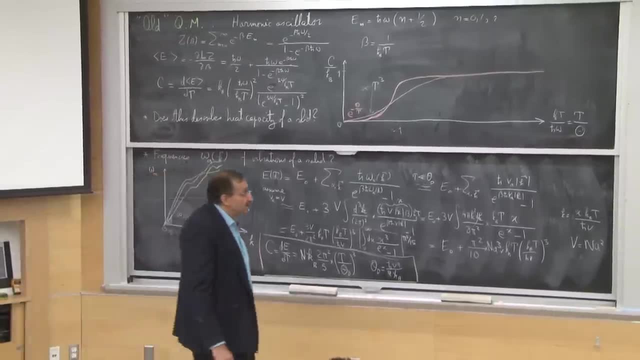 So we would have different. add up properly all of these zero point energies. for this we would have gotten the finite number. It would have been large, but it would have been finite, Whereas here the difference is that there is really no upper cutoff. 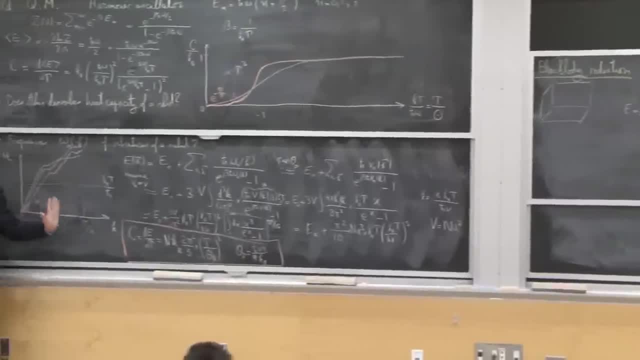 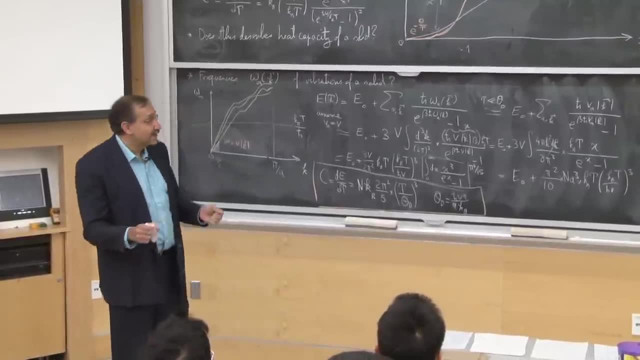 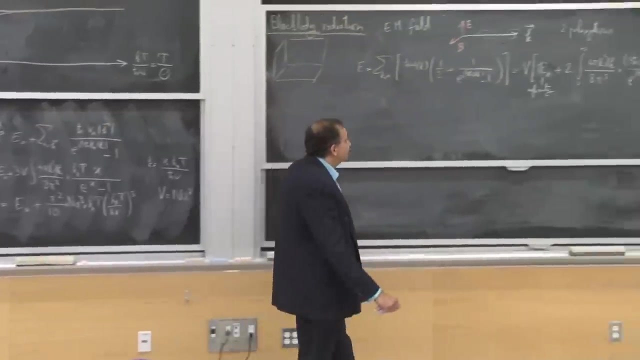 So this k here. for a solid you have a maximum wavelength. You can't, sorry, minimum wavelength. You can't do things shorter than the separation of particles. But for light you can have arbitrarily short wavelength And that gives you this infinity over here. 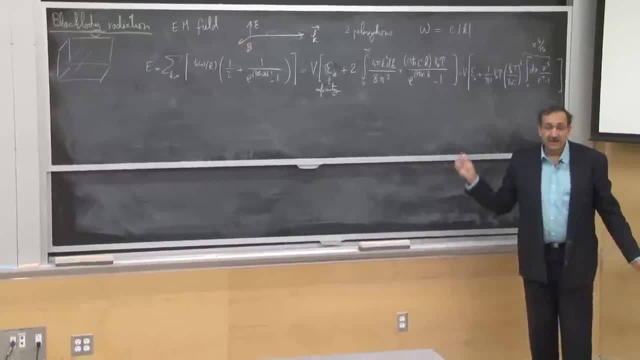 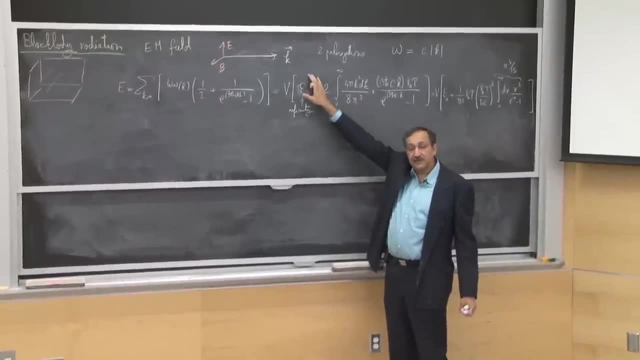 So typically we ignore that. Maybe it is related to the cosmological constant et cetera, But for our purposes we are not going to focus on that at all. And the interesting part is this part that's proportional to t, to the fourth. 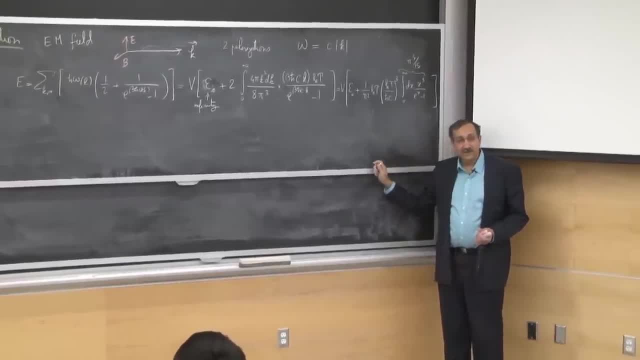 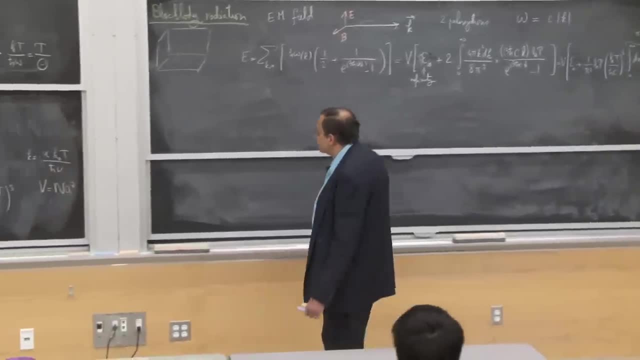 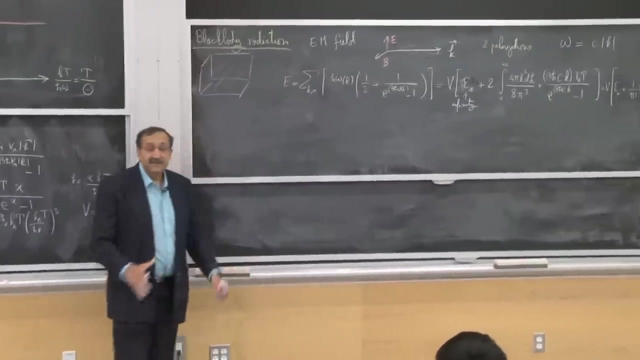 There are two sub-calculations to this that I will do Just give part of the answer, because another part of the answer is something that you do in a problem set. One of them is that what we have here is an energy density. 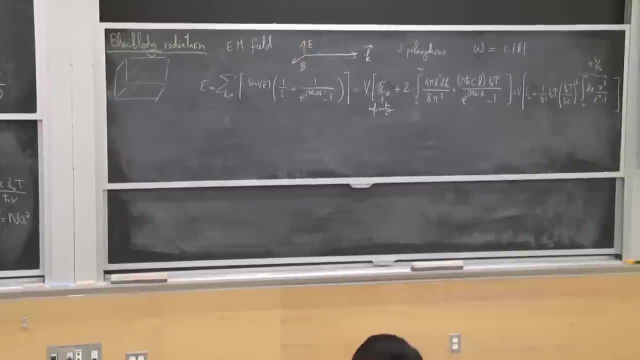 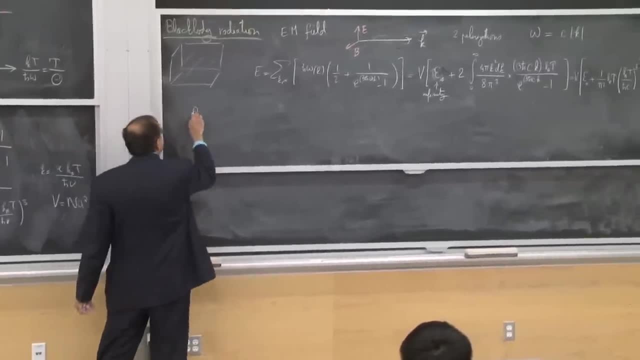 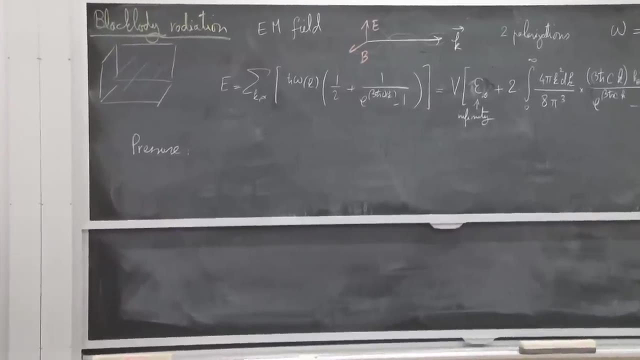 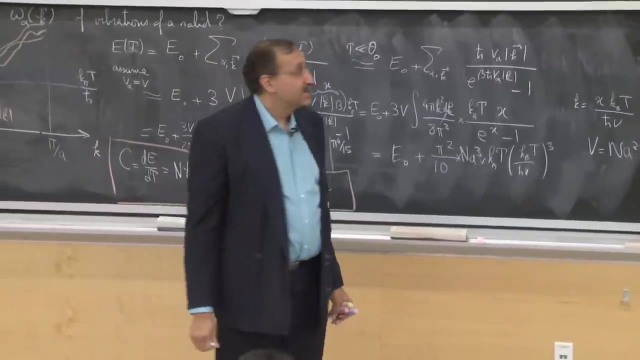 It's proportional to volume, And we have seen that energy densities are related to pressures. So indeed there is a corresponding pressure. That is, if you are at the temperature t, this collection of vibrating electromagnetic fields exerts a pressure on the walls of the container. 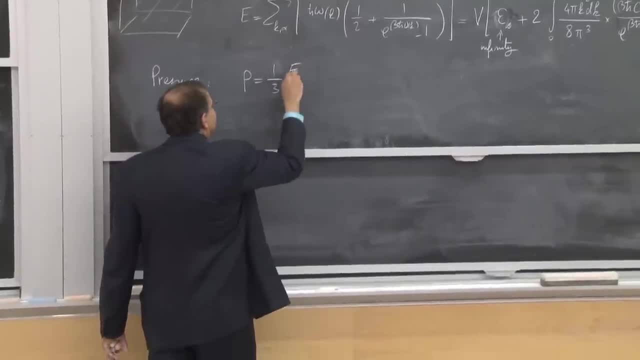 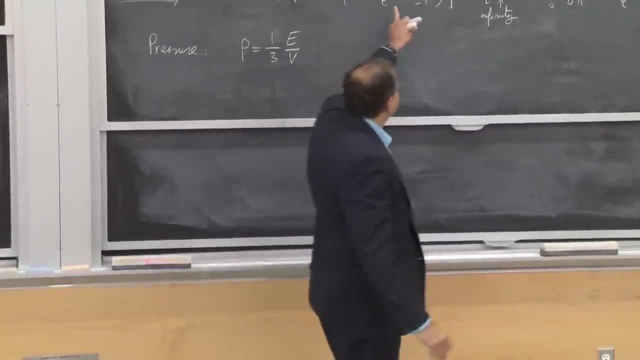 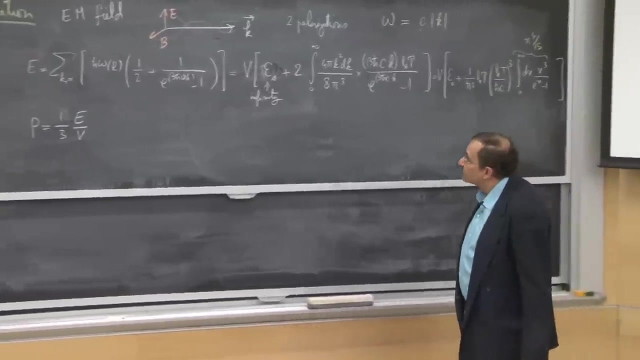 This pressure is related to energy density. The factor of 1 third comes because of this dispersion relation And you can show that in one of the problem sets or you know that already. So that would say that you have an energy density. You would say that you would have essentially something. 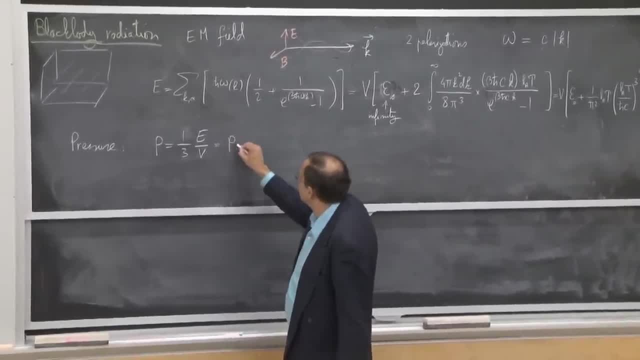 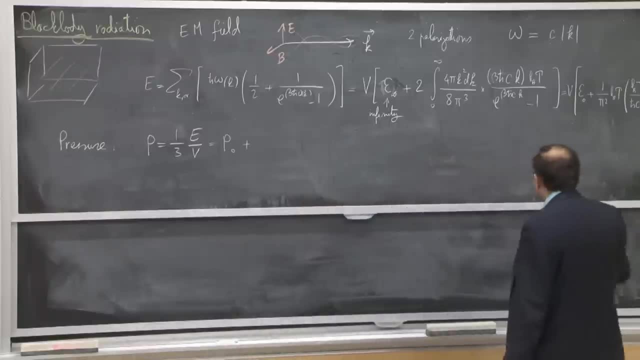 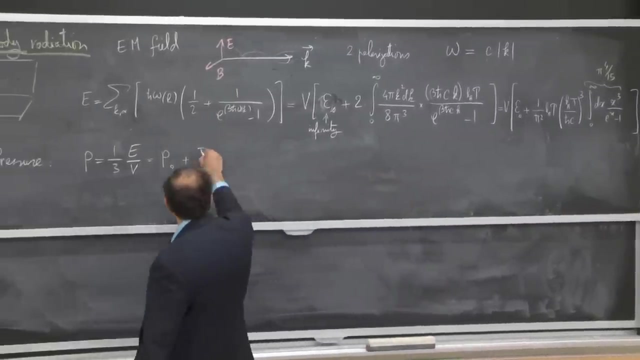 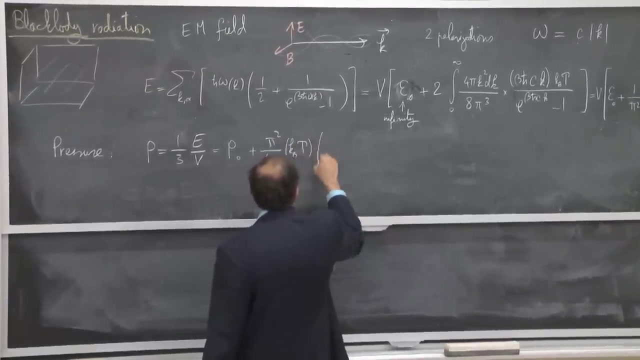 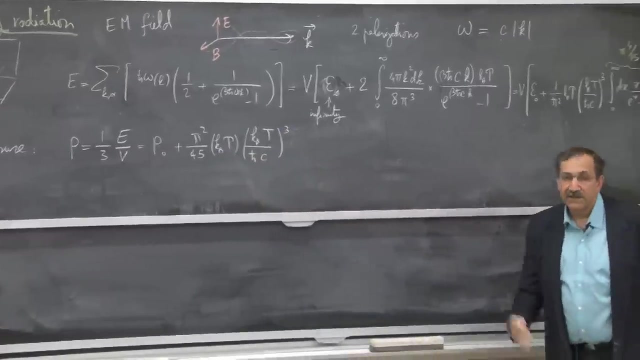 like some kind of a p0, and then something that is proportional to t, to the fourth. So I guess the corresponding coefficient here would be p squared divided by 45 kt over hb, Over h, bar c cubed, So there is a radiation pressure that 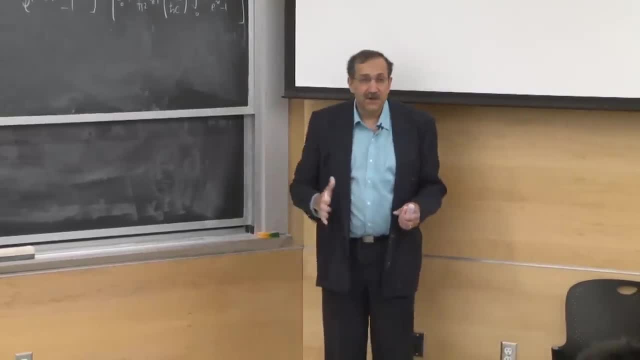 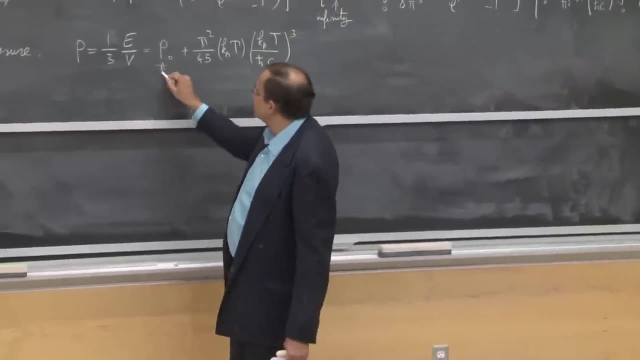 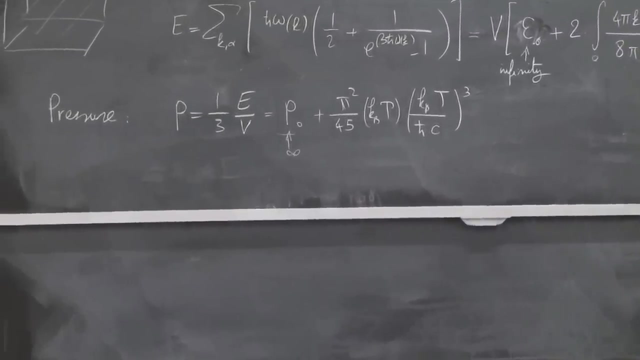 is proportional to temperature. The hotter you make this box, the more pressure it will get exerted from it. There is, of course, again this infinity that you may worry about, But here the problem is less serious, Because you would say that in reality, 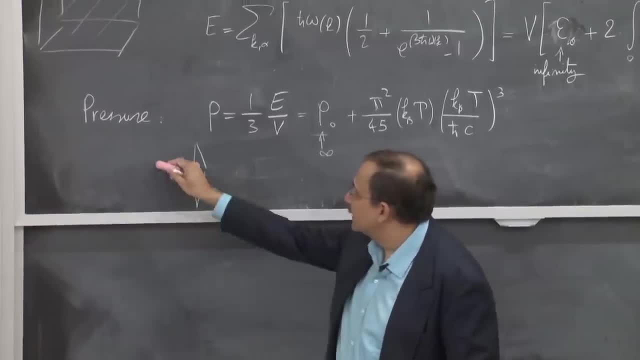 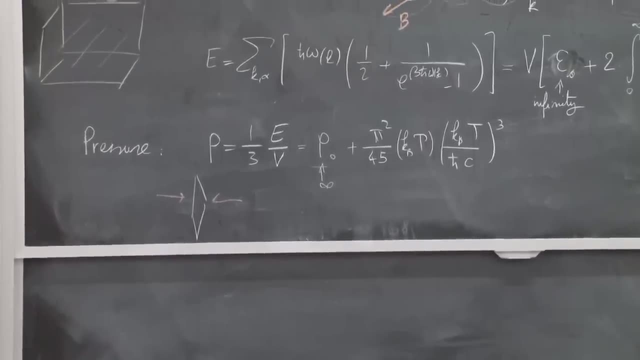 if I have the wall of the box, it is going to get pressure from both sides, And if there is an infinite pressure from both sides, they will cancel. So you don't have to worry about that. But it turns out that actually you 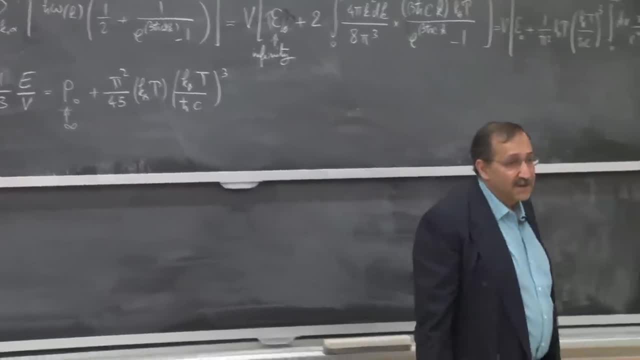 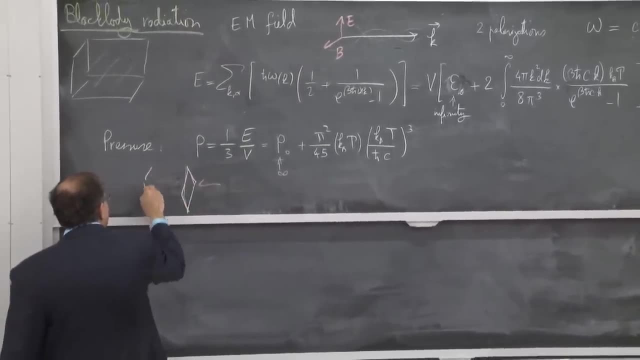 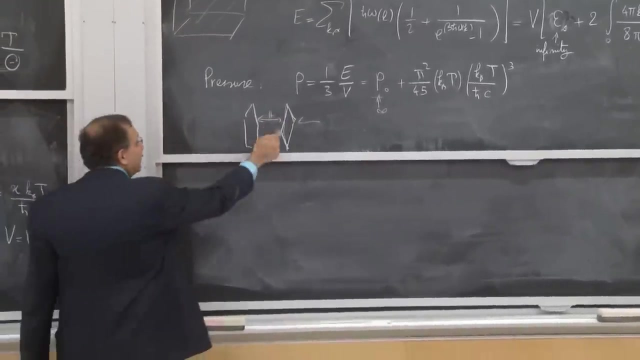 can measure the consequences of this pressure, And that occurs when, rather than having one plate, you have two plates. that are some small separation apart. Then the modes of radiation that you can fit in here because of the quantizations that you have. 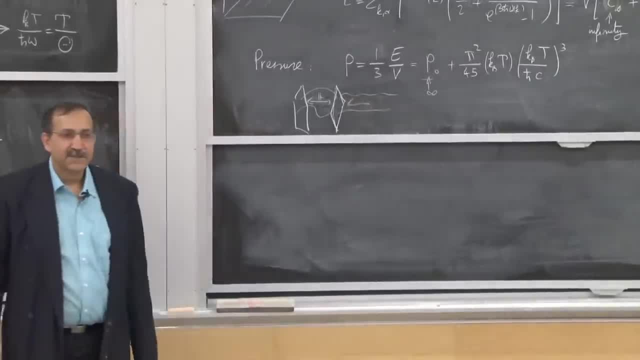 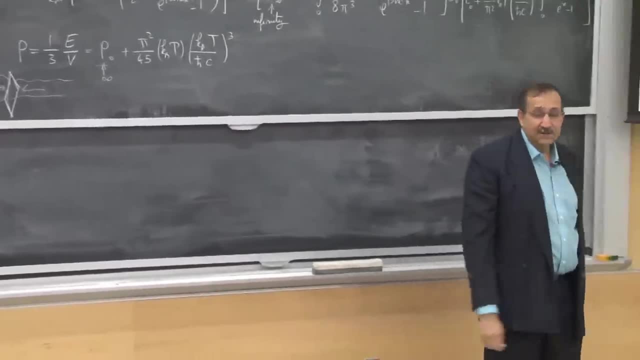 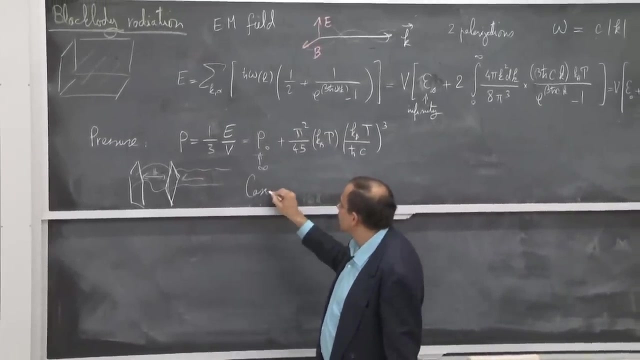 are different from the modes that you can have out here. So that difference, even from the zero point fluctuations- h bar, omega, over twos- will give you a pressure that pushes these plates together. That's called the Casimir force or Casimir pressure. 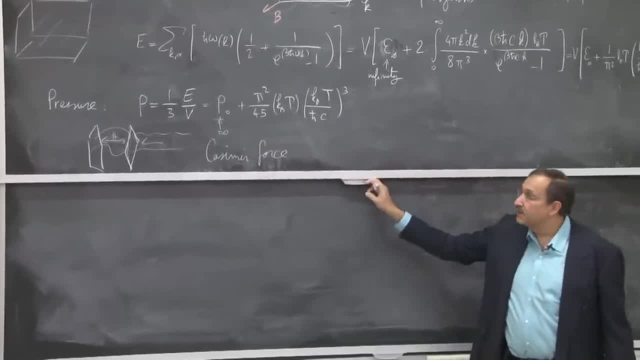 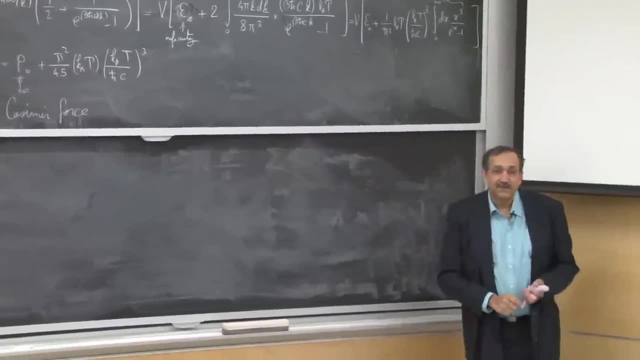 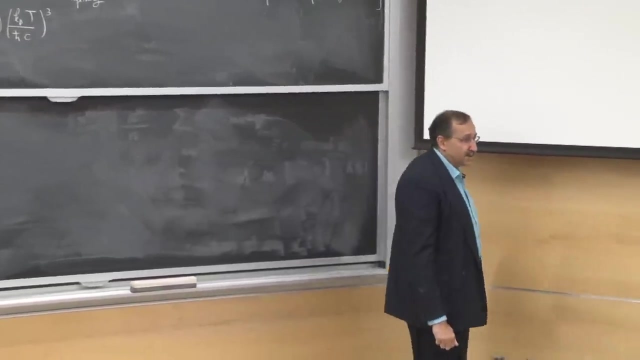 And that was predicted by Casimir in the 1950s and was measured experimentally roughly 10 years ago to high precision, matching the formula that we had. So sometimes these infinities have consequences that you have to worry about. But that's also to indicate that there 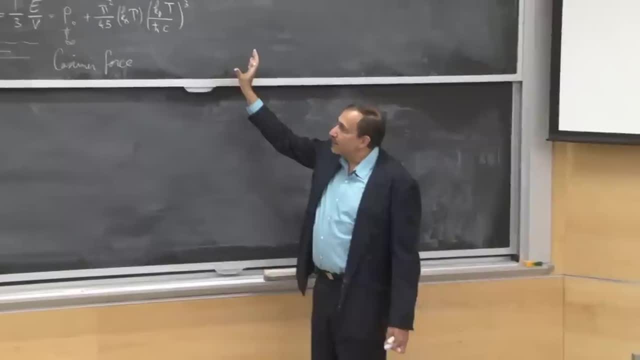 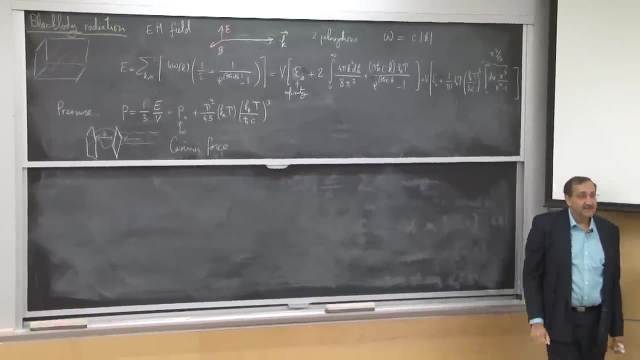 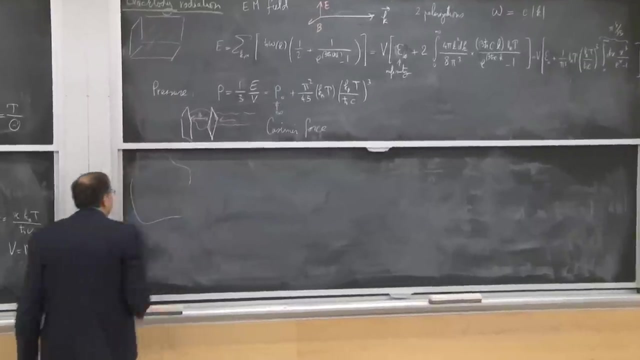 is kind of modern physics to this, But really it was the origin of quantum mechanics. because of the other aspect, It was the origin of the physics Which is: imagine that again you have this box. I draw it now as an irregular object box. 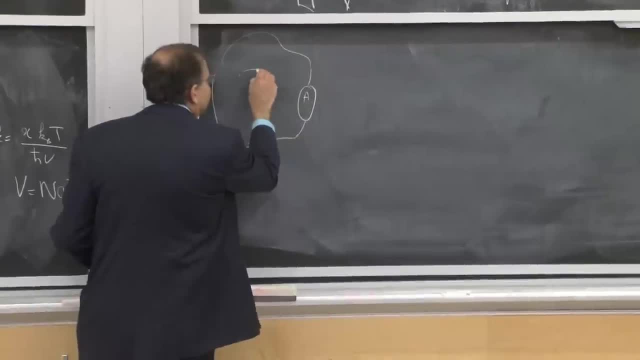 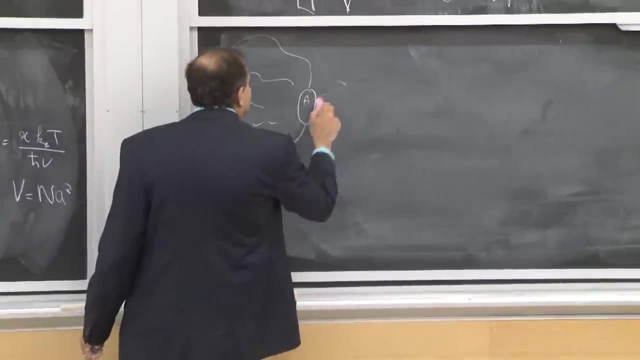 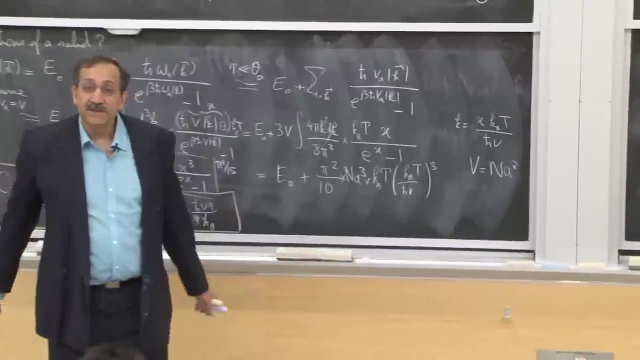 And I open a hole of size A inside the box And then the radiation that was inside at temperature T will start to go out. So you have a hot box. You open a hole in it and then the radiation starts to come out. 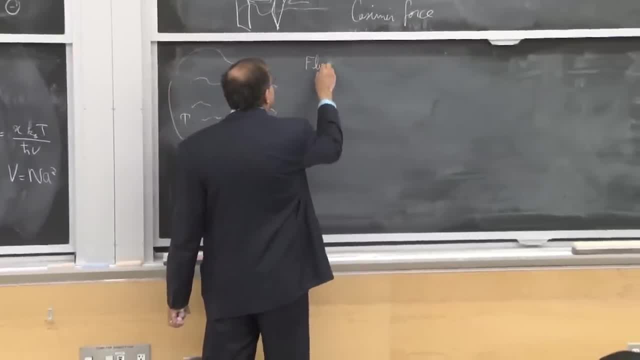 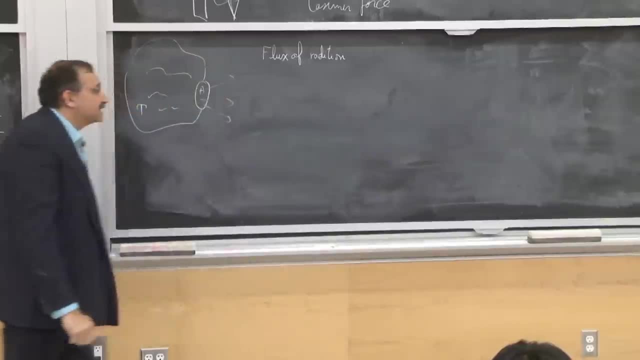 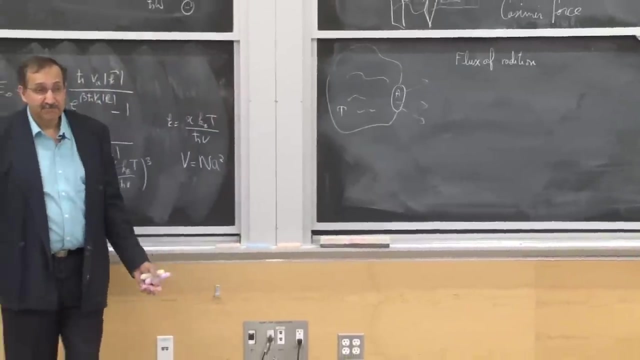 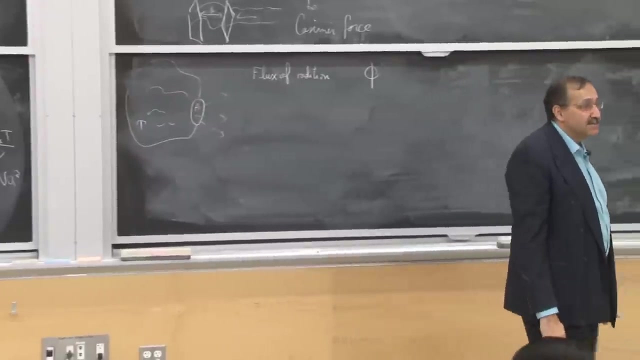 And so what you will have is a flux of radiation. Flux means that it is energy that is escaping per unit area and per unit time, So there is a flux which is per area per time. It turns out that that flux is, and this: 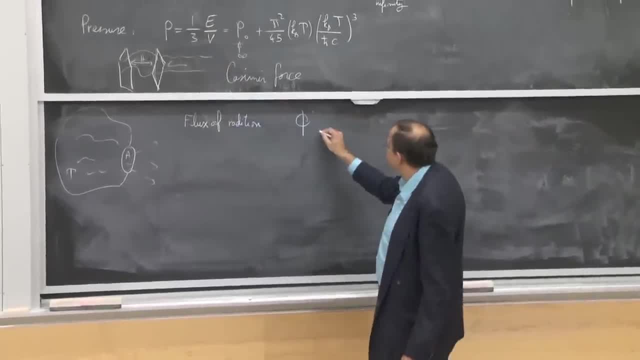 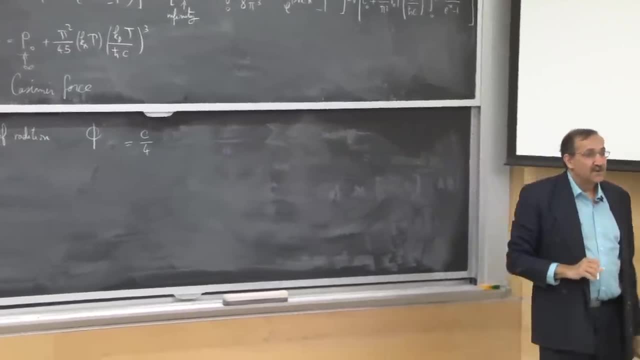 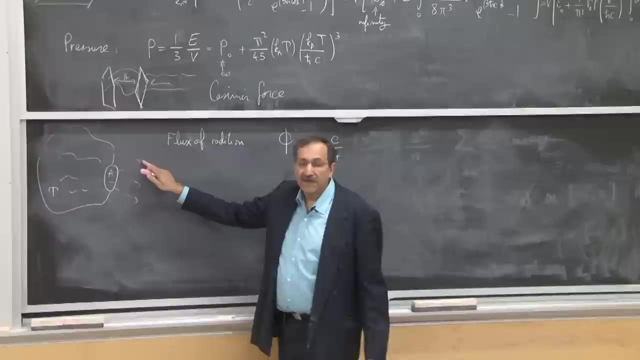 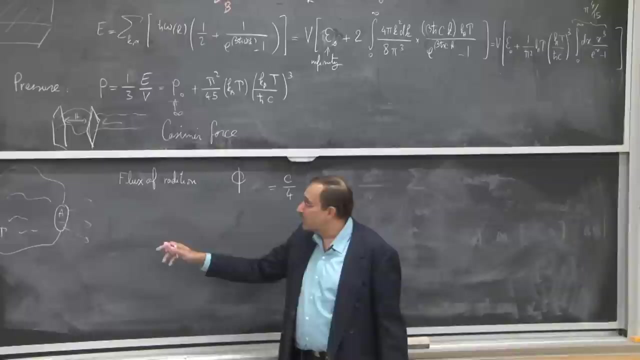 is another factor. this factor of 1 third that I mentioned is related to the energy density, with a factor of 1c over 4.. Essentially, clearly, the velocity with which energy is escaping is proportional to c, So you will get more radiation flux the larger c. 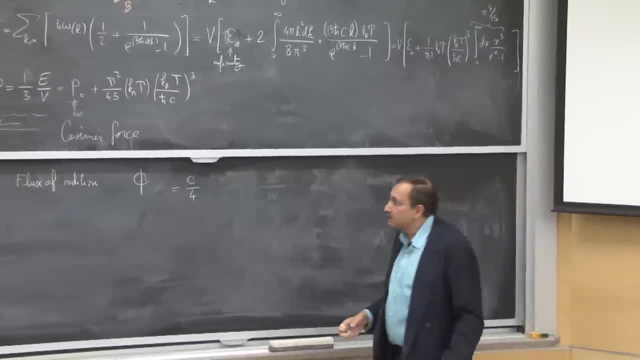 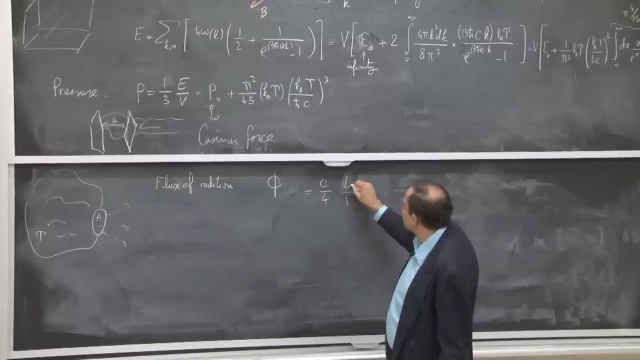 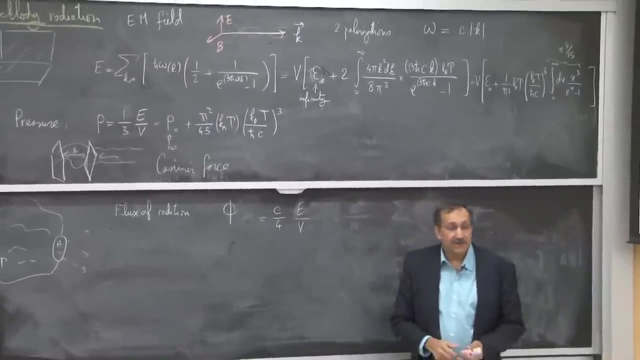 The answer has to be proportional to c, And it is. This is what is inside that is escaping. So it has to be proportional to the energy density that you have inside, some kind of energy per unit volume, And the factor of 1 quarter is one of these geometric factors. 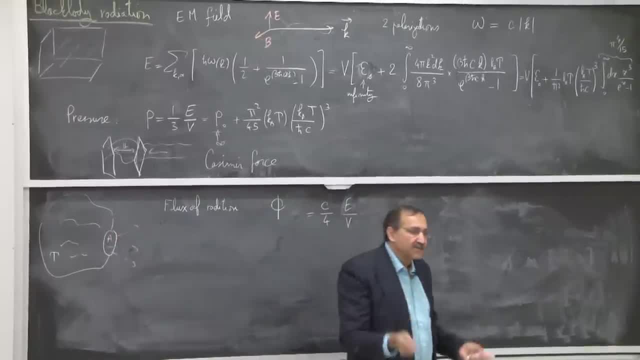 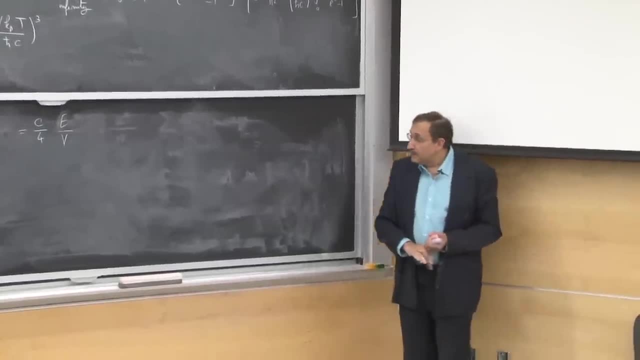 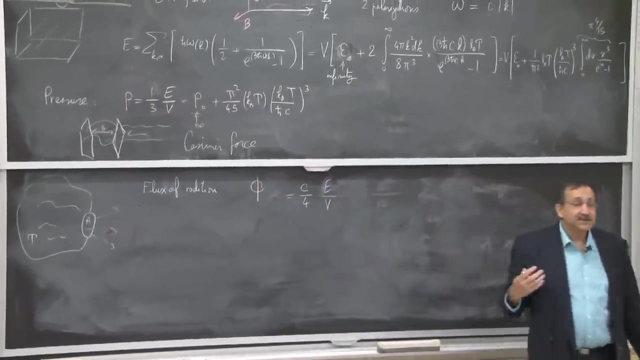 Essentially, there's two factors of cosine, of theta And you have to do an average of cosine squared theta And that will give you the additional 1 quarter. OK, But rather than looking so, this would tell you that there is an energy that is streaming out. 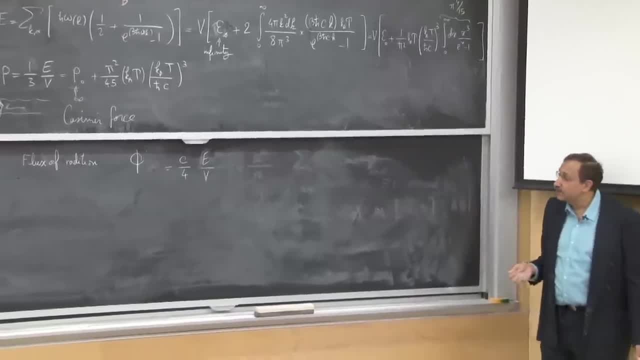 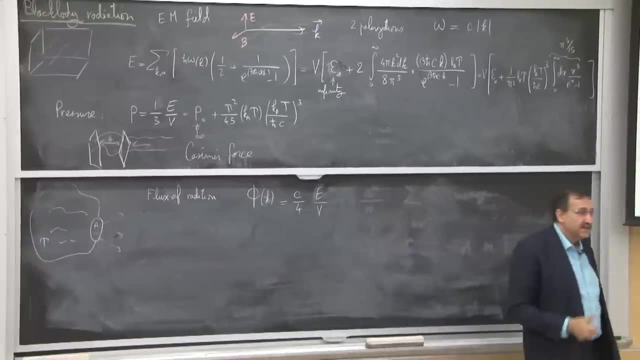 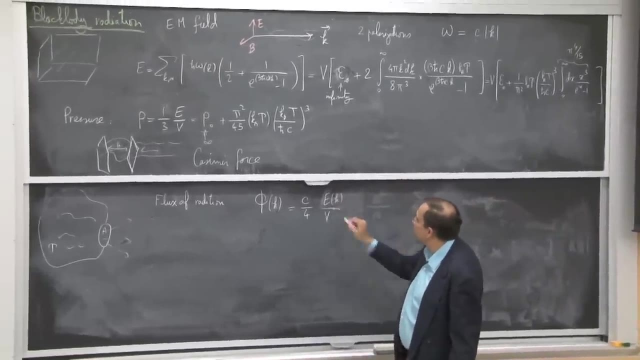 That is, the net value is proportional to t, to the fourth. But more interestingly, we can ask what is the flux per wavelength, And so for that I can just go back to the formula before I integrate it over k and ask: what is the energy density? 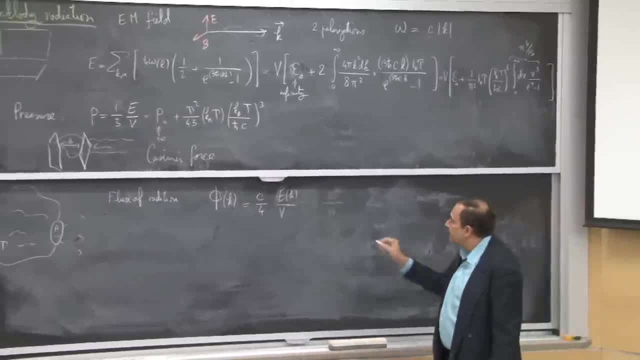 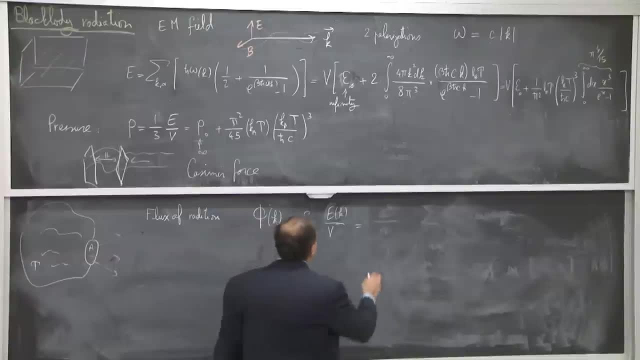 in each interval, OK, In each interval of k. And so what I have to do is to just go and look at the formula that I have prior to doing the integration over k, multiply it by a, c over 4. What do I have? 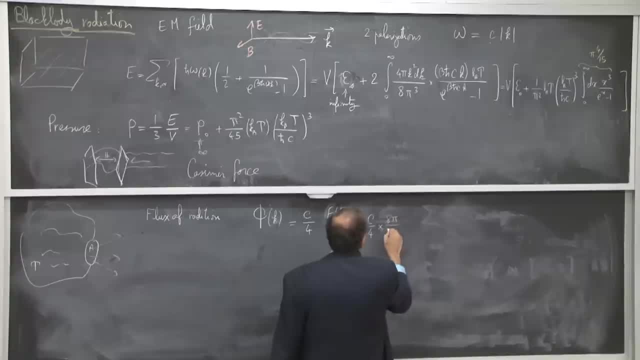 I have 8 pi divided by 8 pi cubed. I have a factor of k squared from the density of states. I have this factor of h bar ck Divided by e to the beta h bar ck minus 1.. OK, 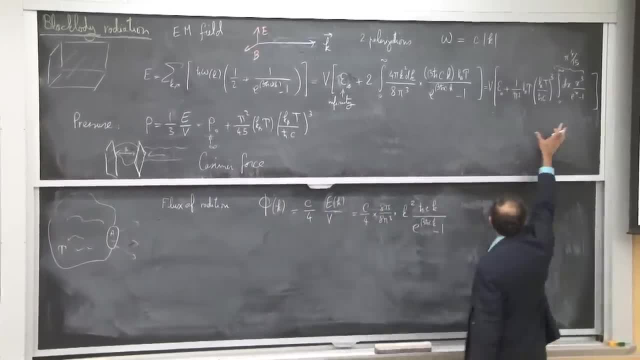 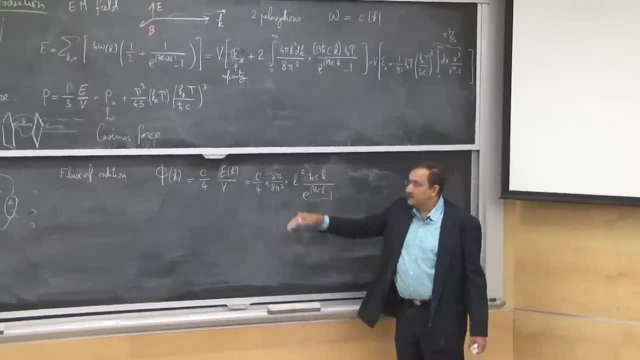 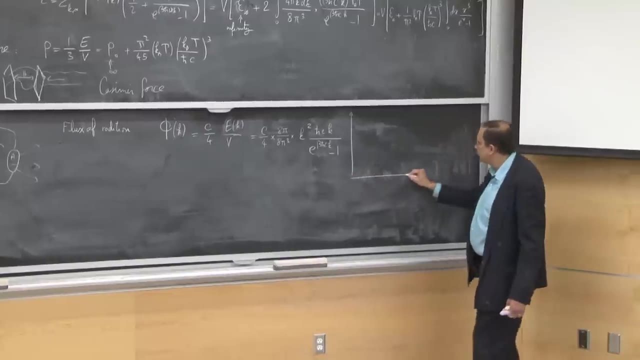 So we can. there is no analog of this because I'm not doing the integration over k, So we can simplify some of these factors out front. But really the story is, how does this quantity look As a function of wave number which? 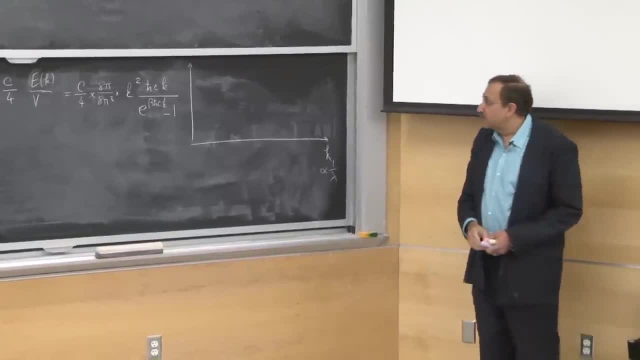 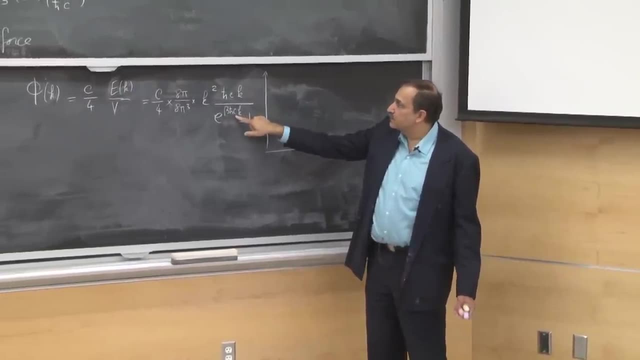 is the inverse of wavelength, if you like. And what we see is that when k goes to 0, essentially this factor e to the beta h bar ck. I have to expand To lowest order. I will get beta h bar ck. 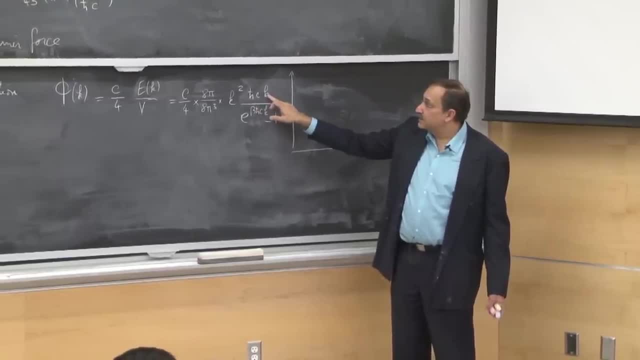 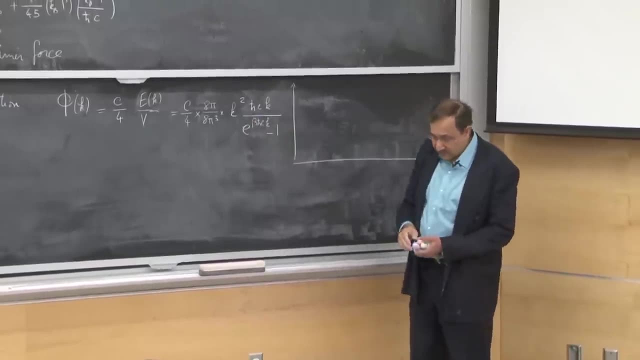 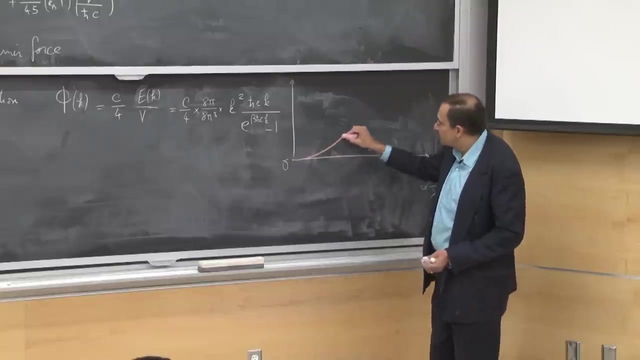 because the 1 disappears, h bar ck is canceled. so the answer is going to be proportional to inverse beta. It's going to be proportional to kt And k squared. So essentially the low k behavior part of this is proportional to k squared, c, of course, and kt. 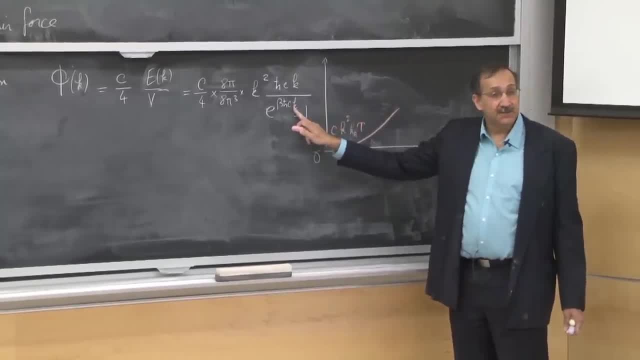 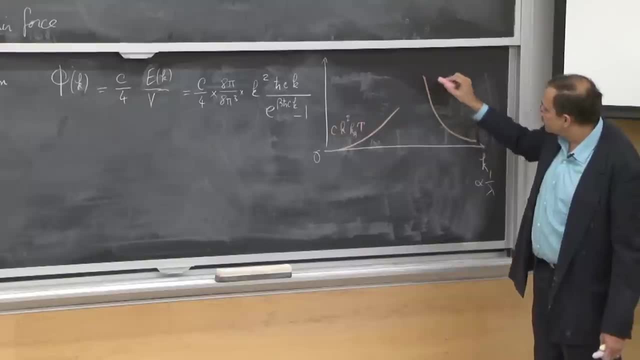 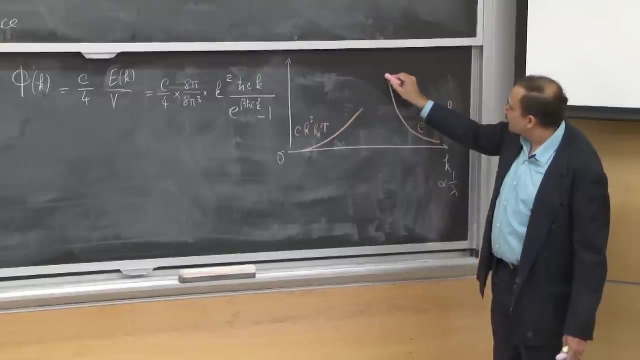 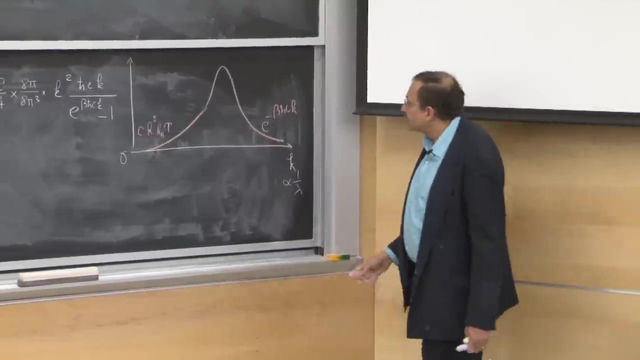 However, when I go to the high k numbers, the exponential will kill things off. So the large k part of this- OK, It is going to be exponentially small And actually the curve will look something like this: therefore, It will have a maximum around the k, which presumably 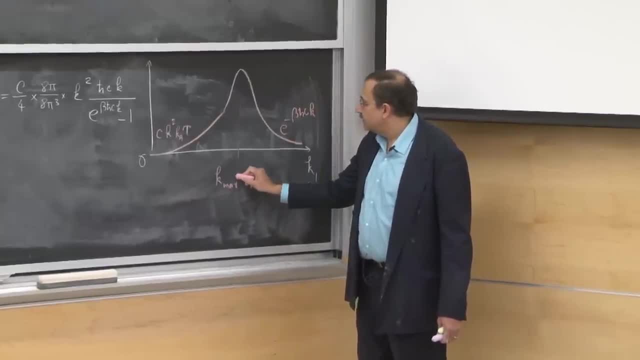 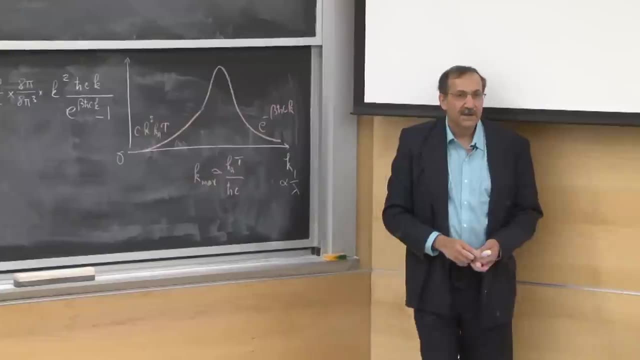 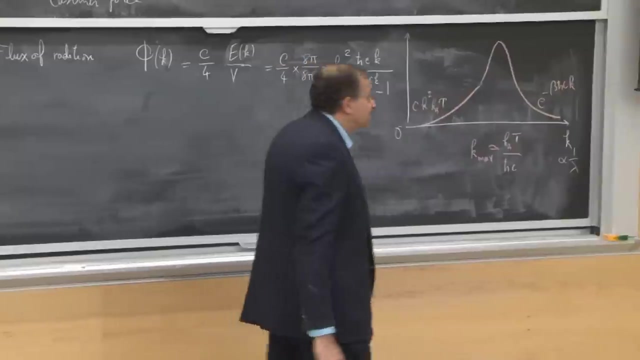 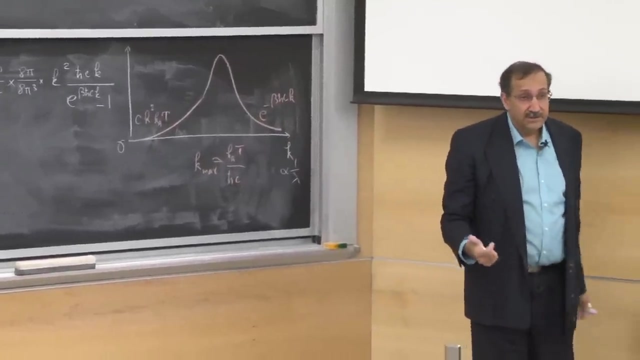 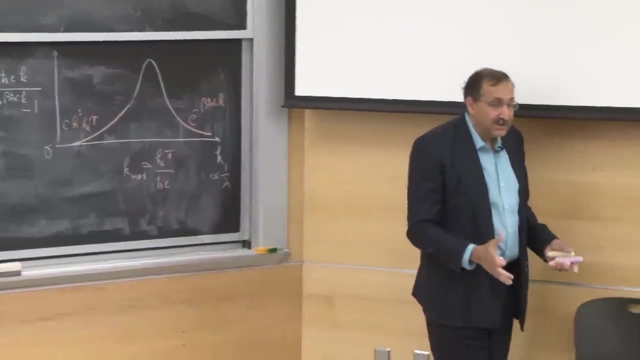 is of the order of kt over h bar c. So basically the hotter you have, this will move to the right, The wavelengths will become shorter And essentially that's the origin of the fact that can you heat some kind of material? 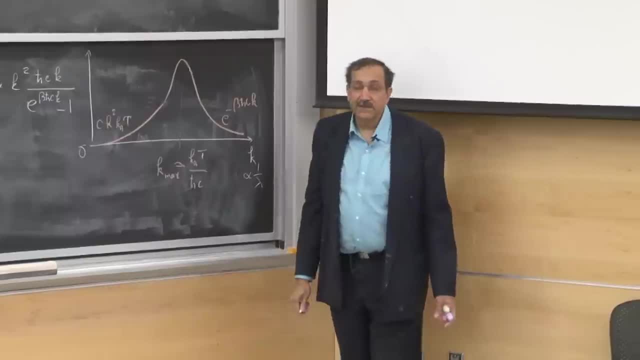 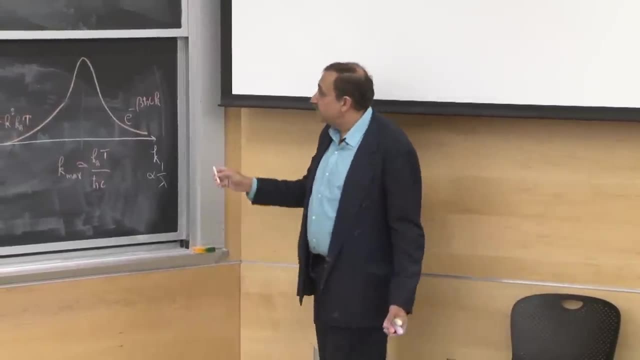 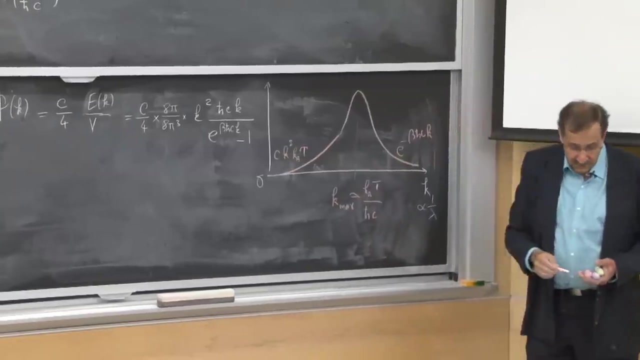 it will start to emit radiation and the radiation will be peaked at some frequency. that is really short, OK. OK, That is related to its temperature. Now, if we didn't have this quantization effect, if h bar went to 0, then what would happen? 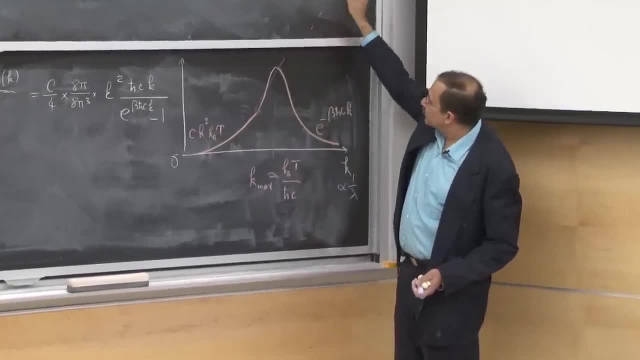 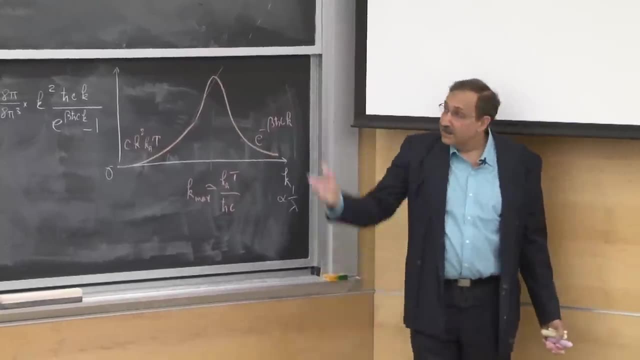 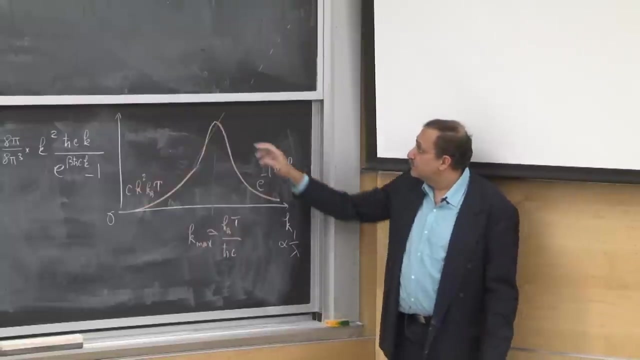 is that this k squared kt would continue forever. OK, Essentially you would have in each one of these modes of radiation, classically you would put a kt of energy And since you could have arbitrarily short wave waves, You would have infinite energy at shorter and shorter. 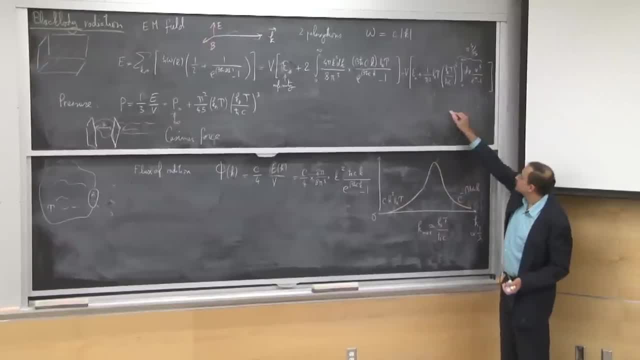 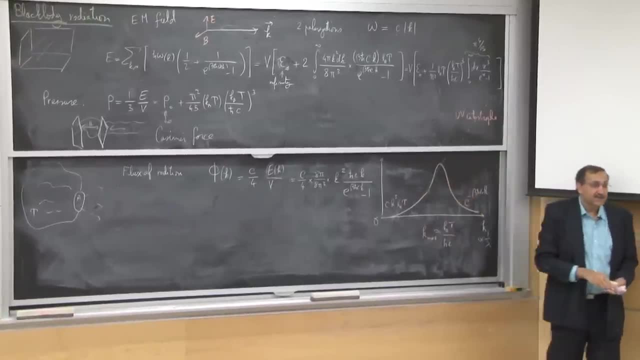 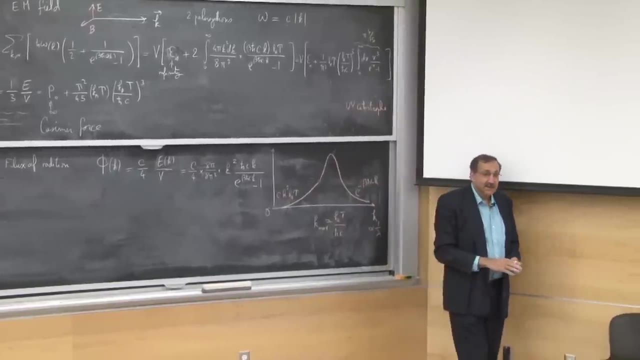 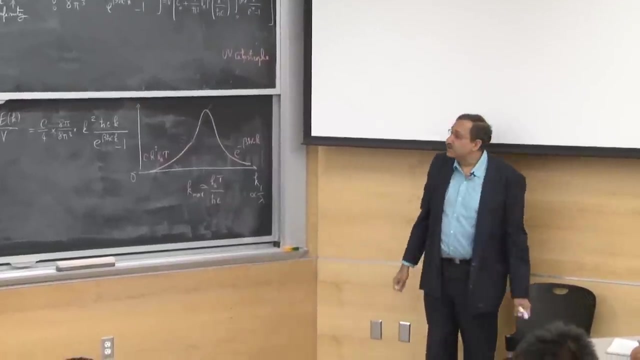 wavelengths And you would have this ultraviolet catastrophe. Of course, the shape of this curve was experimentally known towards the end of the 19th century, And so that was the basis of thinking about it and fitting an exponential to the end and eventually deducing that this quantization of the 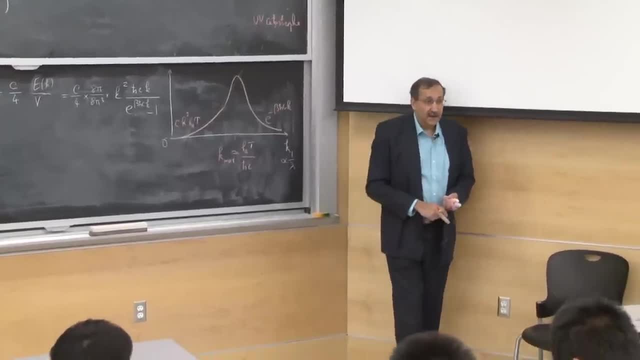 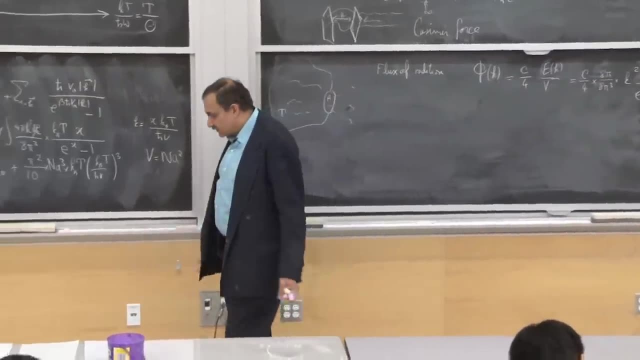 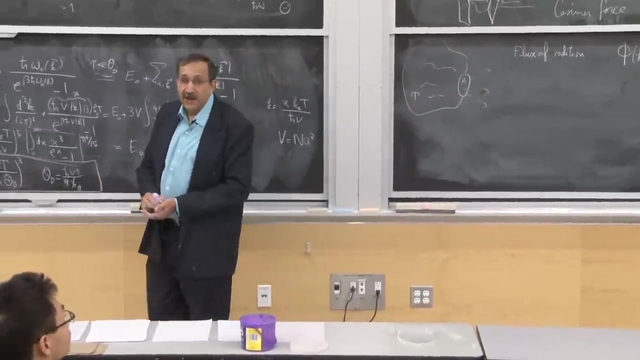 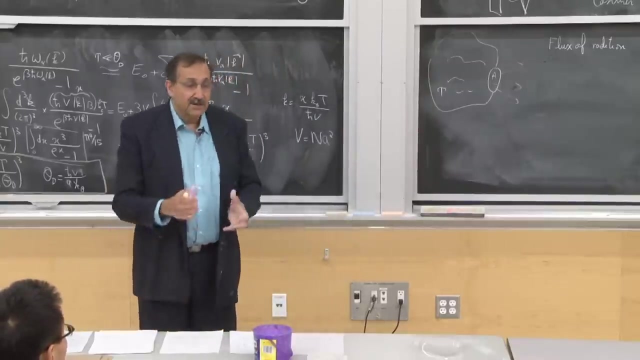 oscillators would potentially give you a reason for this to happen. Now, the way that I have described it. I kind of focused on having a cavity and opening the cavity and having the energy go out. Of course, the experiments for black body are not done on cavities. 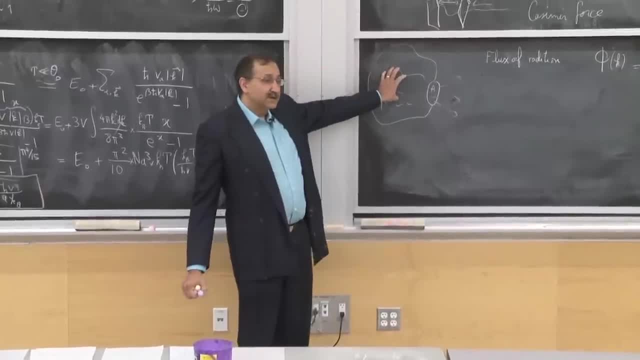 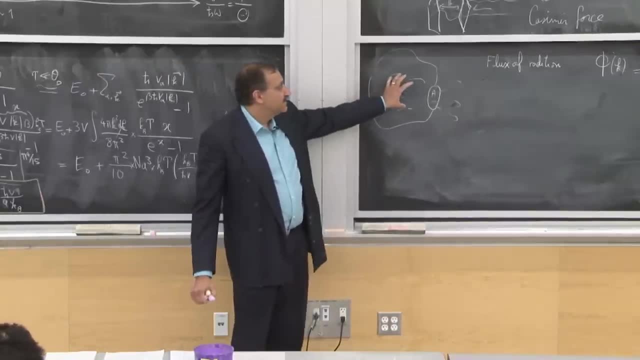 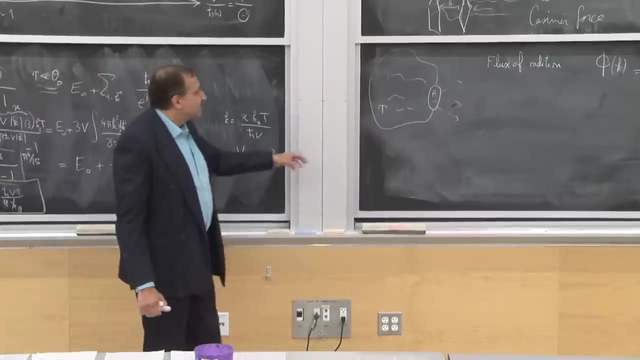 They are done on some piece of metal or some other thing that you heat up And then you can look at the spectrum of the radiation, And so, again, there is some universality in this, But it is not so sensitive to the properties of the material, although there are. 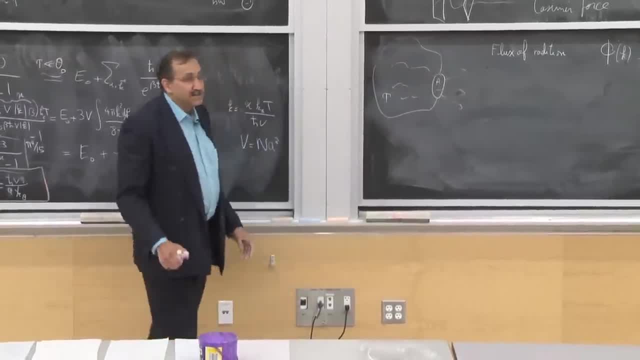 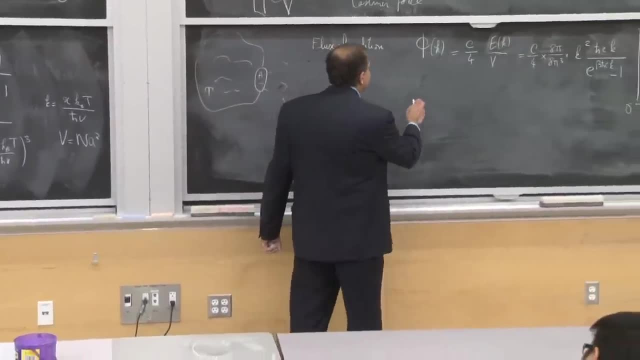 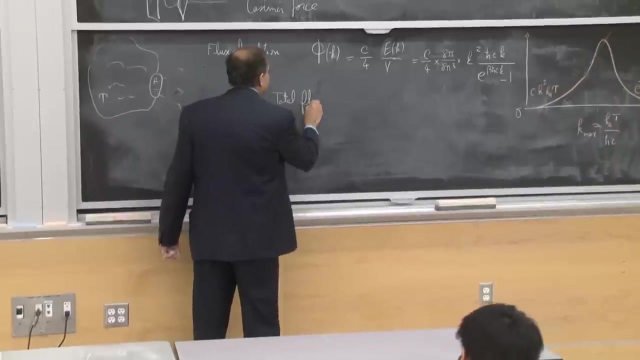 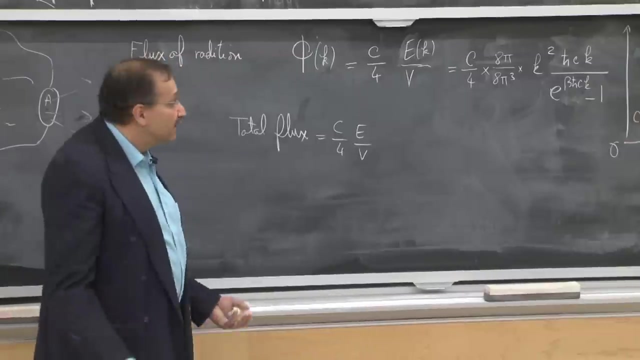 some emissivity and other factors that multiply the final result. So the final result in fact would say that if I were to integrate over frequencies the total radiation frocks, Which would be C over 4 times the energy density total, 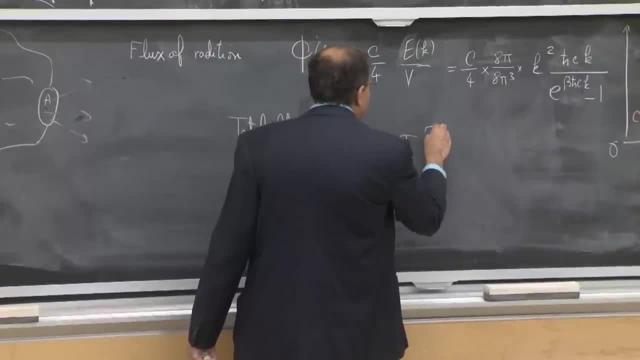 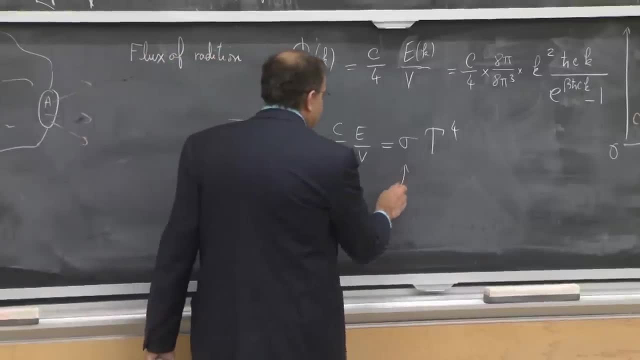 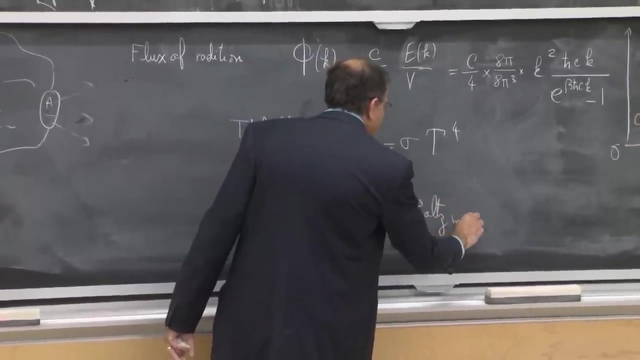 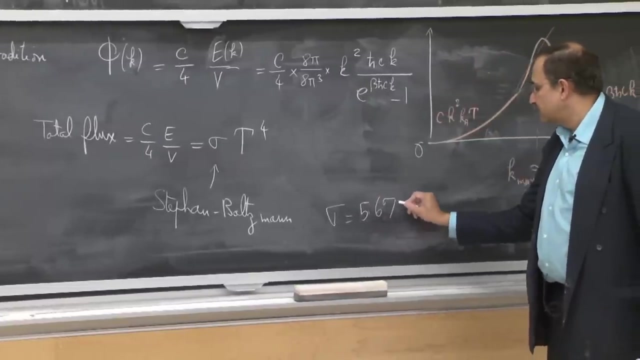 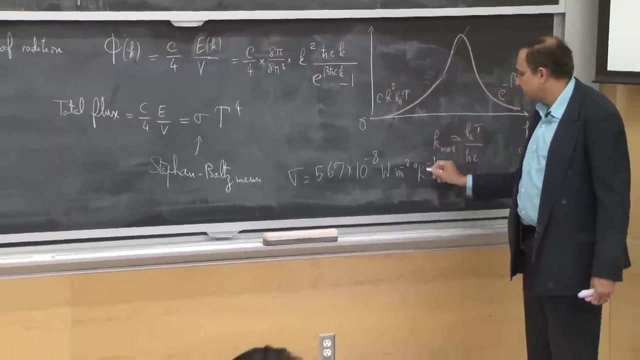 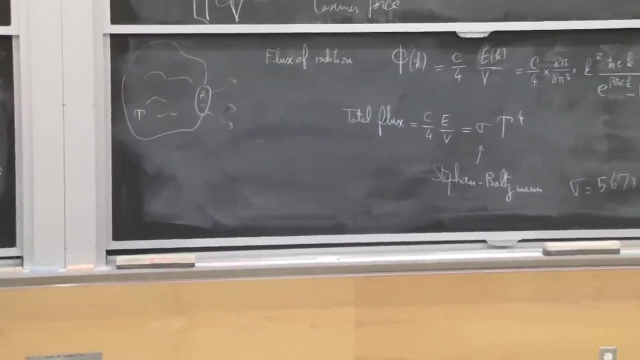 is going to be proportional to temperature, to the fourth power, And this constant in front is the Stefan-Boltzmann which has some particular value. This OK, If you can look up units of watts per area, per degrees Kelvin, So this perspective is rather macroscopic. 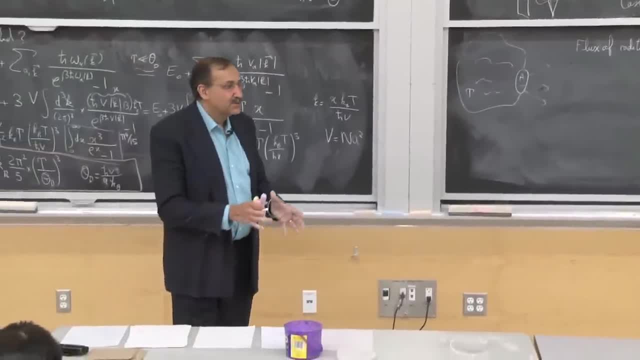 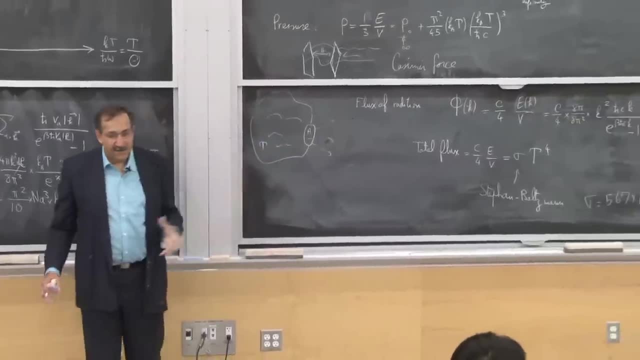 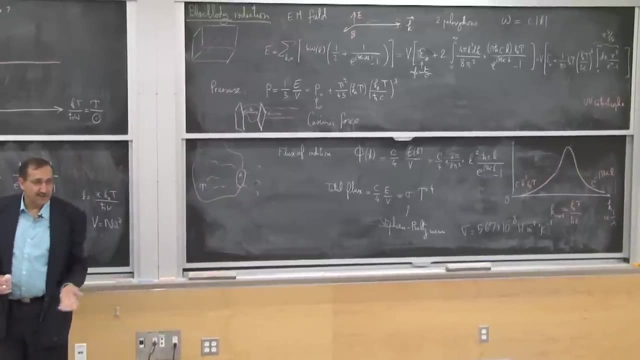 that the radiated energy is proportional to the surface area. If you make things that are Kind of small And the wavelengths that you are looking at over here become comparable to the size of the object, These formulae break down And again to sort of go forward about 150 years or so. 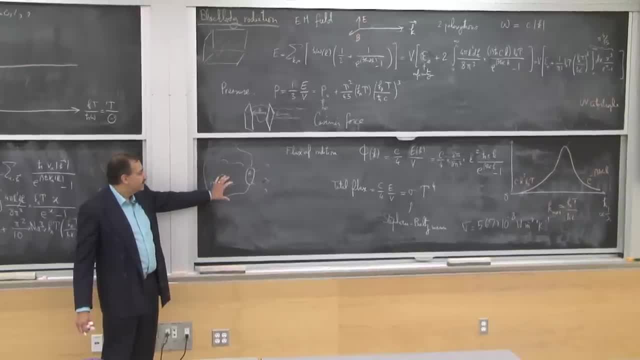 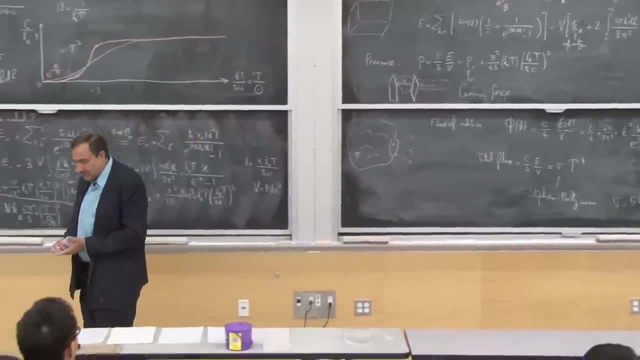 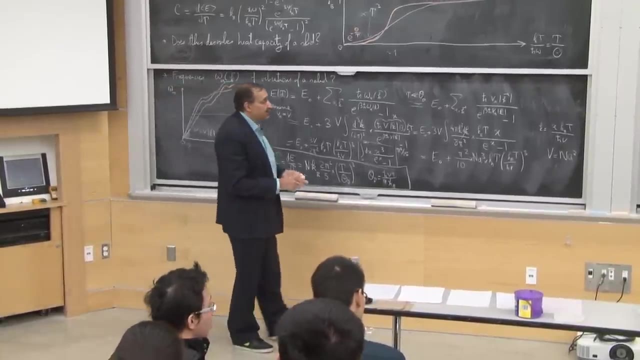 there is ongoing research, I guess more 200 years ongoing research on no 100 and something ongoing research on how these classical laws of radiation work. OK, OK, The laws of radiation are modified when you are dealing with objects that. 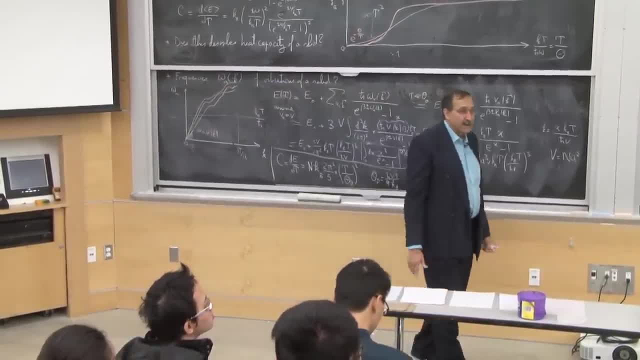 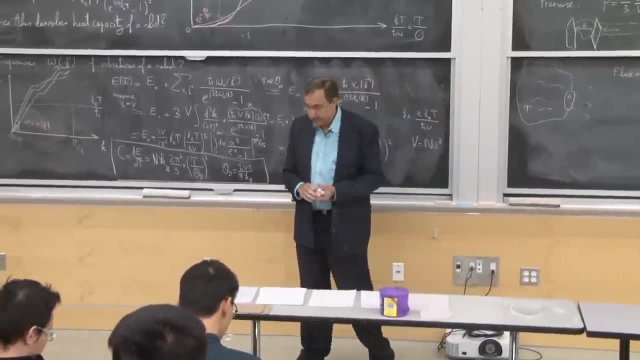 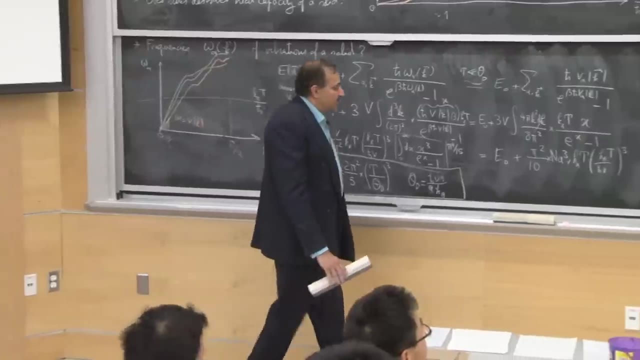 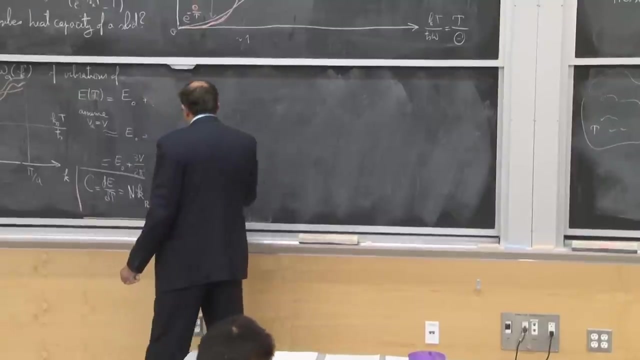 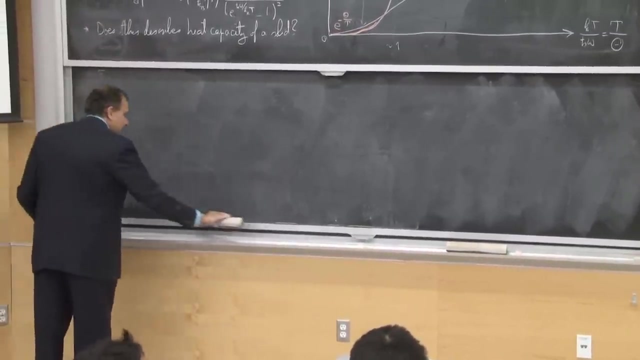 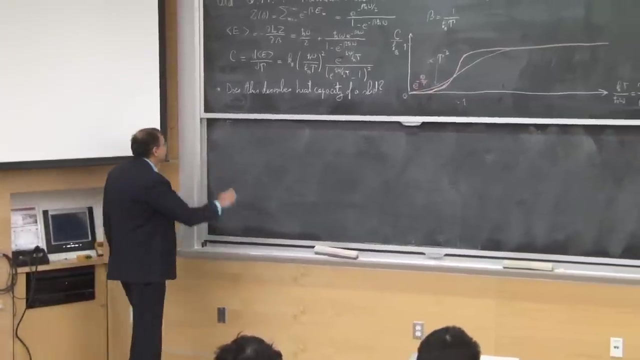 are small compared to the wavelengths that are emitted, et cetera. OK, Any questions? So the next part of the story is: why did you do all of this? I mean, it works, But what is the justification In that? I said there was the old quantum mechanics? 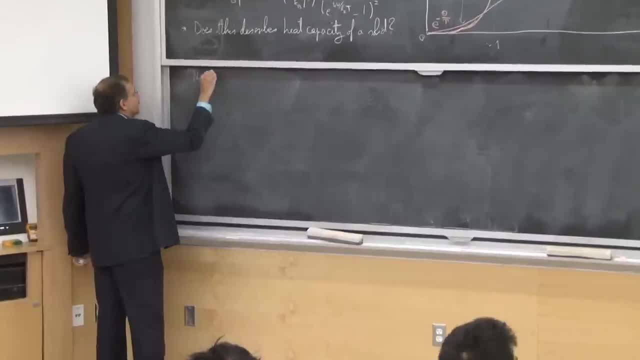 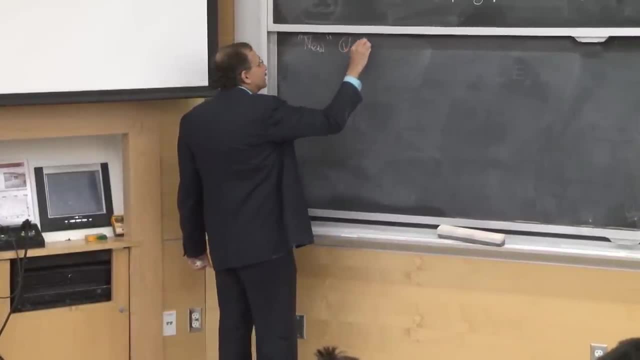 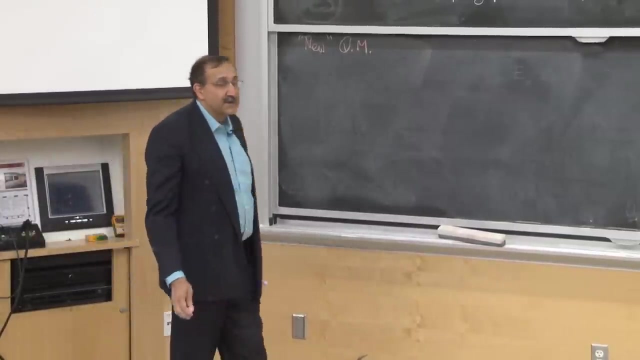 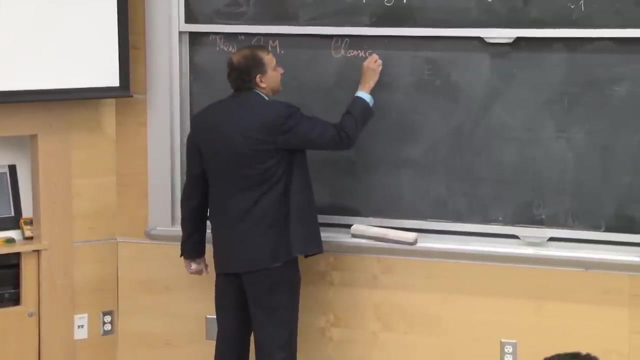 But really we want to have statements about quantum systems that are not harmonic oscillators And we want to be able to understand actually what the underlying basis is, In the same way that we understand how we were doing things for classical statistical mechanics, And so really we want to look at how 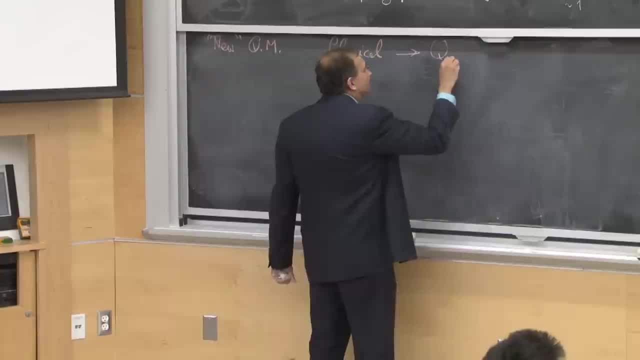 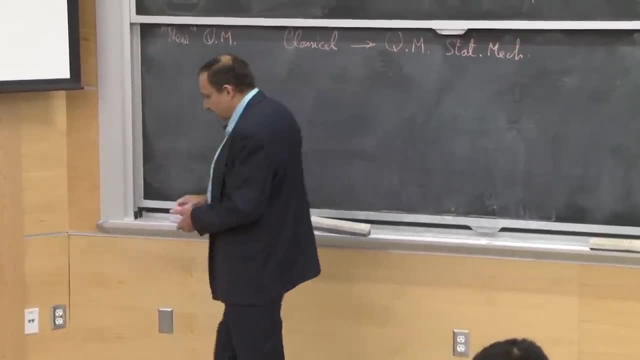 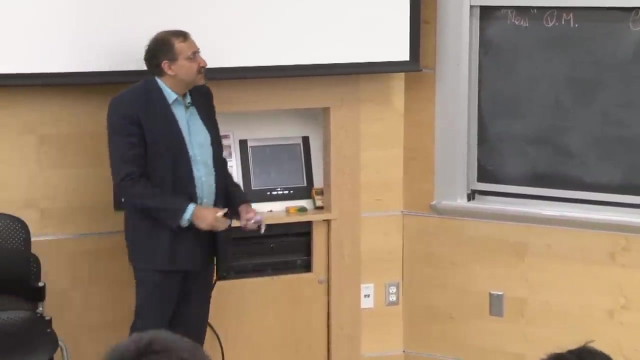 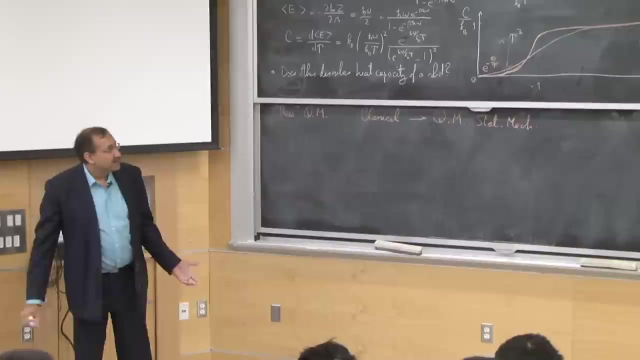 to make the transition from classical to quantum statistical mechanics. So for that let's go and remind us actually. so basically, the question is something. The question is something like this: What does this partition function mean? I'm calculating things as if I have these states that 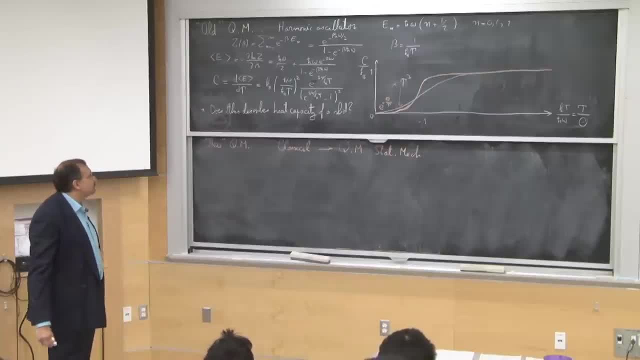 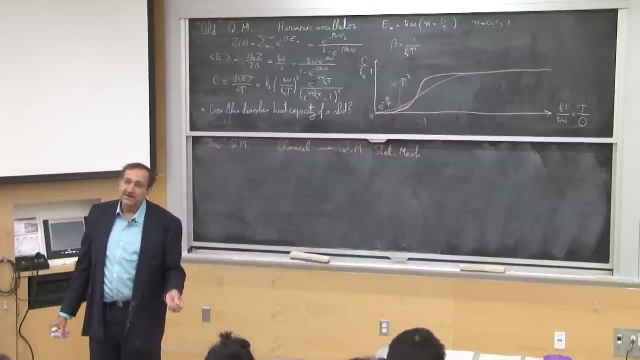 are the energy levels And the probabilities are e to the minus beta epsilon n. What does that mean? I mean classically we knew the Boltzmann weights had something to do with the probability of finding a particle with a particular position and momentum. 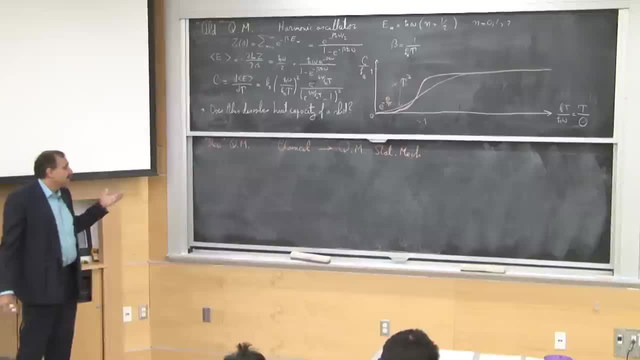 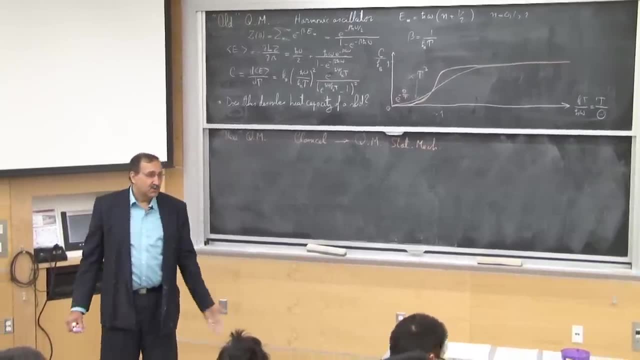 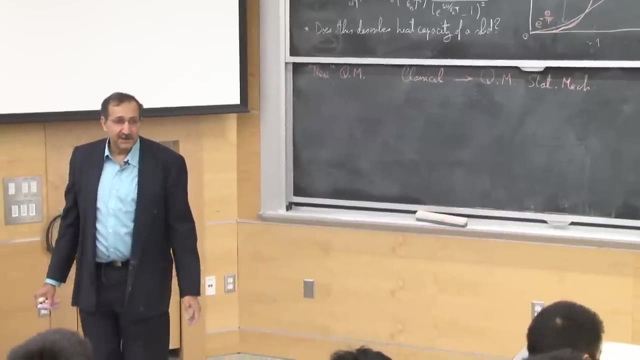 So what is the analogous thing here? And you know that in new quantum mechanics the interpretations of many things is probabilistic, And in statistical mechanics, even classically, we had a probabilistic interpretation. So presumably we want to build a probabilistic theory. 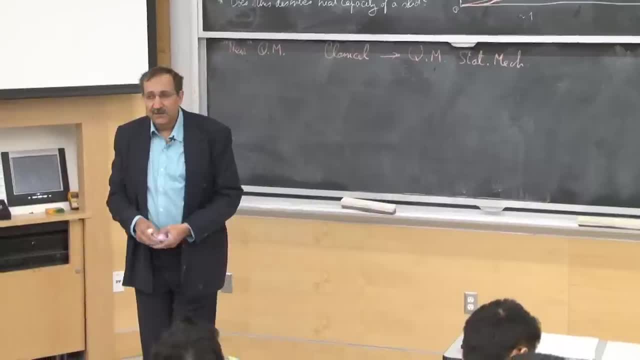 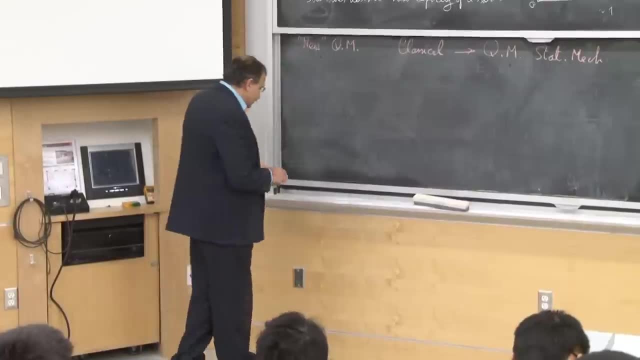 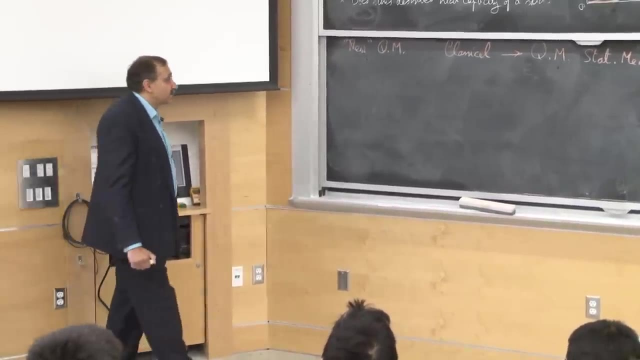 on top of another probabilistic theory. So how do we go about understanding precisely what is happening over here? So let's kind of remind ourselves of what we were doing in the original classical statistical mechanics and try to see how we can make the corresponding calculations when 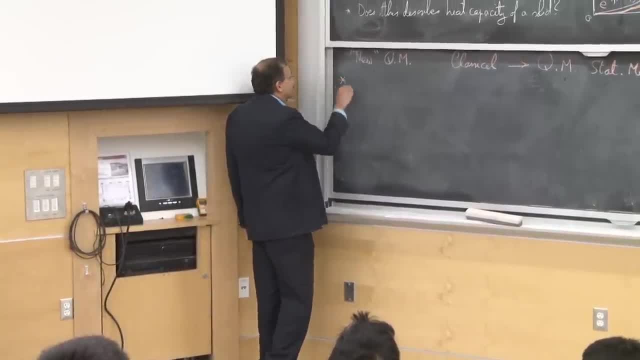 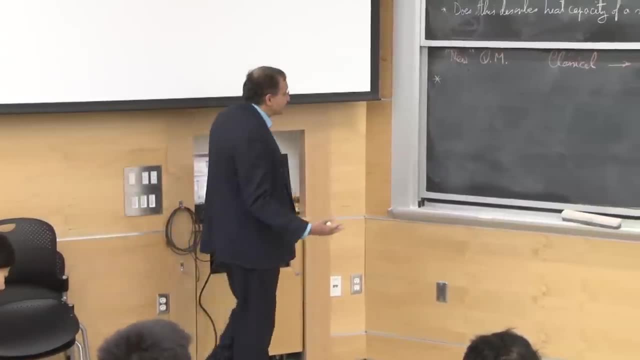 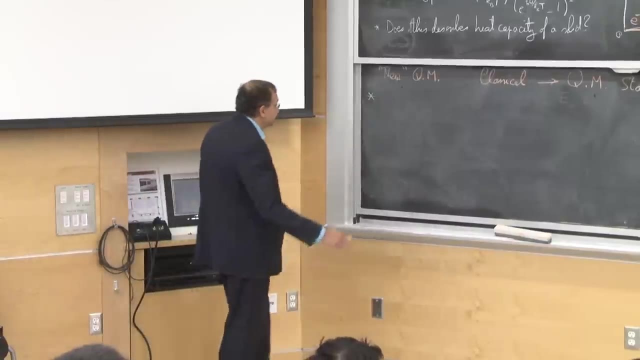 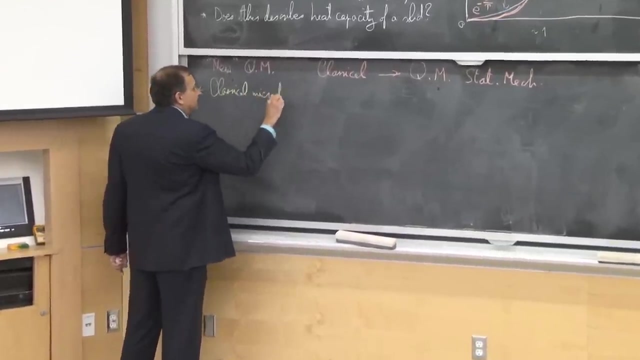 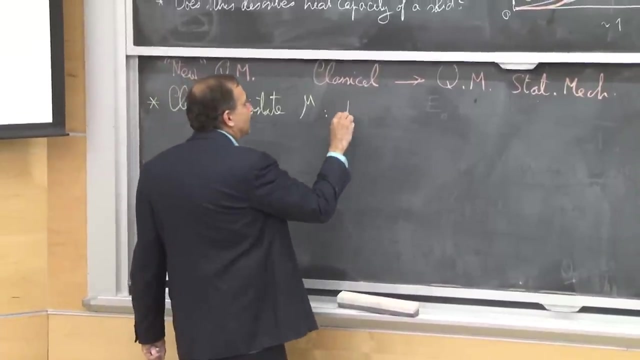 things are quantum mechanical. So essentially the probabilistic sense that we had in classical statistical mechanics was to assign probabilities, And the probability is for microstates, given that we had some knowledge of the macrostate. So the classical microstate mu was a point. 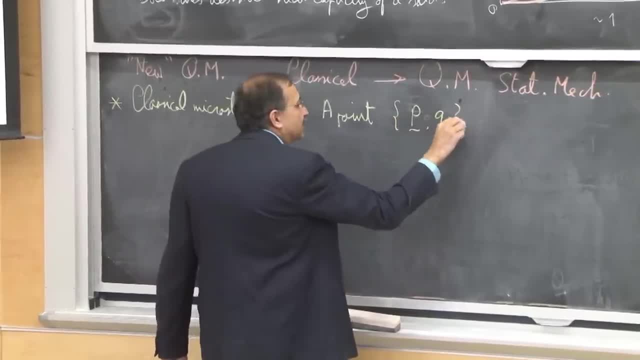 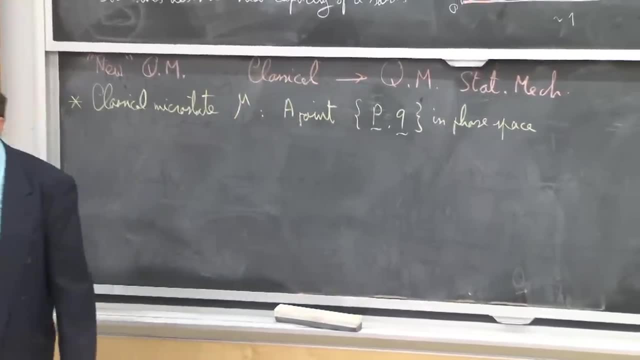 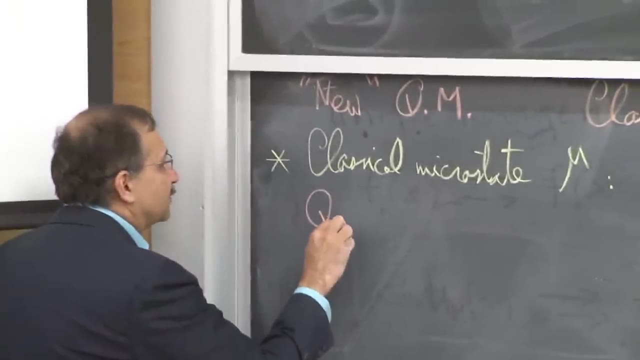 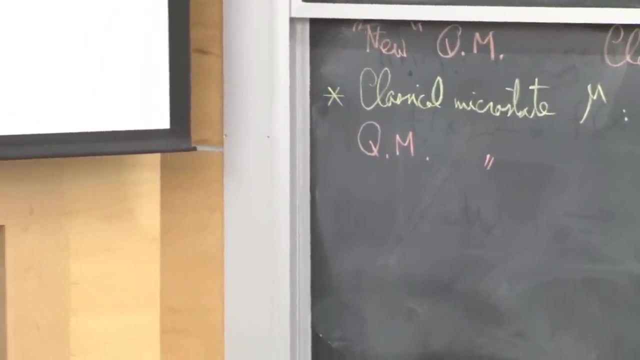 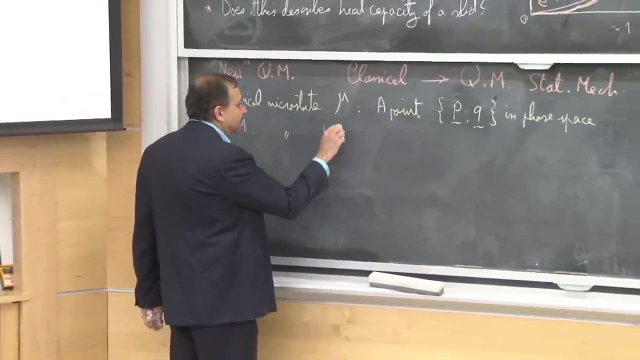 which was a collection of p's and q's in phase space. OK, So what is a quantum microstate? OK, So here I'm just going to jump several decades ahead and just write the answer, And I'm going to do it. 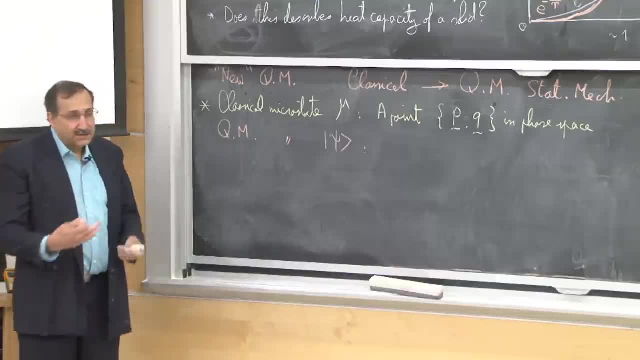 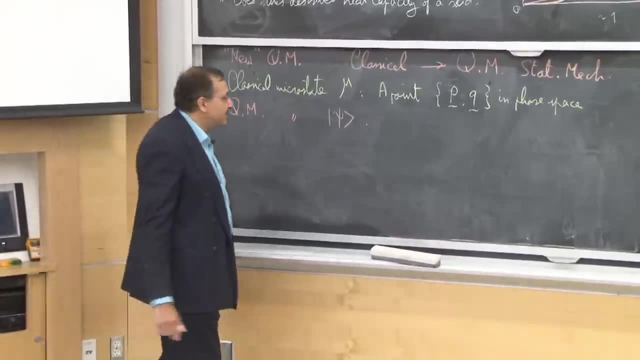 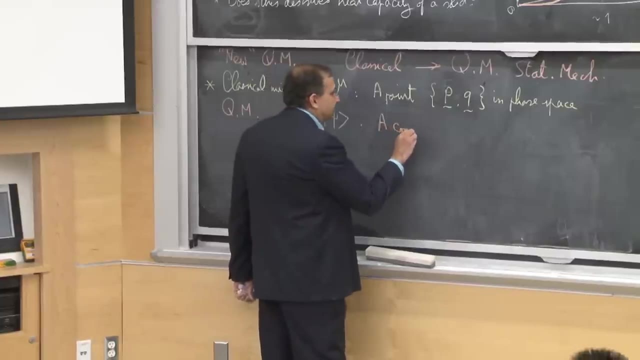 In somewhat of a more axiomatic way, because it's not up to me to introduce quantum mechanics. I assume that you know it already. Just the perspective that I'm going to take. So the quantum microstate is a complex unit vector in Hilbert space. 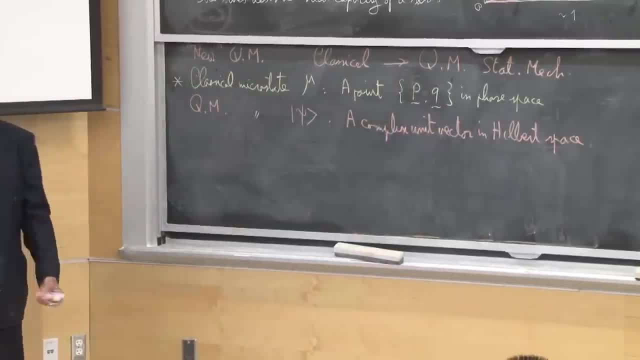 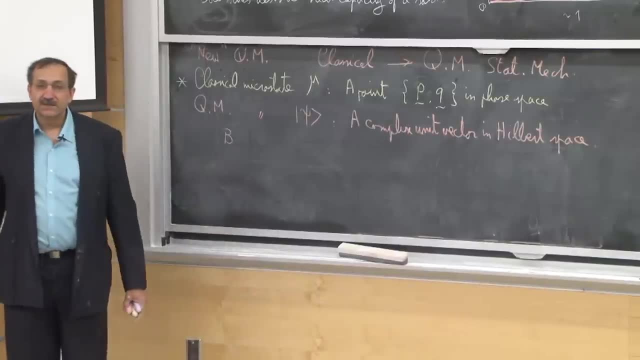 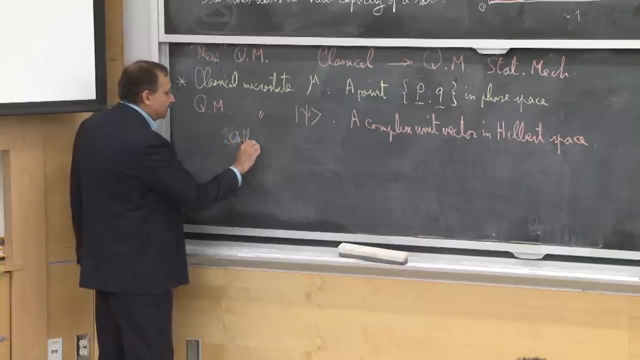 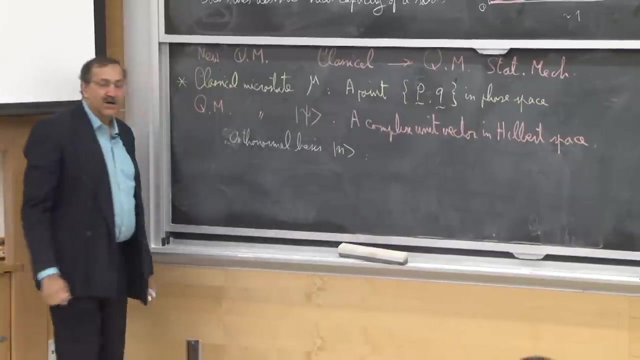 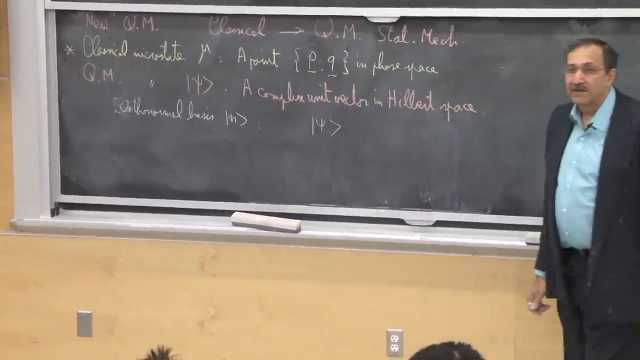 OK, So we can choose. for any vector space, we can choose a set of unit vectors that form an orthonormal basis- And I'm going to use this bra ket notation- And so our psi, The psi, which is a vector in this space, 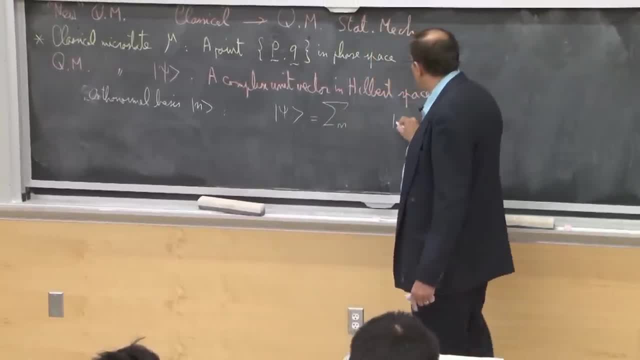 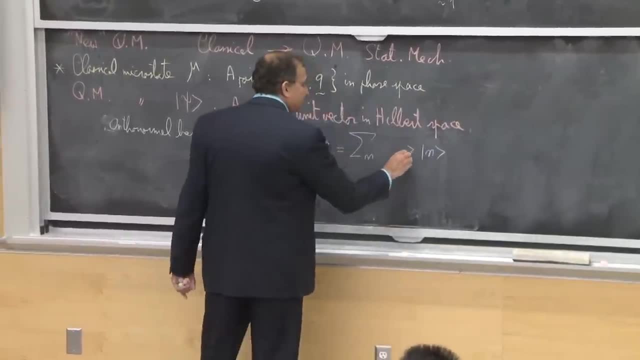 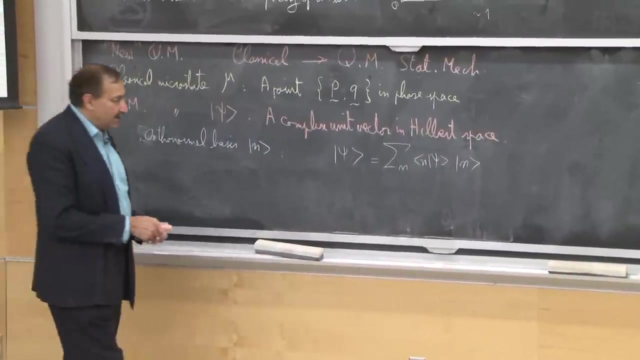 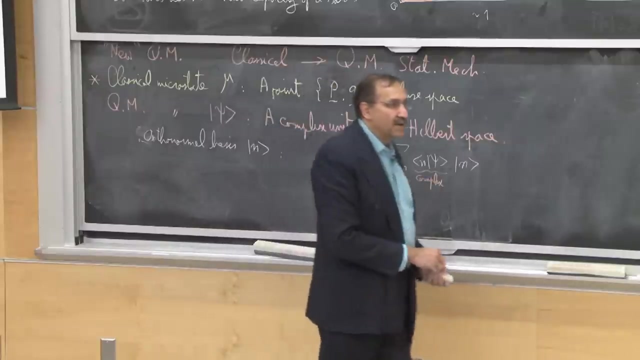 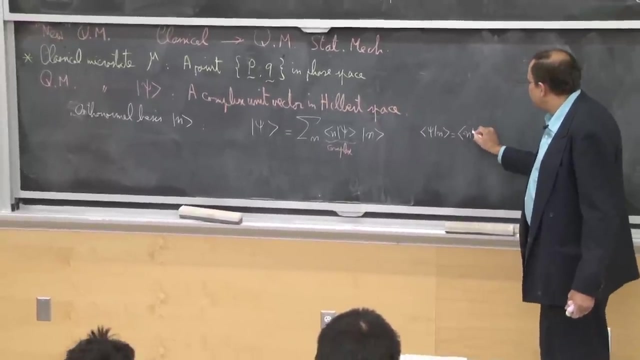 can be written in terms of its components by pointing to the different directions in this space, and components that I will indicate by this psi n, And these are complex And And I will use the notation that psi n is the complex conjugate of n psi. 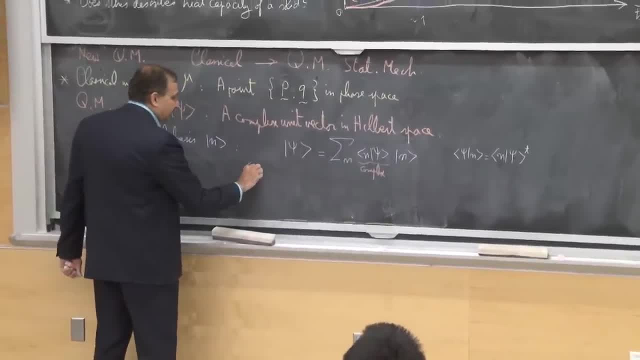 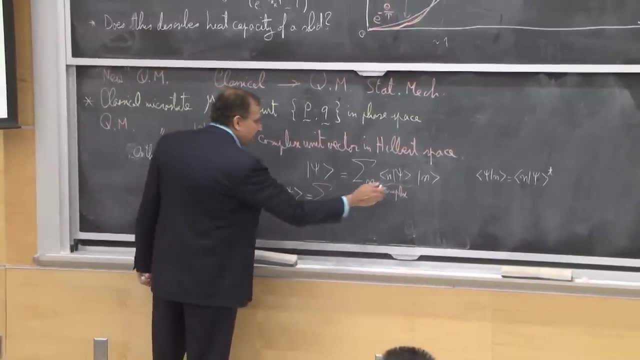 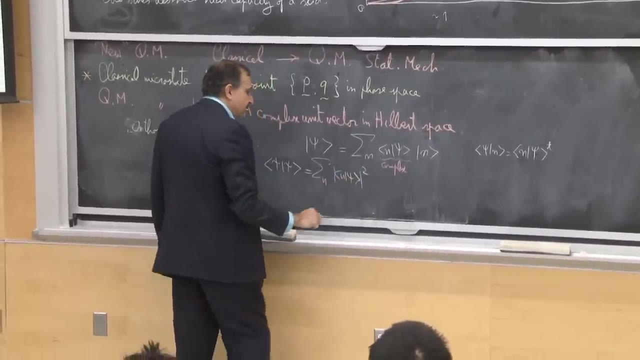 And the norm of this I'm going to indicate by psi. psi, which is obtained by summing over all n psi, psi n star, which is essentially the magnitude of n psi squared, And these are unit vectors. So all of these states are normalized. 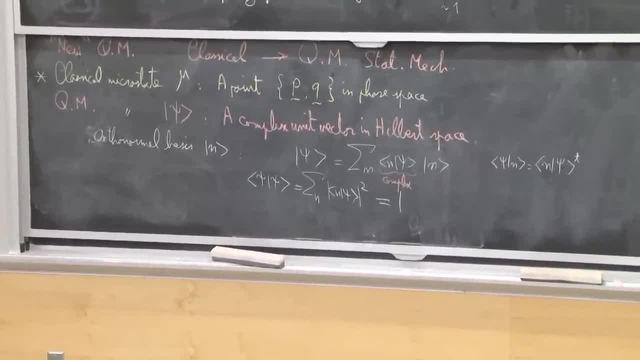 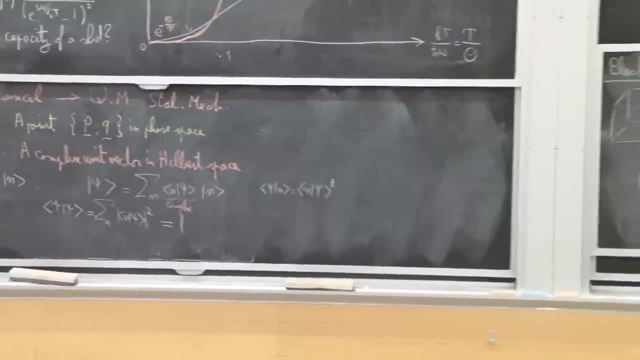 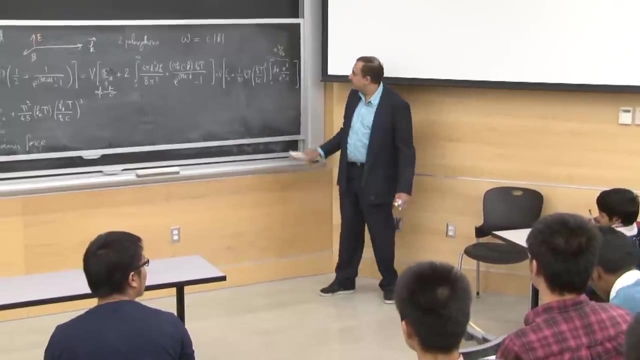 such that psi. psi is equal to 1.. Yes, You're not allowing particle numbers to vary, are you At this stage? no, Later on, when we do the grand canonical, we will change our Hilbert space, OK, OK. 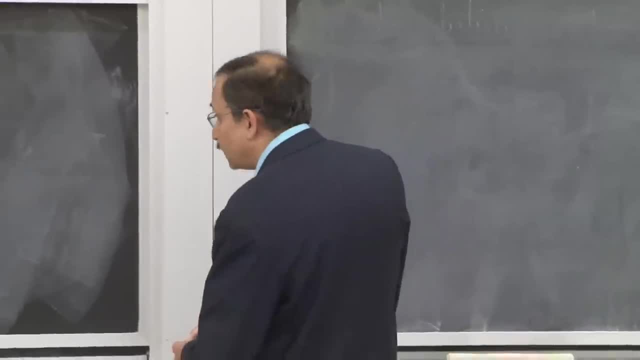 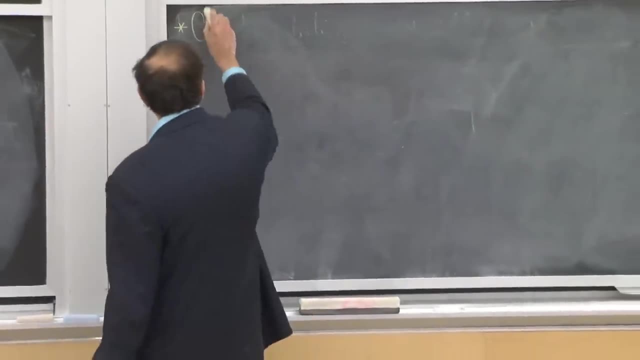 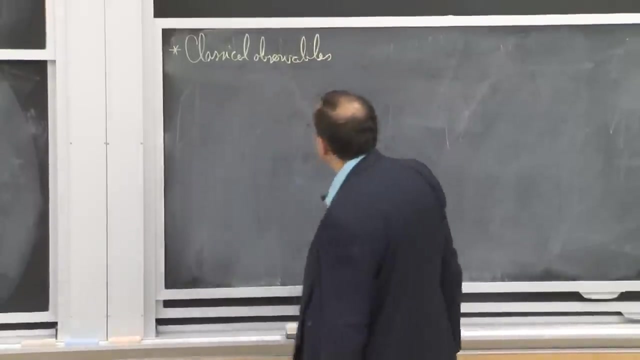 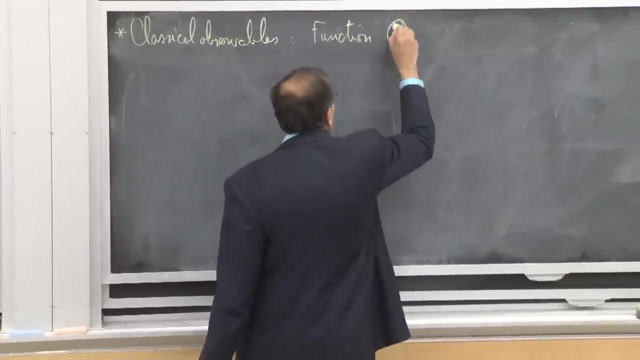 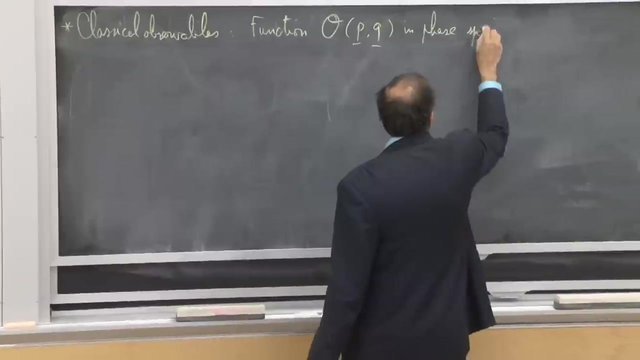 OK, So that's one concept. The other concept: classically, we measure things, So we have classical observables And these are functions, all of which depend on this p and q in phase space. So basically there's the phase space. 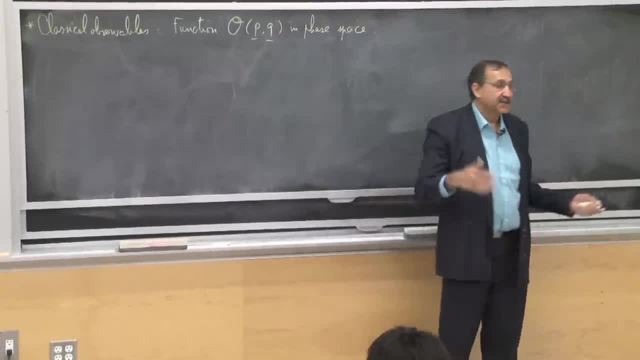 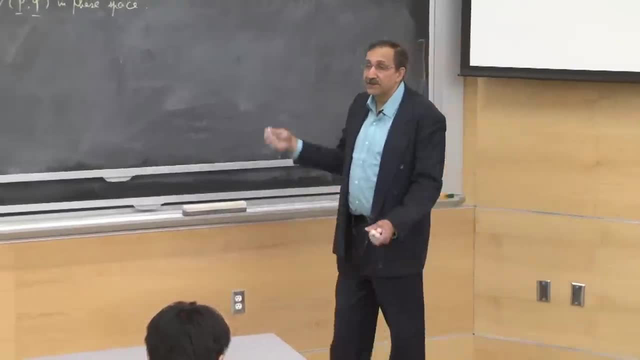 We can have some particular function, such as the kinetic energy sum over i, pi squared over 2m. That's an example of an observable. OK, OK, OK, So you can have kinetic energy, potential energy, anything that you like. 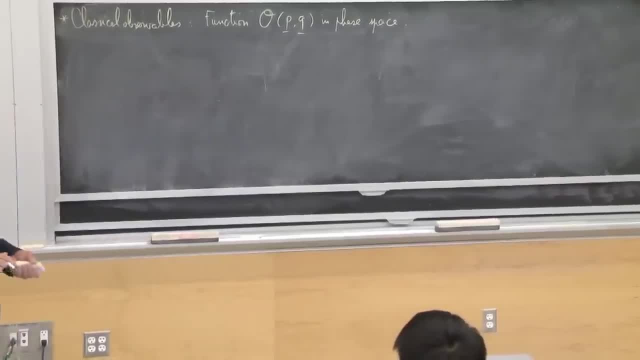 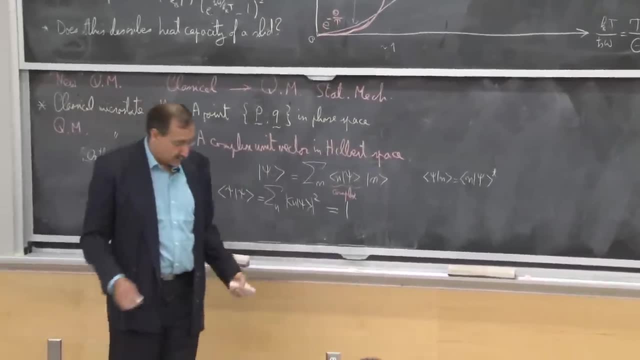 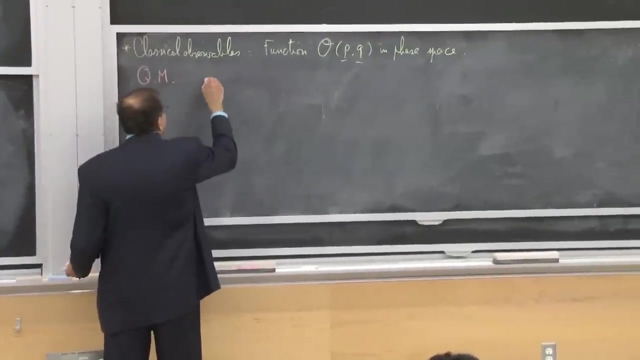 You can classically write as some function that you want to evaluate in phase space. Given that you are at some particular point in phase space, the state of your system- you can evaluate what that is Now in quantum mechanics. observables are operators. 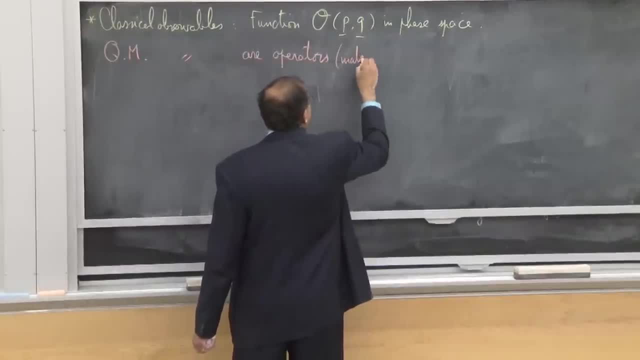 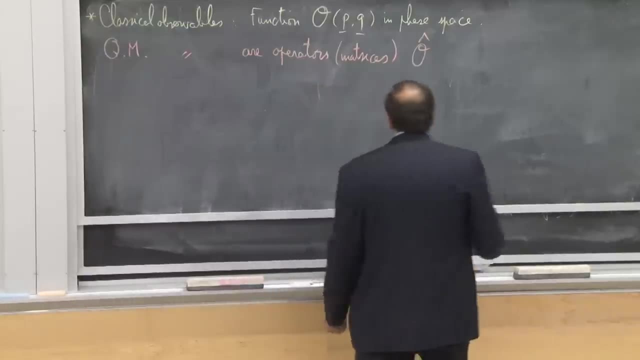 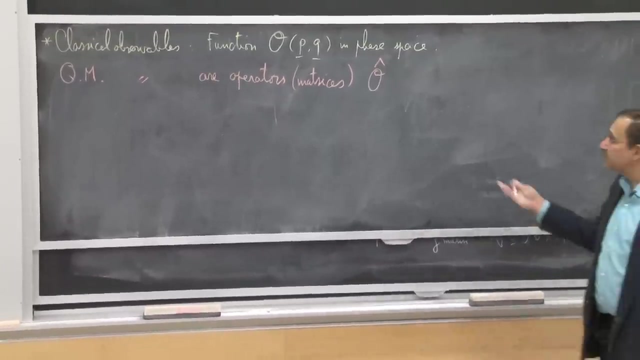 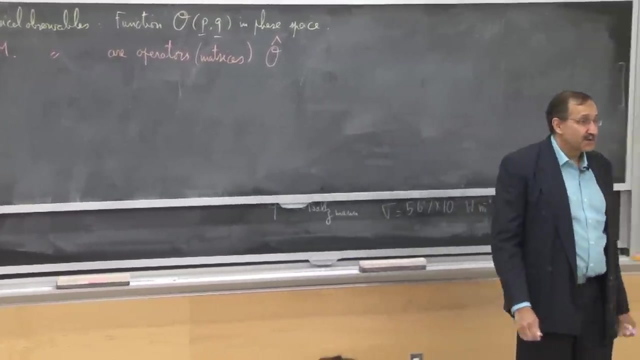 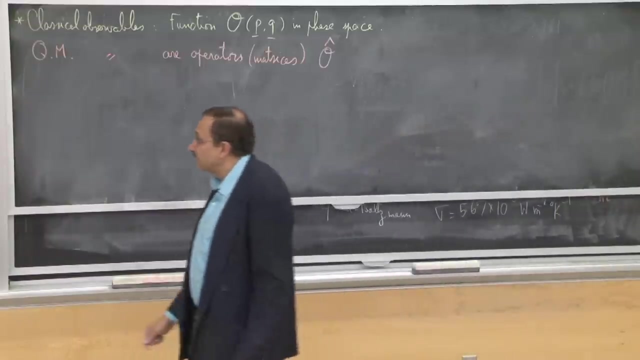 Or matrices, if you like, in this vector space. OK, So among the various observables certainly are things like the position and the momentum of the particle. So there are presumably matrices that correspond to position and momentum, And for that we sort of look at some other properties. 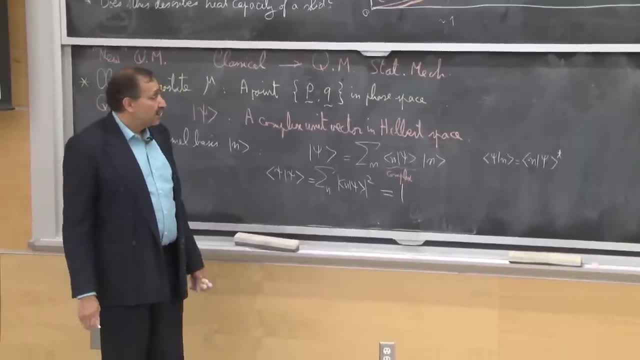 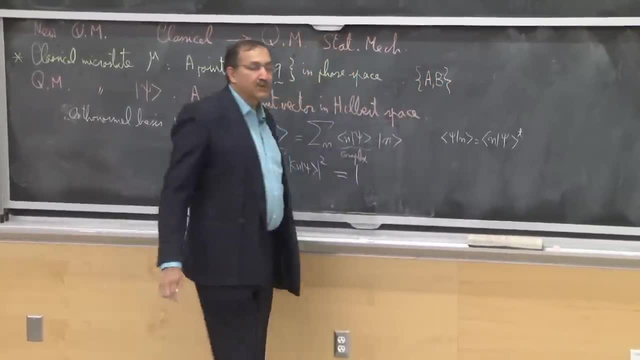 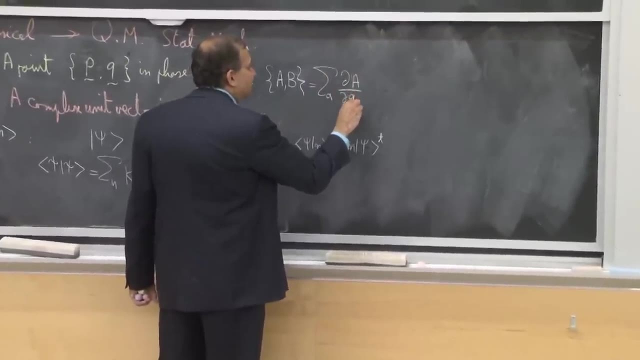 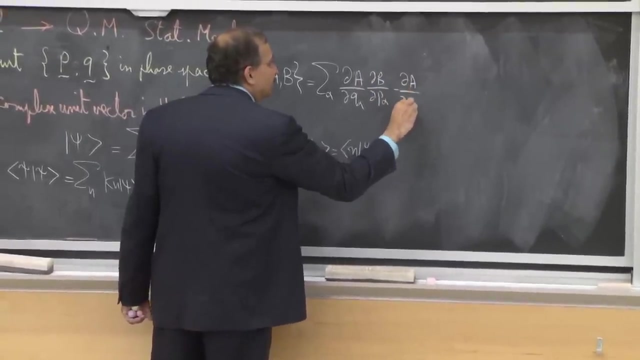 that these classical systems have. We had defined classically a Poisson bracket which was a sum over all alphas: dA by dq alpha. dB by dp. alpha minus dA- OK OK. a by dp alpha. dB by dq alpha- OK. 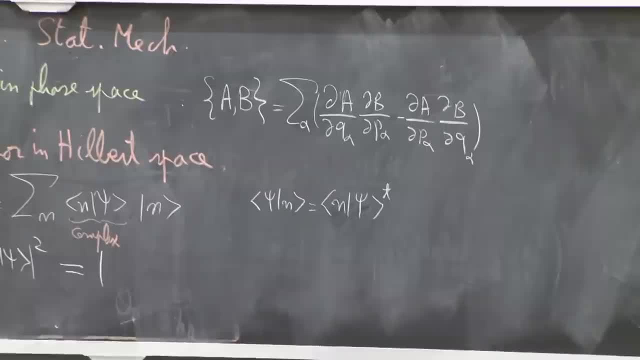 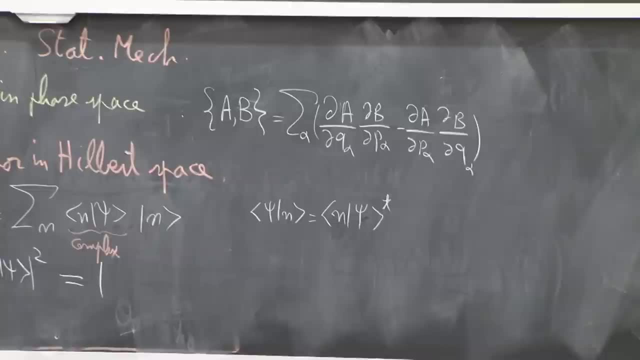 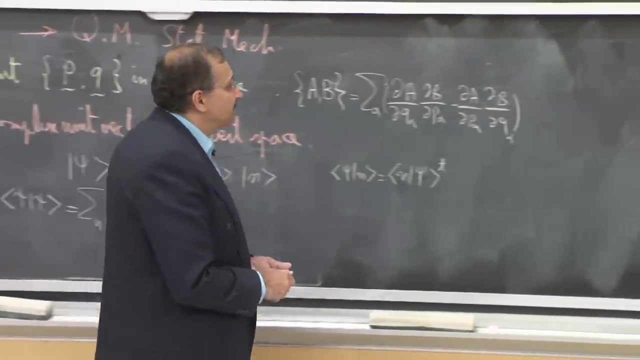 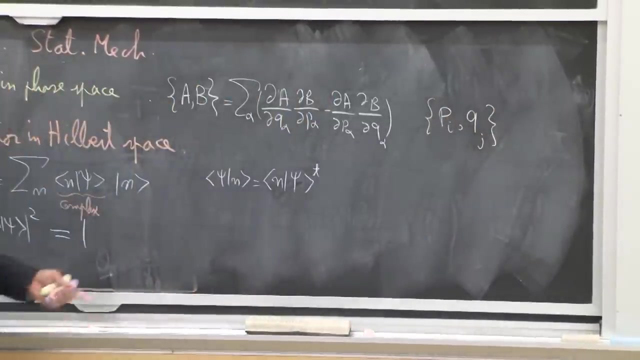 And this is an operation that we would like to and happens to carry over in some sense into quantum mechanics. But one of the consequences of this is you can check that if I pick a particular momentum P and a particular coordinate q and put it over here, 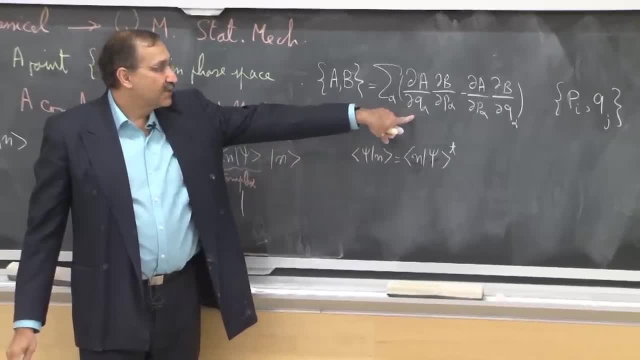 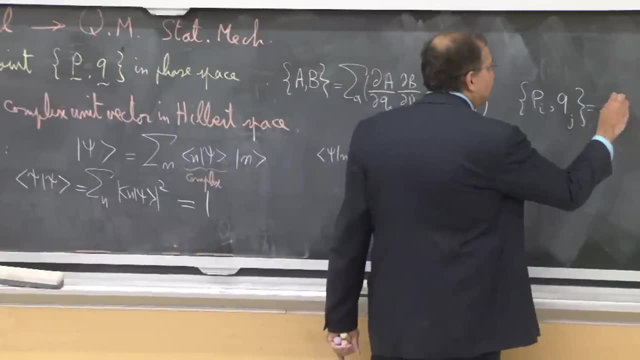 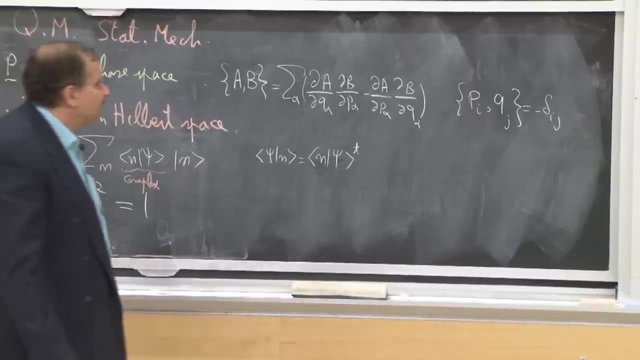 most of the time I will get 0,, unless the alphas match exactly the P q's that I have up there, And if you go through this whole thing, I will get something that is like a delta ij. OK, So this structure somehow continues. 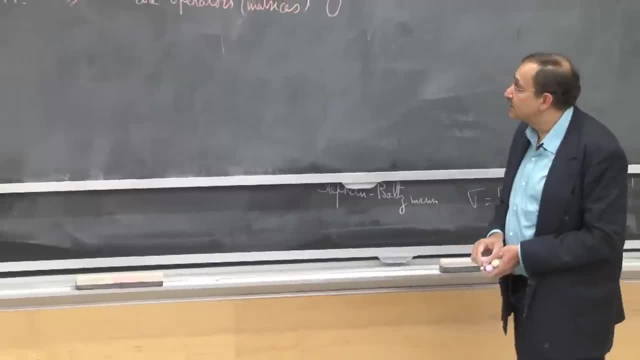 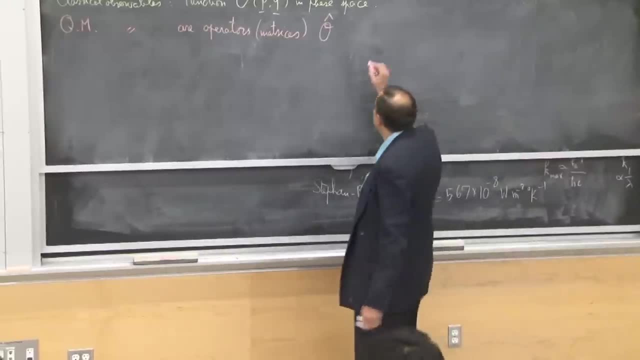 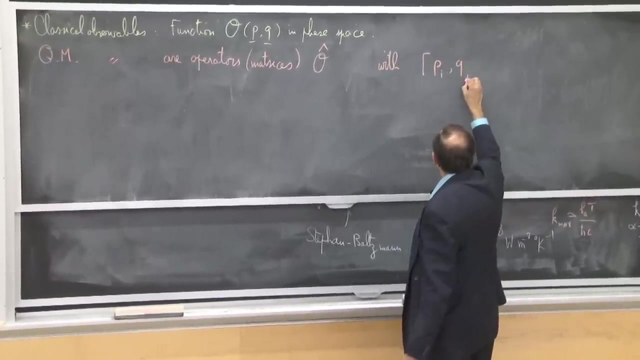 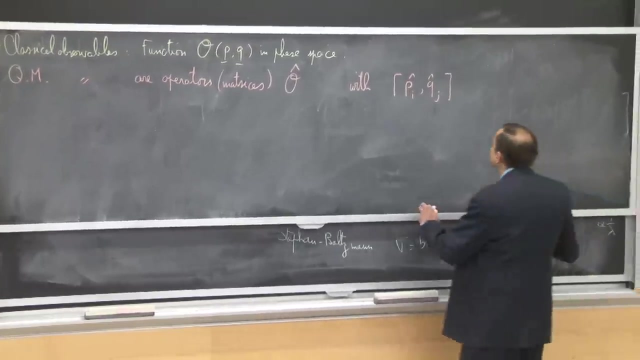 OK, Continues in quantum mechanics, in the sense that the matrices that correspond to P and q satisfy the condition that Pi and qj thinking of two matrices, and this is the commutator. so this is Pi, qj minus qj. 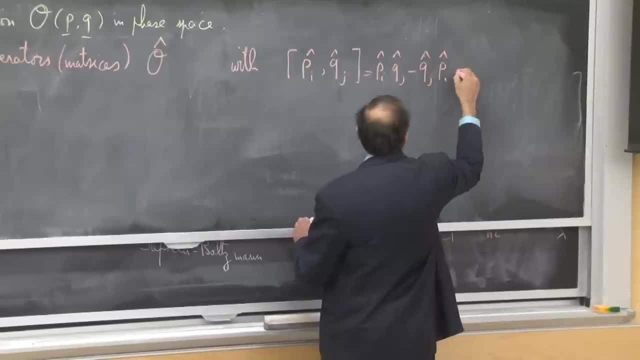 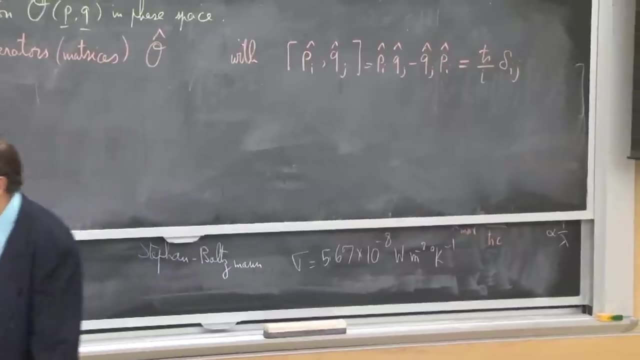 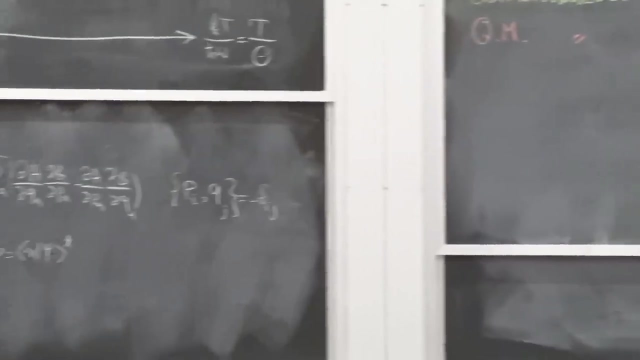 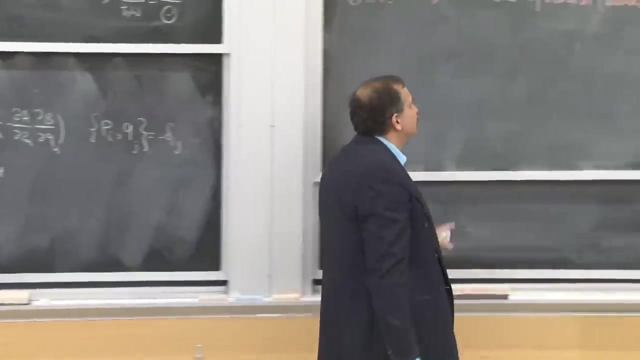 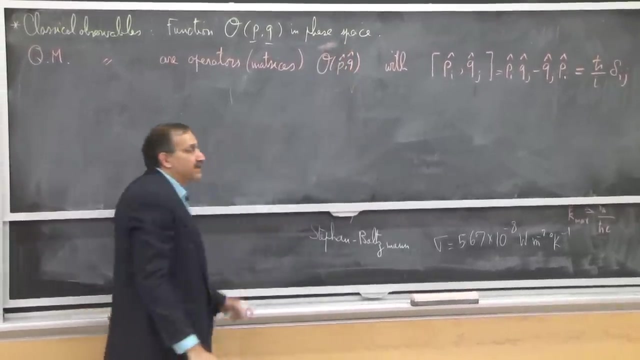 Pi, qj. Pi is h bar over i, delta, ij. So once you have the matrices that correspond to P and q, you can take any function of P and q that you had over here and then replace the P's and q's And then you can take any function of P and q's that. 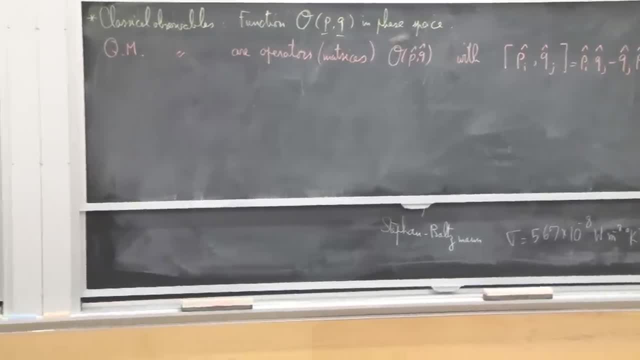 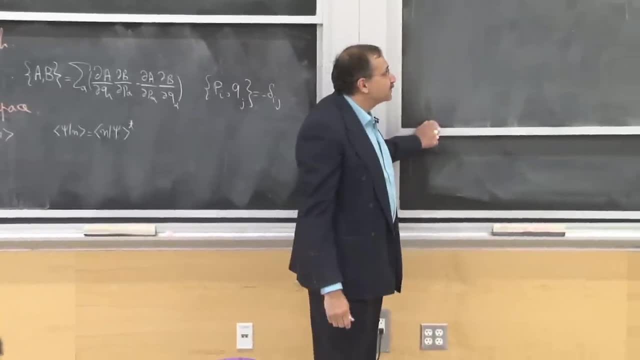 appear in, let's say, a series, expansion or an expansion of this O in powers of P and q, with corresponding matrices, P hat and q hat, And that way you will construct the corresponding operator. There is one subtlety that you've probably encountered. 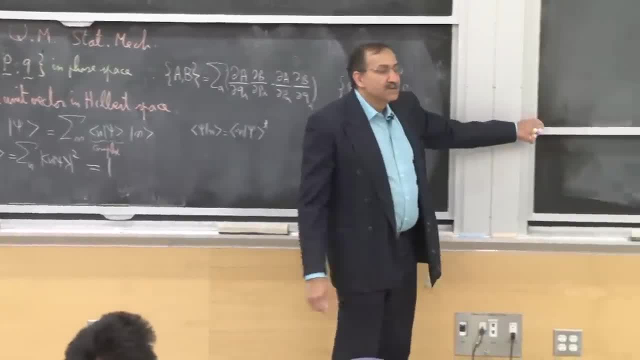 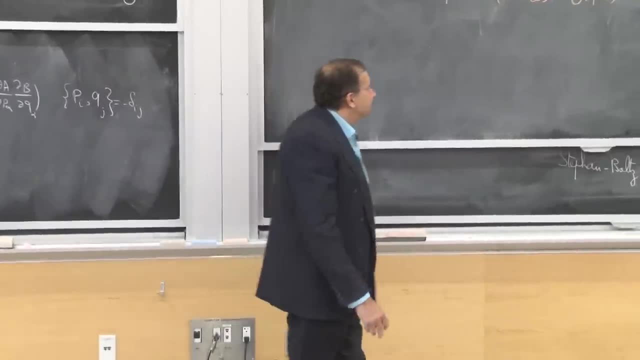 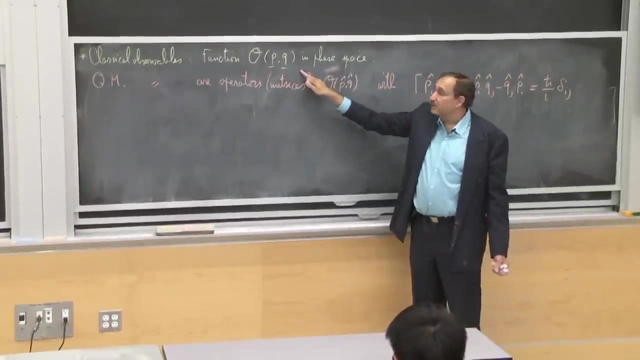 in that there is some symmetrization that you have to do before you can make this replacement OK. So what does this I mean? in classical theory, if something is observable, the answer that you get is a number right. 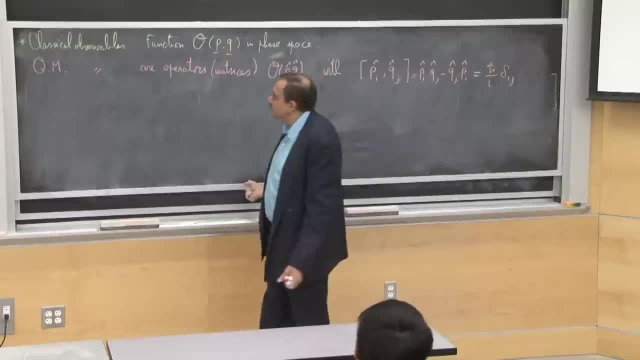 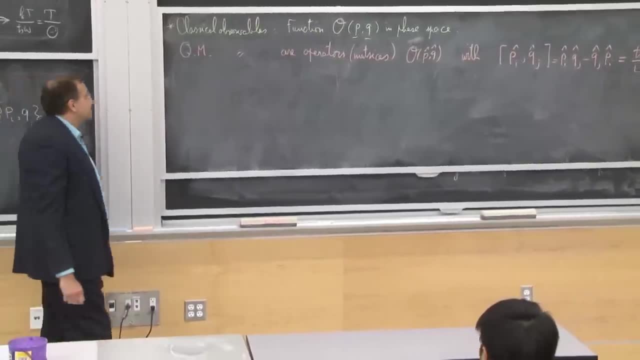 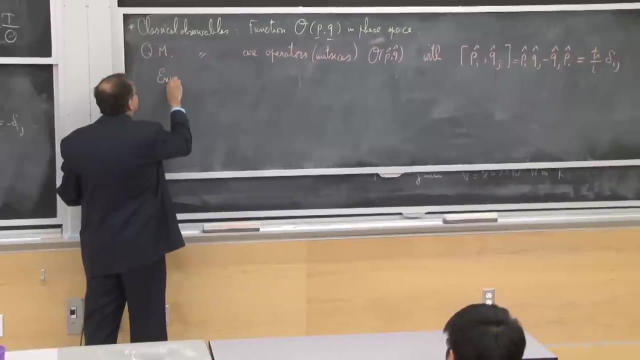 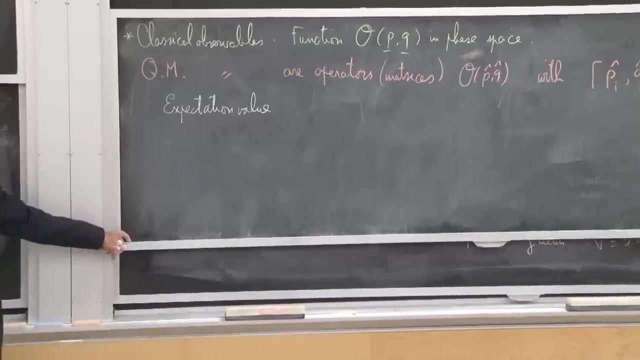 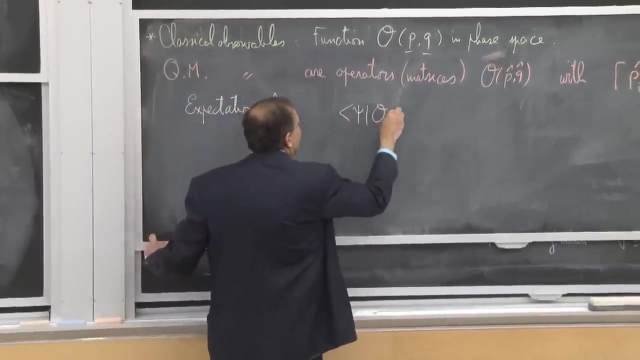 You can calculate what the kinetic energy is In quantum mechanics. what does it mean? that the observable is a matrix? The statement is that observables don't have definite values, but the expectation value of the particular observable O. in some state psi is given by psi, O, psi. 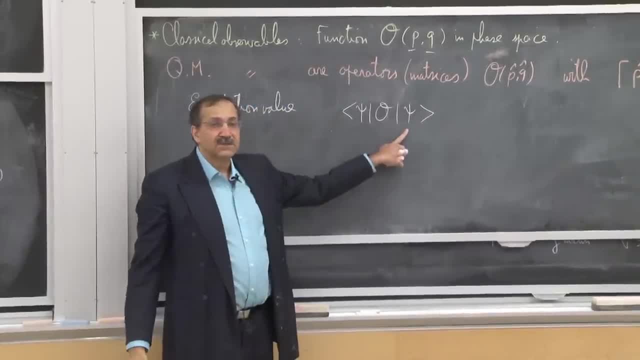 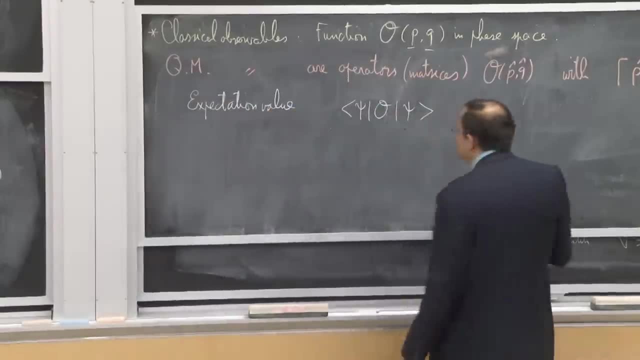 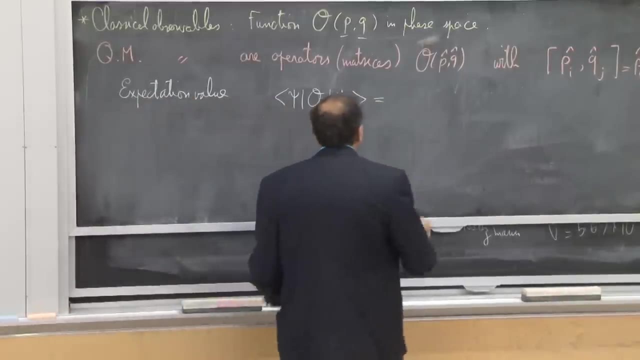 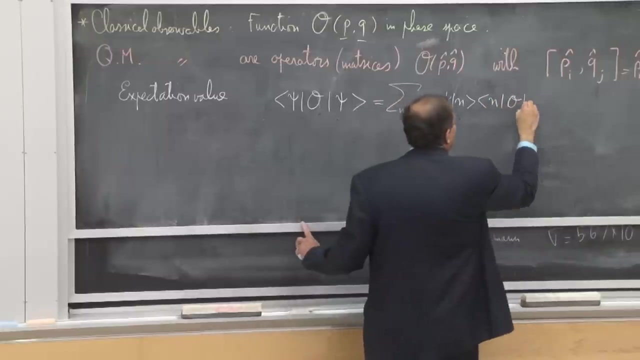 Essentially, you take the vector that corresponds to the state, multiply the matrix on it and then sandwich it with the conjugate of the vector and that will give you your state. So, in terms of elements of some particular basis, you would write this as a sum over n and m psi. n, n, O m m psi. 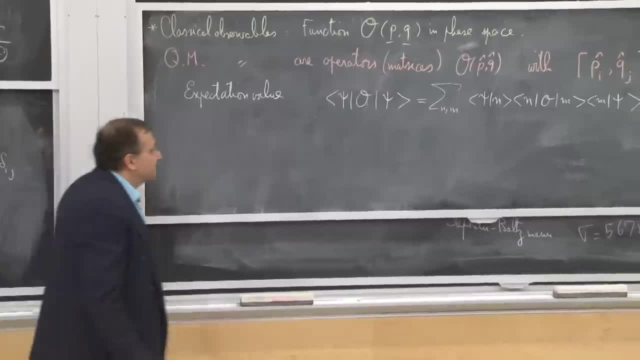 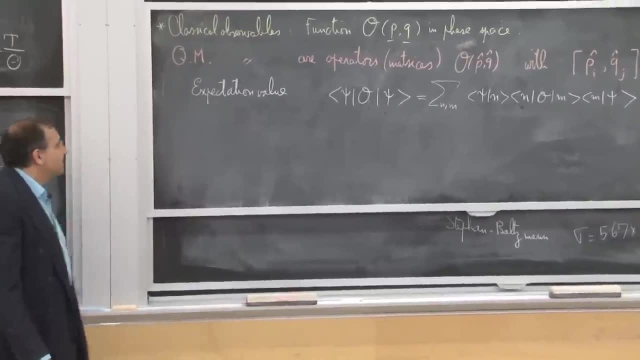 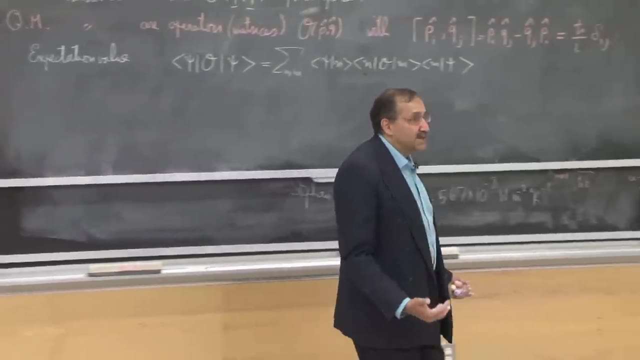 And in that particular basis, your operator would have these matrix elements. Now again, another property: if you are measuring something that is observable is presumably you will get a number that is real. That is, you expect this to be the same thing. 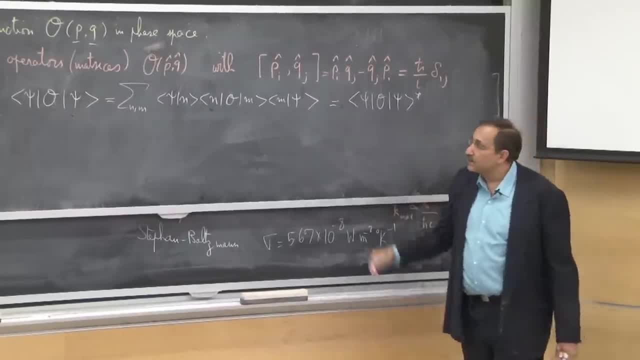 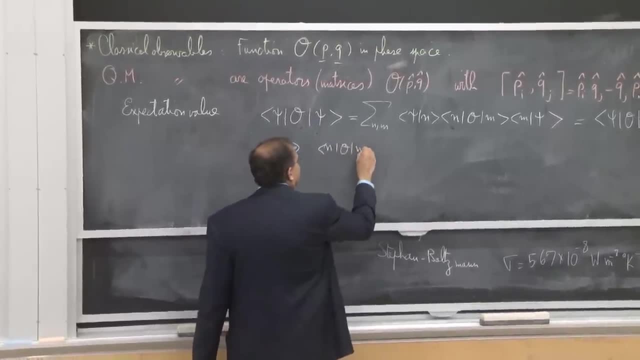 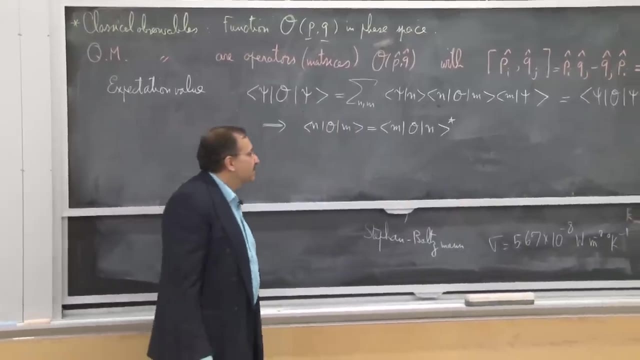 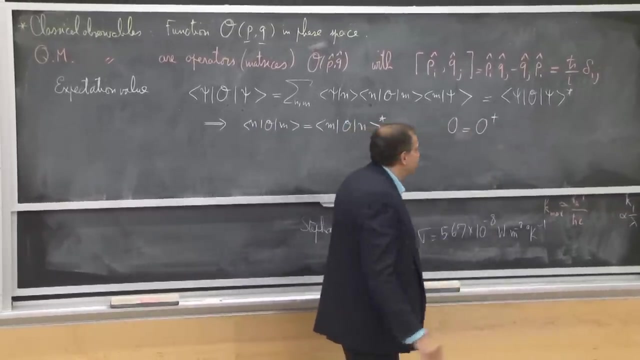 as its complex conjugate, And if you follow this condition, you will see that that reality implies that n O m should be m O n complex conjugate, which is typically written as the matrix: OK, OK, So that's being its Hermitian conjugate. 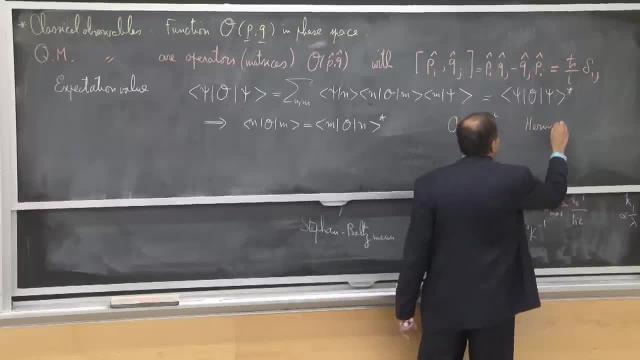 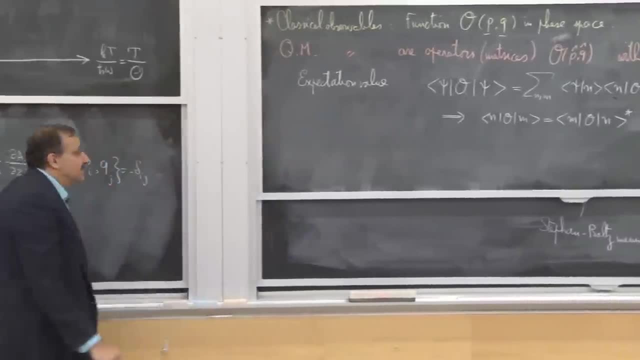 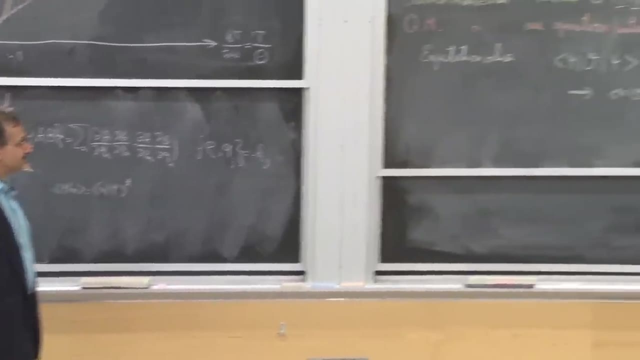 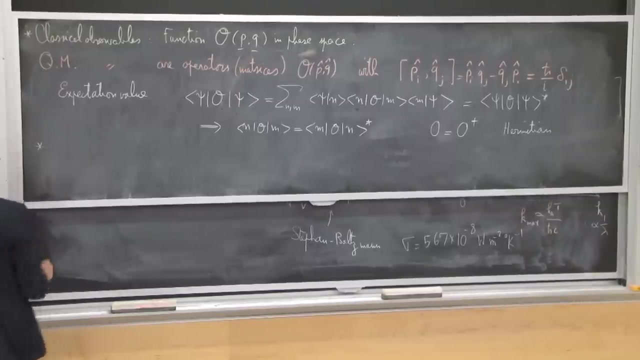 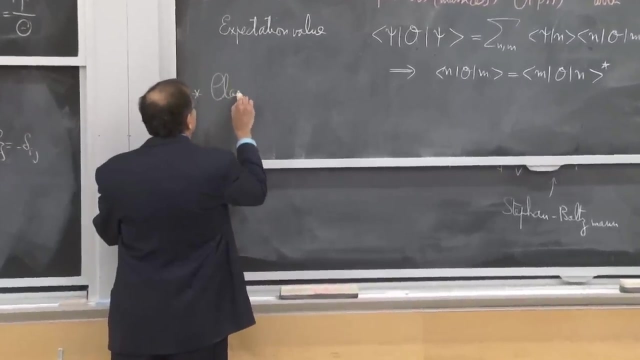 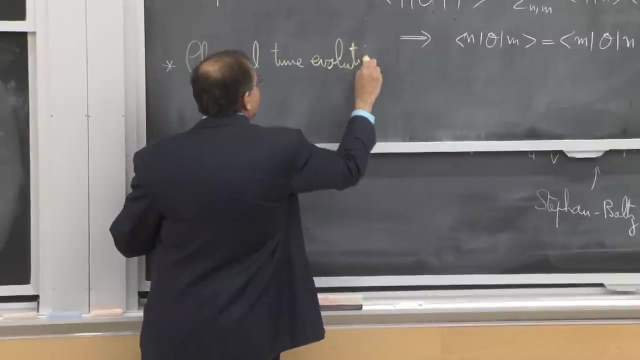 or being Hermitian. So all observables in quantum mechanics would correspond to Hermitian operators or matrices. OK, There's one other piece and then we can forget about Axioms. We have classical time evolution. You know that the particular point in the classical phase 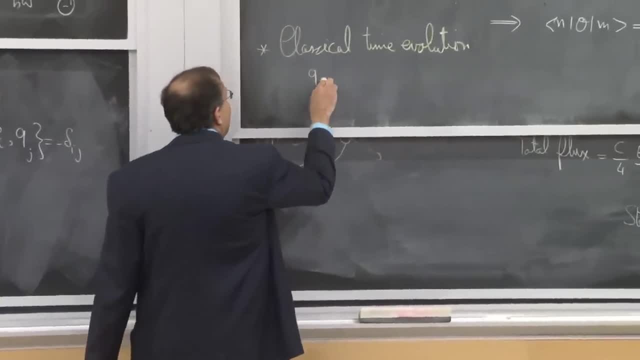 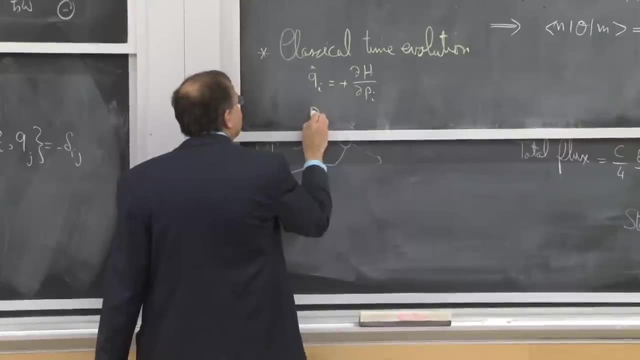 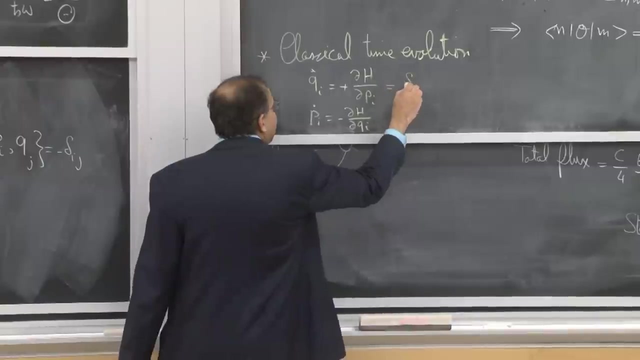 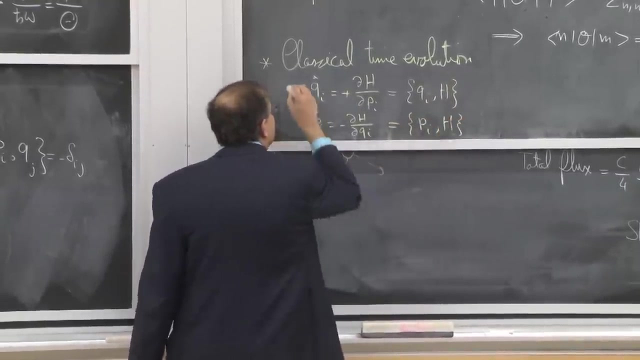 space changes as a function of time, such that qi dot is plus the h by dpi, pi dot is minus the h by dqi. By the way, both of these can be written as qi and h Poisson bracket and pi and h Poisson bracket. 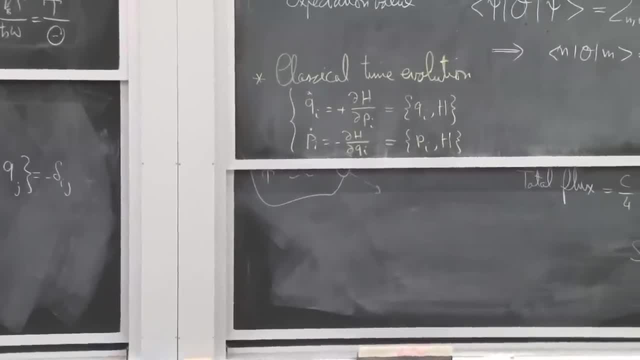 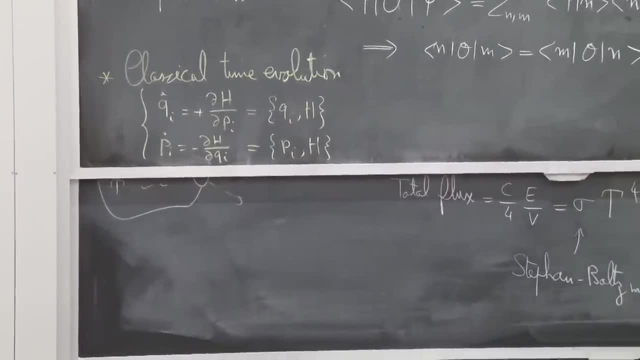 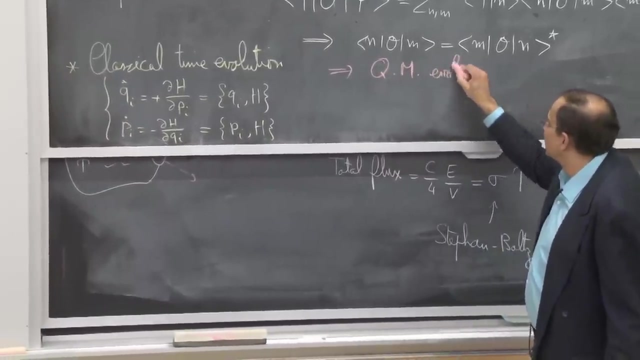 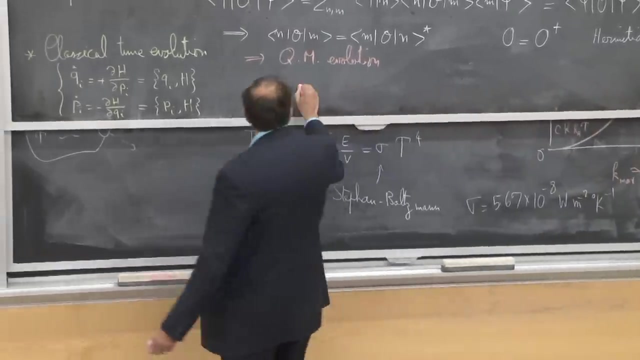 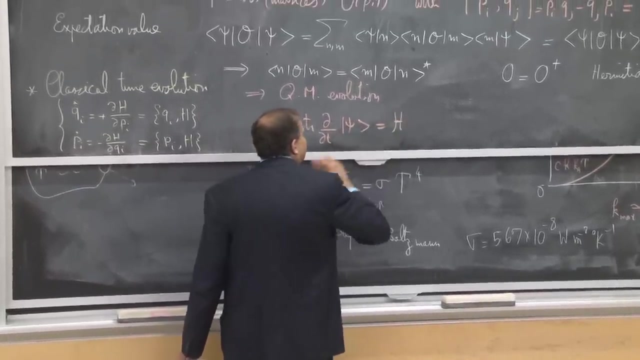 But there is a particular function, observable h, the Hamiltonian, that derives the classical evolution. When we go to quantum evolution, this vector that we have in Hilbert space evolves according to i h bar d by dt of the vector psi is the matrix H acting on psi. 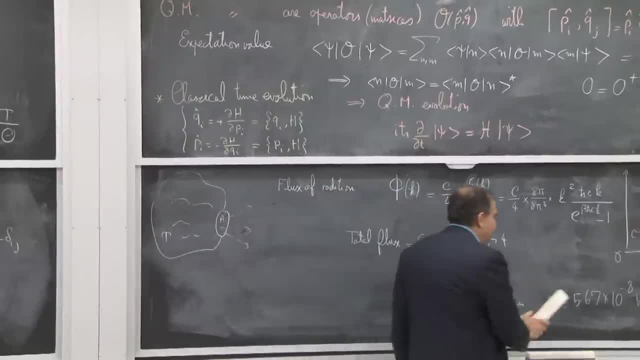 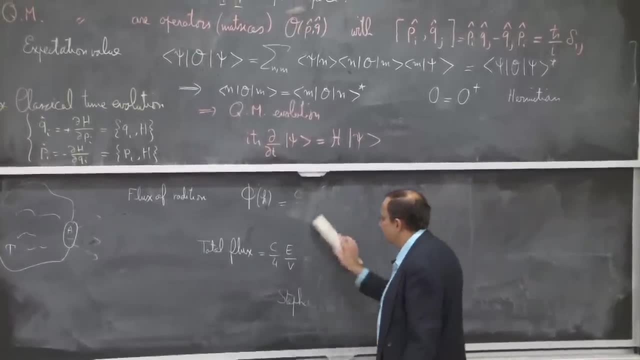 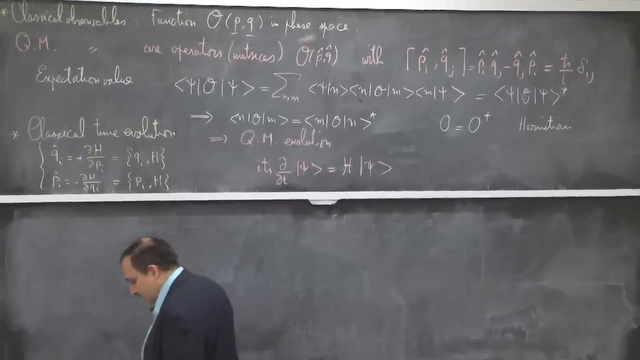 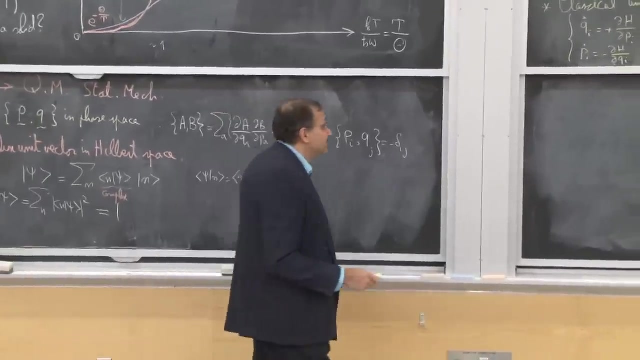 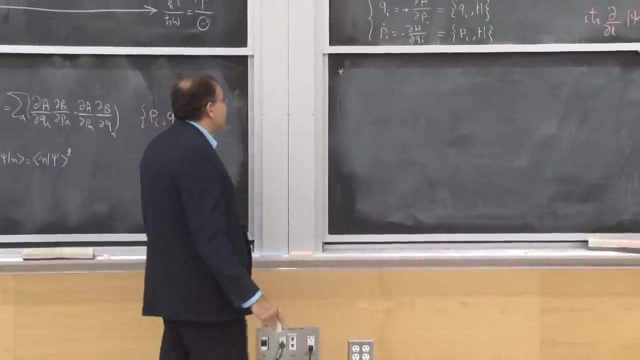 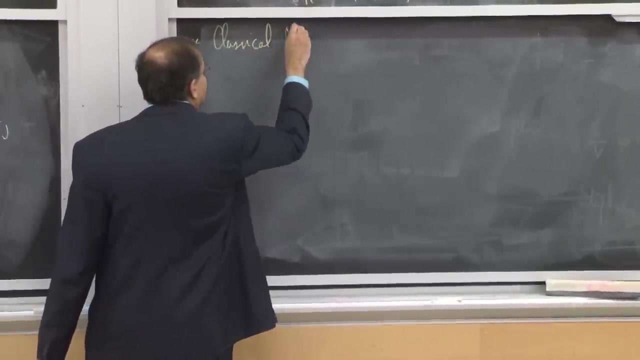 OK, Fine, So these are The basics that we need. Now we can go and do statistical descriptions. So the main element that we had in constructing statistical descriptions was dealing with the macro state. We said that if I'm interested in thinking about the properties, 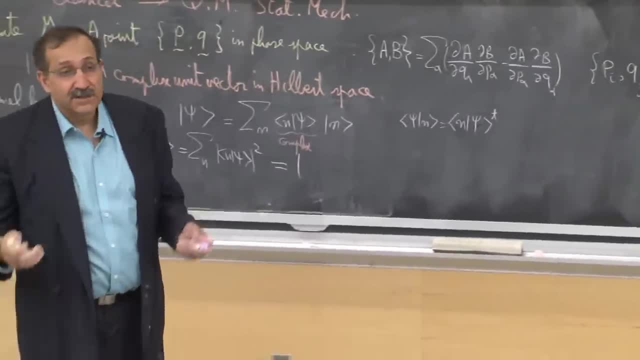 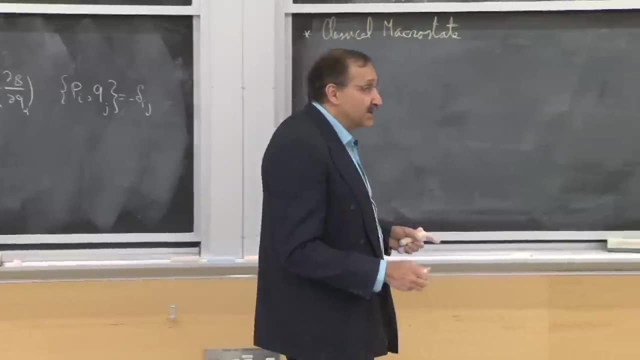 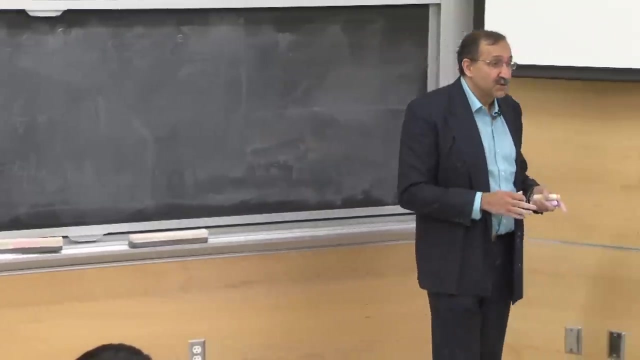 of one cubic meter of gas at standard temperature and pressure. I'm not thinking about a particular point in phase space, because different gases that have exactly the same macroscopic properties would correspond to many, many different possible points in this phase space that are changing as a function of time. 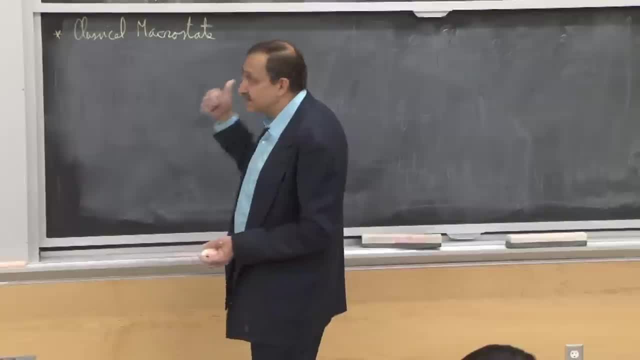 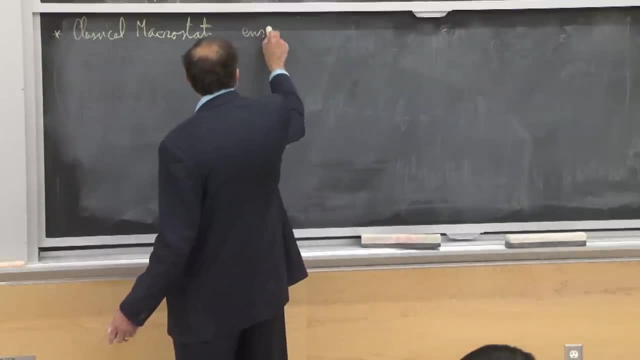 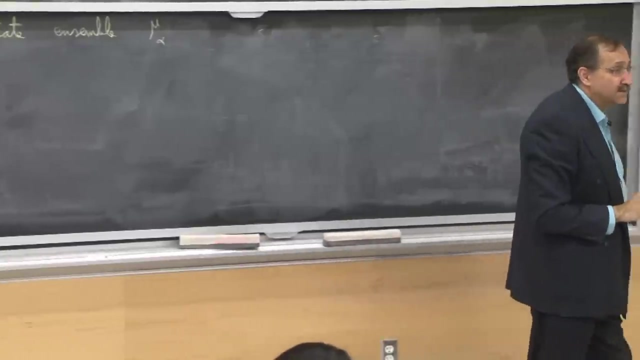 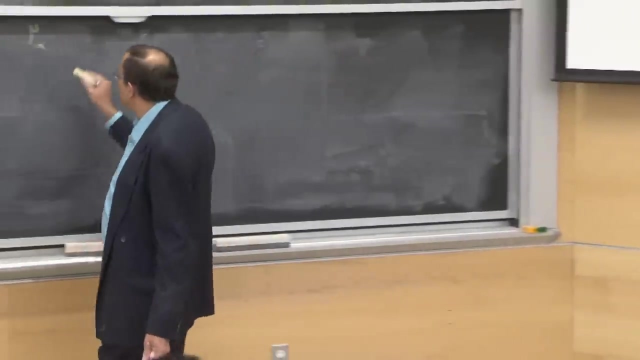 So rather than thinking about a single microstate, we thought about an ensemble, And this ensemble had a whole bunch of possible microstates. In the simplest prescription maybe we said they were all equally likely, But actually we could even assume And assign some kind of probability to them. 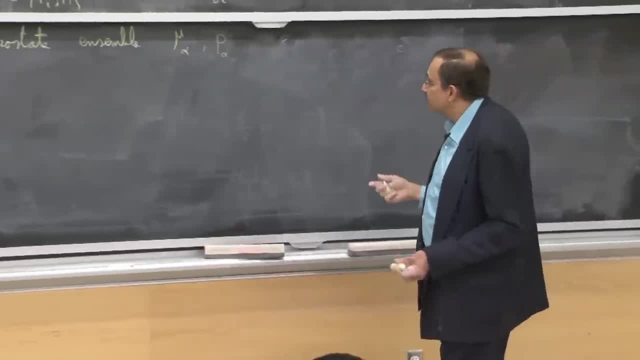 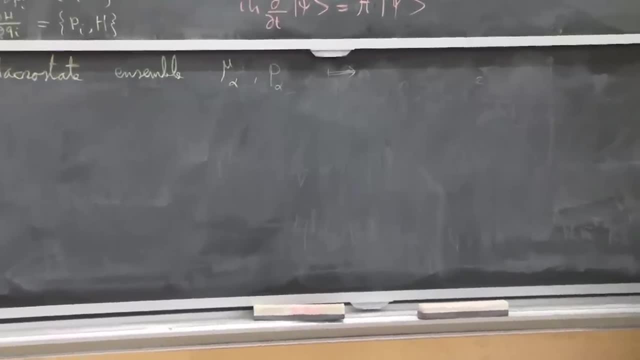 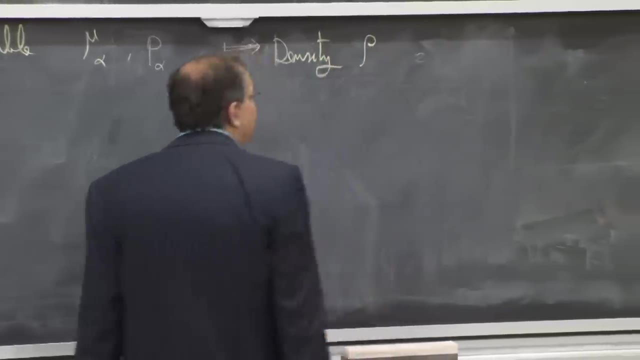 And we want to know what to do with this, Because then what happened was from this description. we went and constructed a density, which was again some kind of a probability in phase space, And we looked at it. OK, OK. 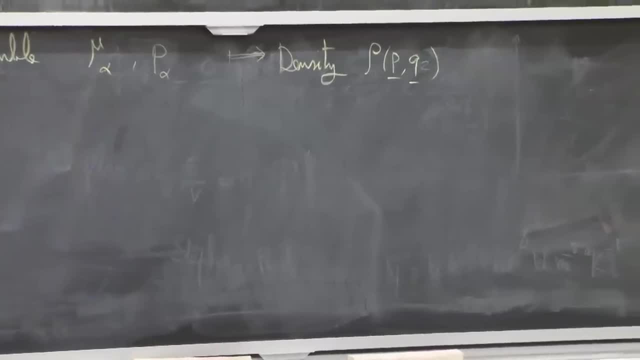 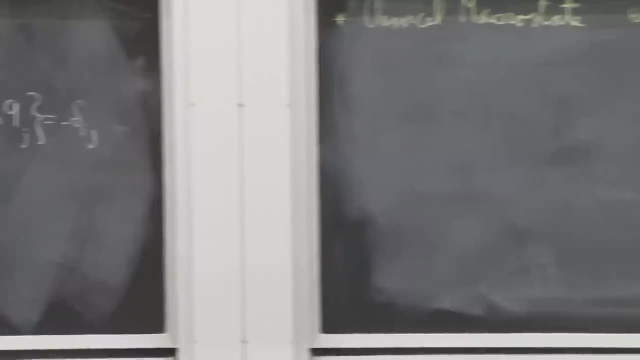 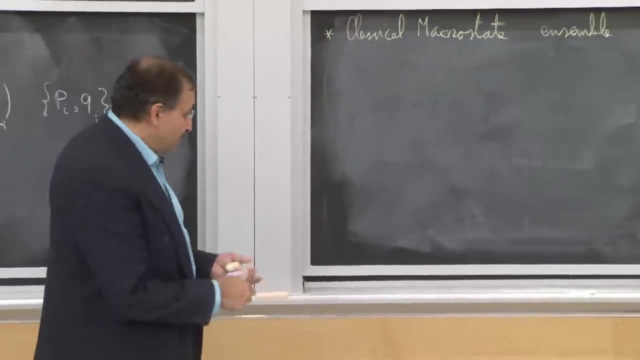 We looked at its time, evolution, We looked at the averages and all kinds of things in terms of this density. So the question is: what happens to all of this when we go to quantum descriptions? OK, We can follow a lot of that. 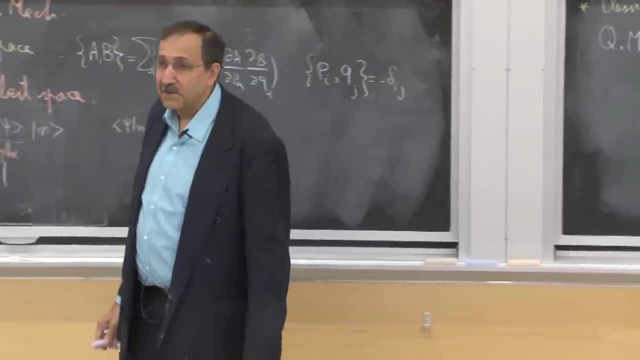 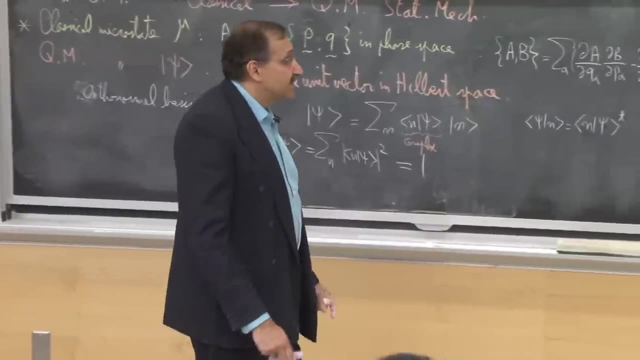 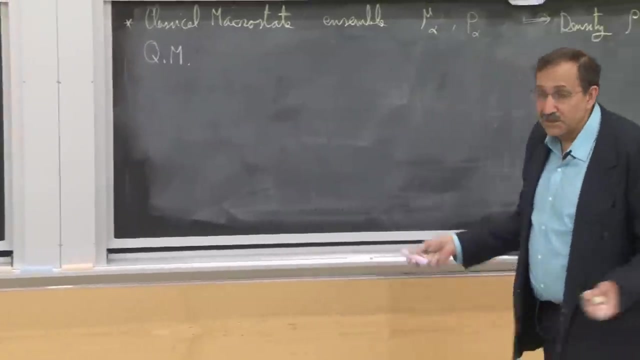 We can again take the example of the one cubic meter of gas at standard temperature and pressure. OK, But rather than describing the state of the system classically, I can try to describe it quantum mechanically. Presumably the quantum mechanical description. 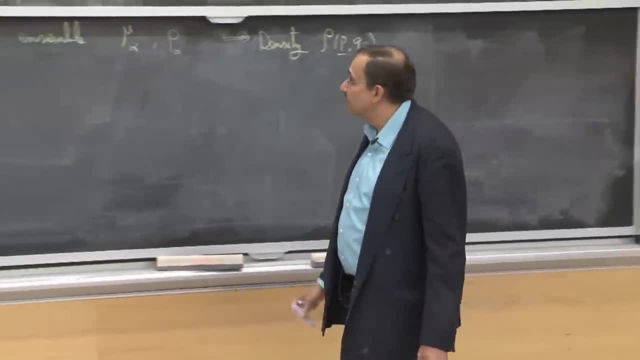 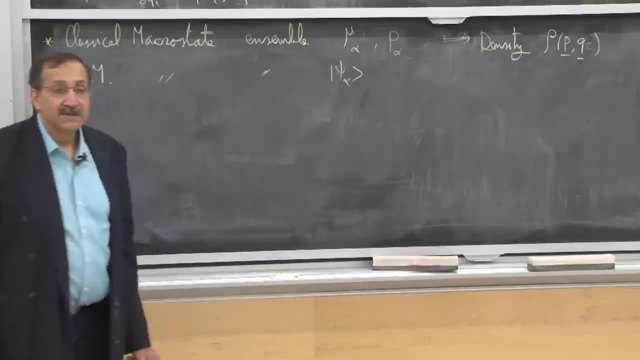 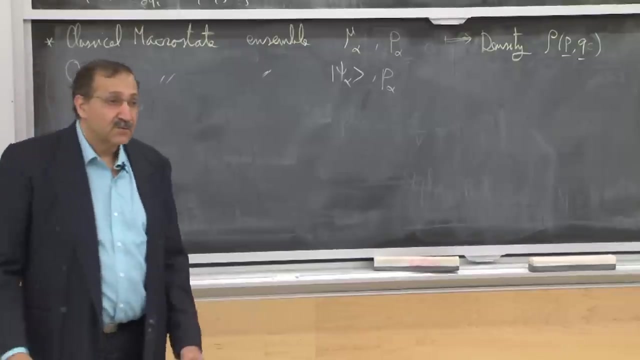 at some limit becomes equivalent to the classical description. So I will have an ensemble of states. I don't know which one of them I am in. I have lots of boxes that would correspond to different. I don't know which one of them I am in. 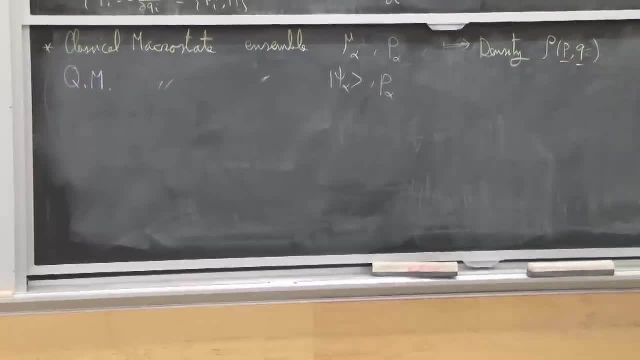 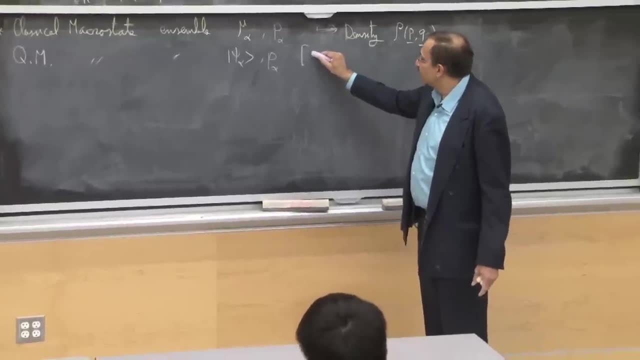 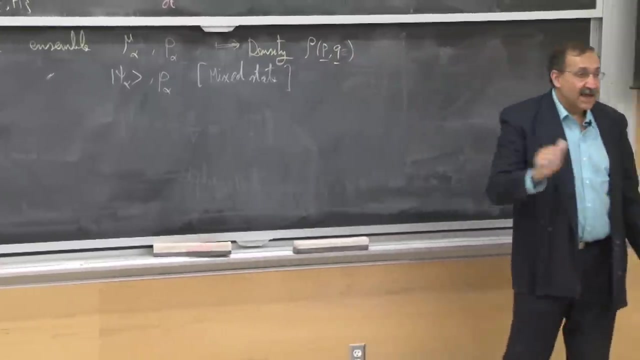 Microstates, presumably. And this has actually a word that is used more in the quantum context. I guess one could use it in the classical context: It's called a mixed state. A pure state is one you know exactly. Mixed state is well like the gas, I tell you. 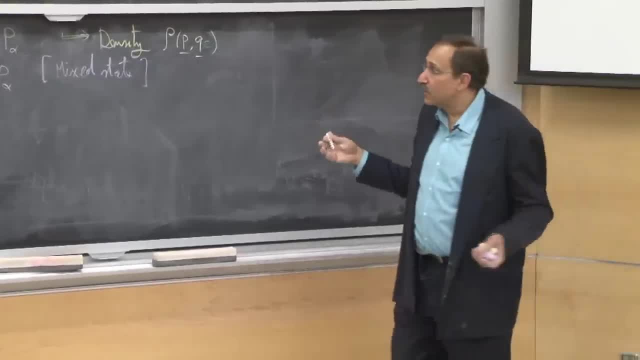 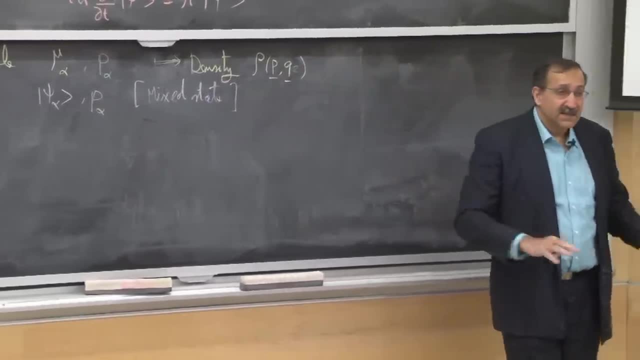 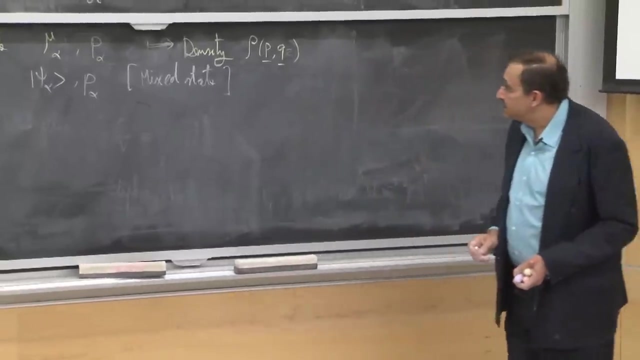 I tell you only the macroscopic information. You don't know much about, microscopically, what it is. There's possibilities And not knowing those possibilities, you can say that it's a mixture of all of these states. OK, Now, what would I use classically, a density for. 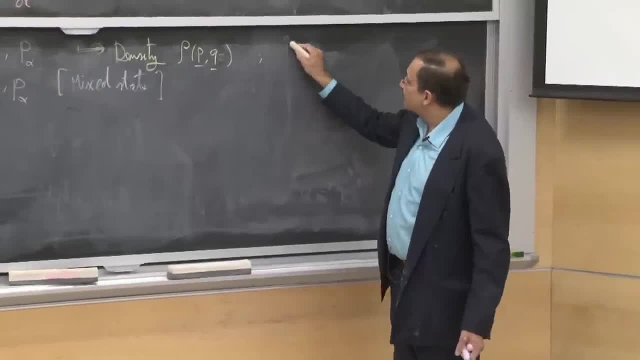 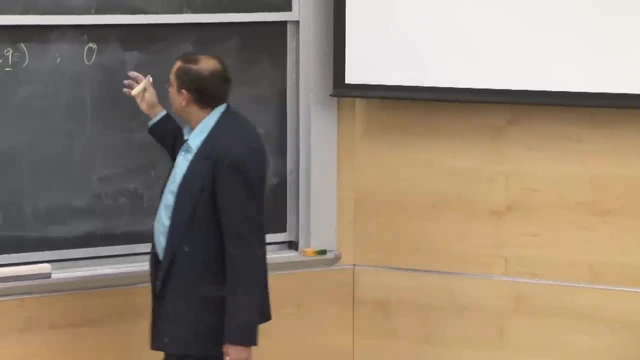 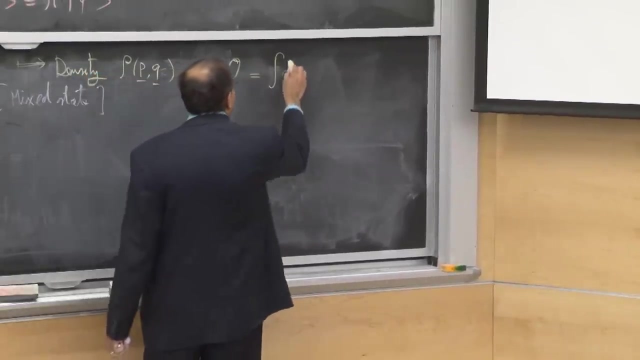 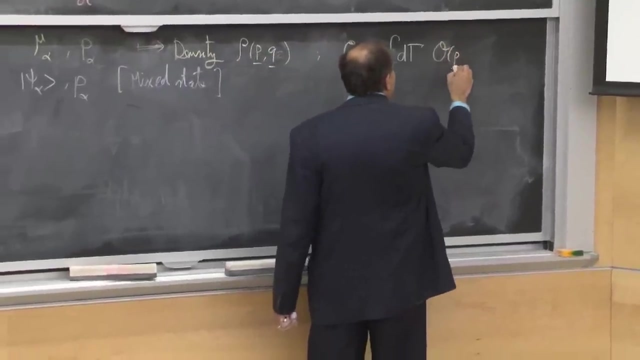 What I could do is I could calculate the average of some observable classically in this ensemble And what I would do Is I would integrate, over the entirety of the 6n dimensional phase space, the O at some particular point in phase space and the density at that point in phase space. 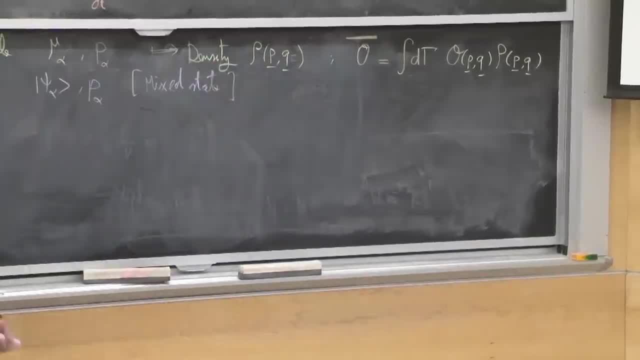 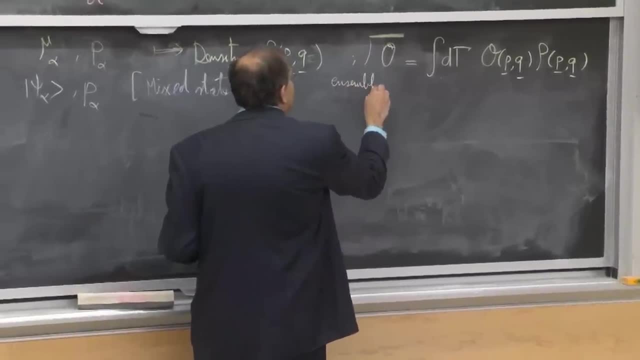 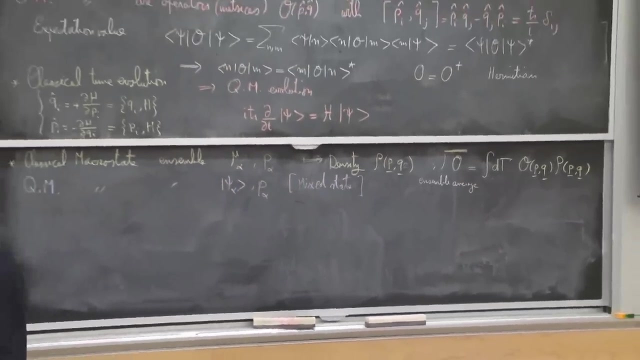 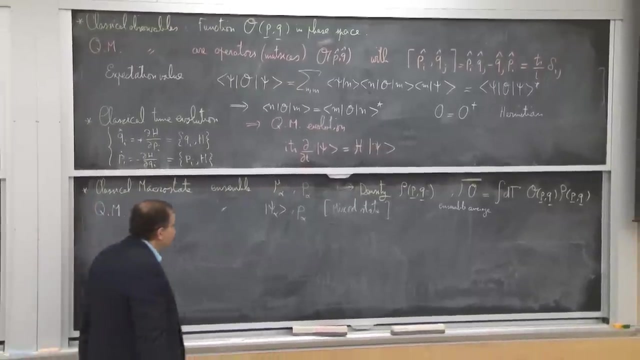 And this average I will indicate by a bar. So my bars stand for ensemble average to make them distinct From these quantum averages that I will indicate with the brackets. OK, So let's try to do the analog of that in quantum states. 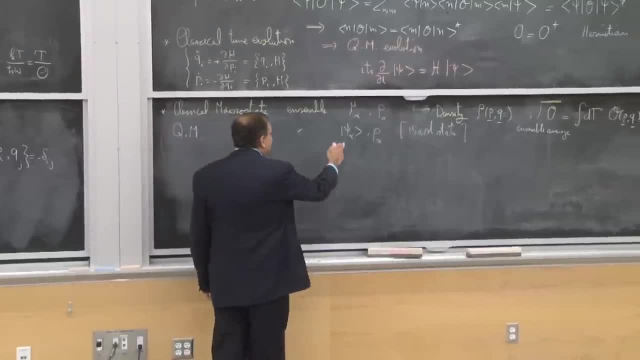 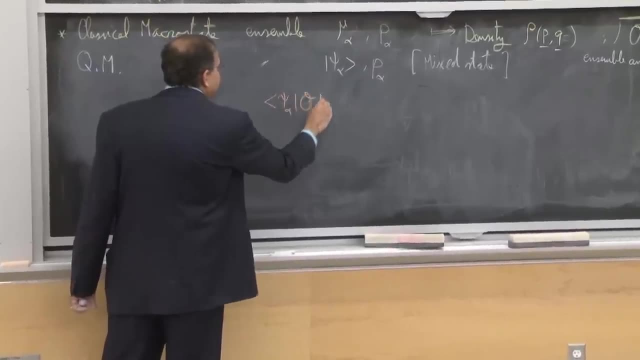 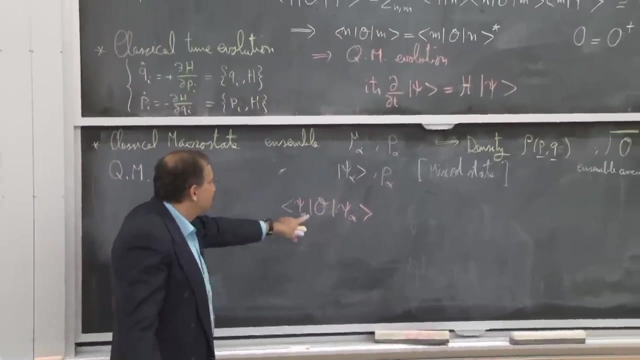 I would say that, OK, for a particular one of the members of this ensemble, I can calculate what the expectation value is. This is the expectation value. OK, That corresponds to this observable O if I was in a pure state. psi alpha. 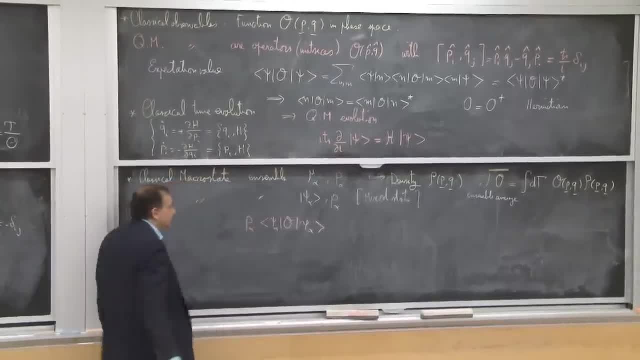 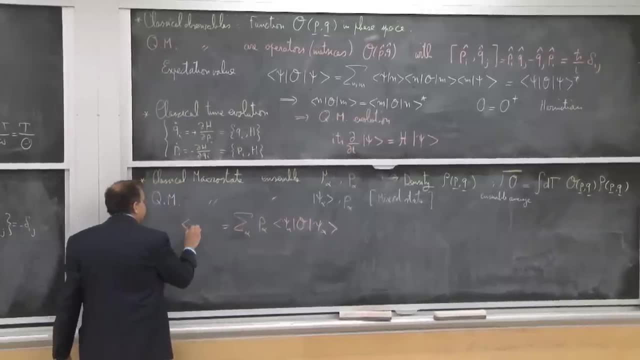 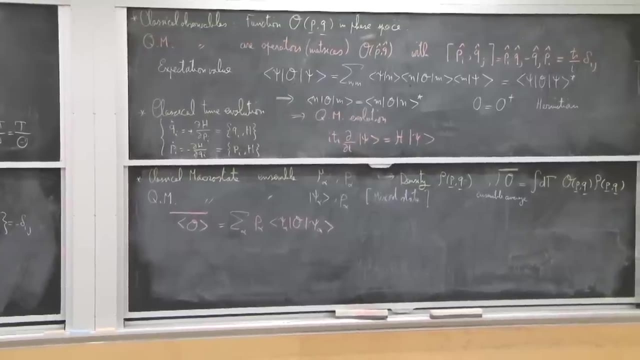 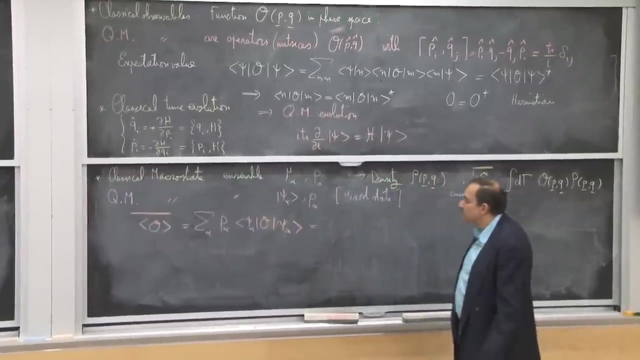 But I don't know that. I'm there, I have a probability, So I do a summation over all of these states And I will call that expectation value, ensemble average. OK, So that's how things are defined. OK, Let's look at this in some particular basis. 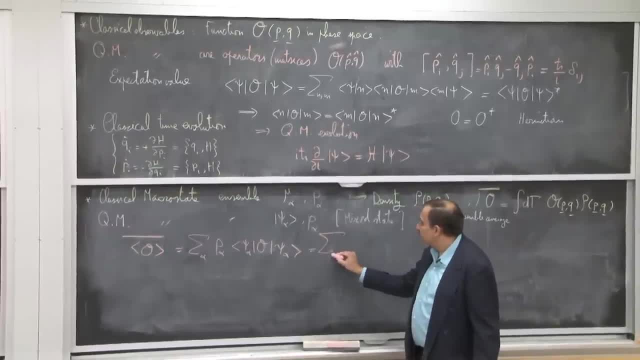 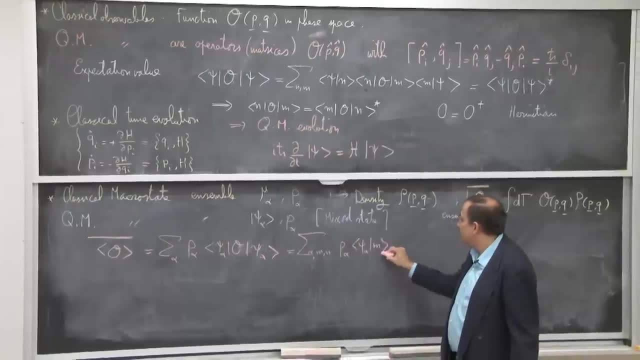 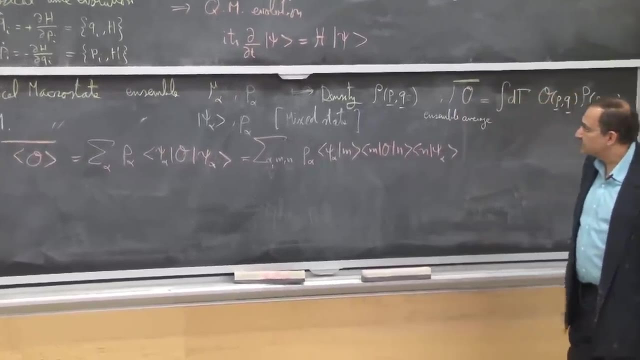 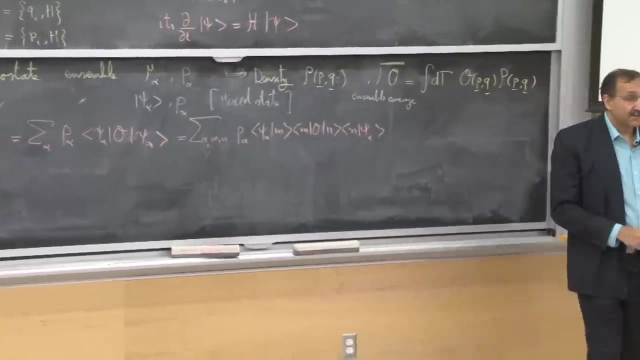 I would write this as a sum over alpha m and n p alpha psi alpha m m O n n psi alpha. So essentially writing all of these psi's in terms of their components, just as I had done above. OK. 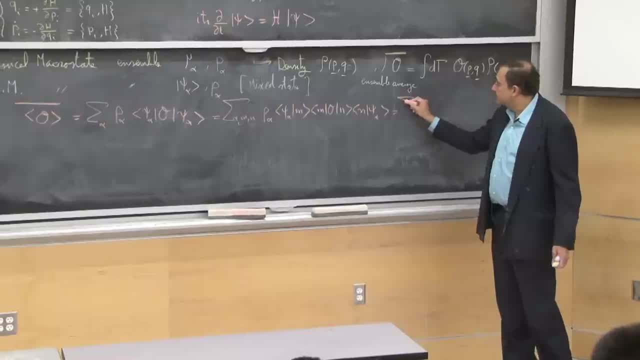 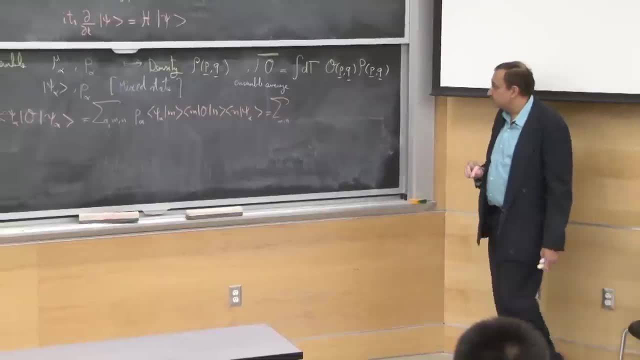 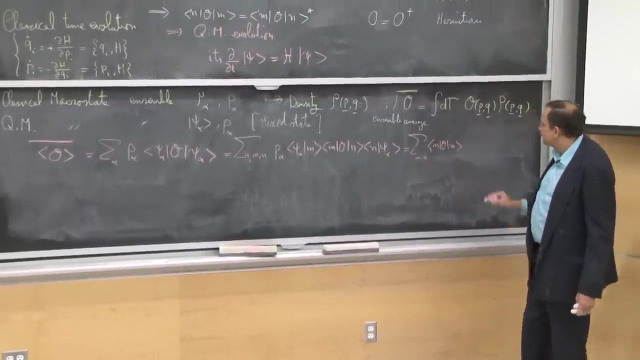 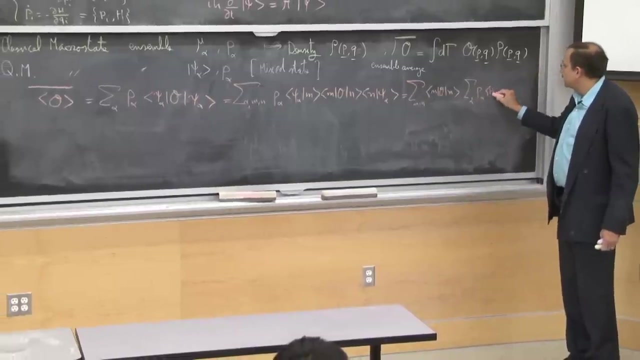 Now what I want to do is to reorder this. Do the summation over m and n first, The summation over alpha last. So what do I have? I have m O n, And then I have a sum over alpha of p, alpha, n, psi, alpha. 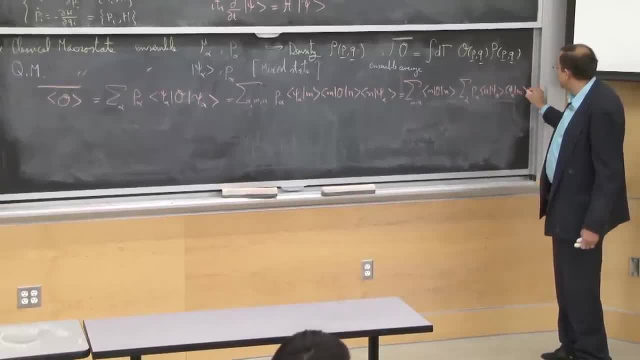 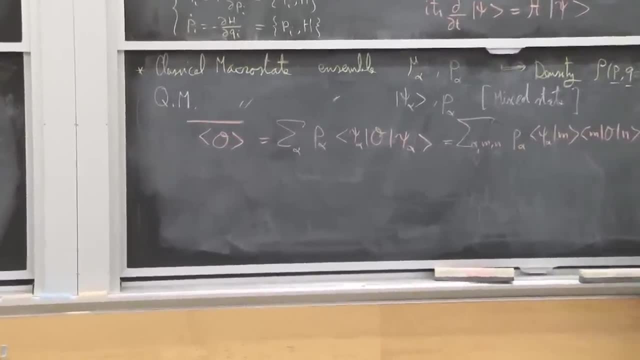 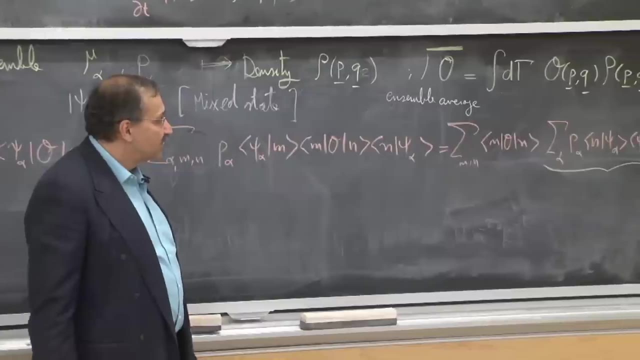 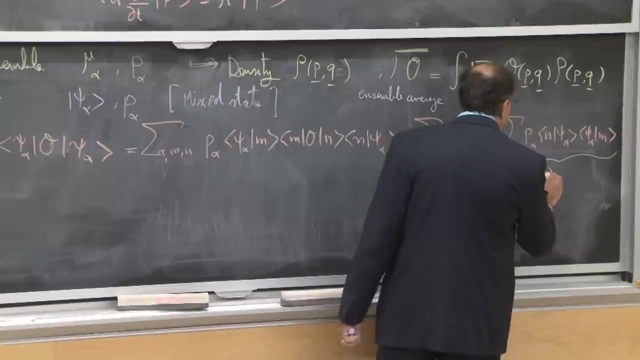 p alpha, psi, alpha m. So what I will do this quantity, that alpha is summed over, so it depends on the two indices n and m. I can give it a name. I can call it n rho m. OK. 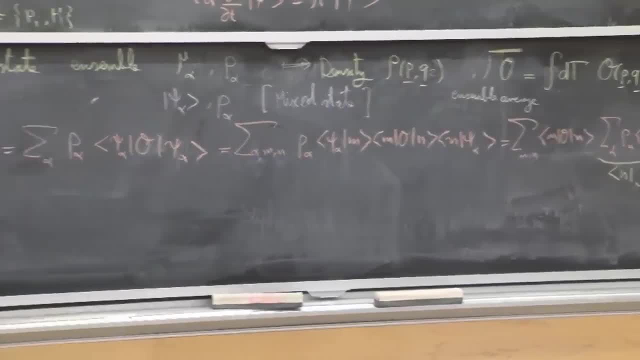 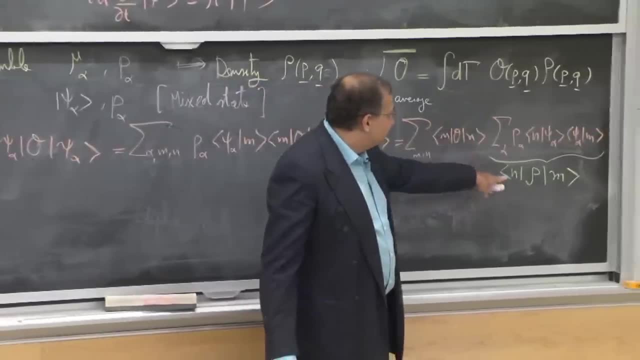 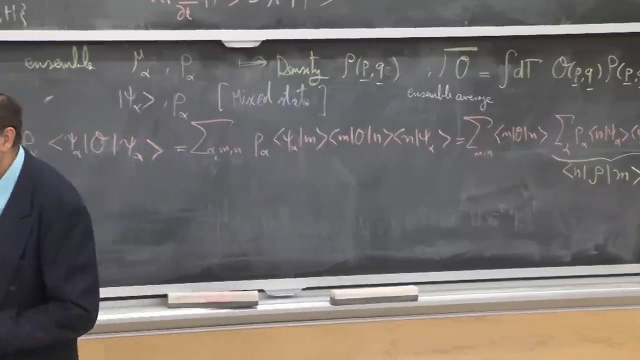 OK, OK, If I do that, then this O bar average becomes simply: well, let's see This: summation over n gives me the matrix product O rho, And then summation over m gives me the trace of the product. 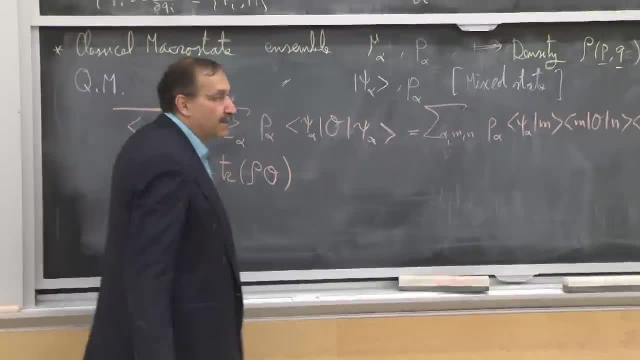 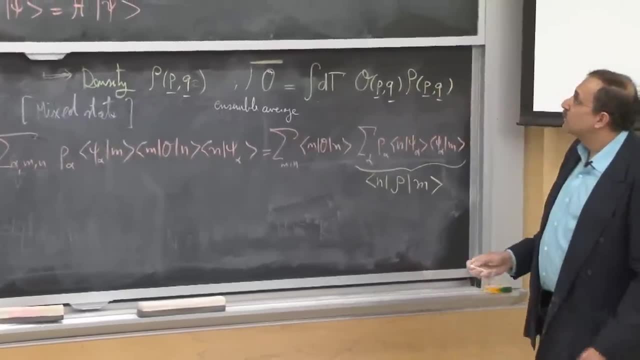 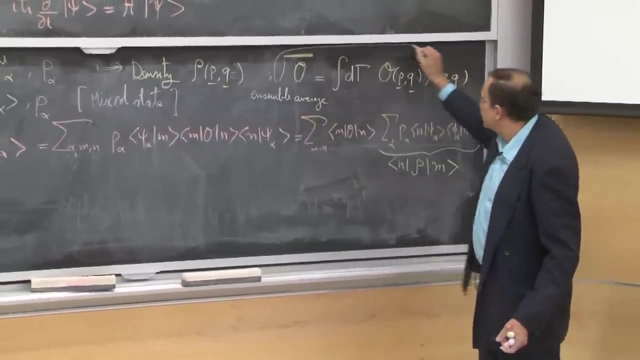 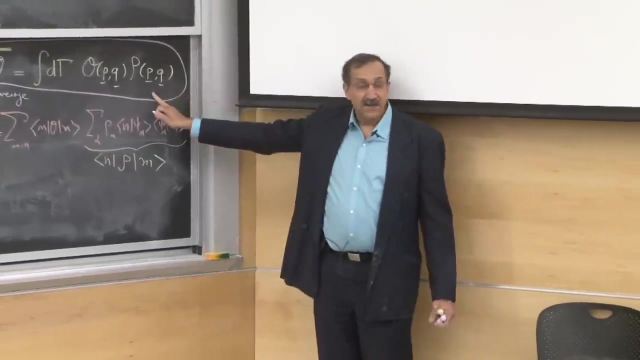 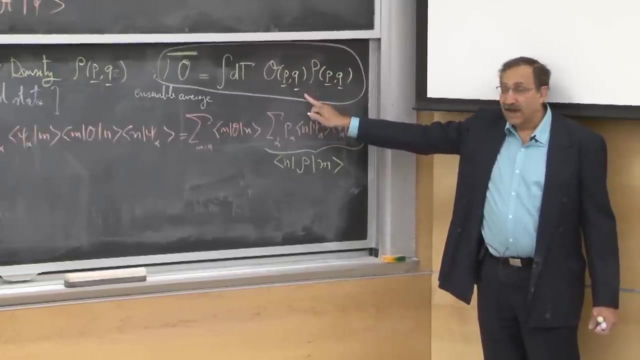 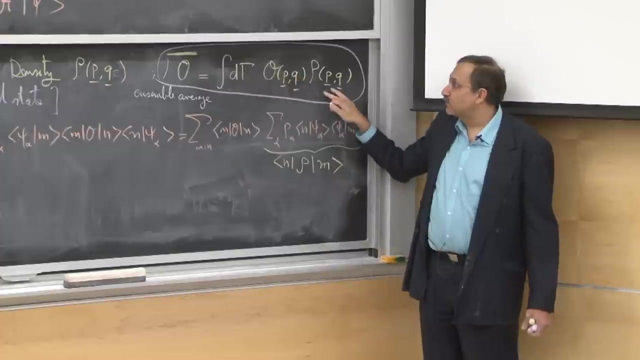 So this is the trace of rho. O OK, So I constructed something that is kind of analogous to the classical use of the density in phase space. So you would multiply the density and the thing that you wanted to calculate observable, And the ensemble average is obtained as a kind of summing. 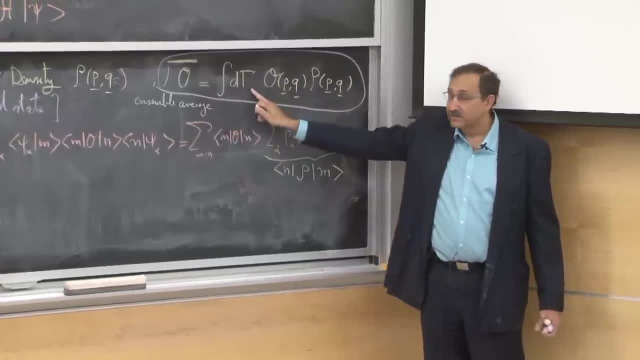 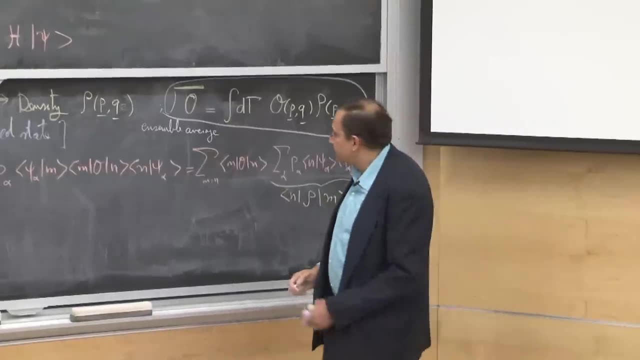 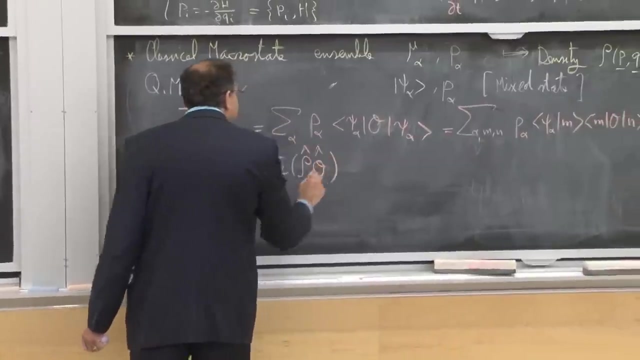 over all possible values of that product, This product in phase space. So here I'm doing something similar. I'm multiplying this O by some matrix rho. So again, this I can think of as having introduced a new matrix on an operator. 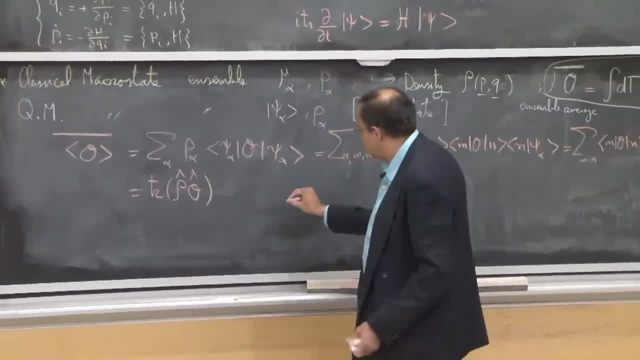 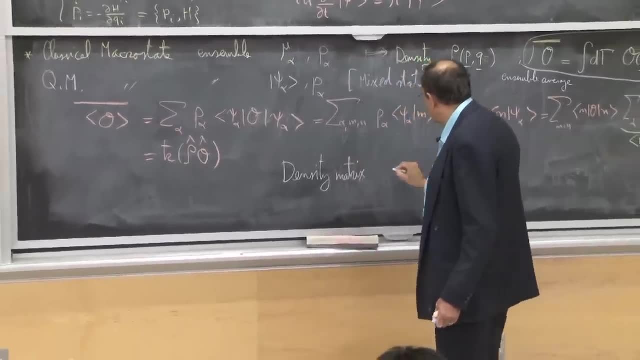 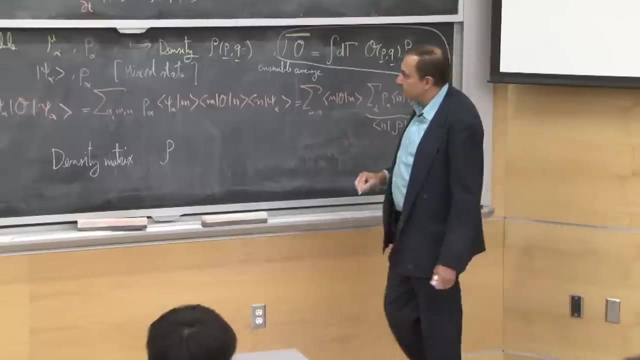 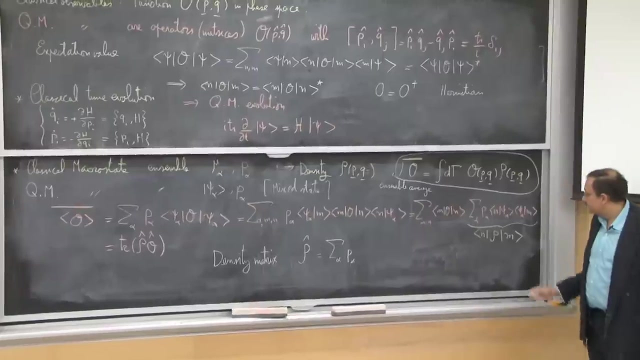 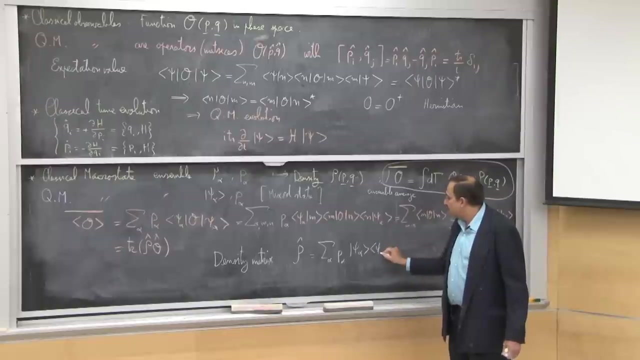 And this is the density matrix. And if I basically ignore or write it in basis, independent form, it is obtained by summing over all alphas, the alphas and essentially cutting off the n and m, I have the matrix that I would form out of state alpha. 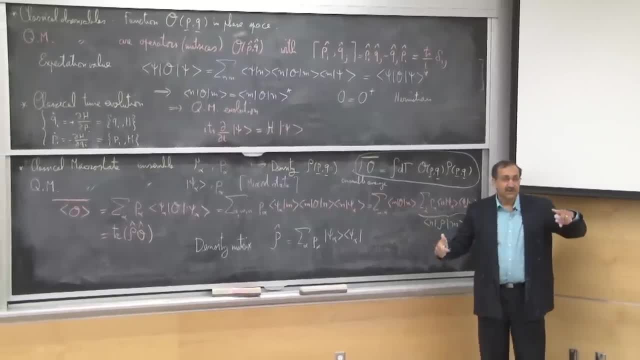 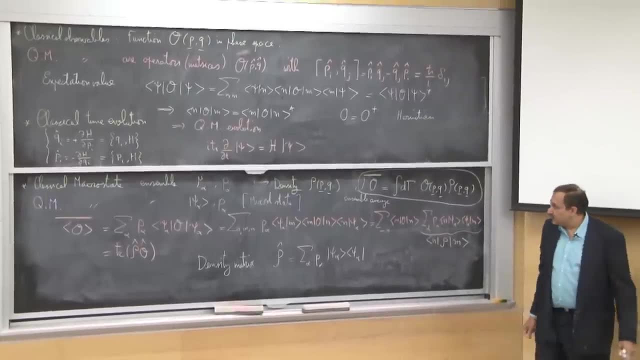 by essentially taking the vector and its conjugation- OK OK, OK, OK, OK, OK, OK. So dipping into that, they're perfectly 각 to get- and multiplying rows and columns together to make a matrix, And then multiplying or averaging. 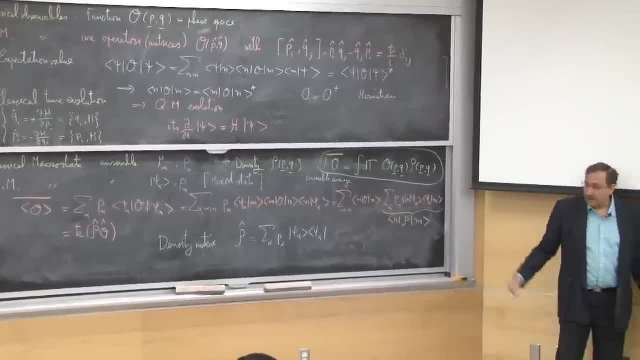 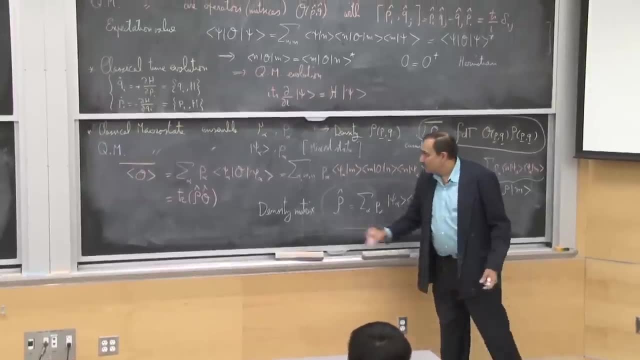 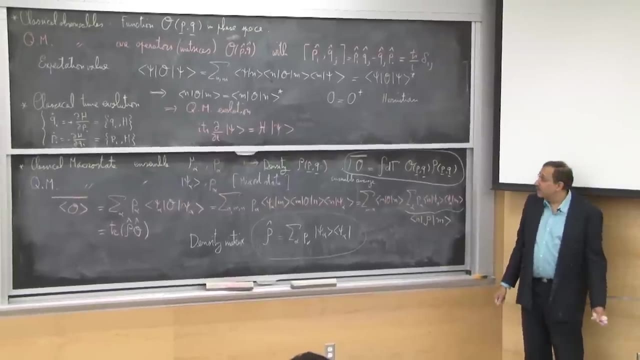 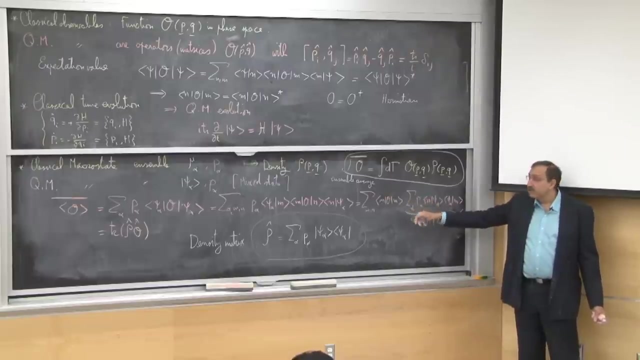 that matrix over all possible values of the ensemble, Elements of the ensemble, would give me this density. So in the same way that any observable in classical mechanics goes over to an operator, or in quantum mechanics, we find that we have another function in phase space: this density. 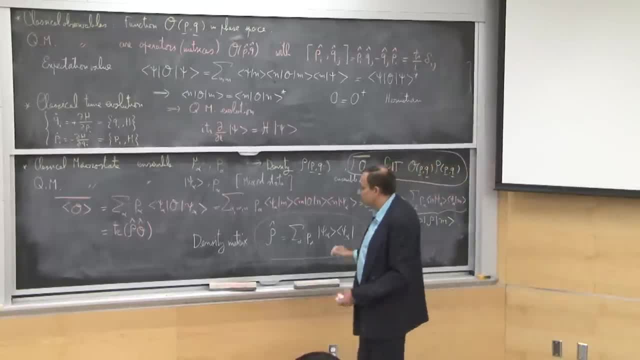 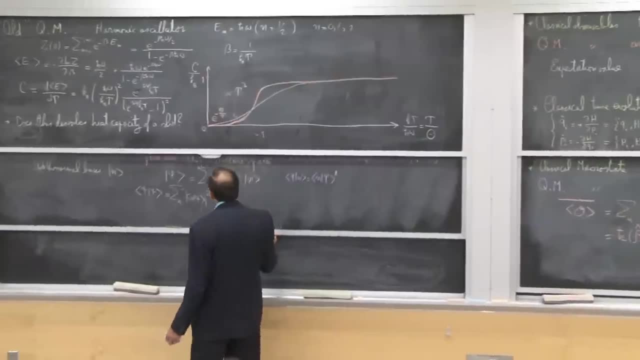 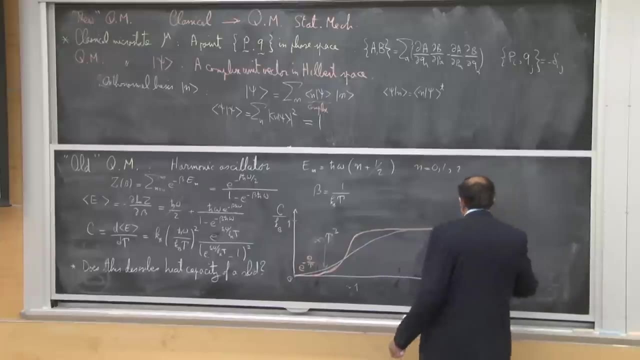 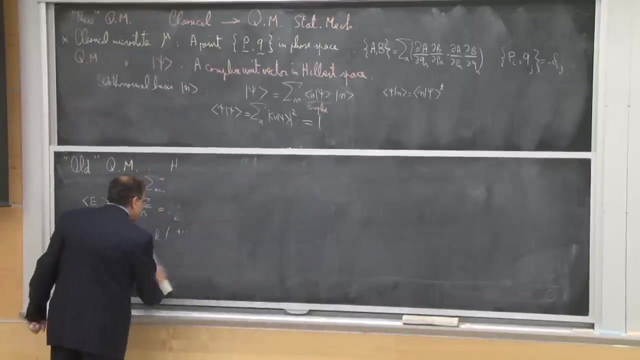 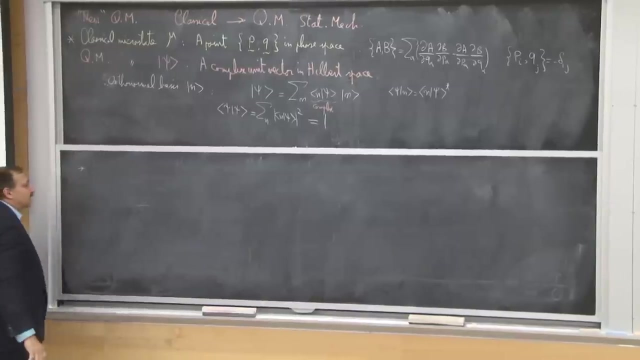 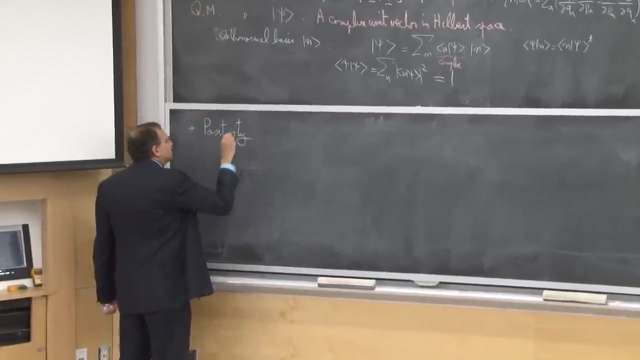 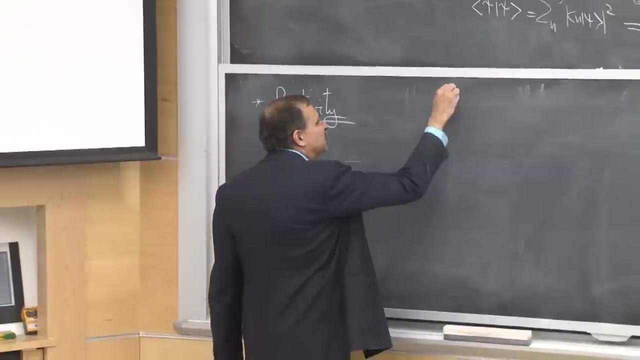 This density goes over to a matrix or an operator that is given by this formula. here It is useful to enumerate some properties of the density matrix. First of all, the density matrix is positive, definite. What does that mean? It means that if you take the density matrix, 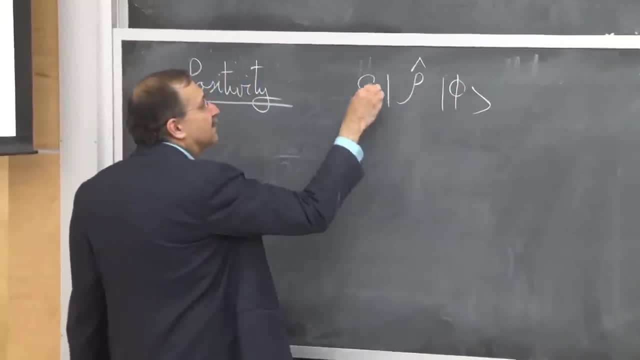 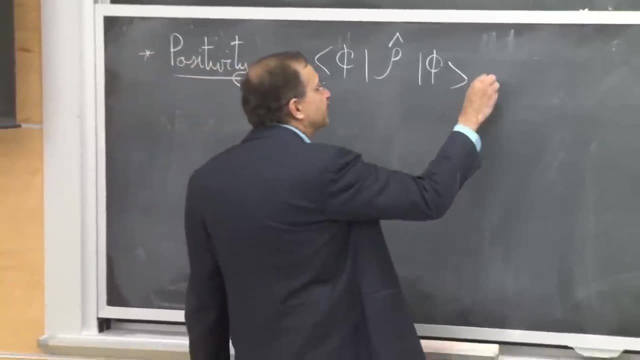 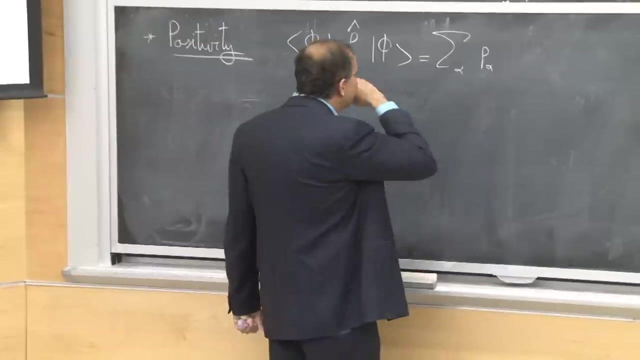 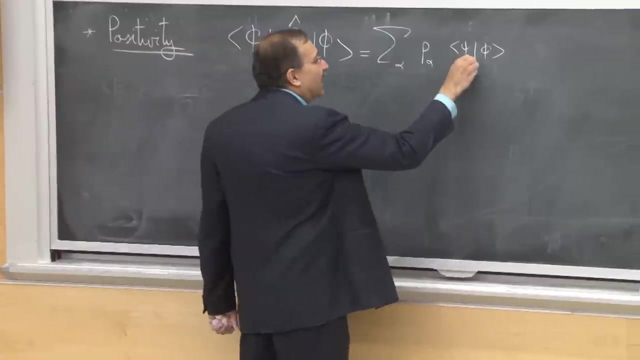 multiply it by any state And on the right and the left, to construct a number. this number will be positive Because if I apply it to the formula that I have over there, this is simply sum over alpha, p, alpha. Then I have phi, psi, alpha, and then psi, alpha, phi. 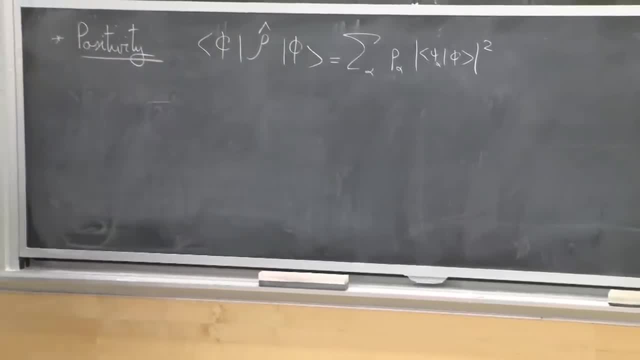 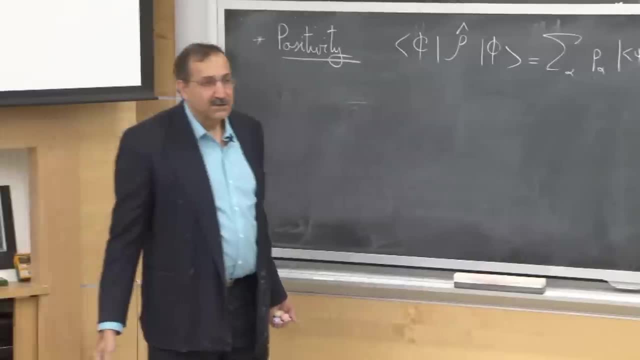 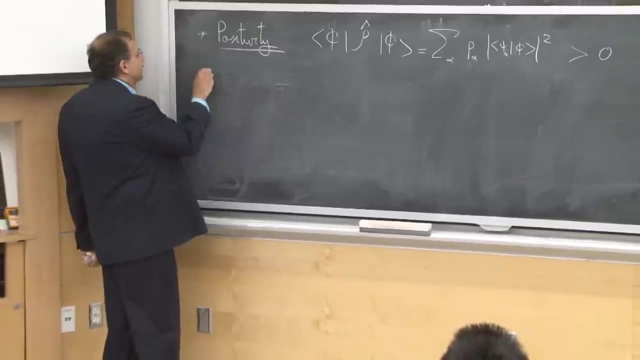 which is its complex conjugate. So I get the norm of that product, which is positive. All of phi, All of the p alphas are positive probabilities. So this is certainly something that is positive. We said that anything that makes sense in quantum mechanics. 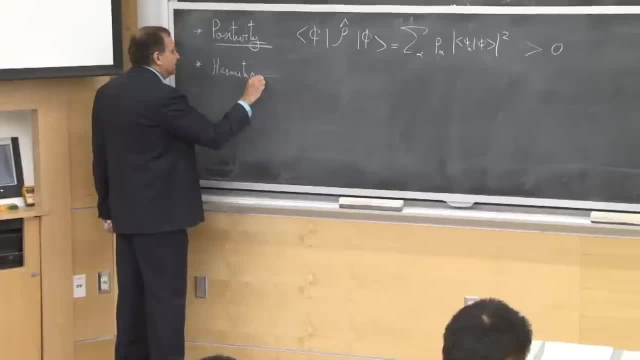 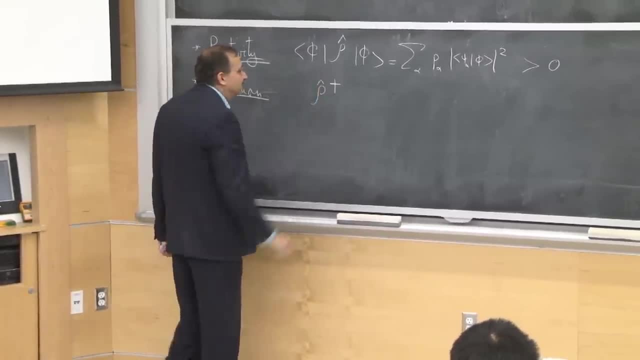 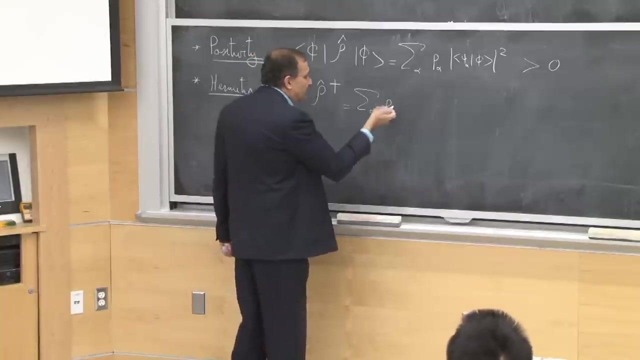 should be Hermitian And it is easy to check that. if I take this operator rho and do the complex conjugate, essentially what happens is that I have to take sum over alpha. Complex conjugate of p alpha is p alpha itself. 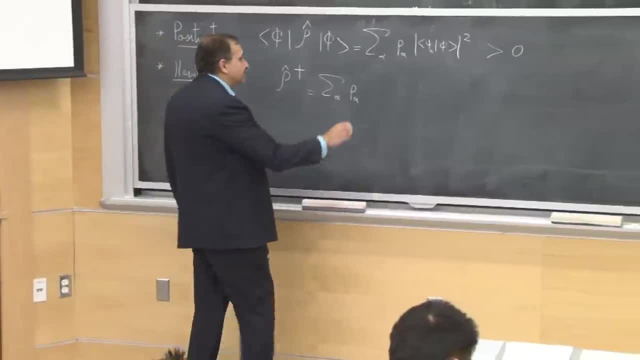 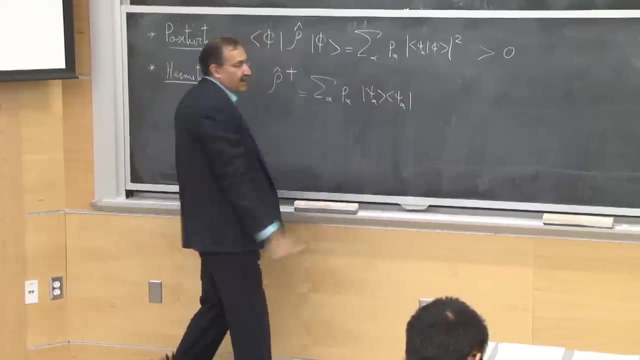 Probabilities are real numbers. If I take psi, alpha and conjugate it, essentially I take this and put it here, And I take that and put it over there And I get the same thing. So it's the same thing as rho. 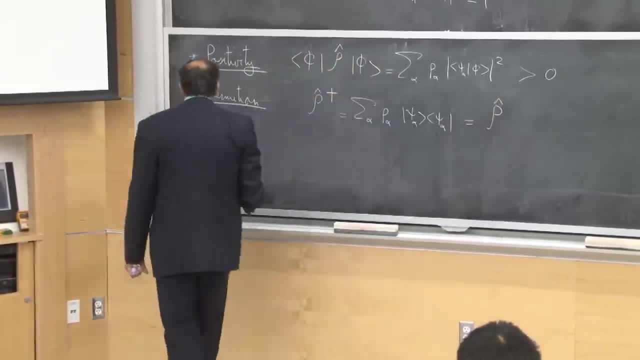 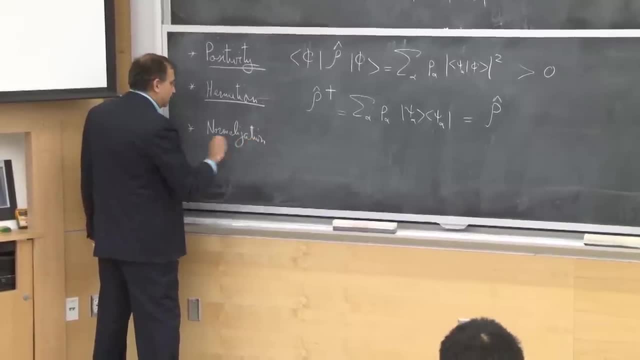 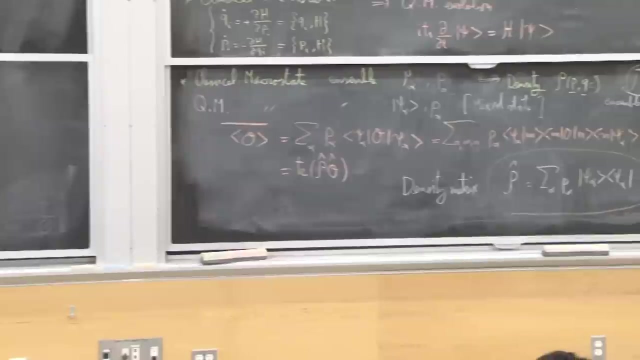 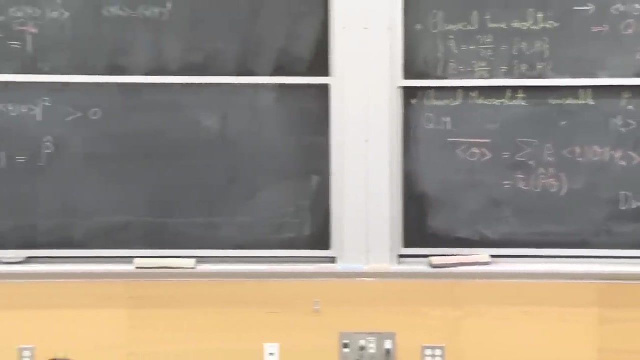 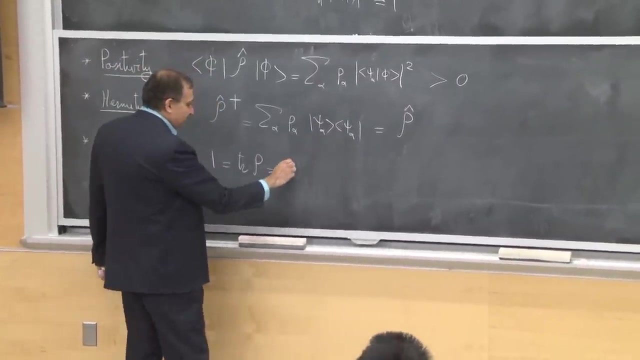 And finally there is a normalization. If for my o over here in the last formula I choose 1, then I get the expectation value of 1 has to be the trace of rho And we can check that the trace of rho. essentially. 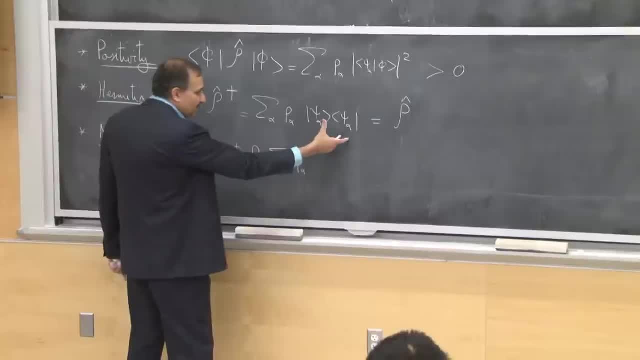 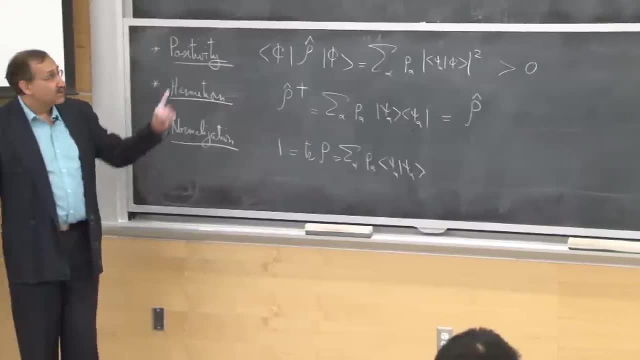 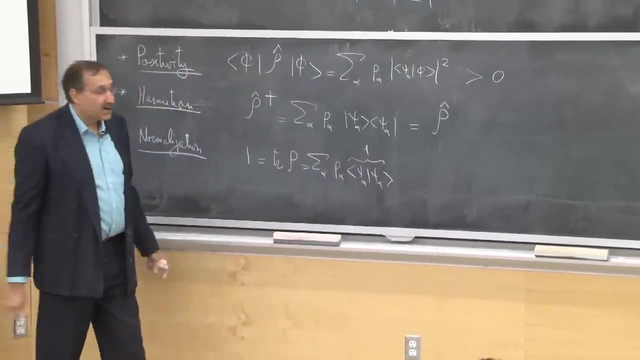 is obtained by summing over all alpha, p alpha And the dot product of the two psi alphas. since any state in quantum mechanics corresponds to a unit vector, this is 1.. So I get a sum over alpha of p alphas. 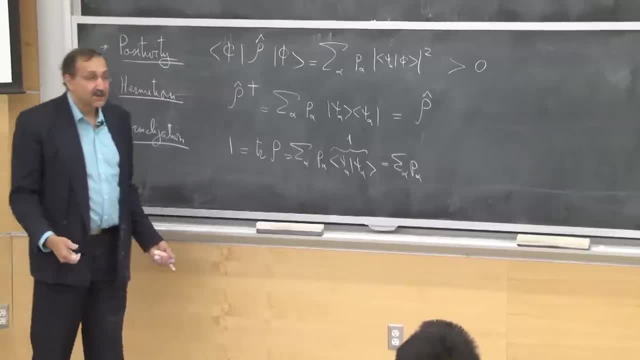 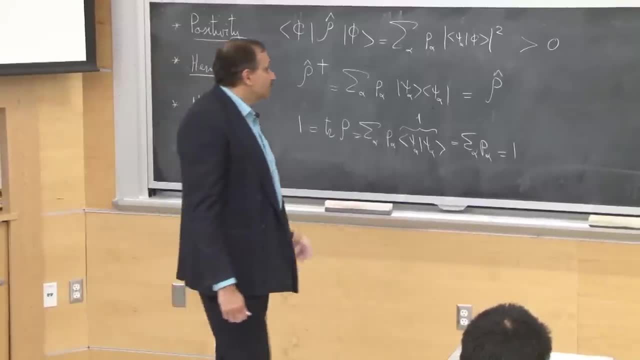 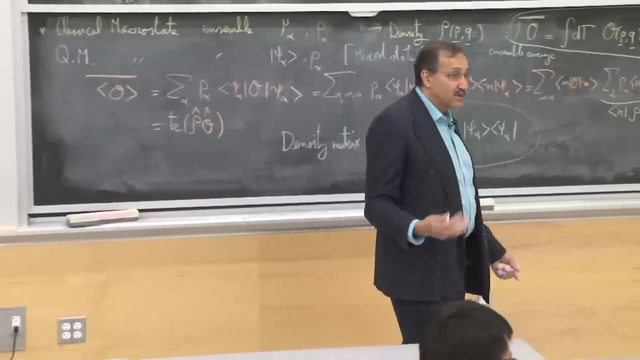 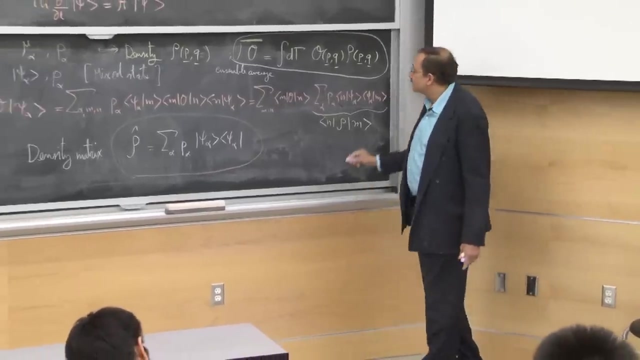 And these are probabilities assigned to the members of the ensemble. They have to add up to 1.. And so this is like this: The quantity that we were looking at and built essentially all of our later classical statistical mechanics on, is this density. 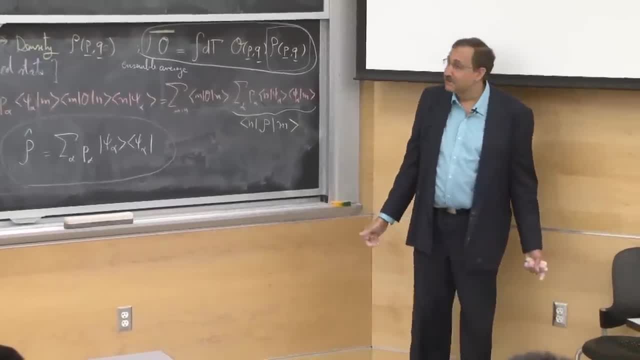 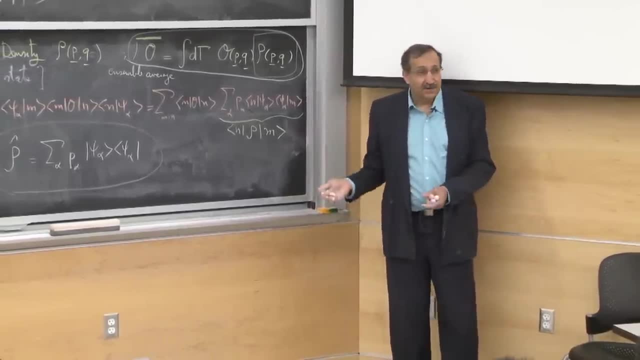 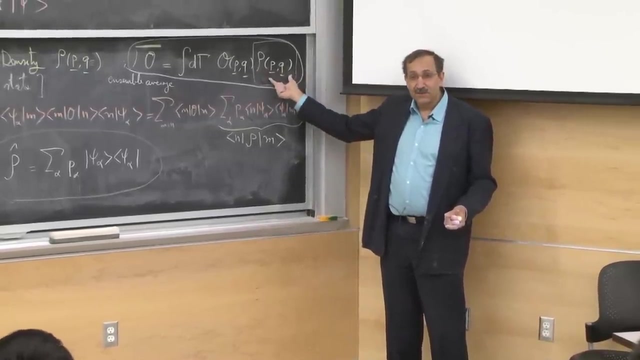 Density was a probability in phase space. Now, when we go to quantum mechanics, we don't have phase space, We have Hilbert space. We already have a probabilistic theory. Turns out that this function, which was the probability in phase space, classically 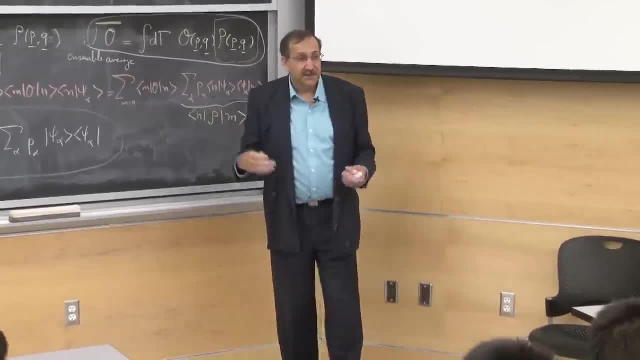 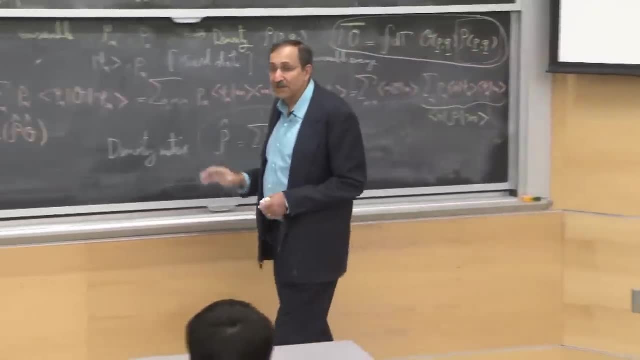 gets promoted to this matrix, the density matrix- that has, once you take traces and do all kinds of things, the kinds of properties that you would expect the probability to have classically. But it's not really probability in the usual sense, It's a matrix. 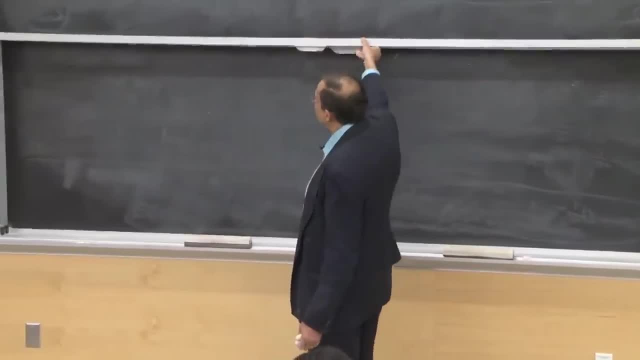 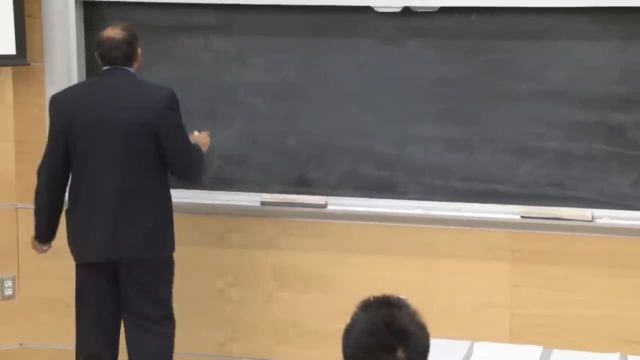 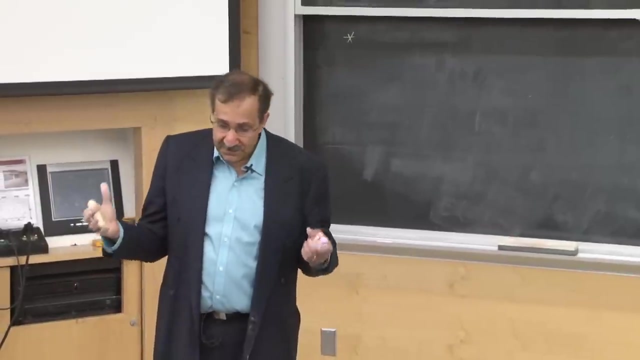 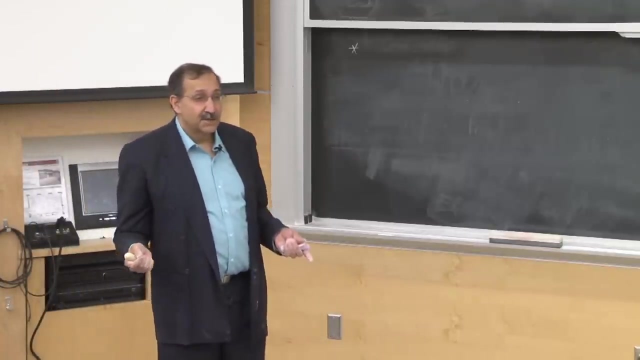 There is one other, Another element of this to go through, which is that classically we had we said that, OK, I pick a dense set of states. They correspond to some density, But the microstates are changing as a function of time. 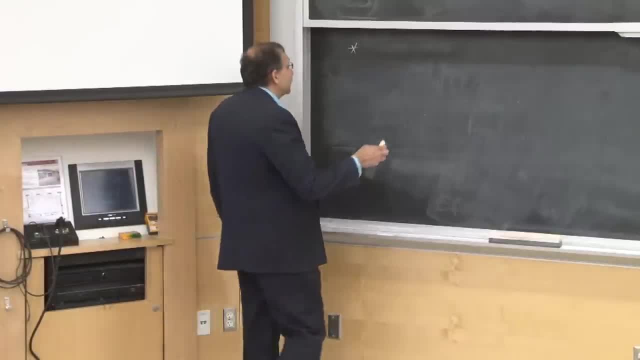 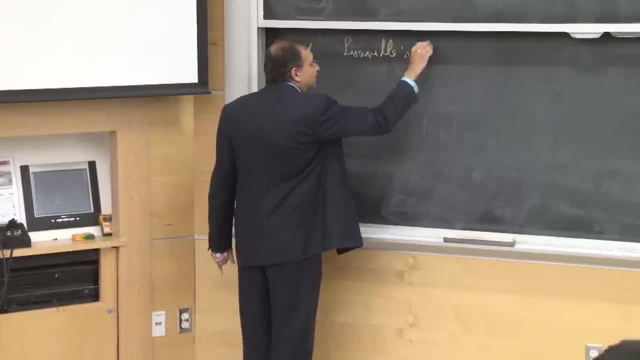 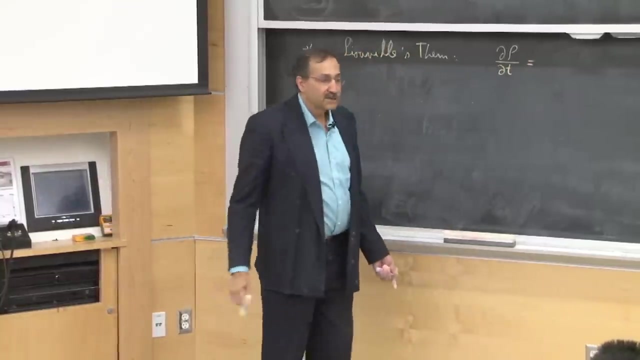 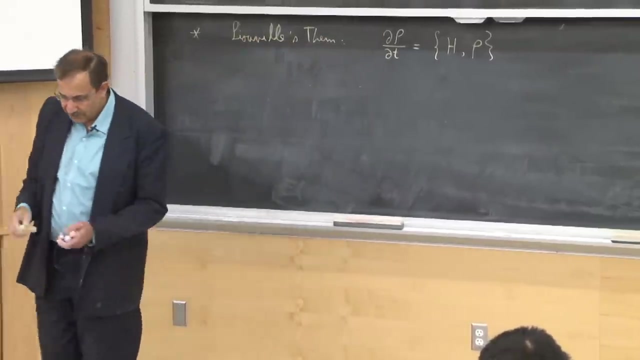 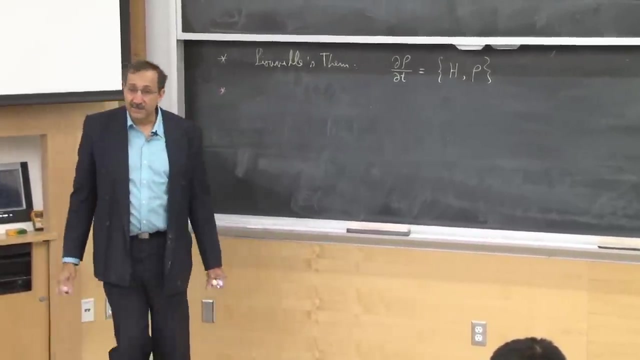 So the density was changing as a function of time And we had Neuwirth's theorem Which stated that the d rho by dt was the Poisson bracket of the Hamiltonian with rho. OK, So we can quantum mechanically ask what happens to our density matrix. 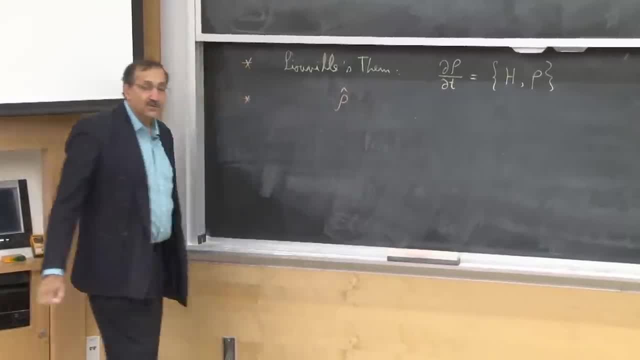 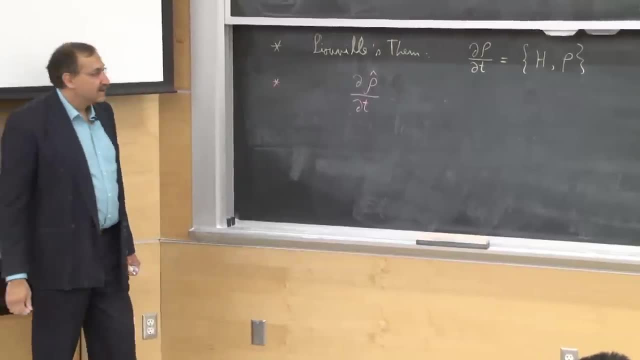 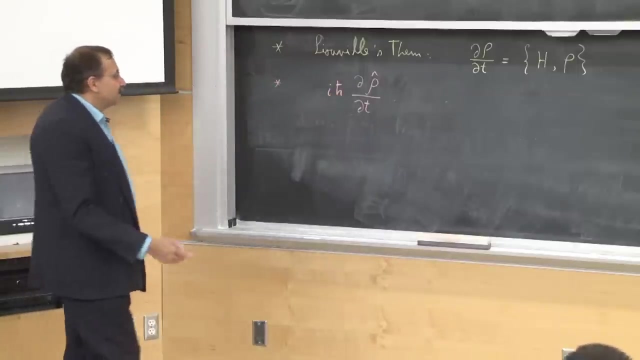 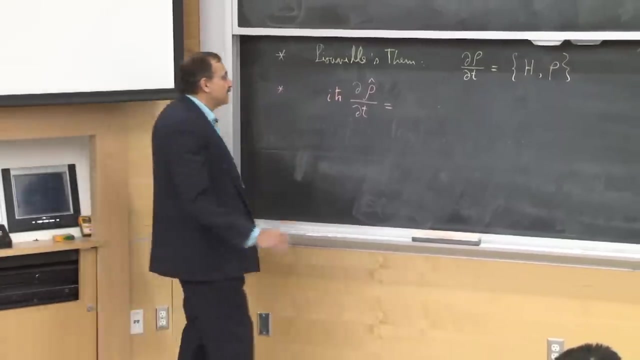 So we have a matrix, rho, I can add the density. I can add the density, I can ask what is the time derivative of that matrix? And actually I will insert the i h bar here Because I anticipate that essentially, rho having that form, what I will have is sum over alpha. 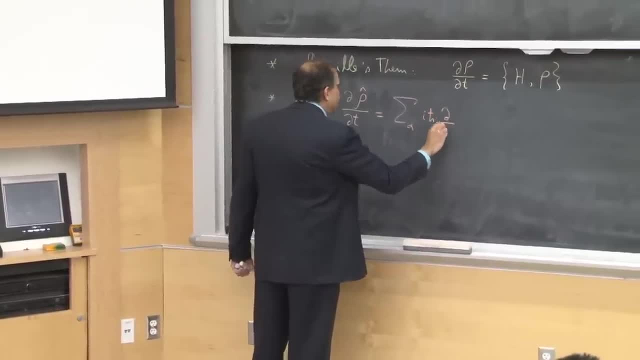 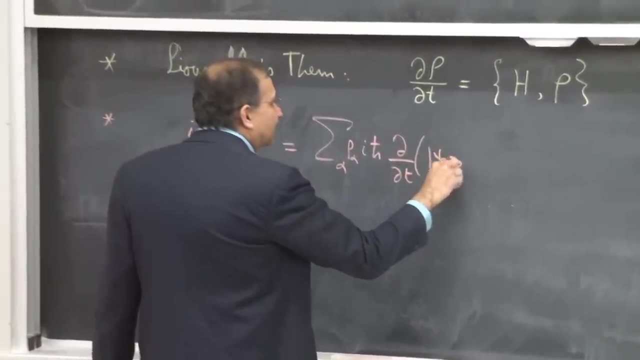 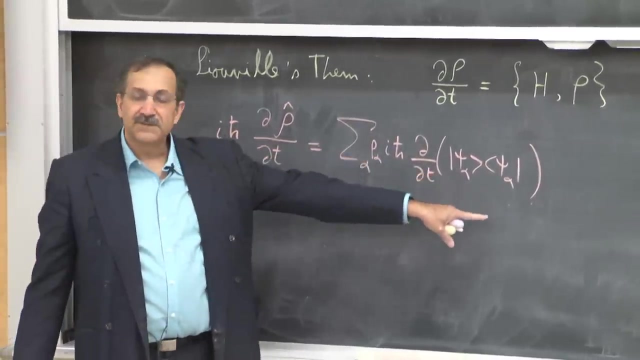 And then I have i h bar d by dt acting on these p, alpha, psi, alpha, psi, alpha. OK, So the rho is sum over alpha p, alpha, psi, alpha, psi, alpha, Sum over alpha p, alpha. I can take outside. 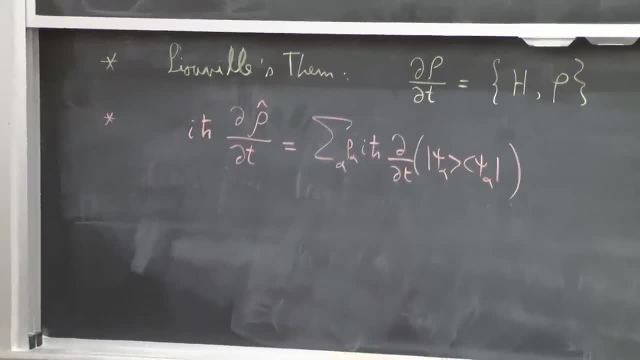 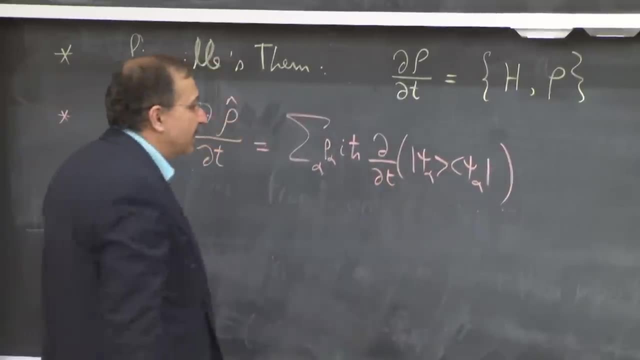 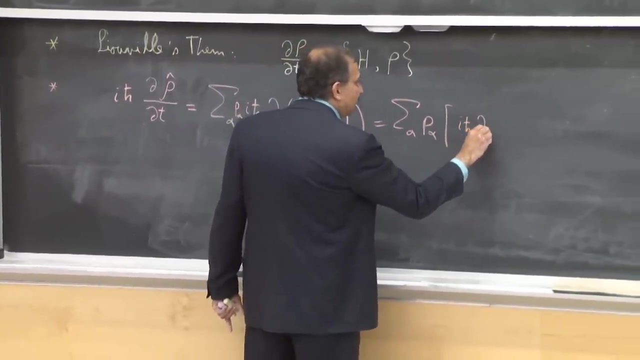 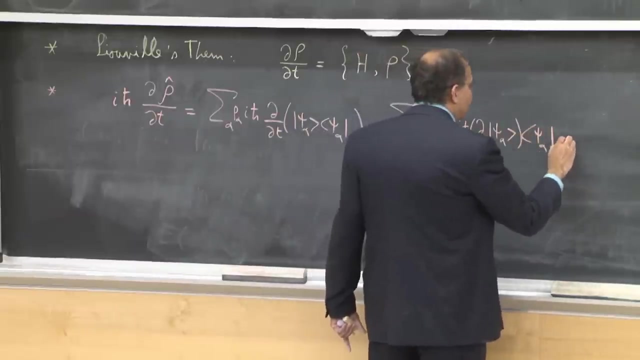 i h bar d by dt acts on these two sides that are appearing as complex conjugates. So it can either d by dt act on one or the other. So I can write this as sum over alpha, p, alpha, psi alpha, psi alpha. i h bar d by dt acting on psi alpha, or i, or psi alpha. 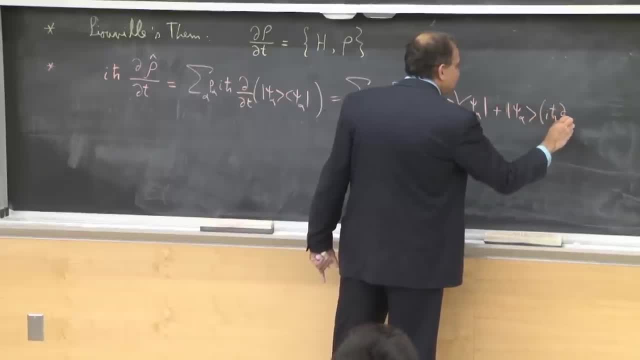 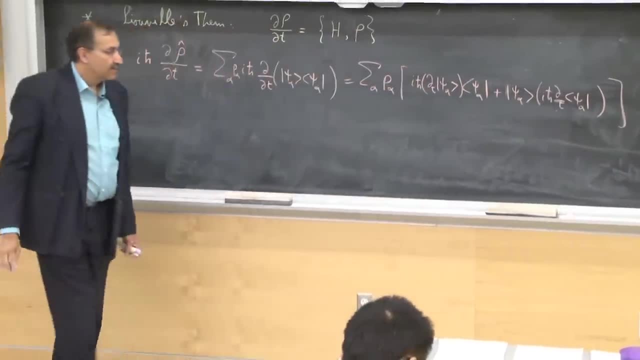 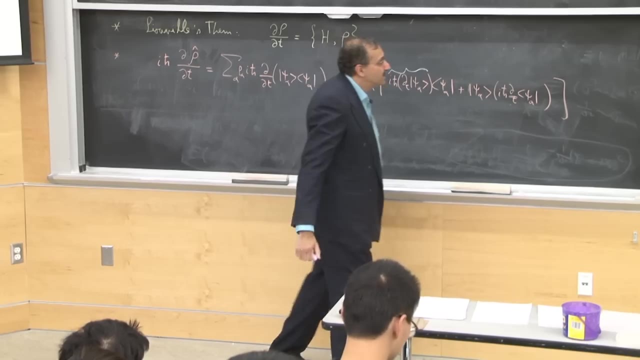 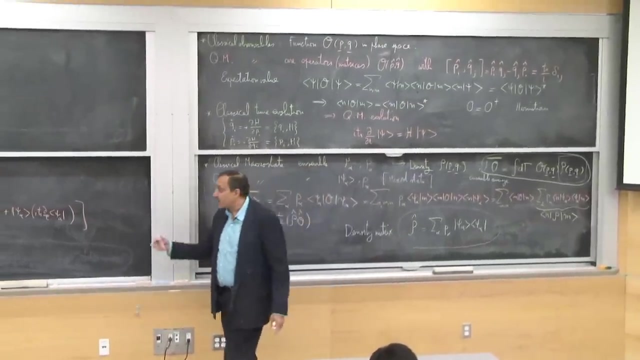 And then i h bar d by dt acting on this psi alpha. OK, Now i h bar d by dt, psi alpha. we said that essentially the classical- sorry- the quantum rule for time evolution is. i h bar d by dt of the state will give you. 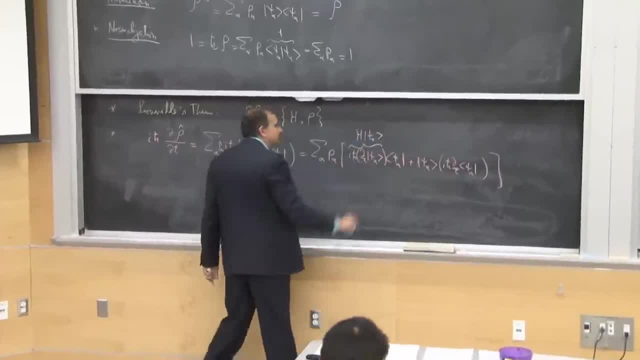 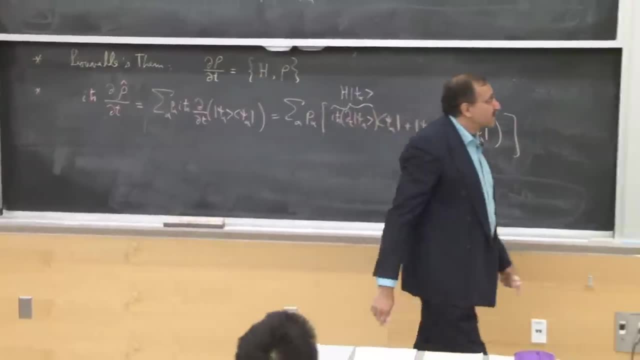 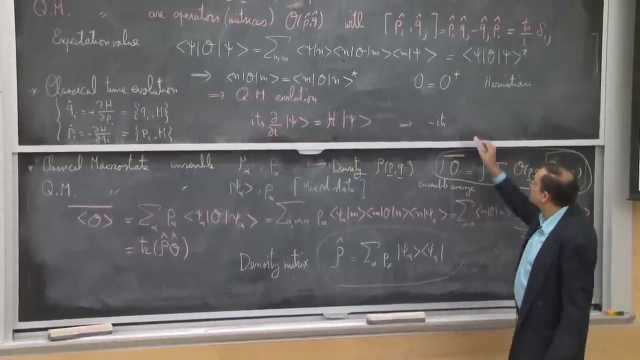 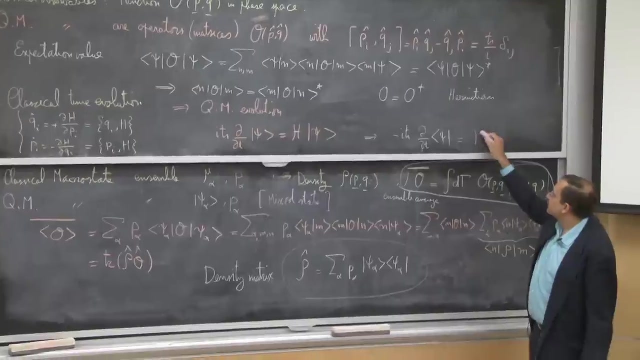 is governed by h times acting on psi, alpha. If I were to take the complex conjugate of this expression, what I would get is mu, Minus, i, h, bar, d by dt acting on psi. that is pointing the other way upon complex conjugation. 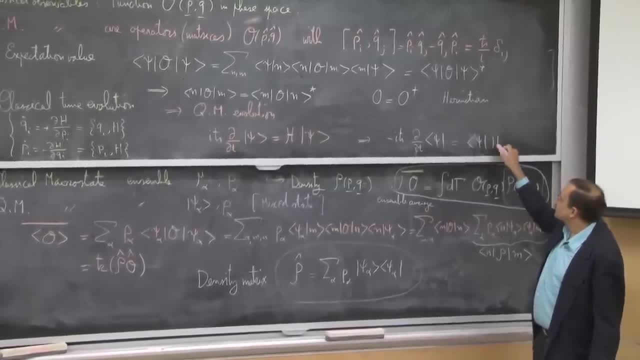 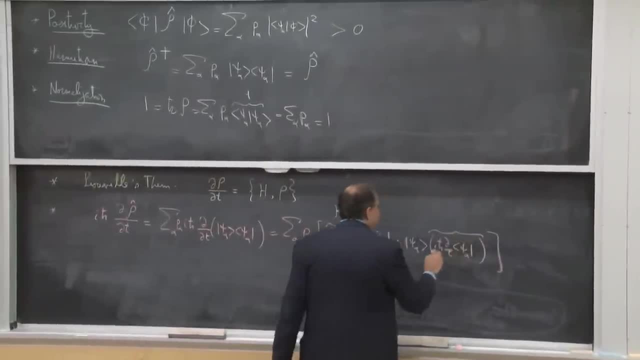 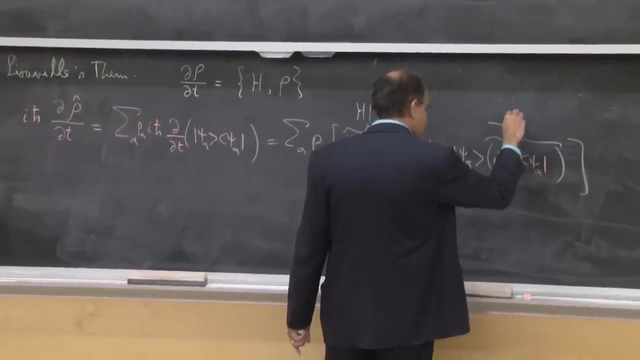 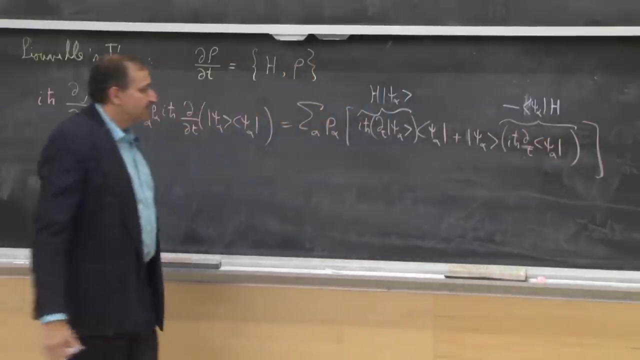 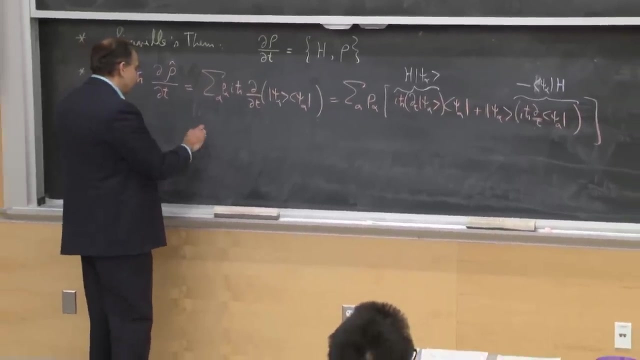 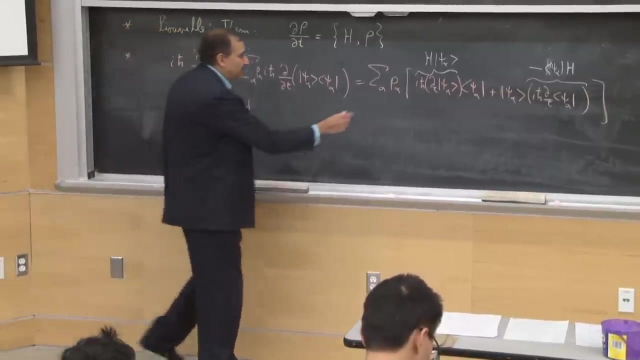 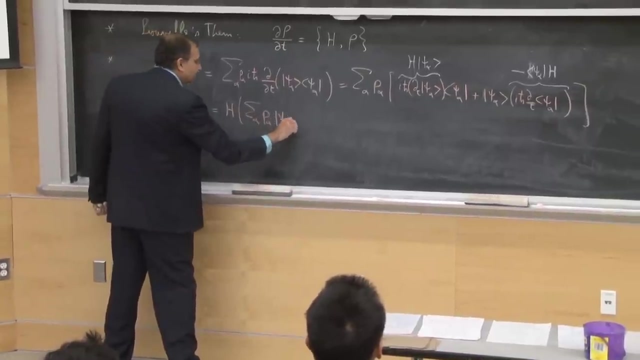 is h acting on psi in the opposite way. So this thing is minus, So i alpha, with h acting on it. OK, So then I can write the whole thing as h For the first term. take the h out front. I have a sum over alpha, p, alpha, psi, alpha, psi, alpha. 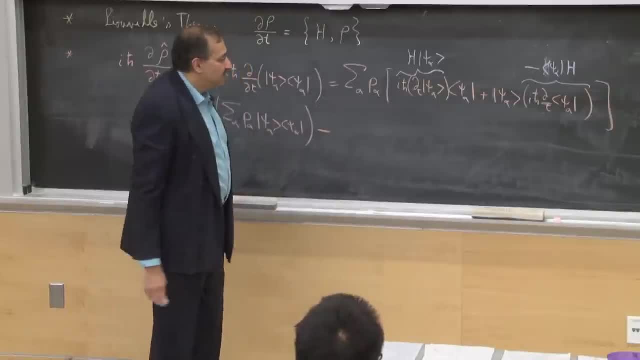 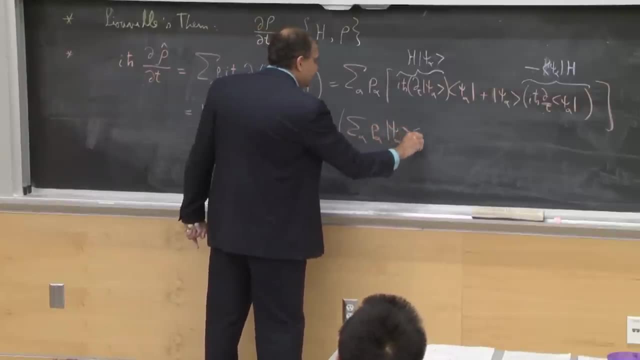 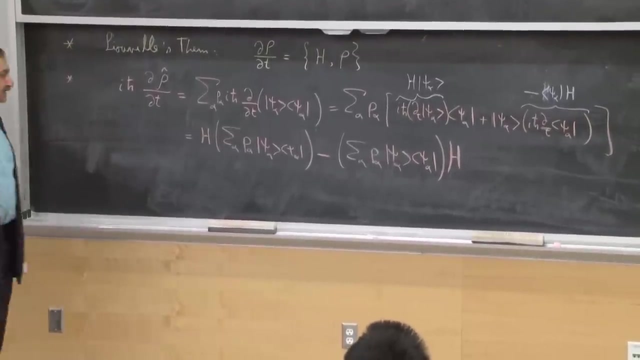 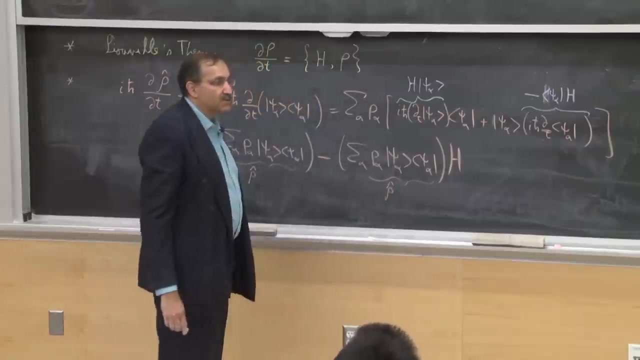 Minus from this complex conjugation. Here h is completely to the right. I have a sum over alpha, p, alpha, psi, alpha, psi, alpha, And then we have h. Now these are again getting rho back. So what I have established is that i h bar d by dt right. 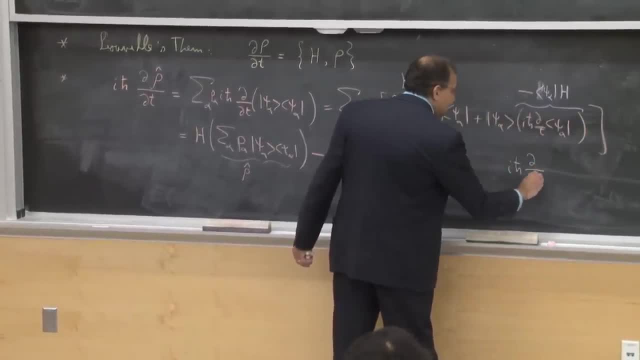 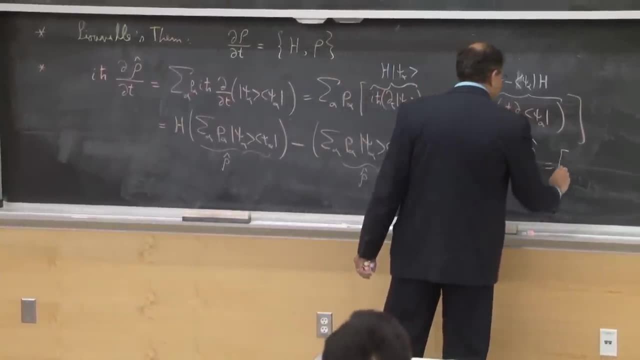 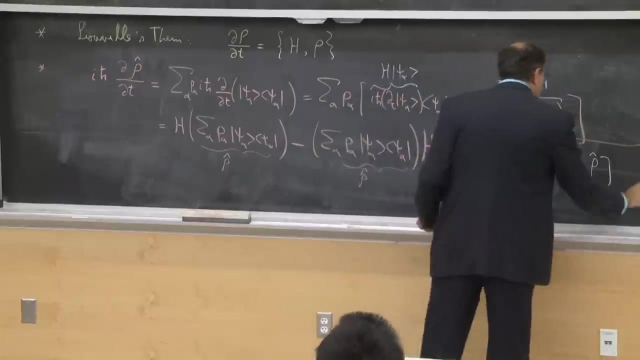 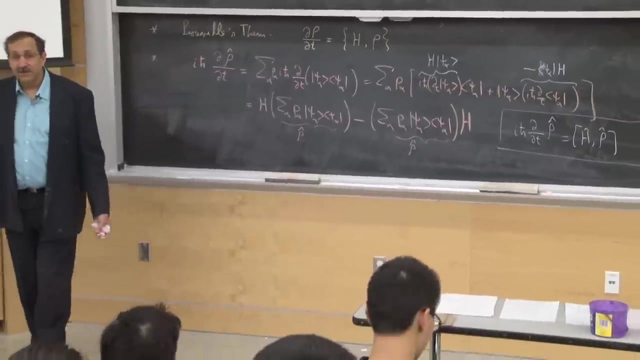 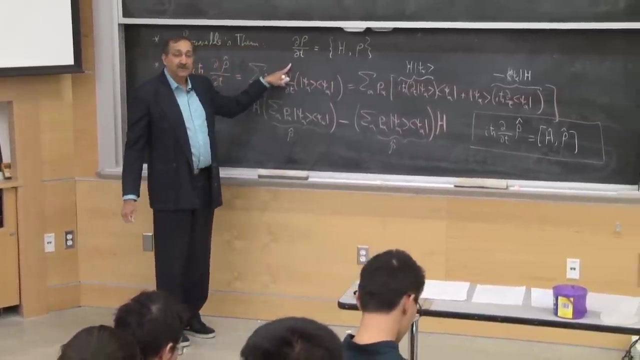 OK, OK, So i h bar. the time derivative of this density matrix is simply the commutator of the operators h and rho. So what we had up here was the classical Liouville theorem, which is equating the time derivative of the density. 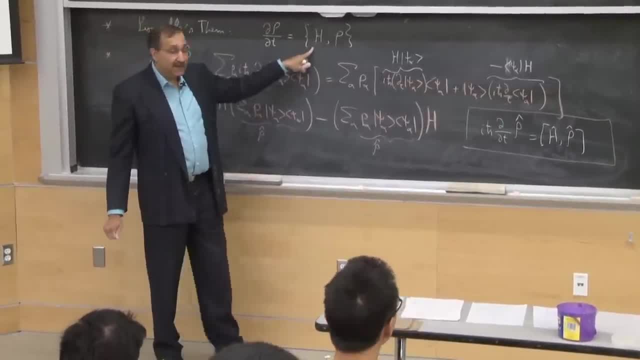 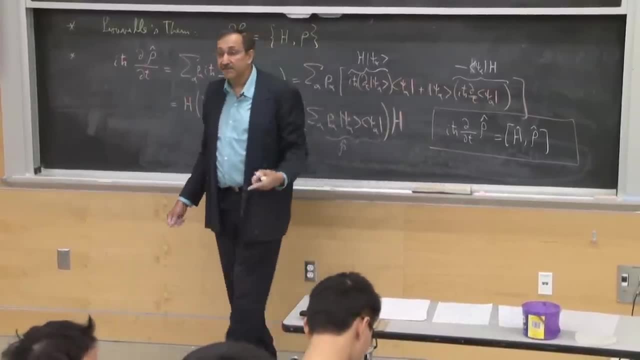 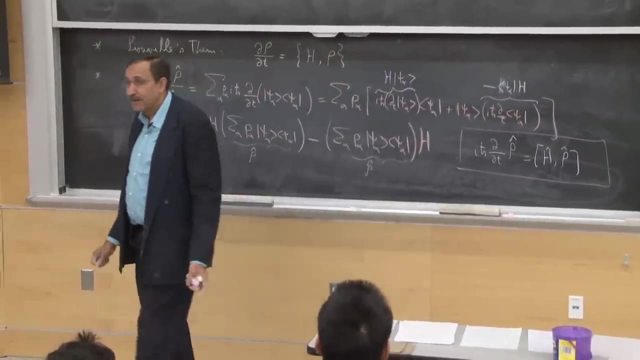 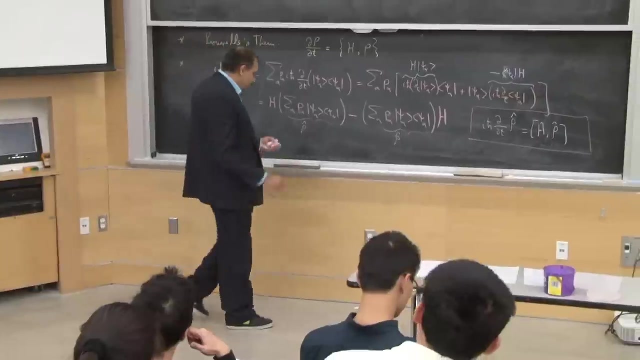 in phase space to the Poisson bracket with h. What we have here is the quantum version, where the time derivative of this density matrix is the commutator of rho with h. Now we are done, Because what did we use this Liouville theorem for? 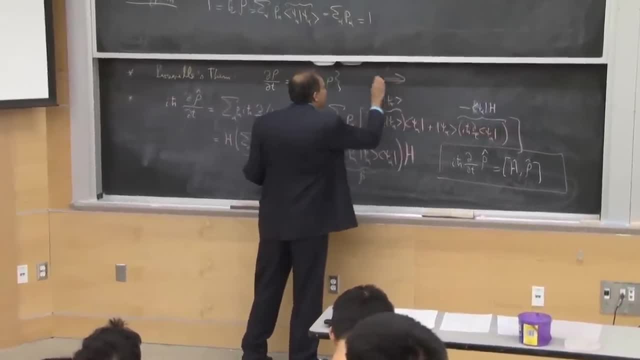 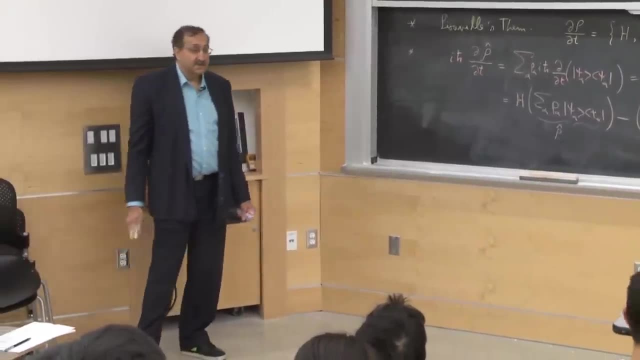 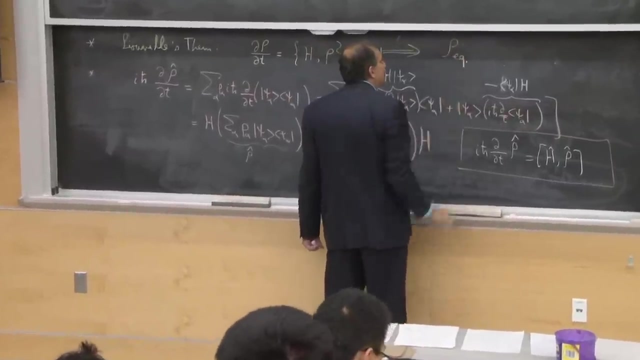 We used it to deduce. We deduced that if I have things that are not changing as a function of time, I have equilibrium systems where the density is invariant. it's the same then, rho of equilibrium not changing as a function of time. 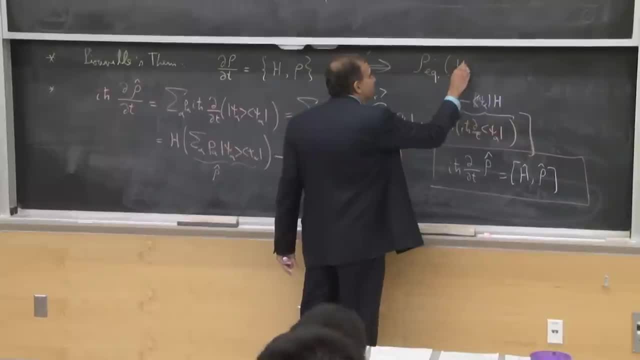 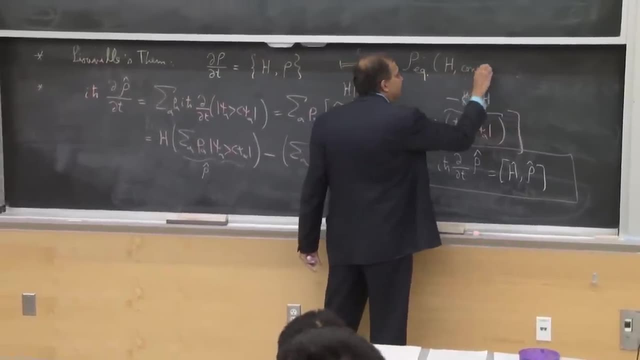 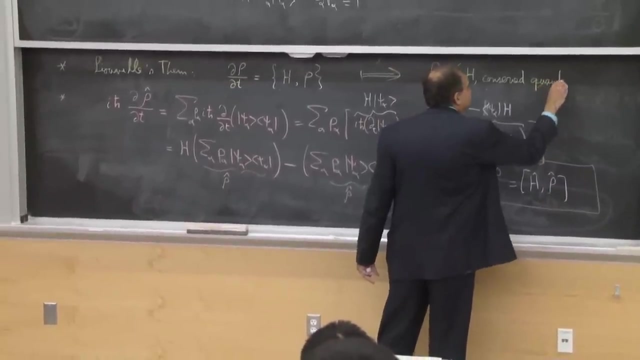 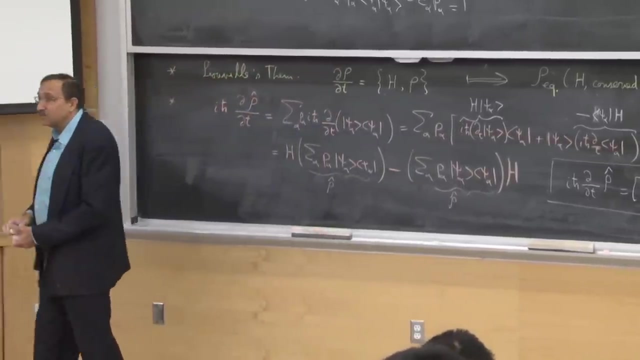 can be achieved by simply making it a function of h, and more precisely, h and conserved quantity. OK, Conserved quantities that have 0 Poisson brackets with h. How can I make the quantum density matrix to be invariant with time? 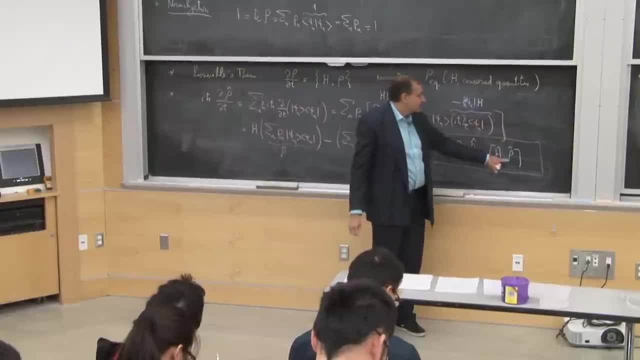 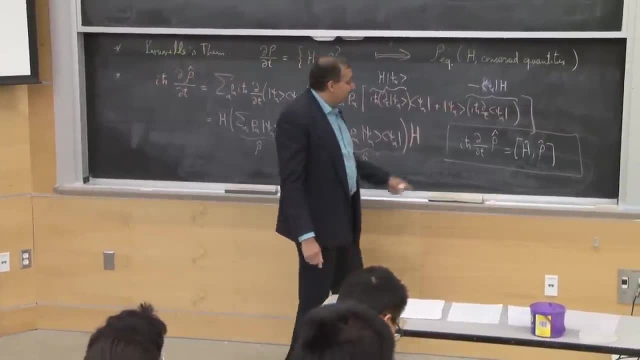 All I need to do is to ensure that the Poisson bracket of that density with the Hamiltonian is 0, not the Poisson bracket, the commutator. Clearly, the commutator of h with itself is 0.. hh minus hh is 0.. 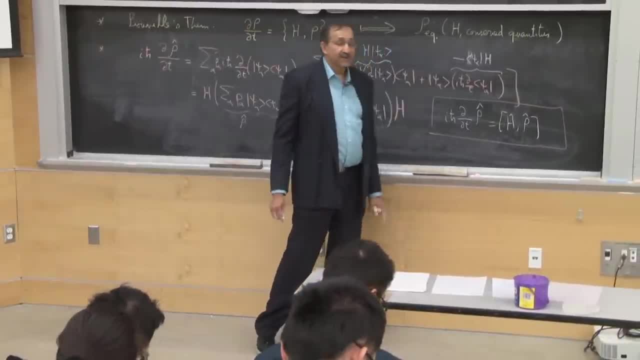 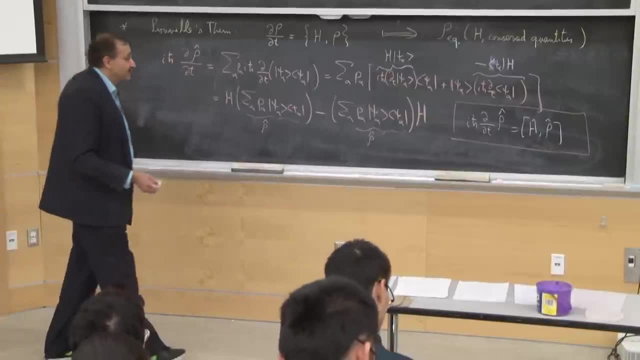 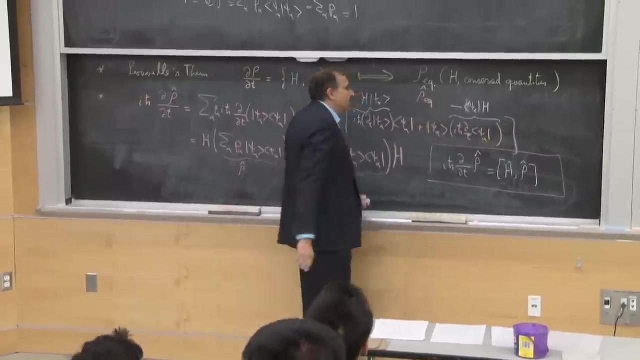 So this I can make a function of h And any other quantity also that has 0 commutator with h. So essentially the quantum version also applies. That is the quantum version of rho equilibrium. I can make it by constructing something. 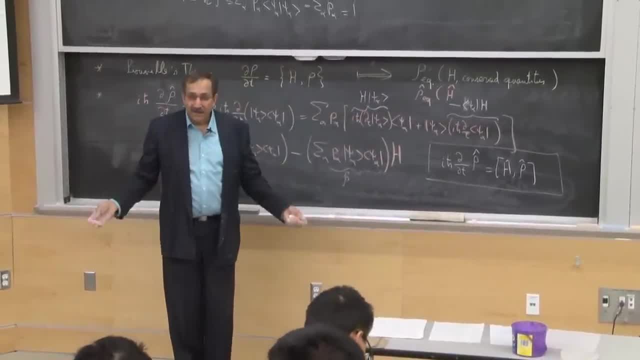 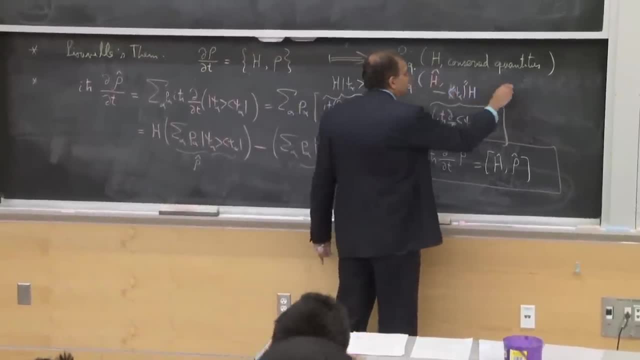 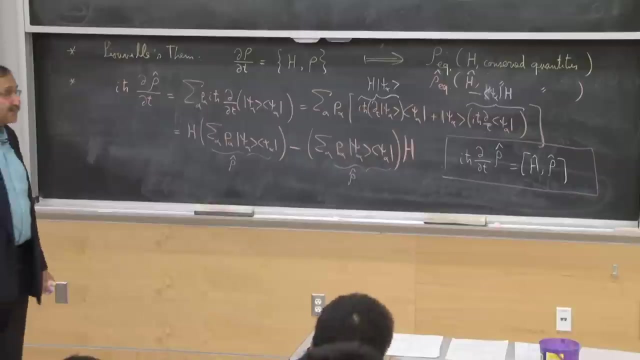 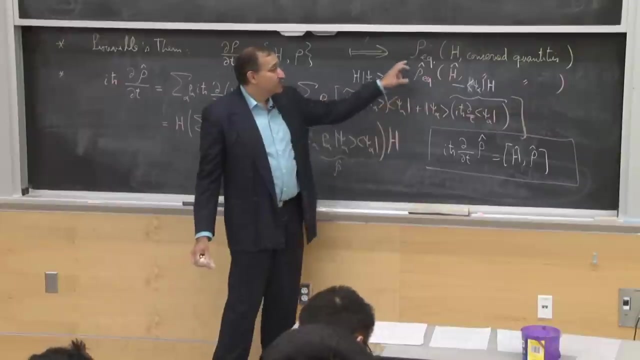 That depends on the Hilbert space through the dependence of the Hamiltonian on the Hilbert space and any other conserved quantities that have 0 commutator, also with Hamilton. OK, So now, what we will do next time is we can pick and choose whatever rho equilibrium we.